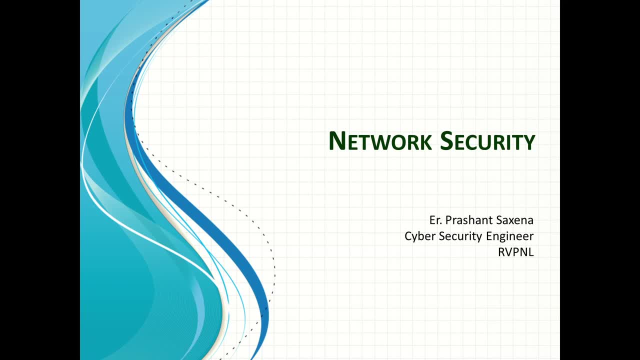 Okay, So Correct. So try to mingle up with the structure And I am assuring you that you are lucky to have such a great platform of CBIP and definitely at the end of the session we will talk and we will find that you are on a very, very good pace. 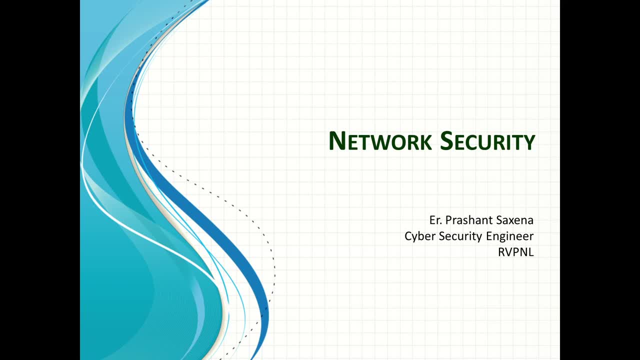 Okay, So that's not an issue, So rest assured about it. Okay, So we will be talking about network security. Again, I will be talking something you already know, but to To conclude my today's discussion, I need to prelude the topics also, so that I can have a better overview to you people. 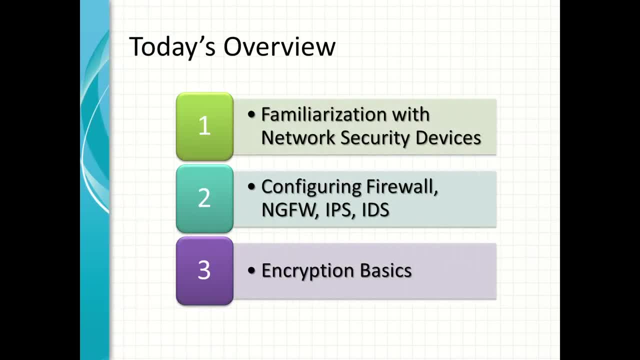 Okay, So today we will be talking about the familiarization with network security devices. Probably you will ask, Thinking that you have already discuss about firewall, IPS, IDS, but today we are going a little bit deeper into it. today we will be talking about host based firewall, network based firewall, and I have especially deployed 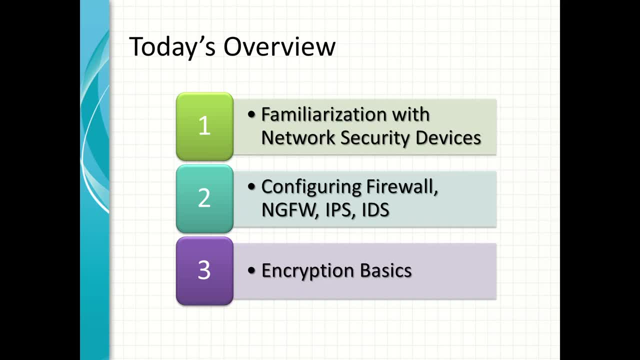 a firewall at my home today and I will be showing to you live demo of my in-house firewall. about the zoning, about the creating the rules and all so and after that we will be talking about IPS and IDS. then we have a very good IPS IDS SNOT. I think some people are knowing about it, so we are. 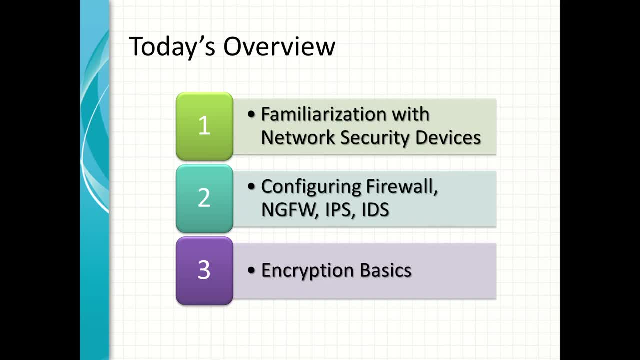 going to configure it and we are going to create some rules in that SNOT and after that we will be talking about encryption, and in encryption we will be talking about symmetric, asymmetric encryption. then we will be creating the GPG keys by installing the you gnu gpg software and then uploading it to the pki public key infrastructure. so this is the 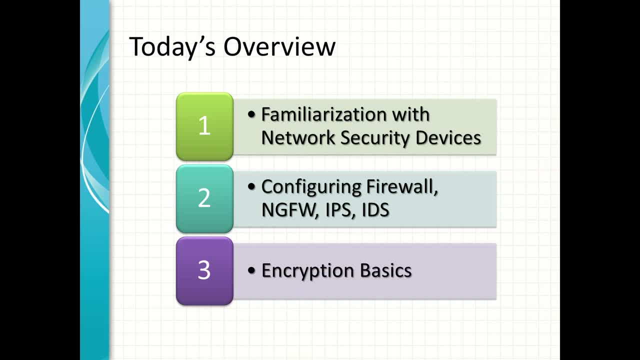 target that I have taken down. I think the class is of three hours, now 10 to 1, as per your schedule. yes, yes, yes, yes, yeah. so if you don't mind if I take a half an hour more because there is a lot of things I need to cover, okay, okay. so this is about today overview and 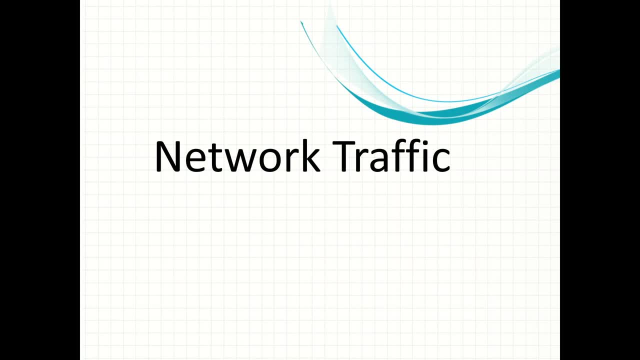 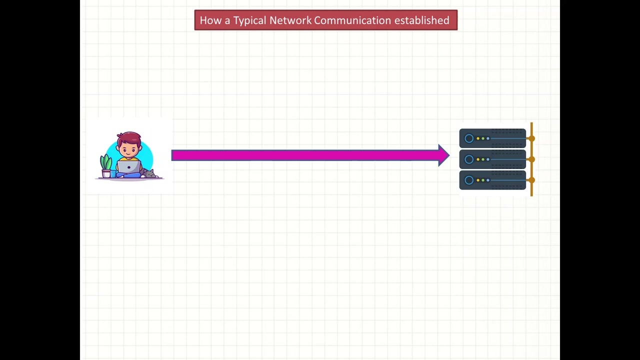 let us start this class signal. oh, okay, so what is a network traffic? how a typical Network communication established? okay, so just think of a scenario with this is a person- this is a kid actually- and he is a trying to communicate, uh, with some server. okay, any server, maybe it is a Google or something like that division, okay, so 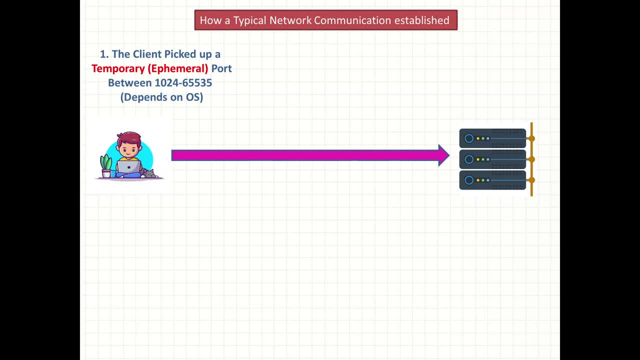 or something. to establish this communication he need to send a data packet, and for sending the data packet he need to have a ip address and a port address. okay, so to send a data packet he need to pick a ephemeral port or a temporary port between the ports 1024 and 65535, why i have put. 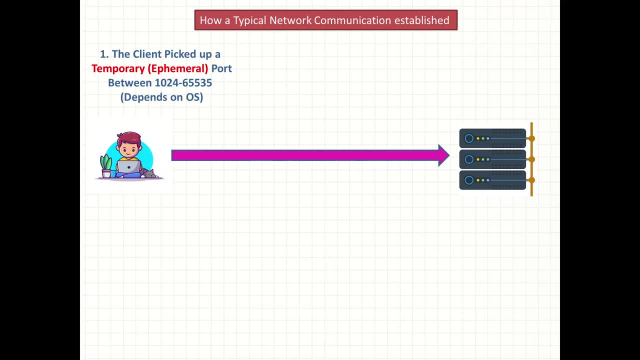 down especially this port number in front of you, because the total number of ports in a system are zero, two, six, five, five, three, five and zero, two, one, zero, two, three ports are reserved ports. okay. so whenever a communication established the target ports are from the zero to one, zero, two, three, if 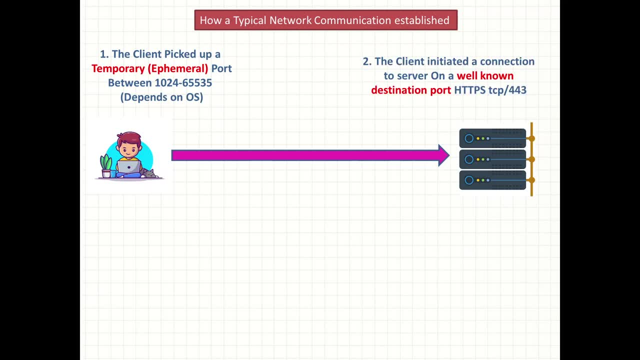 they are not specified. okay, so a client pick up an ephemeral port and also a client initiated a communication to server on a well-known destination port. uh, probably it is https on tcp protocol on port 443. okay, so this is a communication which we are going to discuss, so every communication is basically having two parts. 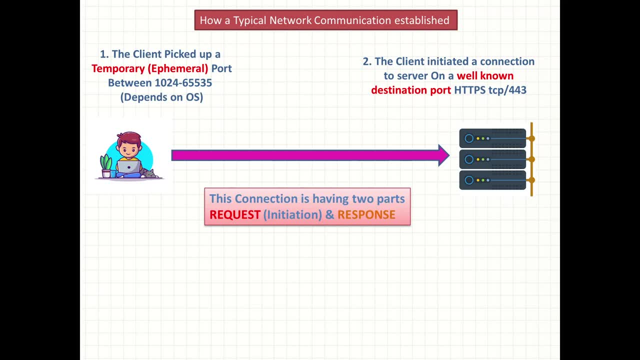 one is a request, the one who is using: yeah, anybody's saying okay. so every uh communication, every connection is having two parts. uh, one is a request part and other one is a response part, big. without response and request, uh, one cannot establish a communication because when you have seen the tcp id, the client is sending a sin request and the server is sending. 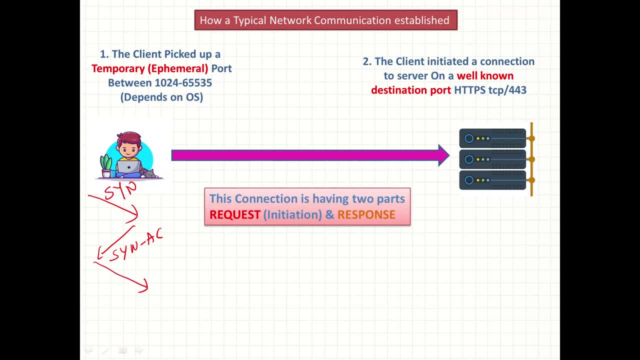 a synac request and for com confirming uh the communication, the client is again sending the accurate quest. so this is a typical uh communication in the tcp ip. okay, so this communication is having two part uh request. the first is a request and second is a response. okay, 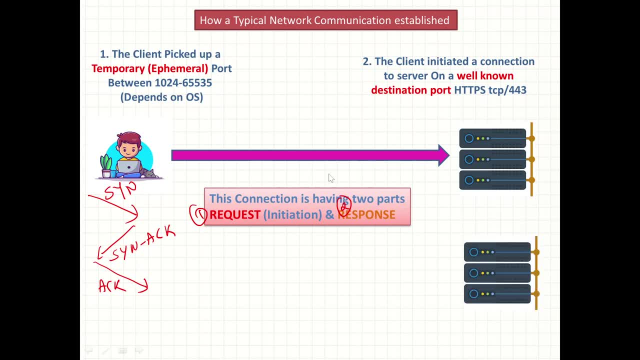 why i am telling you i will. you will, uh, going to let it know after a few minutes. so once a server received a request to communicate, it will again reply back to the client. get, sir, i have received a request and it is basically. uh, we have seen that this is a request. 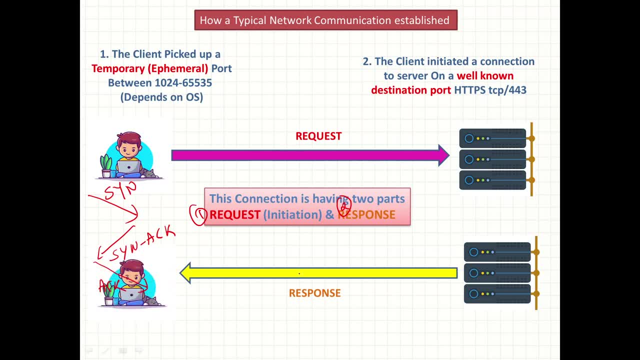 that is done by the person and this is the response that is given by the server. okay, now the client has received the, the required material he used to have. okay, so this is a very, some simple communication where, uh, one person is talking to the other server and server is returning back. so 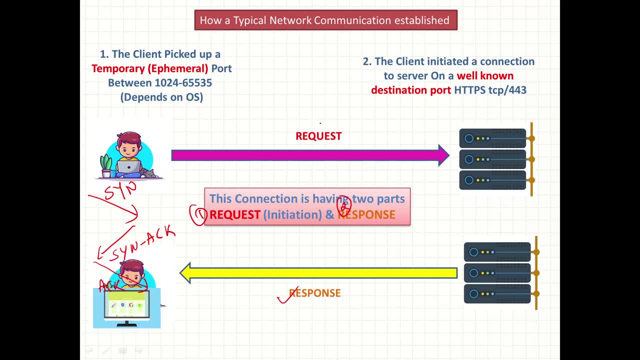 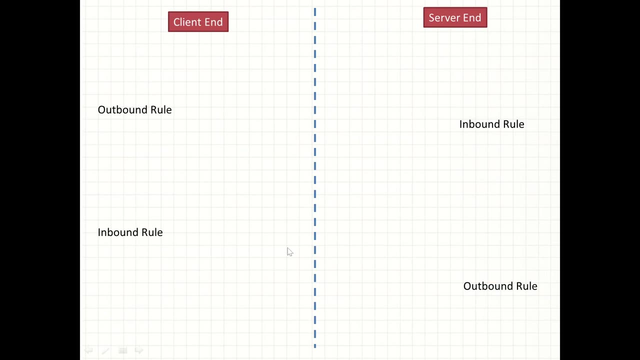 what is going to uh important in this part is request and response. so just keep in mind till now that for every uh communication a request and response is very much required. okay, now uh think of uh sorry, yeah, please sorry. can you repeat, repeat again on the port numbers what it will like? 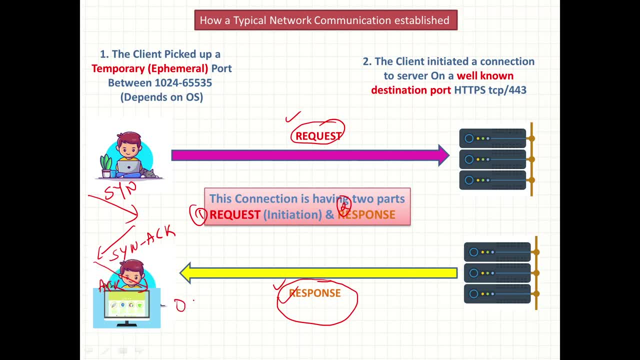 to be between one zero, two, four, two, six, yeah, yeah, actually there are total ports between zero to six, five, five, three, five. sixty five thousand five hundred thirty five are total number of ports. okay, and zero, two. one, zero, two, three are reserved ports, reserve ports, which includes your tcp port. 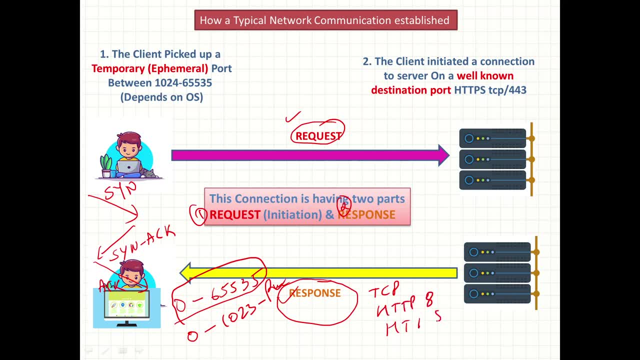 your http, uh, that is 80. your https, that is four, four, three. okay, your ftp port, your telnet port. so these are the reserve ports between zero to one, zero, two, three and above zero. from one zero, two, five, three, five are ephemeral ports or you can say temporary ports. your system can pick any port. 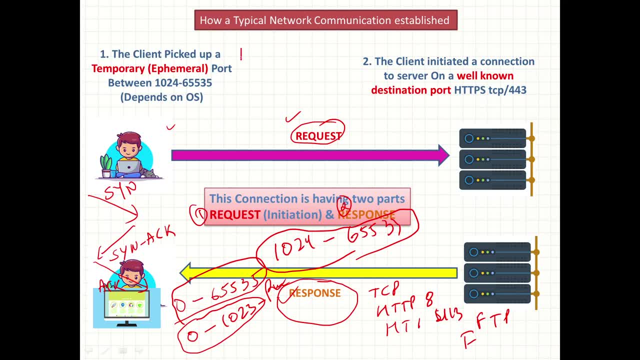 to communicate with the other server. okay, so if mr a is sending a request to mr b, so he will be using port 1024265535. when you see the ip, when you see the tcp ip packet, and in the uh layer, uh four, you will see the ports. in the osi model layer three, you will see the ports. you will see, uh, the port. 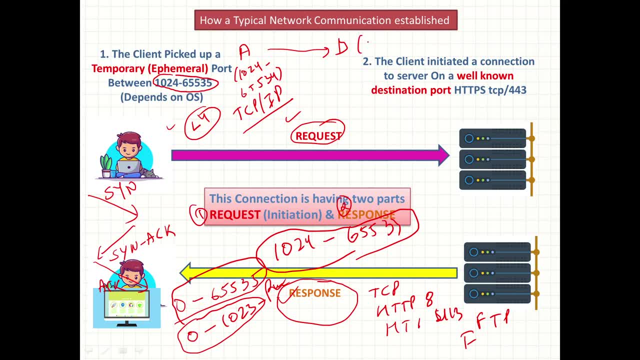 of the sender is this, and the receiver port is usually from zero to one, zero, two, three, because you are trying to connect to some, uh, well-known destination. because if you are trying to do ftp, you have a dedicated port. if you are trying to do telnet, and you have a dedicated port. okay, so is it? 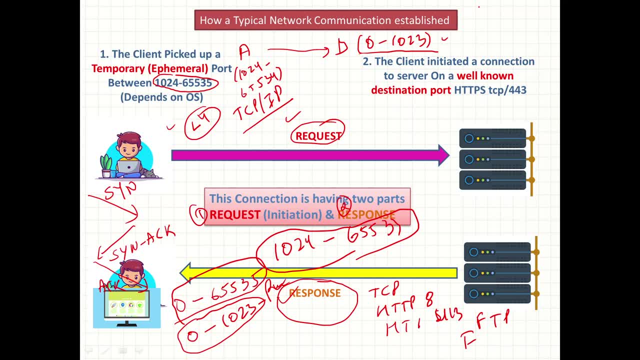 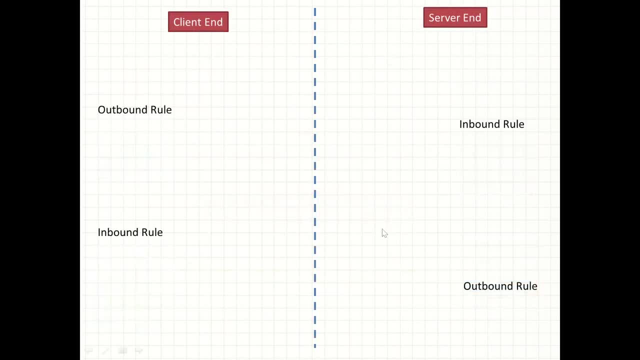 clear, sir. yeah, it's clear. thank you, yeah, thank you. so just focus on that. for every communication, you need a request and a response. okay, so now uh talk, uh. i'm talking, uh, about a typical client and servant communication. let this uh sit, child sit again. and this is our server on which we are working in the last slide. okay, so we have seen each. 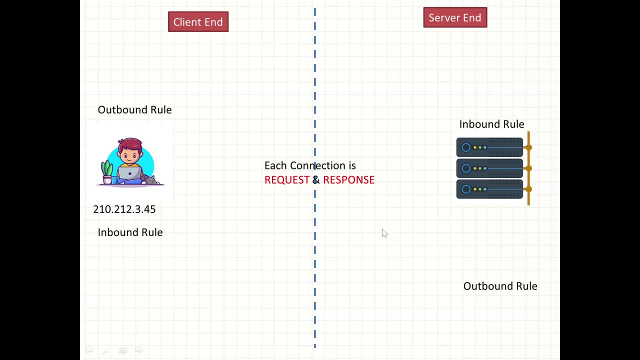 communication is requiring a request and a response. so let us take it uh this client as an ip address. this client ip address is 2102123.45 and the server address is 103 23- 4.56, just taken randomized value. now, when the client is sending, uh, some packet to the server, then you 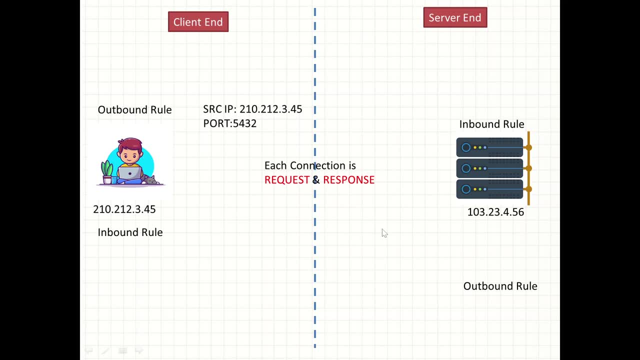 can see. then there is a source ip and there is a source port. so in this case the source ip is the ip of the user and the port any ephemeral port that the system will decide- and this decision is depending upon the operating system that how is deciding the ports. also, it will be requiring a 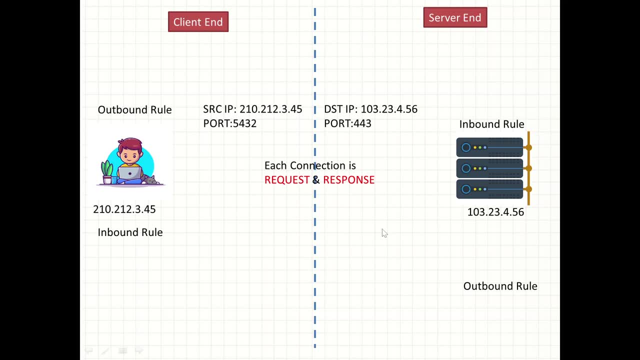 ip and a destination port. so in this case, we are uh sending a https packet over a tcp and the destination port is 103, 23, 4.56. now the connection is absolutely is. give is established, a signal or a packet is being sent uh from the client to server. okay, this packet is being transferred. 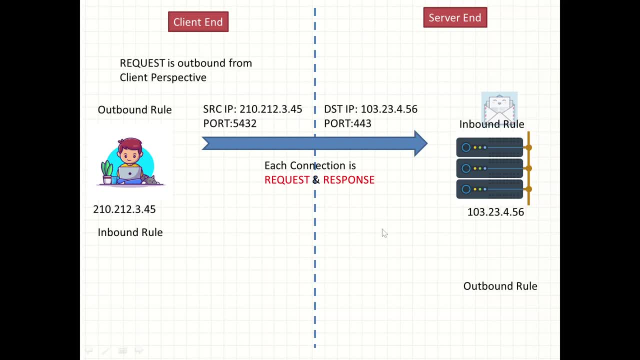 from client to server and in the respond you can see now, there are two types uh of communication is established, where request is outbound from the client, client perspective. what? what i am going to focus in this thing is now that for this person, this person, this is a client. 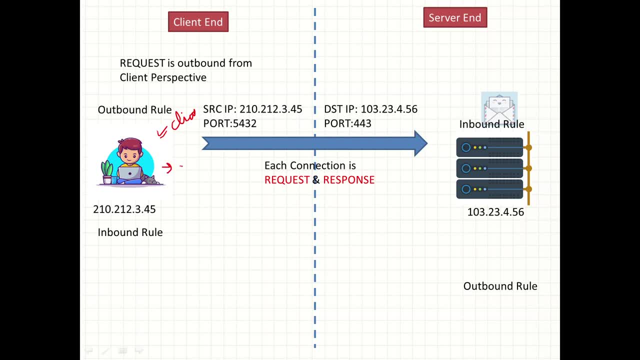 so he need a outbound connection, outbound rule. i would say: this person need an outbound rule to send this packet from this place to this. okay, on the server side, he need an inbound rule to receive this packet into his network. is it fine? is the thing i'm telling you? yes, sir, okay, so this client need an outbound rule and this: 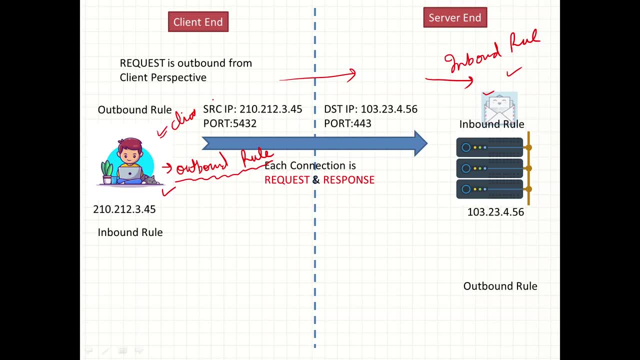 server need an inbound rule. so you can see, for a single communication. this is a single communication where one packet is sent from this source ip to destination ip, from this port to this port. so two: outbound on the client side and inbound from the server side. now, when the server respond, when the server respond to the request, now this server will having which? 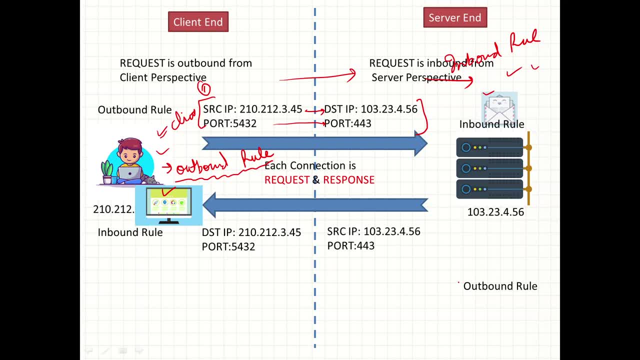 type of rule to send this packet outbound. okay, and now this client will be requiring: which rule is you want outbound Inbound, because packet is coming into his network. so whenever a packet coming into your network, you will be need to configure inbound rule and whenever you are exiting a packet you need to do a outbound rule. 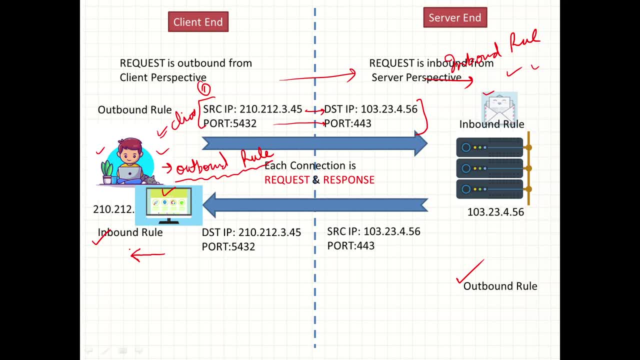 Okay. so this slide, these two slides, I have specifically designed to make you people understand what are the inbound and outbound rules, because for a single communication, two type of rules are required. just keep it in mind: for a single communication, two types of rule are required. one is outbound and one is a inbound. okay, where it will be using. just hold on when we will be talking about type of firewall. 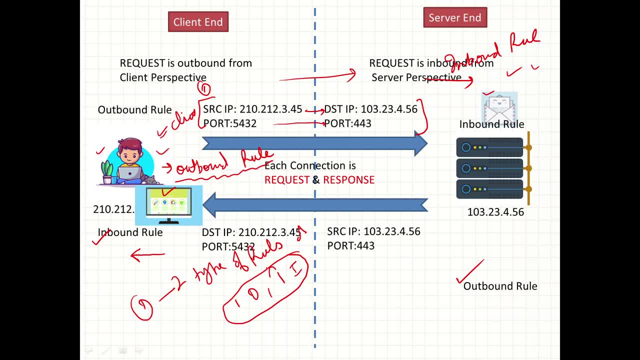 Then this logic will come into picture. okay, any issues into this, sir? this question is like: our destination port 443 means communication is happening on TCP IP. so if source has that port, then why it is not using that port? why it is not using random port, sir? random port is used because the client communication is established by client side, so it is always done by ephemeral port. 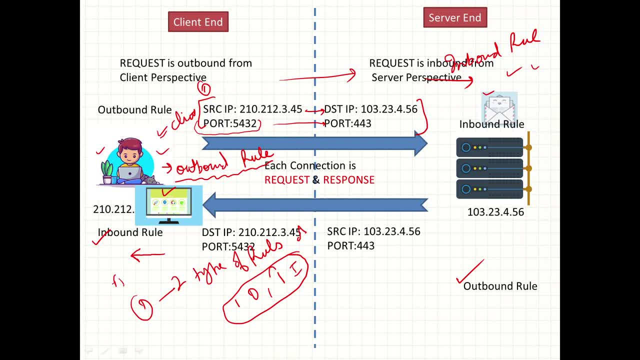 If we are doing FTP, suppose. if we are doing FTP, then communication will be done on same port. okay, generally this is also done to maintain the integrity and security, because the data which is going from your end is echoing somewhere. okay, so the data which is coming from the client end always uses ephemeral port and in target it keeps 443 port, and when reply will come, then it will keep 443 port, and when reply will come, then it will keep 443 port. 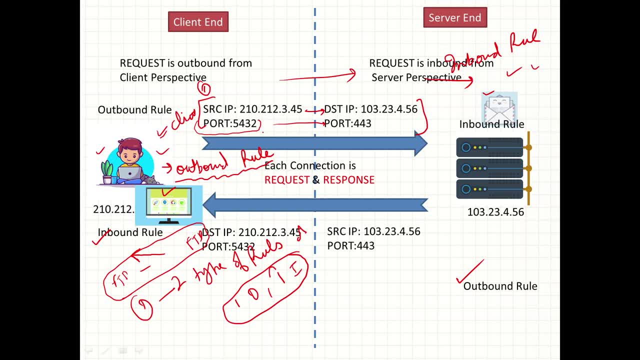 So the data which is coming from the front also will come from 443 and will come on your this port and it is possible that this port number also changes. in reply, When we will do analysis on wireshark, then you will see this thing, practically that how the traffic of HTTPS goes. suppose, if we are taking any unencrypted on port 80, then how the traffic goes, that will be clear to you when we will do firewall today. 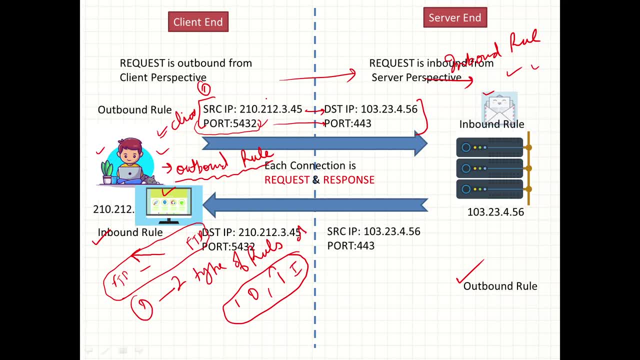 Prashant ji, I think you are saying that we have to do porting basically. So the actual porting which we are doing, So the actual port is 443, which is there at the back end, but front end the traffic which will go on internet will go on some other port. 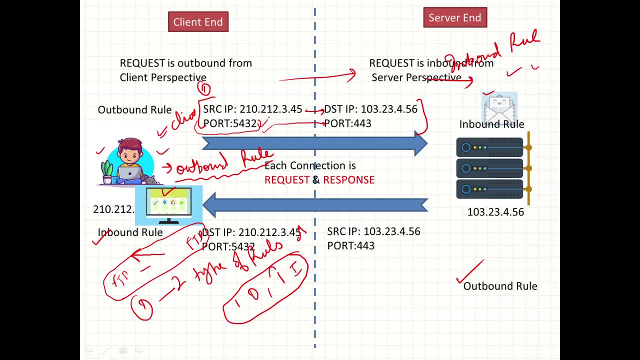 So that we can maintain the integrity and security. So this logic, which I have told you about the inbound and outbound, just keep it with you for the next 15 to 20 minutes when we will be talking about type of firewall. then this topic will again come down to discuss many things, okay. 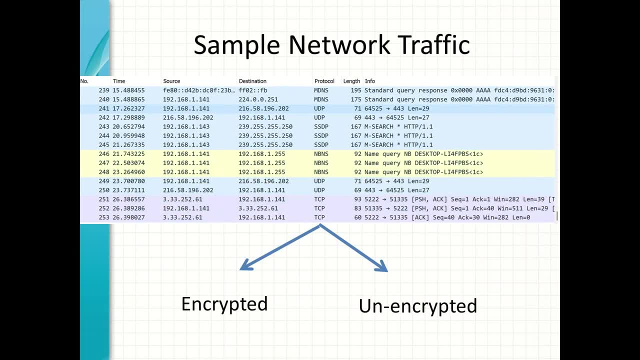 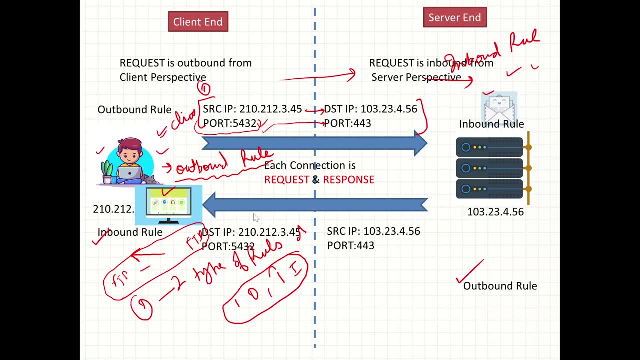 Now see this, Sir. sorry to interview. I have heard one more term, ie ingress. So is ingress related to inbound and outbound? Actually, I will tell you that the word ingress is used in router reference. Sorry to interrupt. Can you speak in English? 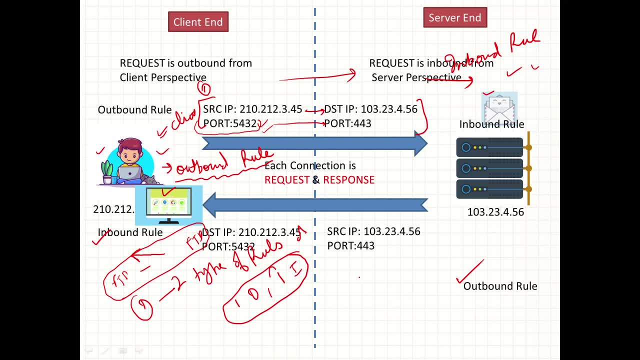 Yeah, yeah, sorry. Actually, the portion is in Hindi, so I have started in Hindi, No issues. So ingress and outgress- actually. ingress and egress- actually, these are two words, And it is usually come About the router when we are talking about router. 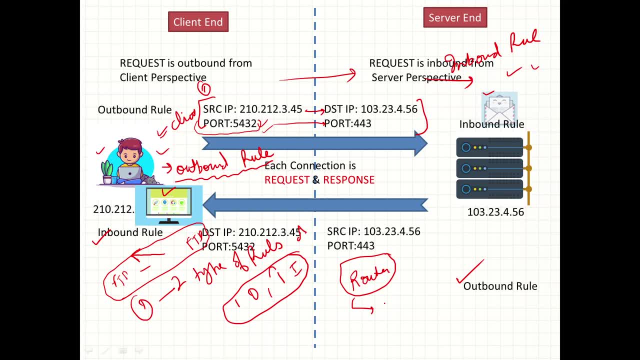 So when we will be talking on router. actually, there are two issues. When router has a control plane- Okay, Control plane, and it has a data plane, There are two different type of planes when we talking about router, Since this class is not about router, but definitely in future I will be talking deeper into the router. what are the control plane, data plane? 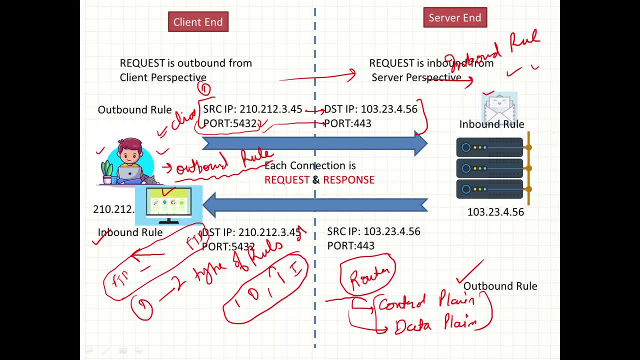 So Whenever a request came, It came to the data control plane, Control plane, transfer the data request to data plane. Data plane again processes and delivered to control plane And control plane then again transferred to further Okay. So this is a ingress and this is outgress. 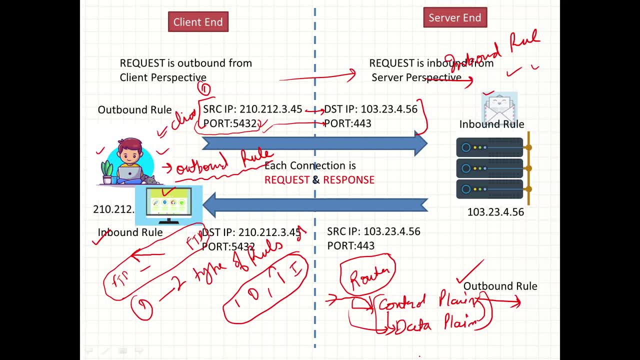 Egress. I think so Is it fine? Yeah, I think it is Yeah. Ingress and outgress, Okay, Okay, So Ingress and egress. I will also write, Sir, how the client- Yes, please- Decides which port to use for sending the data. 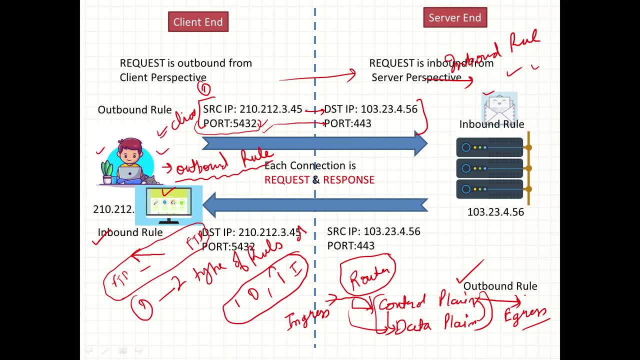 Yeah, I have just followed. How the client decides which port to use Which Mam, your voice is not good. How the client decides which port to use for sending the data. Yeah, How the client decides. Okay, If you are opening. 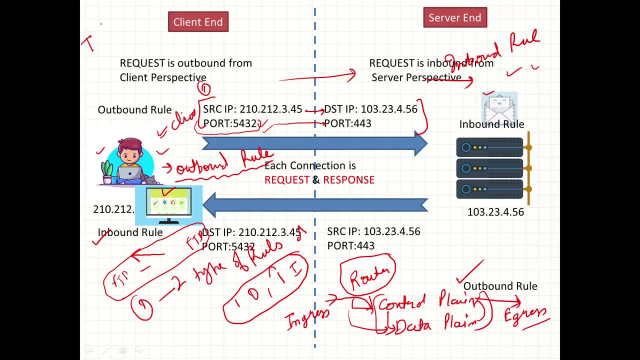 Trying to opening a website. Okay, If you are trying to opening a website And The Port For HTTP is 80.. And HTTPS 443.. Okay, Just keep it This there. For HTTP use 40.. And for HTTPS. 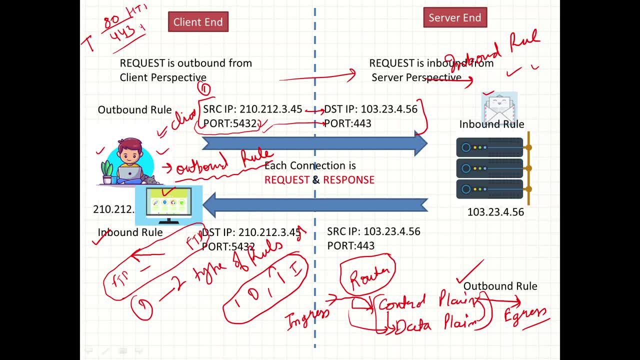 We use 443.. Now If that Website is encrypted? Okay, If the website is using an encryption, It will be Traveling through the HTTPS port- Okay. Now If the Website is Encrypted? Okay, HTTPS. 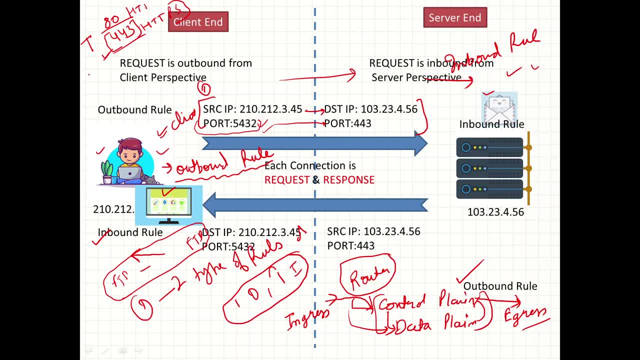 Port On the port 443.. So The client Is Is knowing When it is sending The DNS query It will be getting A response That the That the Opposite Website is using Which protocol. 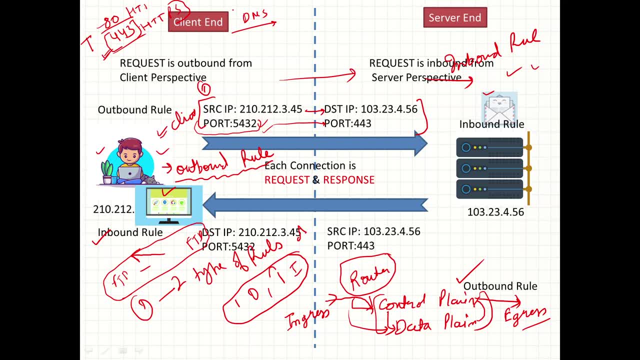 80 or 443.. In the same case, When you are using Telnet- Okay, When you are using Telnet, And in that Telnet You need To Talk on which port Is The Telnet? 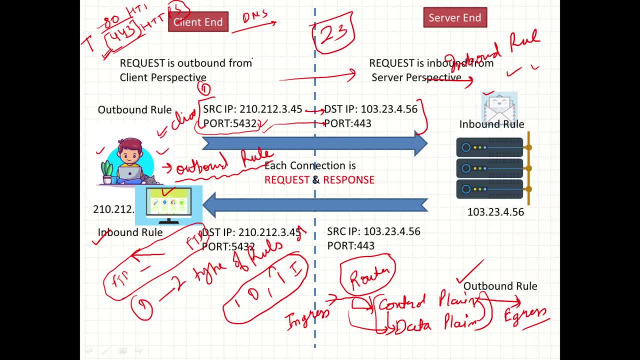 Port 23. Yeah, 23.. So Telnet Port Is 23. So To Initiate A Communication, You Need To Start A Communication From 23. And 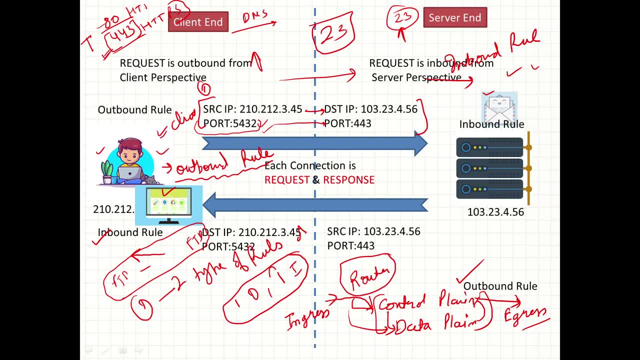 Then Again On The Port. But The Computer Know, The System, Know That For Sending A Particular Packet Which Port Is Going To Use, Because 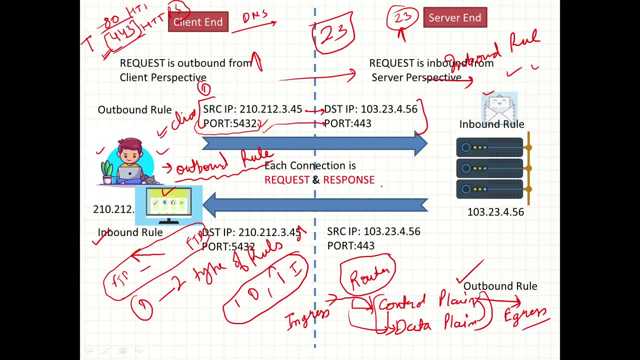 Because On The Same Port The Communication, So It Can Fetch Randomly Anywhere. Yeah, Yeah, It Is Randomly Fetching From, I Tell From This: 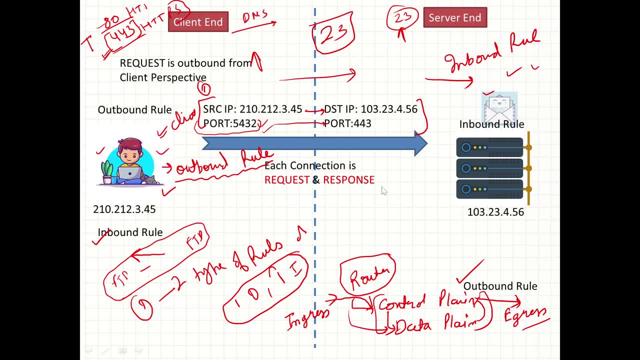 So This Is An Alien. I Have Question: When We Accesses Gmail Outlook Client, Then For Sending It Is Using SMTP Fort And For Receiving 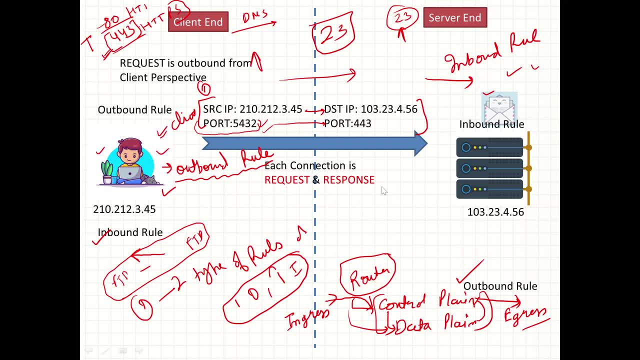 It Is Your Decision That You Have Configured A Pop Three Or I Map Configuration Okay. So That Is A Different Port For Communication, Because 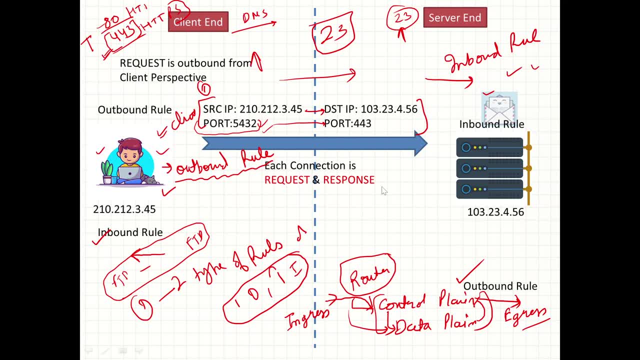 They Have A Different Protocol. They Are Not Using The Sttp Or Sttp As They Are Using Smtp. They Are Able To Solve Your. 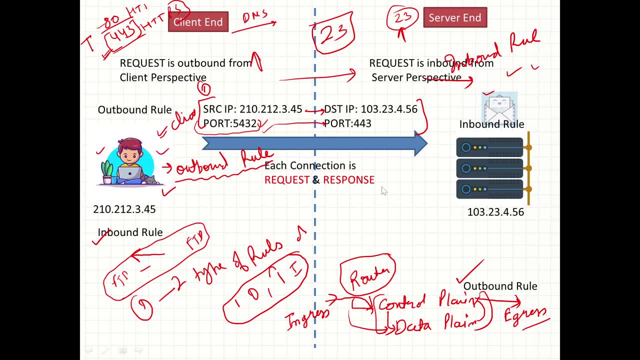 Issue: Yes, Yes, Sir, Yes, So I Have One Clarification. Yeah, Yeah, I Have One Clarification. So This Outbound Rule You Have Mentioned As 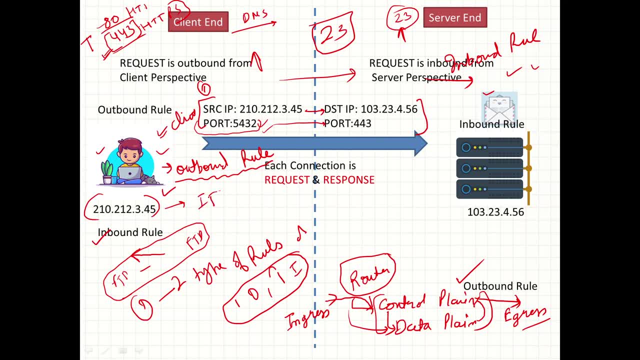 A System I P And Probably Your Isp Has Given This Or Your Network Has Given This. Okay, This Is Manually Assigned, It's Not. 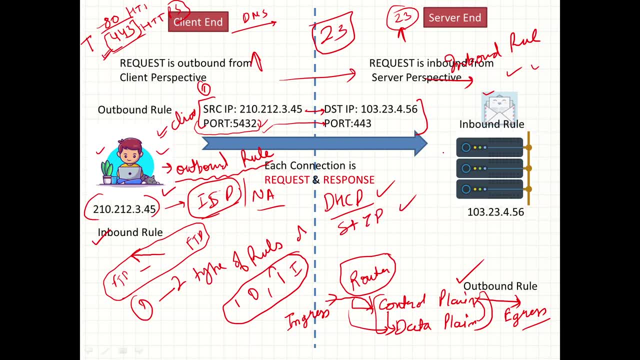 Automatically Assigned By Any. It Depends If This Each Character Any You Can Explain To Us. Okay, Yeah, IP. This Is An IP Address, Actually, This. 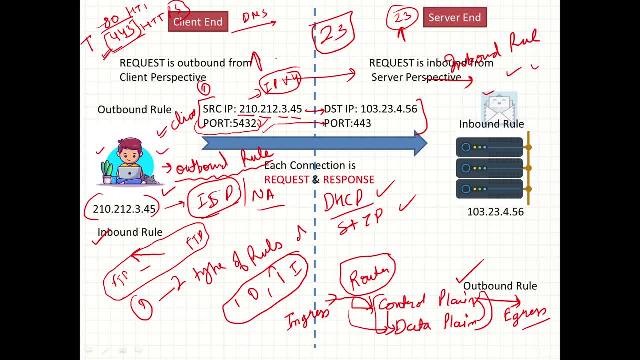 Is An IP Address And This Is A Specifically Why Part. Okay, So It Is A Long Time. It Is A Very Long Discussion, If I 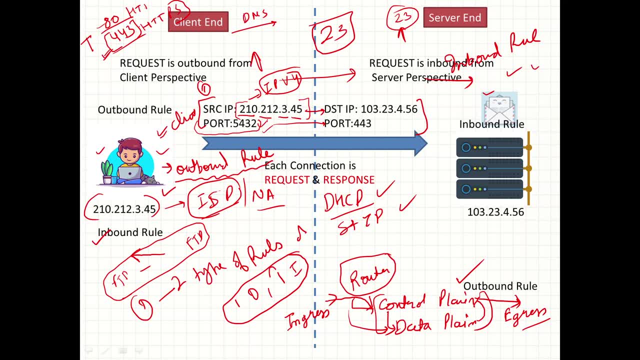 Talk About IP, Because Then We Need To Talk About Subnetting And Lot Of IP. If, Till I Disconnect From The Network, It Will Be 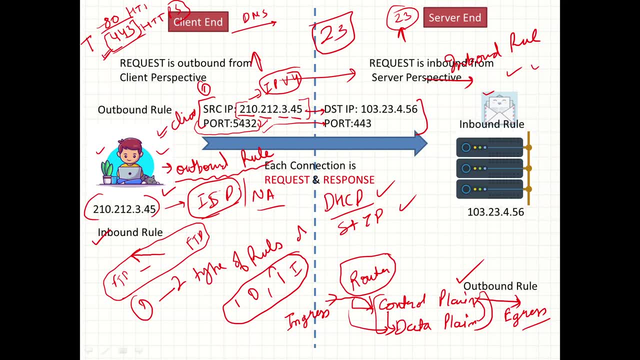 The Same And Same Number. It Will Not Get Changed. Now Think Of A Scenario: Whenever You So Basically Every Time Your Mobile Is Getting An. 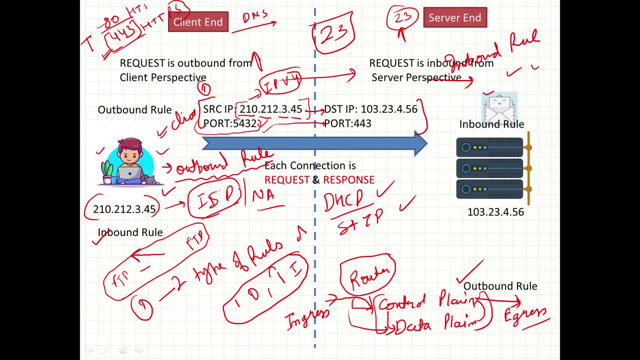 IP, But The Server, The DSCP Server Of Your- A Little Of Any Companies Is- I Is Assigning A Different. That Is All The DNS. 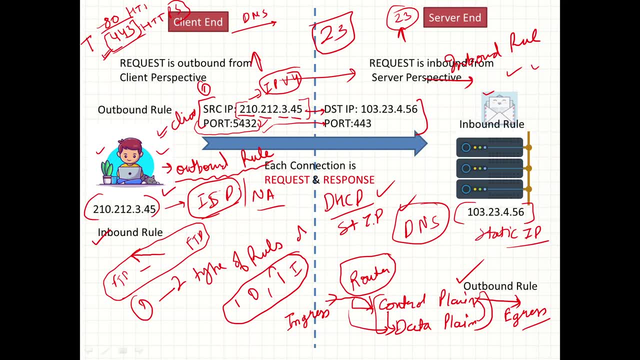 Queries, They Need To Have A Static IP. Even Clients Can Also Have A Static IP, But They Are Chargeable. Actually, Static IPs Are Not. 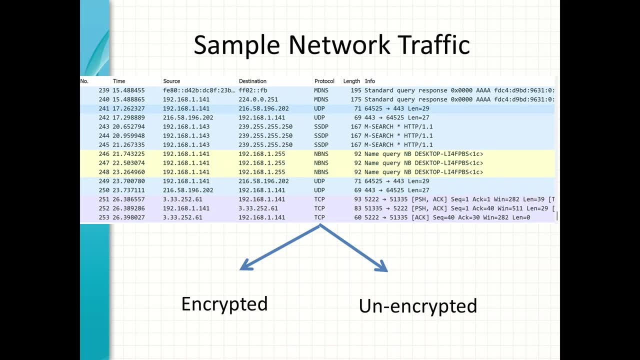 So This Is A Simple Network Traffic, Okay, And We Will Be Talking About How We Going To Capture The Network Traffic And All, But When? 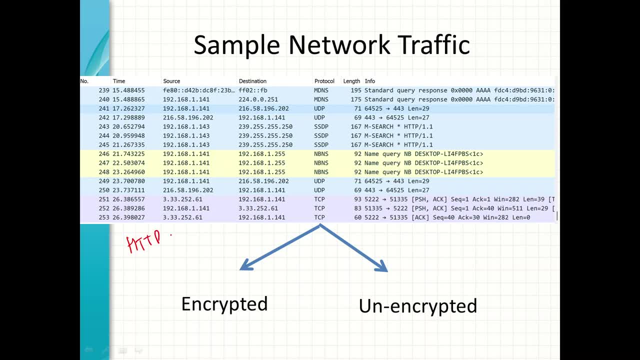 You See, We Have A HTTP Protocol On Port 80. To Communicate Over The Internet, Okay, But The Problem In The HTTP Is That That 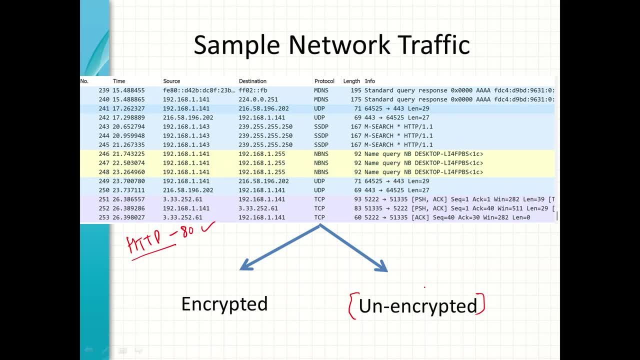 It Is An Encrypted. If You Want To Connect To The Network, And We Will Be Talking About The Network And We Will Be Talking 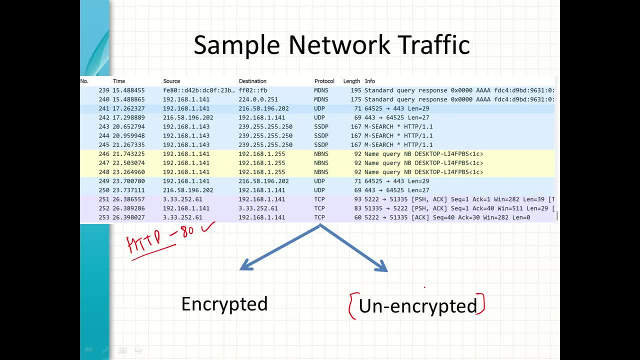 About The Network And We Will Connect To The Network And The Connect To The Network And My Browser And The Network Will Connect To A. 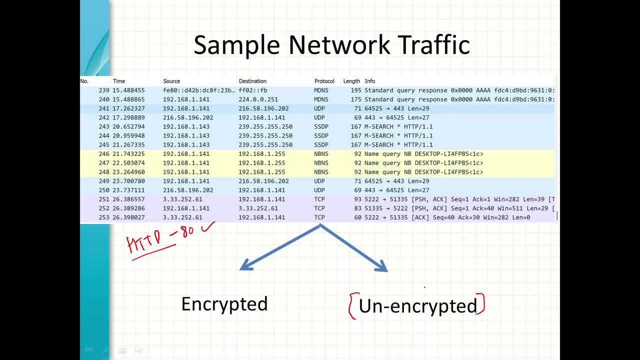 P Network, Everybody Will Be Connected To The Network And Connect To The. Thank you, Thank you, Sorry, sir. Sir, can you go to the previous slide, This one, Yeah. 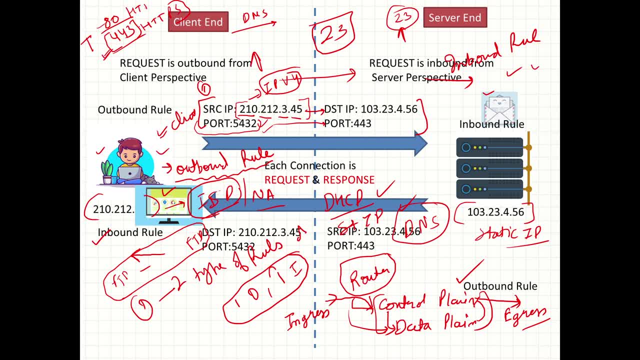 Sir, you mentioned inbound rule and outbound rule. Do you have any list for that? What are the inbound rules? What are the outbound rules? Okay, So you need to know about some example. Yes, exactly. Yeah, just a moment. 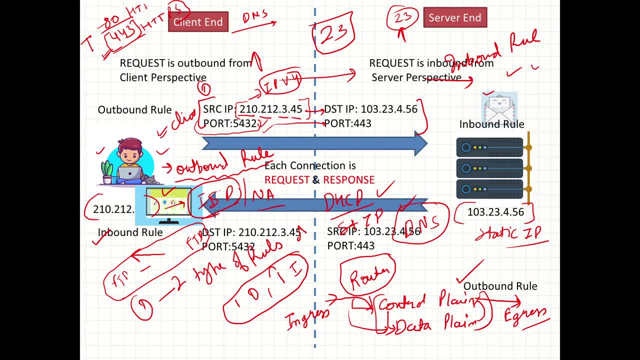 So if I talk that, to let us take a non-IT example, because I love these non-IT examples. Okay, So you have a neighbor with you. Okay, So let us suppose your name is Mr A and your neighbor name is Mr B. 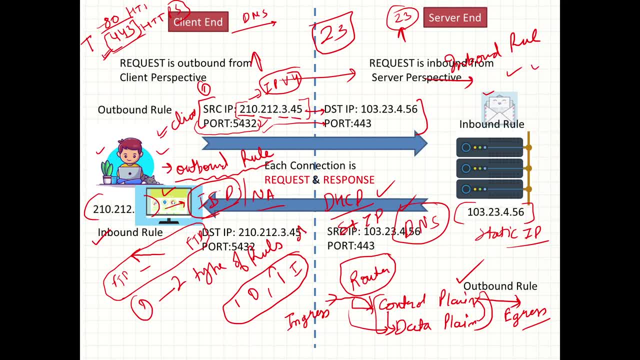 Okay, So now you ask your child to talk only to son of neighbor B. Okay, So this is an outbound rule. You are telling your child that you need to talk only to the son of the neighbor B, not his daughter. 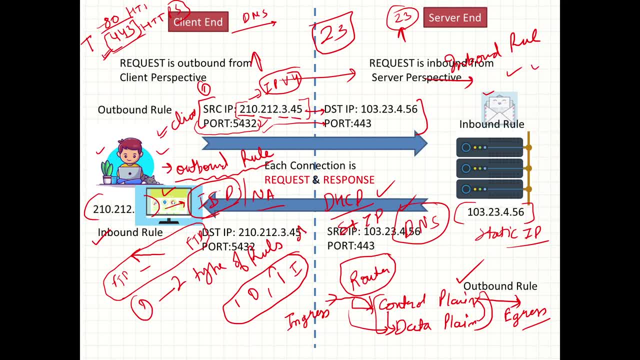 Not his daughter. Okay, So this is an outbound rule. In this case, you are allowing your child to talk to someone, but you are disallowing your child to talk to someone. Okay, So this is an outbound rule. 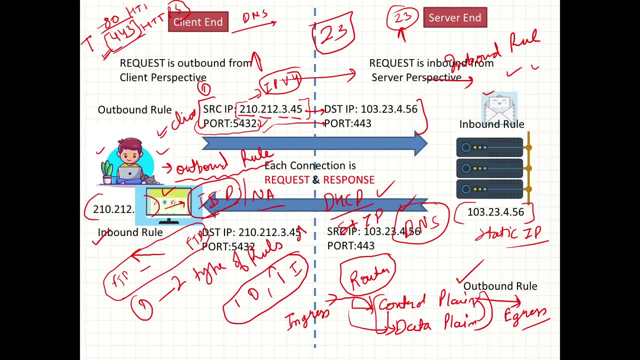 And let us suppose on your neighbor's side- I think I am getting echo from someone- Okay. So again from your neighbor's side, if your neighbor is saying that do not talk to the children of Mr A, Okay, So, even if you are trying to talk with them, they are not talking with you. 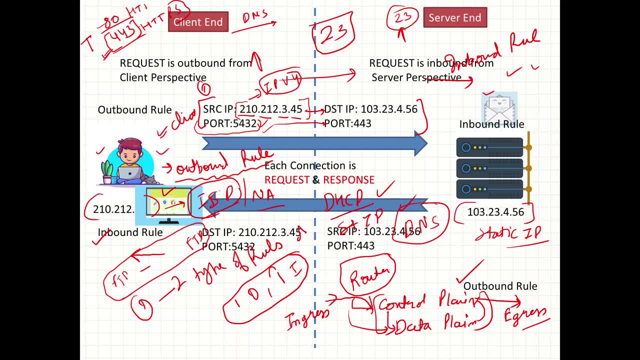 Okay, So from your side, you have an inbound rule and from their side they have a separate inbound rule. You have outbound, they have an inbound, But to have a proper communication between both of you, you need to take care that a proper rules are to be set off. 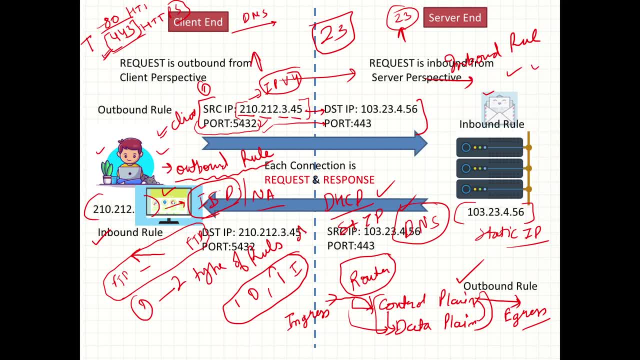 So that if you are sending a packet, he will be receiving that packet. You understand now, sir. Yes, sir, Thank you. But how? that is ARM data, how we have to block between this rule. Yeah, yeah, yeah. 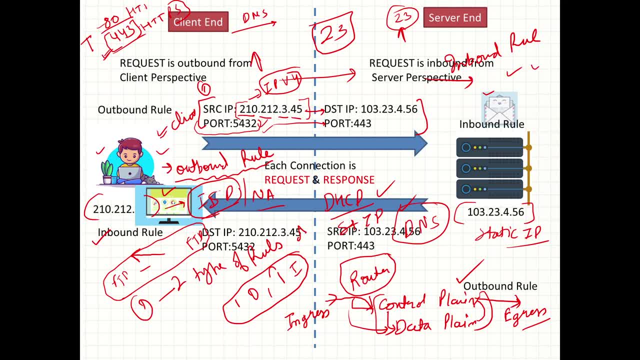 Today. I have already said I have a specific firewall for you. I have deployed at my home And today we will be talking on that. So rest assured that's not an issue. Okay, Thank you, Sir. Yeah, please. 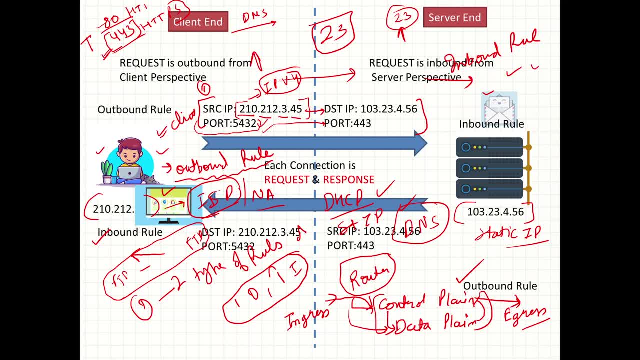 Sir, can you please explain what is DNS and what is ISP? Okay, DNS and ISP. I think these topics are not covered in your last lecture. No, sir, Okay. okay, These were not covered In the first lecture. it was told what is ISP. 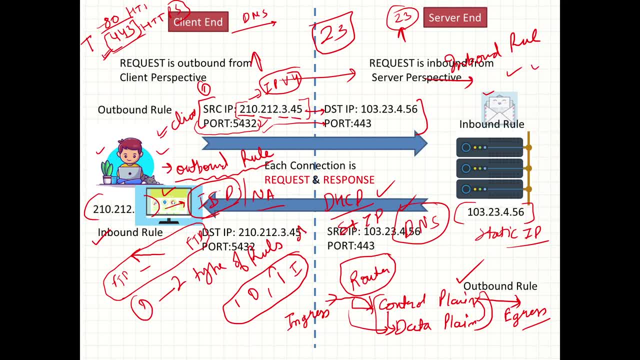 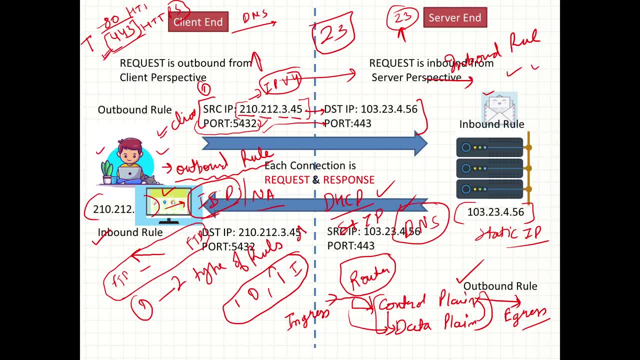 Let's talk about it. Let's talk about it. Let's talk about DNS. Can anybody tell in class what is DNS? Domain name, sir. Domain name, sir. Mapping of IP address to the well-known name. It's like a telephone yellow page, sir. 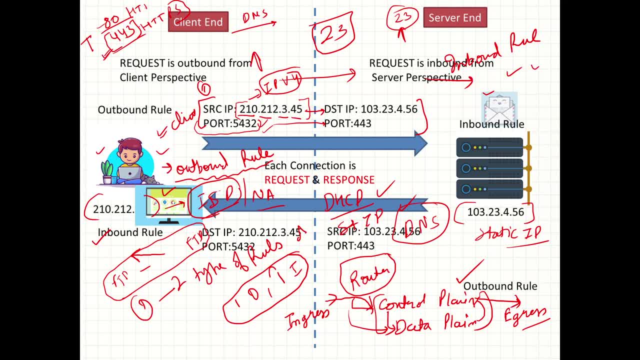 Yeah, it is a yellow page, sir. Yes, perfect, perfect. And how exactly it works. Mapping is So basically, Yeah, Mapping is Domain name to IP address. I think it is query-based system where we raise the inquiry. 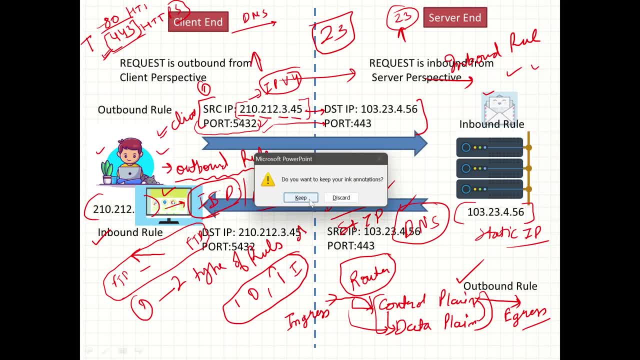 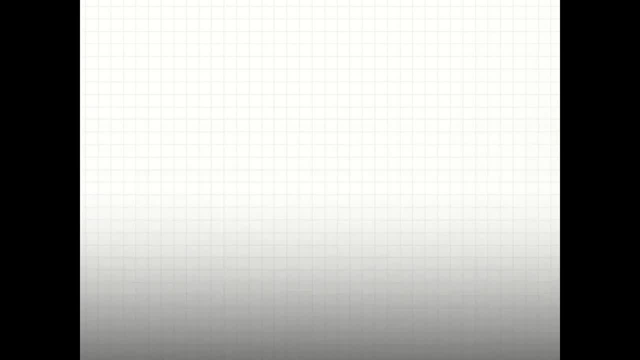 and get the sorted path. I think Okay, Anyone else Domain name helps us to resolve from host name to IP address and IP address to host name. so these are very unique like globally accessed. uh, i mean, if i keep one dns name cannot be changed. 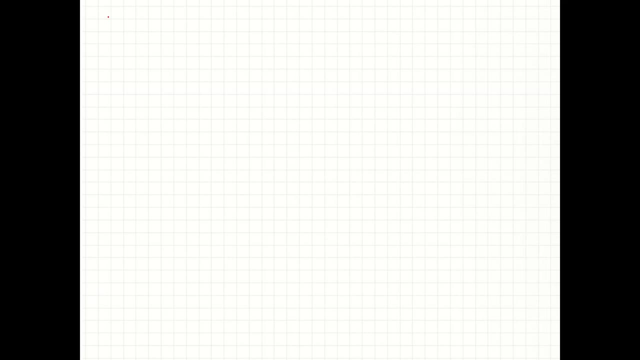 uh by or same name cannot be keep by any other people, so it's a unique name, perfect, perfect. anybody else it is, it is. it is uh if we, if we find some analogy between uh telephone connection, landline connection, so uh ip address is like a telephone number and uh subscriber's name is like 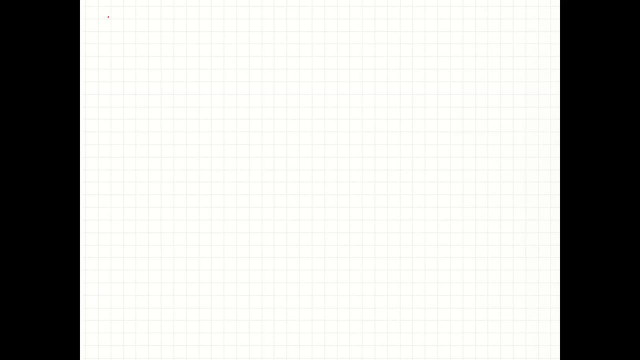 domain name server. perfect, perfect, perfect, sir. so we have a 13 uh root, dns root servers involved, so they are managing the uh dns services, dns services. okay, so let me. let me explain in just a few minutes what is exactly a dns server. okay, i think most of the people have. 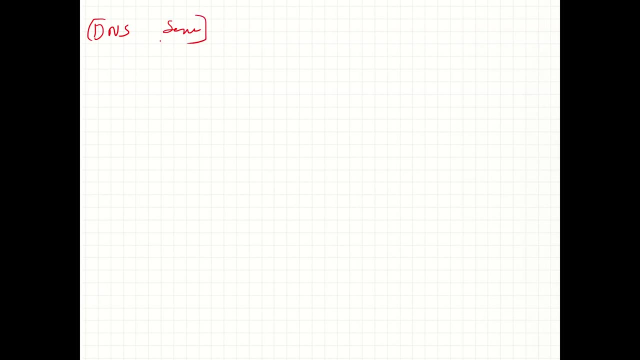 already know, but if, because definitely someone has asked, so i need to resolve his query also. so what is a dns server? let me give you an example: this: this is a 103.122.36.1. okay, so this is an ip. okay, this is an ip of a website. okay, this is an ip of a website, uh, of your. 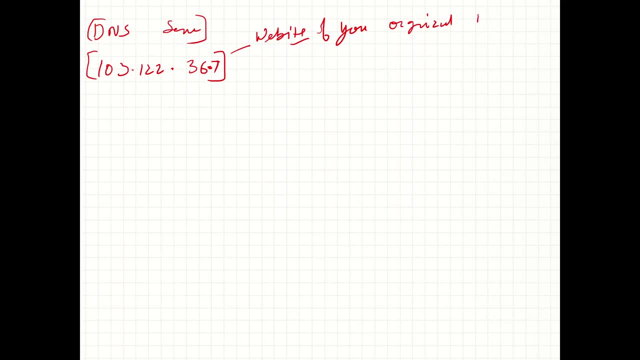 organization, okay, organization, erp, particularly erp, where you apply cl or your medical leaves or privilege leave, okay. so if your network admin is tell you that this is your ip to apply for your cl, pl and each of everything, then it's very hard for you to remember this ip address because- because it is- 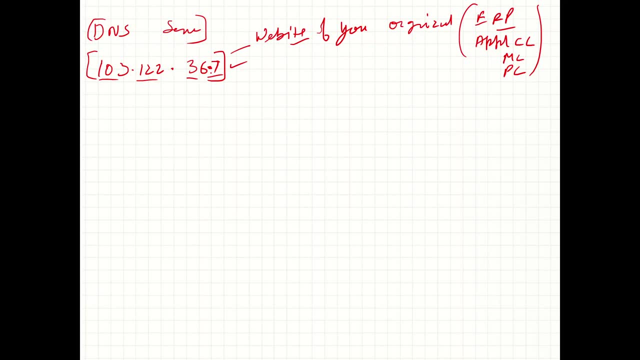 four octets and it is a lot of numbers, so there is a chance that you may forgot this number. so what the network have, what the technology has done, they have created a dns technology domain name server. okay, domain name server, okay. so whenever you type in your browser that wwwgooglecom, okay, let. 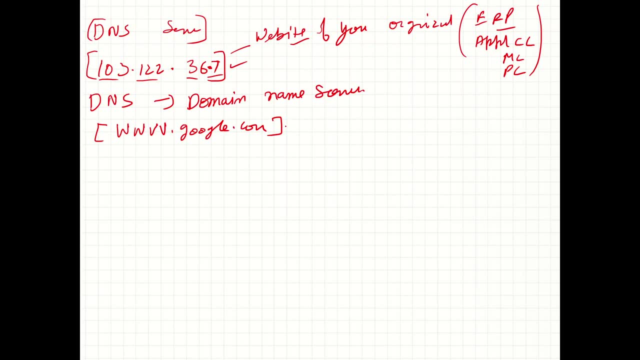 us suppose. uh, take a example of googlecom. whenever you type this word wwwgooglecom, at that moment of typing this word, wwwgooglecom becomes your domain name server, and so whenever you type your name on your browser as well, um, there is a real reason why you have created. 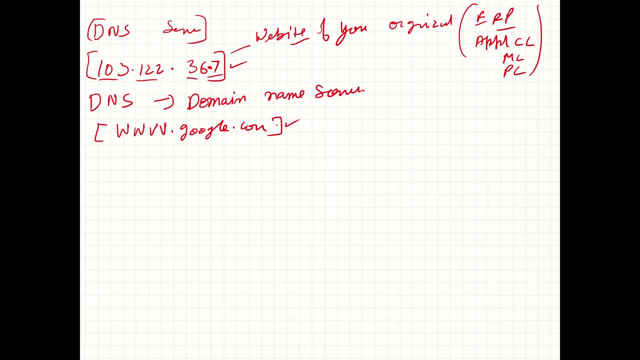 domain names. so this is a very common thing, and so that is the reason that we have created time. your computer is not knowing anything about wwwgooglecom. he do not know anything about googlecom. what he will do? he will directly go to the dns server. it will send a request. 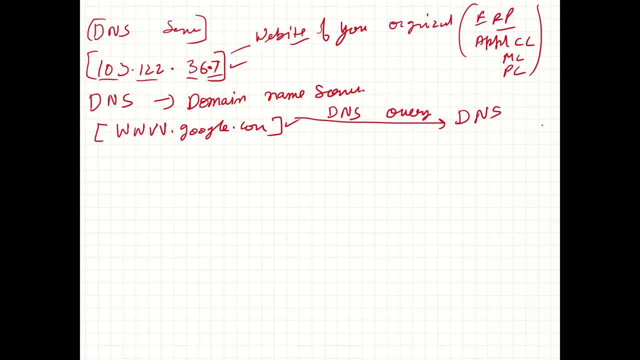 that is, we called it as a dns query. okay, we send a dns query to the dns server and it will ask him that who is googlecom? he will ask literally when we see in wireshark, he will ask who is googlecom. to that, this dns server and this dns server will provide an. 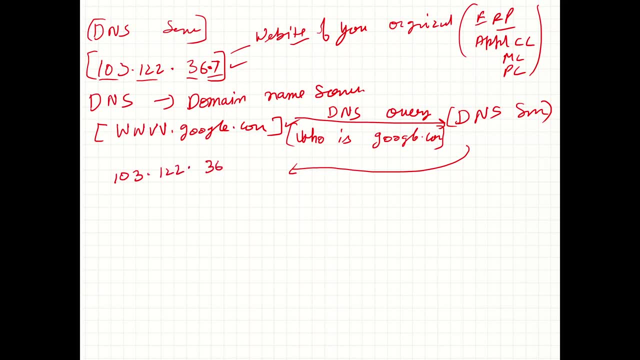 ip address to your system that googlecom has hosted a services on this particular public ip. okay, on this particular public ip. So okay, So, So. So this is exactly a dns. actually, dns servers are maintaining tables and maintaining tables, uh, in their records where a domain is mapped with the ips. somebody has correctly said that. 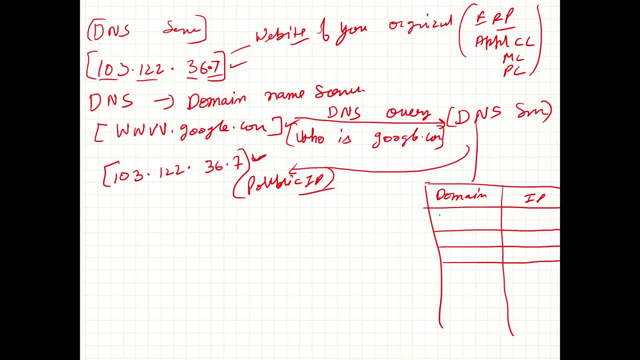 dictionary, that telephone directory and all. so it is hyper directive where this ip 103- not one, two, two- is written as googlecom. okay, so every time you need to go to the dns server to resolve your query. actually this process is called resolve of query. okay, now a question is: 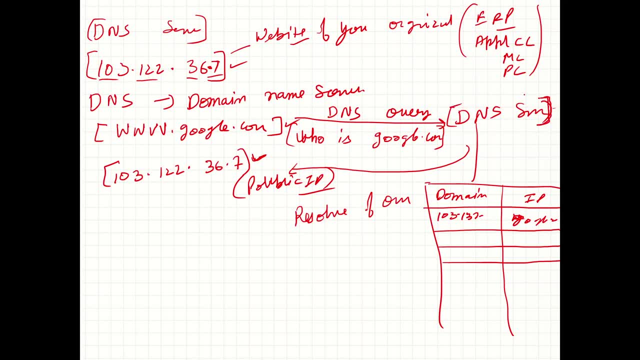 coming into your mind that how your computer know that which dns server is going to be reached, yes or no? yes, sir, there is a question. so the solution is: you, when you are configuring, when you are configuring your system. okay, let me tell you when you are configuring your system. 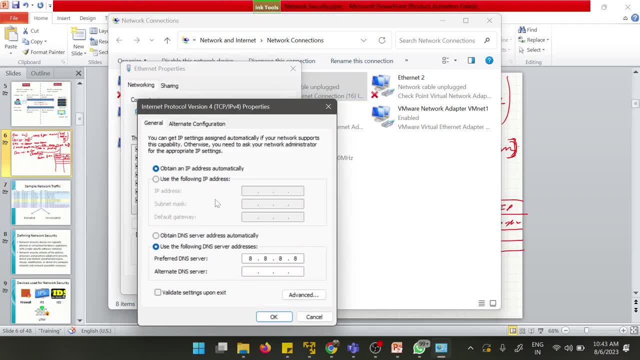 when you are configuring your system, you usually use this type of settings: okay, obtain ip address automatically in case ip is not provided it. and you also use this one: obtain dns server address automatically. okay, yes, sir. so what the thing is when you do this automatically? the dscp server who is providing? 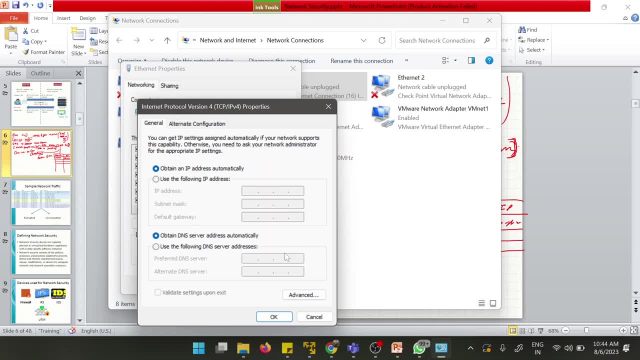 you the ip. it is also providing you with dscp, a dns server ip, also, okay, and in case you want to put it of your own, you can use 8.8.8.8. it is a google dns services, okay, so you can use this 8.8.8.8. 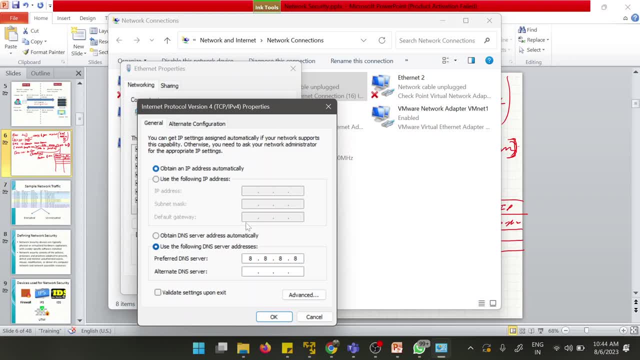 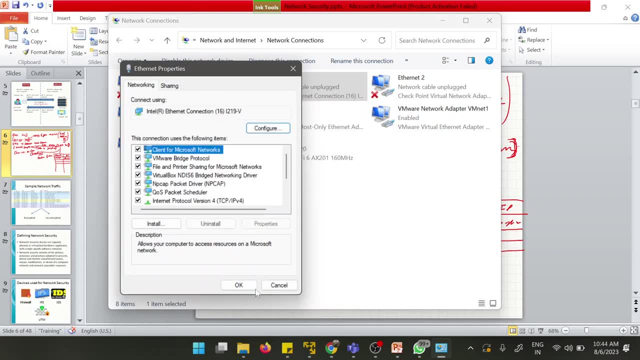 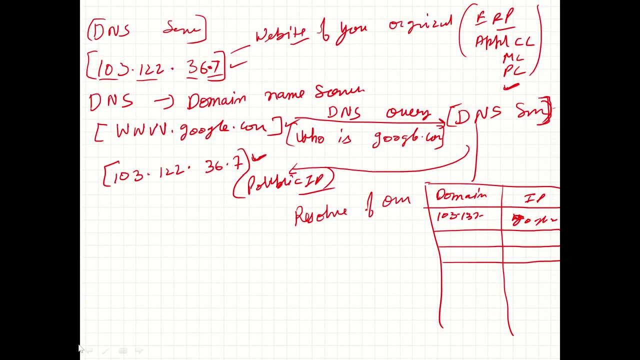 can use this 8.8.8.8 dns services, so every time your packet will be transferred to this server, this is a dns server 8.8.8.8. okay, understood, now is it clear to everyone who has asked this question about dns. 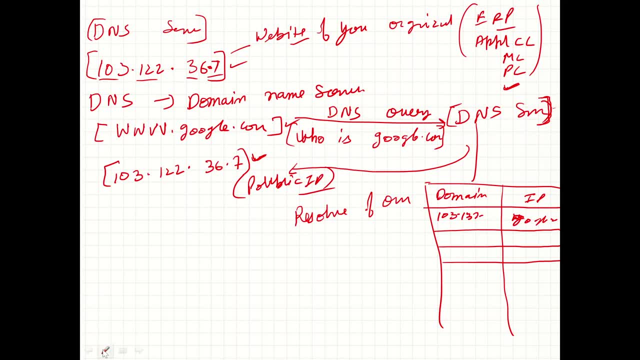 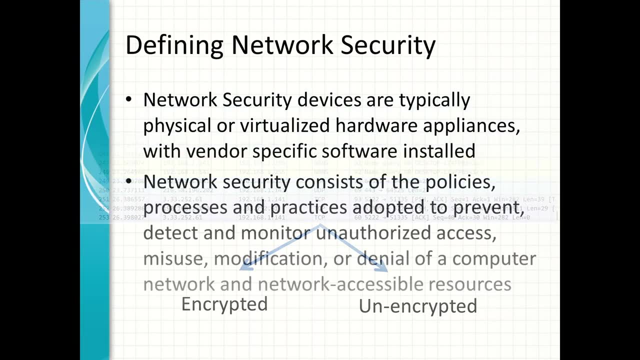 yes, sir me palav. yeah, palavji, is it clear at your end? yes, sir, clear, yeah, yeah, thank you, thank you. okay, so we have seen that there are two type of network traffic: one is encrypted and one is an unencrypted. now, defining network security network. 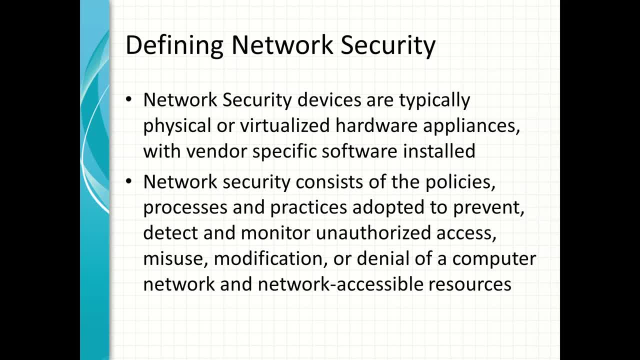 security devices are typically physical or virtualized hardware appliances with vendor specific software installed. network security consists of the policies, processes and practices adopted to prevent, detect and monitor unauthorized access, modification, denial of service, network network accessible resources and misuse of the network. so this is our motive when we're talking 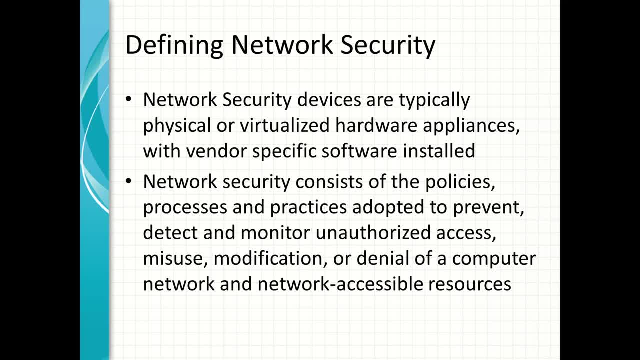 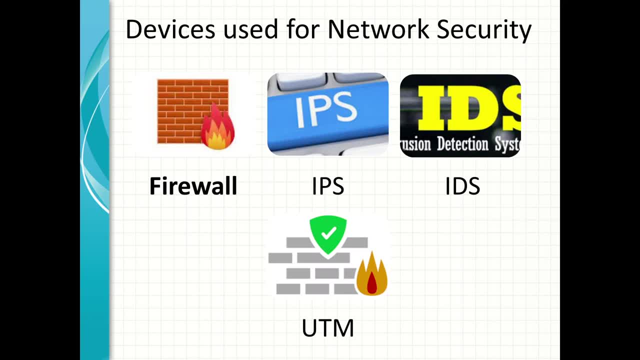 about the network security. okay, uh, can somebody tell uh, using the dns query, which type of attack is happening these days? yeah, perfect sir. so using the dns attack, uh, these man in the middle, attacks are happening so much and when. we will be talking about different type of attacks. 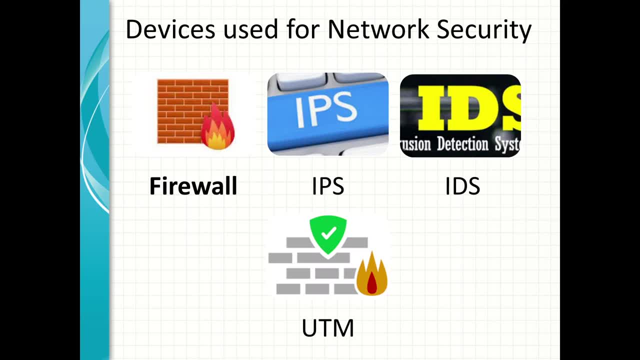 we will be talking on this about the mitm attack, about the ddos attack, the dos attack. so just hold for the while. there are a lot of things to come and we are trying to base, uh, build a very good base for only people, so let us concentrate on this thing now. uh, what are the different type? 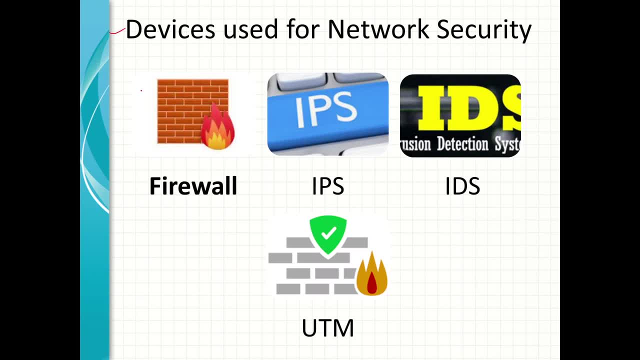 of different devices used for the network security. i think everybody is knowing about the firewall. everybody is knowing about the ips ids and utm, yes or no. you can use your checkboxes, ad box, to do to type yes or no, because i have a habit to ask a lot of questions from the participants. 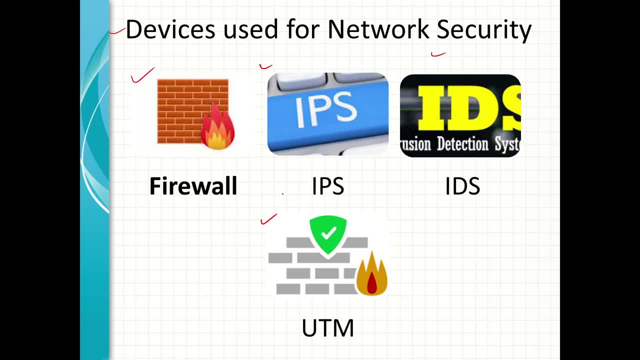 so you can just write yes or no, not not an issue. yes, so can anybody tell what is the difference between ips and ids? first, ips is preventing and ids is deducting, and then only it can prevent. okay, okay, a set of rules which match with them. perfect, perfect, we will. we need to drill down more deeper into this. 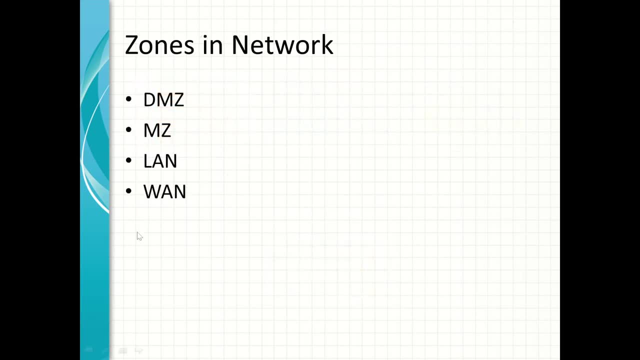 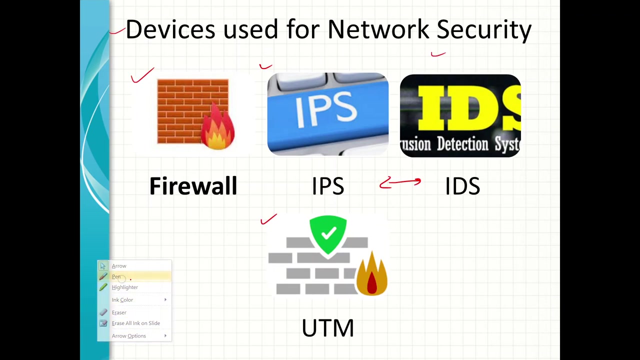 okay, so i think you have talked about the zones in the uh. previous class zones are covered or not? what is utm, dmz html? is a unified threat management? we will be. we will be coming on this. yeah, they have covered about zones. it is trusted zone and dmz zone like that. okay, unified threat. 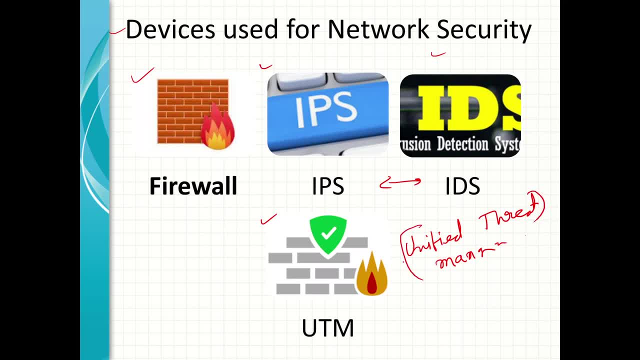 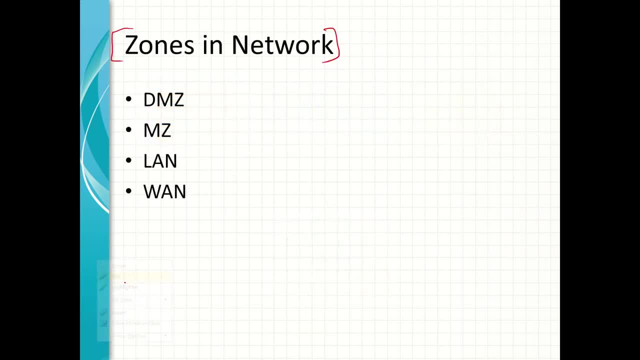 management. okay, this is a type of device only we will. we will be talking about each and everything, just, uh, rest assured, okay. so we will be talking about each and everything, just rest assured, okay. so i think zone is covered now. we militarized militarized local area. wide area, wide area. 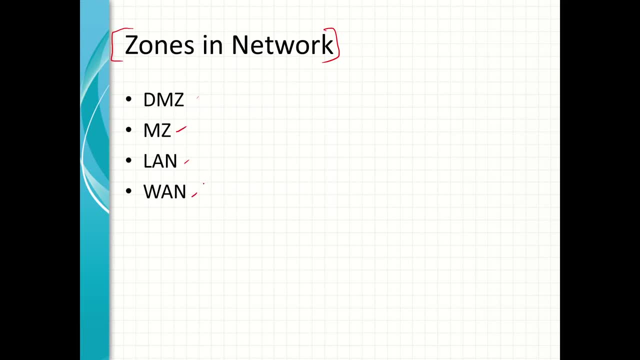 okay, so everybody is knowing the meaning of dmz, mz, lan, when. okay, let me give you a small uh scenario to make you people uh crystal clear concept about the zoning. okay, because if you not able to understand the uh zoning, then you are not able to configure a firewall. and i think these lectures 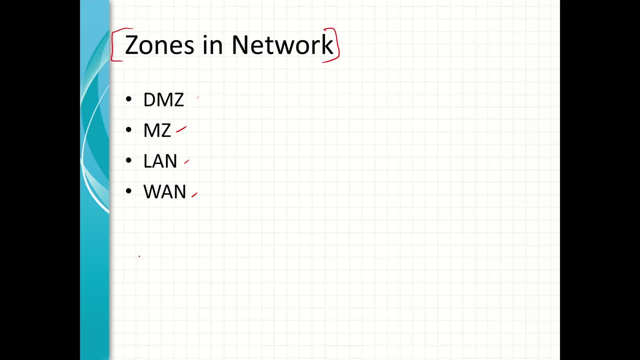 series are to make you people uh aware and to make you people as an expert to configure your firewall, to understand how. what is the firewall rule is in your organization? firewall is: is it yes or no? yes, sir, i will request you to explain on the land and went, but because uh zoning was. 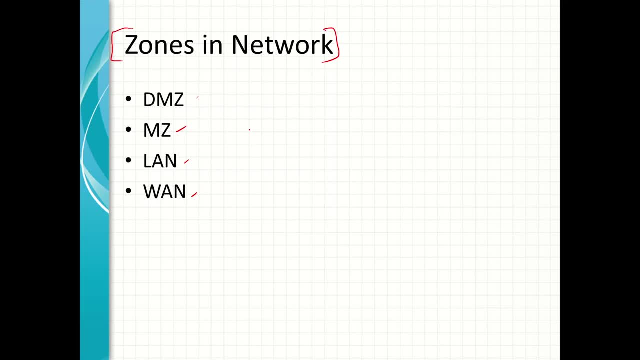 explained. but, uh, in terms of operation, uh, uh, yeah, yeah, i i'm going to talk on that, on a practical. i will create a practical scenario for you, then we will talk that: what zone are this? okay, okay, so let me start with it. okay, so one question is there. yeah, sir, what is the difference between? 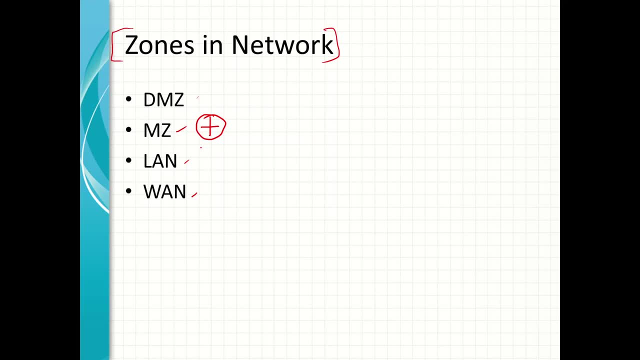 dmz suite and firewall. just hold for a moment. after this you will getting your answers. self explanation after this example. okay, otherwise i will take your question and i'm not an issue. okay, okay, so just concentrate on this. uh, let us suppose that this is a input: internet connectivity from. 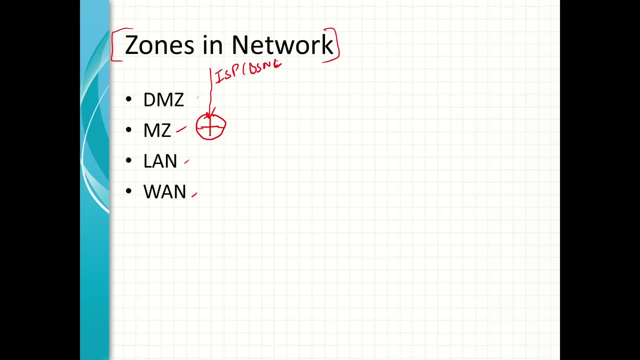 probably bsnl or something. now the connectivity coming to your router and from router you have put down a firewall. you have put down a firewall. okay, you have put down a firewall. and on this firewall, after this firewall, you have installed a switch. usually we called it as a core switch. okay, from this core switch, now what happened? uh? 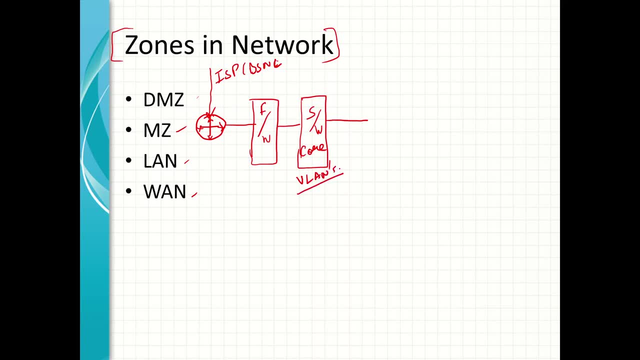 this course is having a lot of vlens. i think vlens is already covered for separate vlens, a separate switch. okay, so you have put down a firewall and on this firewall, after this firewall, you have put down a firewallن. this next vlens. the vlens is not there, that is the vlens of a deploy Terminal. 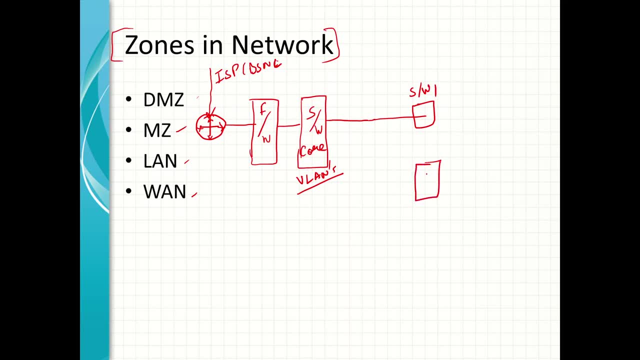 then this vlens gives back exposed works for you whichcitb over here. so this is less than half of that fresh vlens. then next vlens is less than half of vlens after this firewall. okay, good, so this is the only vlens now you have control over. obviously. now this is a bWs container. okay, and finally i have. 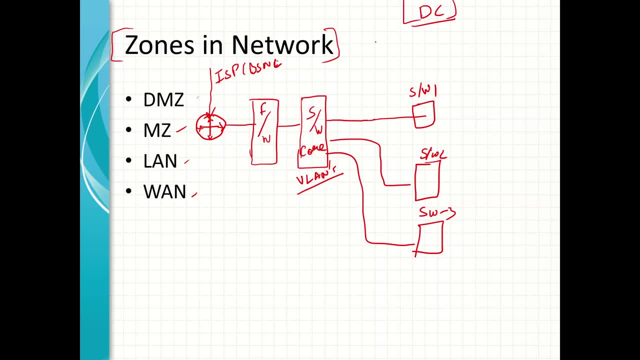 completed process. i just want to say you have not turn this on vln. the vlens is a yes, no, you want to turn it off, so right. so now let's just see what we are done here. first, we call it as convention after this founded in vlens. once we come back. so this vln when one side of clean vlin to be created. 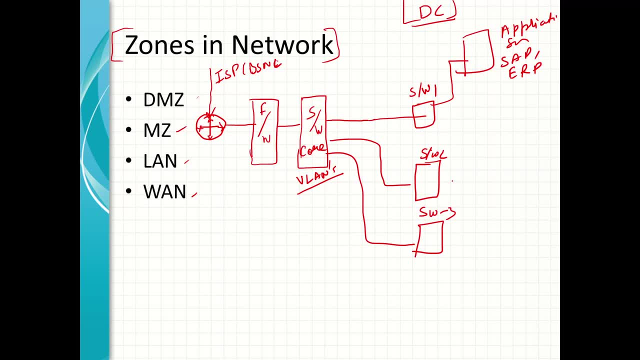 probably your erp servers- okay, application. and on this switch to what you have deployed. you have deployed your db servers: okay, database servers or some you can say that syslog server are there. okay. and on the switch 3 you have connected your workstations. okay, now, on switch 3, you connected your workstation. now, let us suppose: uh, this is a person. 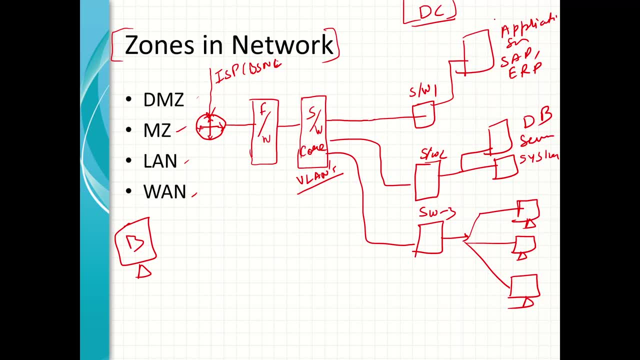 this is a person b and he want to access. he want to access this application server. he want to access this application server. so what would be the way? he will be going to the internet cloud and this internet cloud will make him connect to this ISP broadband and then he is lending to the router: from router to firewall to firewall to core switch. 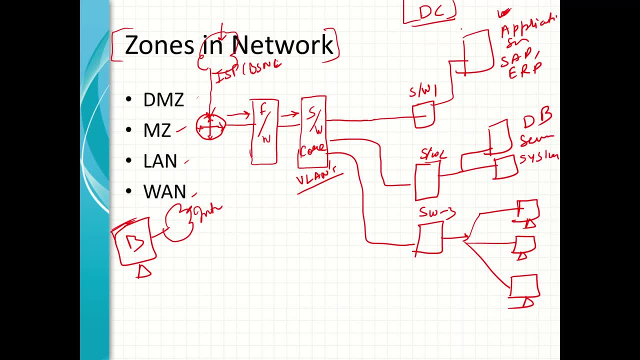 and this core switch will decide that. let us suppose the application server IP is 103.2.2.1 and he has written here 103.2.2.1. okay, so in this case he want to access this resource. Mr B want to access this resource and this resource is available in this data center. 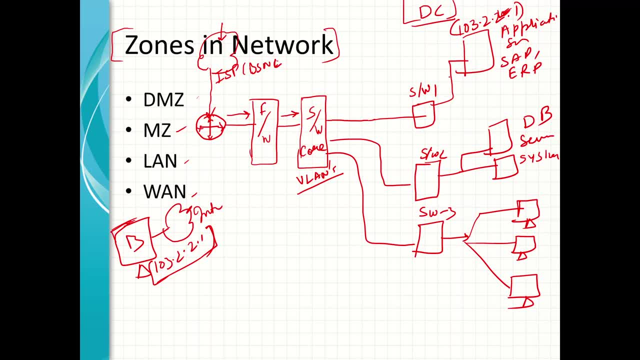 under the switch one. okay, so this is the probable way of travelling to the application server. okay, now think of a scenario. this application server is hosting a website is hosting a website where it is asking for a username and password with a submit button. okay, mostly websites nowadays are using this type of functionality: login password. 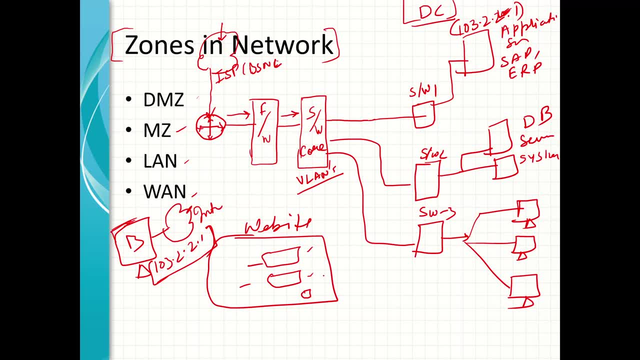 So for login password, can anybody tell now the application server will move to which server to go to verify the login id password? db server, database server, because sql is in this and all the user id password is stored in sql. okay, usually it can be done through other technology also, but this is a like common technology using sql. okay. 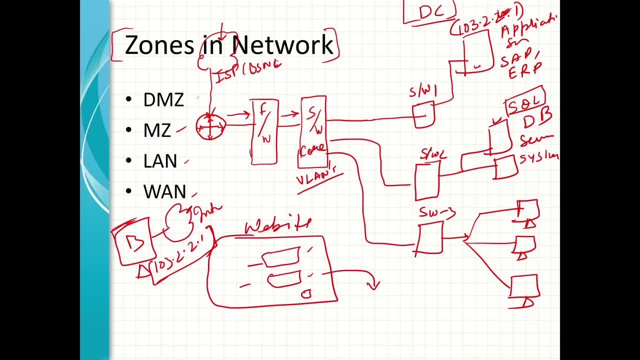 So now This application server will again go to switch one. then this is the route, yes or no? yes, you can use pointer when you use it. no, can you use. can you please use pointer, sir? yeah, yeah, yeah, I can use. I can use it so for to communicate. so, and sorry for my drawing, it's very bad actually. 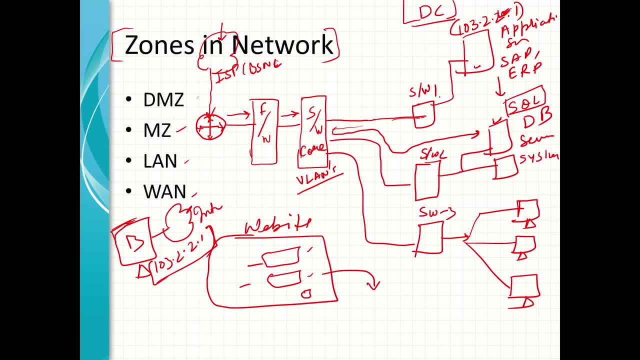 so for to communicate from application server to the data server. He need to again back to the uh. this code switch and to this okay. so now I have a question from you people: which type of access are mr b need to have about to the application server? 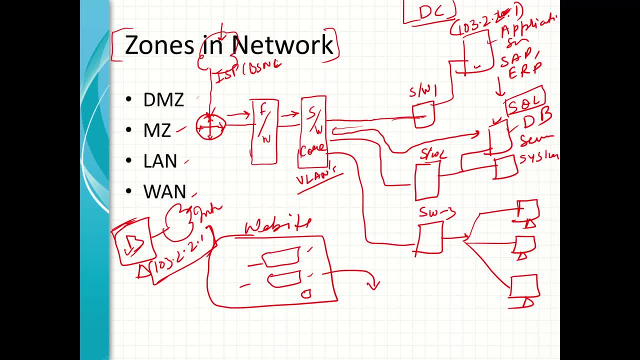 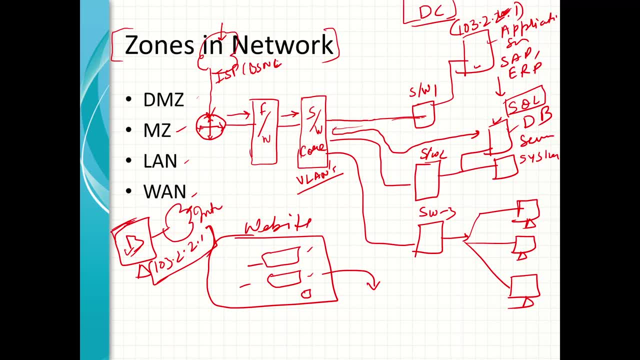 is it yes or no? yes, yes, yes. so now I am going to draw the zones. now I am going to draw the zones, but before that I need to cut out these workstations. sorry to interrupt you, so just a basic question. so what is the difference between core switch and other switches here? 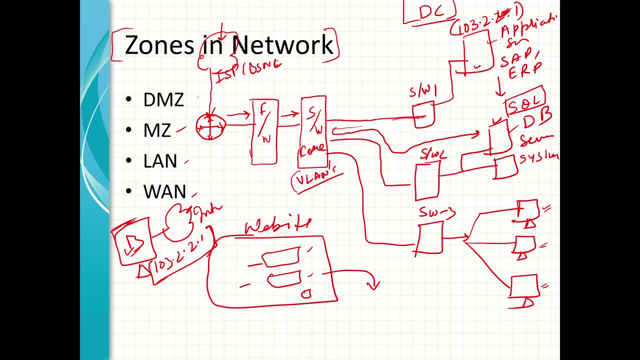 sir, core switch is something which is a all-in-one Okay. So all the network, uh, like you can say, all the network rules, uh that, what are the different vlans, uh who will be assigning the which uh ip pool? so all these works are usually done. 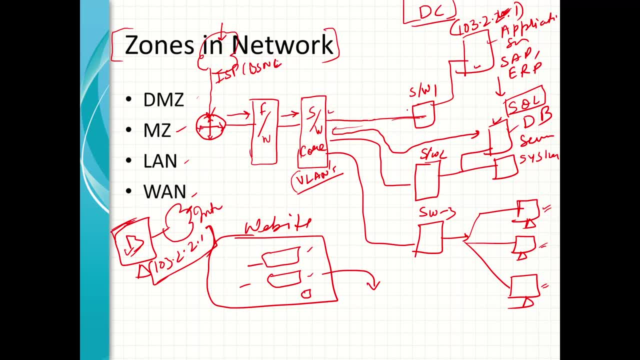 on the core switch. actually, these switch are same. these switch are same, but usually cores which are having a higher, higher capabilities because they need to switching the data very fast on a very high, high rate. so probably, uh, a high capacity switch is used as a core switch. so you need to have a layer 3 and layer 4.. 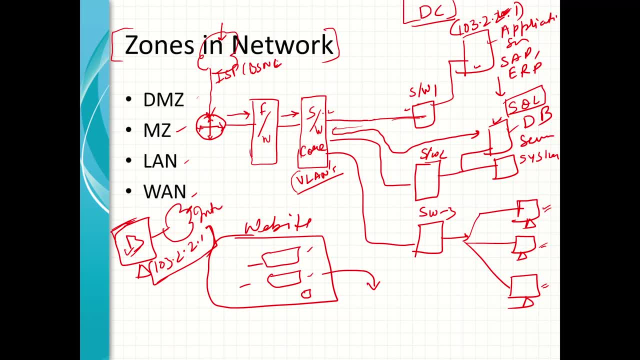 Thank you, Because rules are defined. yes, rules are defined in the core 3 for communicating with the switches. perfect, perfect, sir. perfect, okay. we need to have a layer 3 switch, sir? yeah, definitely, because, because it is, you are going to write ip table, okay. so till now, any issues there. 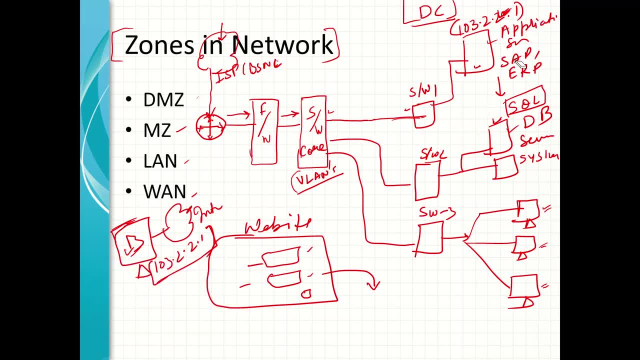 is. there is one clarification, sir, can you tell? Yeah, Yeah is going to access through the switch three to the application server, switch one. so this is going to be a truly internal communication. this need not have any connection with the external side. yes, yeah, so when he sends a query, when he sends a query, it goes via switch three through the core. 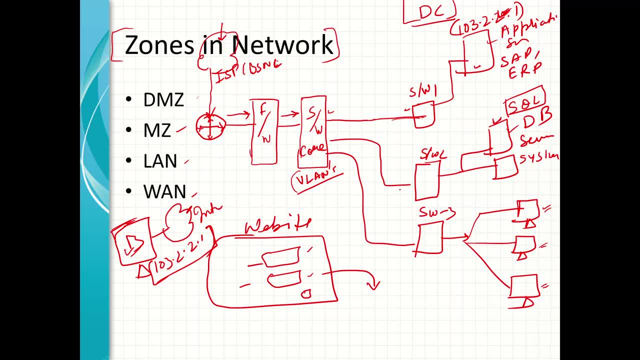 switch, then switch one. yes, yes. after this, you said that the database is also holding some data, so from the application server it will come back to switch one again. it will go back to switch two and fetch the data data. yes, is it right our understanding that, yes, yes is it it is right? 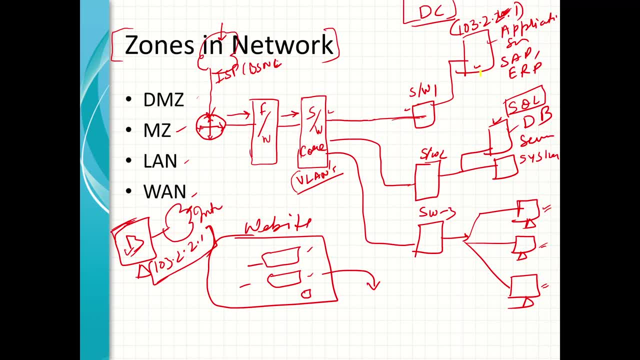 now, what i am trying to say is that switch one can't access this. okay, so this application server can access this, but these users also cannot access this. okay, these users cannot access this. which is these users, workstation users? okay, okay, for for accessing the application they need to go. 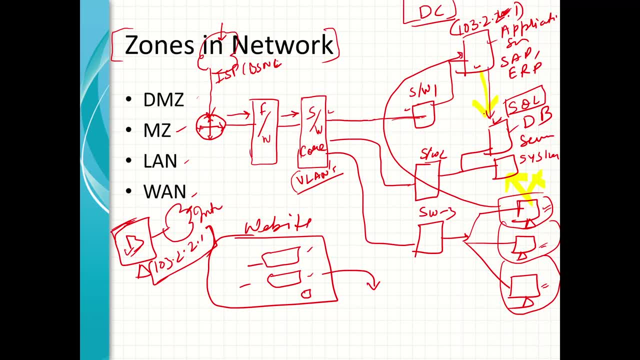 to the database. this is application server and only application will talk to this, understood? so so this is a communication. okay, let me delete all this so that. okay, now just think of a scenario. if i put it in, if i say this is a single zone, and let us suppose, if i say that this is also a single zone and if i say that this is also. 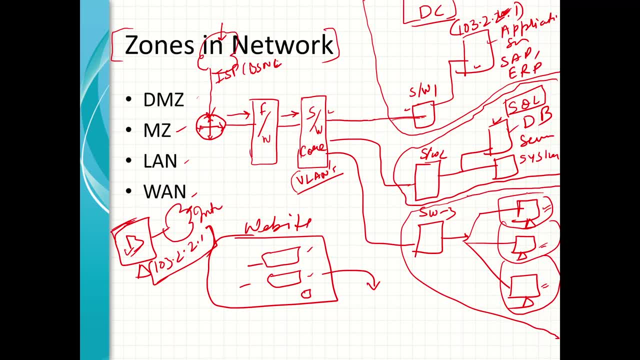 a single zone. so these are different zones, yes or no? your sketch is not reflecting the zone. whatever you are drawing there now it's appearing, there is a time like yeah, so these are different zones, zone two and zone three. okay, so if i say yeah, can i? i? i i'm asking you a question. can zone three talk? 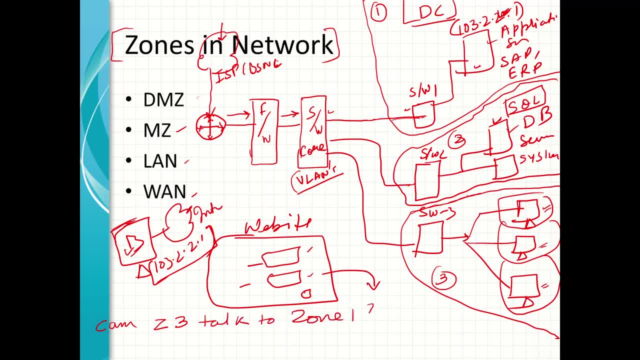 to zone one, Yes or no? Yes, Without core switch. No, Can zone 3 talk to zone 1?? Yes, because workstation also need to access the application. Yes, it can talk. Yeah, it can talk, Can? Okay, now again question. 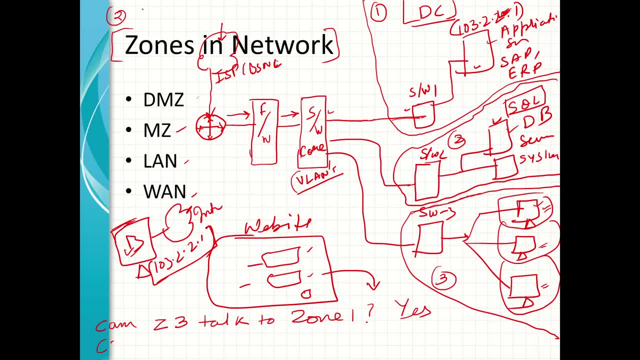 There is a pan issue. My second question is: Can zone 3 talk to zone 2?? No, No, Because every time zone 3 will go to zone 1 and zone 1 will talk to zone 2 and get back the replies. 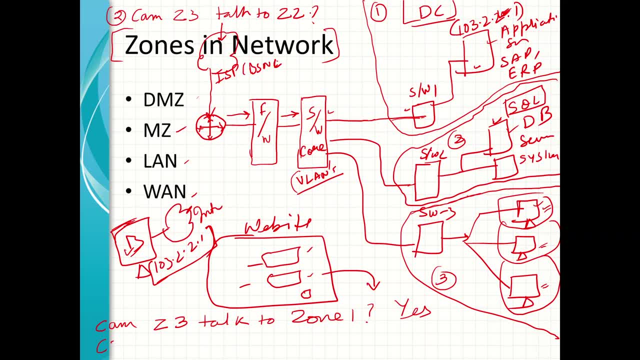 And then it provides to zone 3.. Is it fine? Yes, I am not able to see the screen here. Can you please reshare it? It is visible to us. It is visible to us. It is visible to us. I am just confirming on my second laptop. 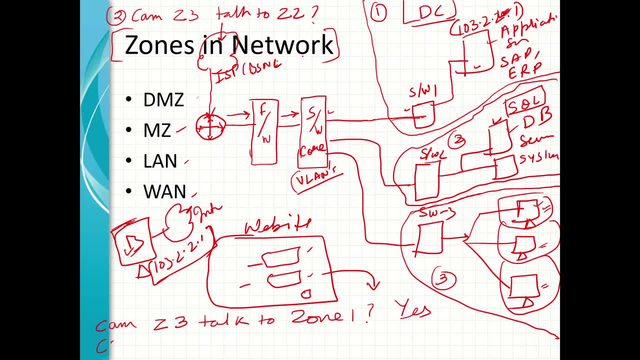 It is visible to us. You can try to log out and log in again, sir. Yeah, I will log out and log in again. Okay, so I have not talked anything about DMZ, AMZ, LAN WAN. I am talking about different zones. 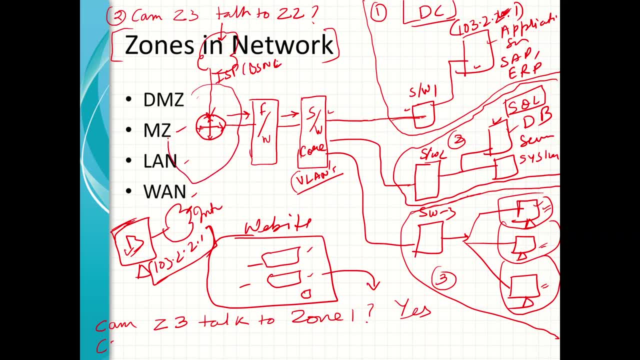 in your network And this is a separate zone. We called it as a zone 4.. Can I say it as a WAN? Yes, Now coming to the definition of DMZ, You have studied DMZ yesterday. What are the DMZ definitions? 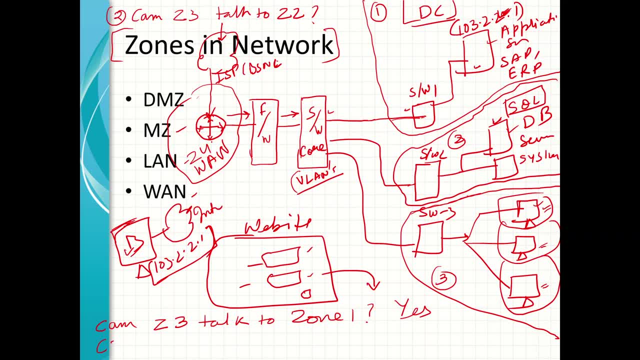 When you want to protect your data or your application servers directly from the internet, you are putting it on to a separate zone, So can I write it as a DMZ? Okay? So this type of zone is called a DMZ zone, Okay. 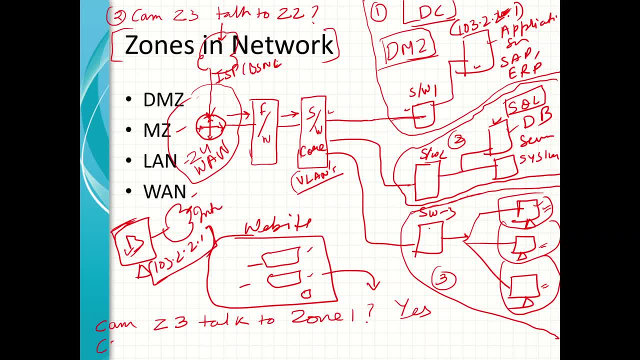 Can you repeat the last one, zone 4, once again, sir, Sir, zone 4 is WAN zone. Your internet, where your internet is landing, You can call it as a WAN zone. Yes, Okay, I will take one more example. 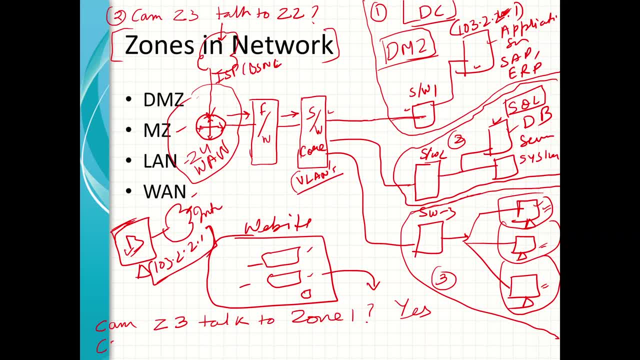 I am going to give more time on this concept. because zoning in network is very important? because, until and unless you do not understand the zoning in network, it is very hard to configure a firewall. Okay, So, rest assured, I am going to solve queries of each and every. 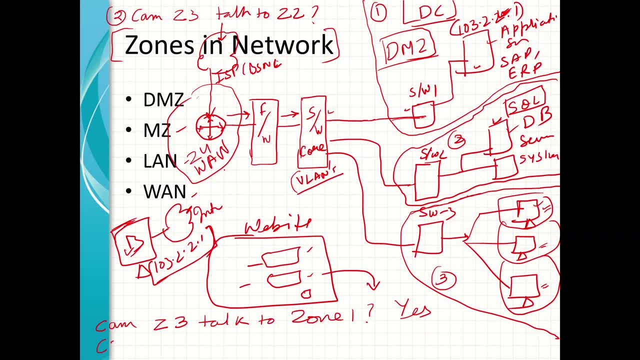 participants. Okay, So don't worry about it. Okay, So this is a WAN zone. Any problems up to this? No, sir, So now this is a DMZ zone. Okay, DMZ- Demilitarized zone. This means your user can access. 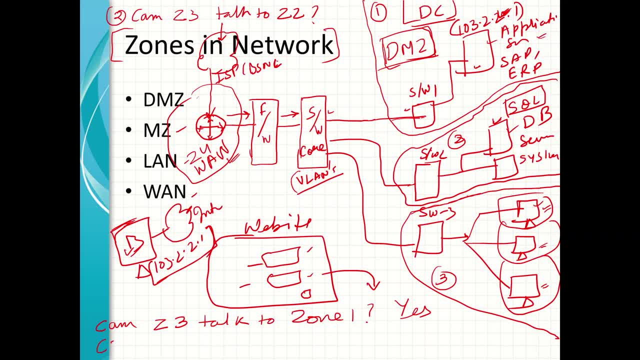 to this application server by having a proper network security peripheral devices on the boundary. Okay, Now can somebody tell which zone is this Out of these four? which zone is this? Public zone? Land zone, I can say, Because this is a local network. 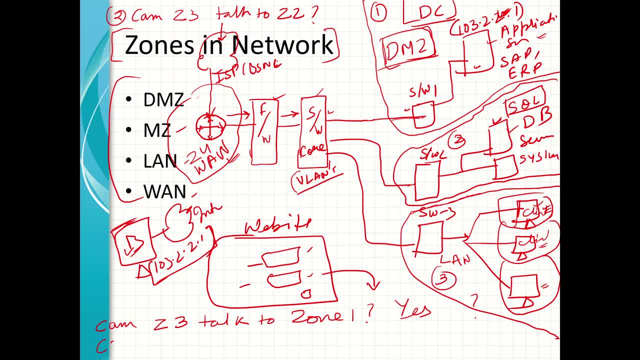 Your clients are here. Yes, sir, Okay, This zone is called militarized zone. Okay, This zone is called militarized zone Why I have told, given it is a name, militarized zone, because it is more secure than this, because this application server is. 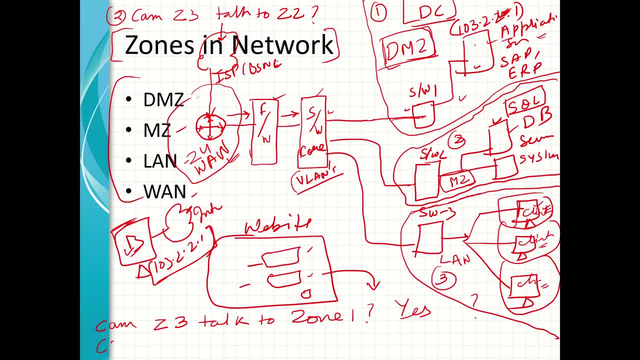 because this application server is publicly visible. Sir, your voice is cutting out. Yeah, ma'am, Your voice is gone. Now I have audible. Yes, sir, Yes, sir. So I've talked about DMZ and MZ. Okay, Now take it as a new. 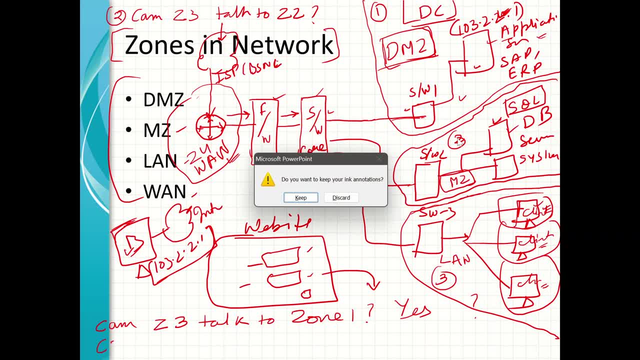 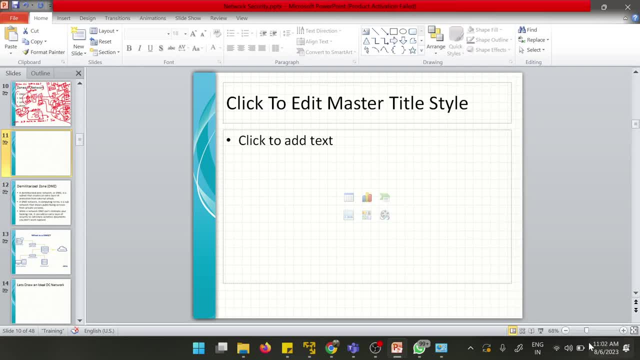 Excuse me, sir, MZ is managed management zone or militarized zone. No, militarized zone. MZ is militarized zone. Okay, Now I have a simple question from you people: which is the most secure zone in your network, MZ or DMZ? 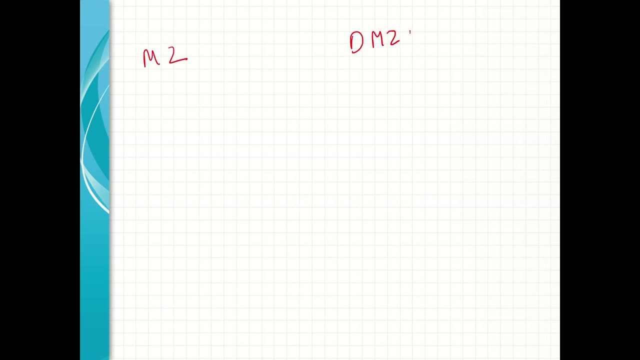 MZ. MZ because it is having a least access. It is a local, It is having a least access Right And DMZ is actually a public. access is there because the the people who are on the internet, they can access the application. 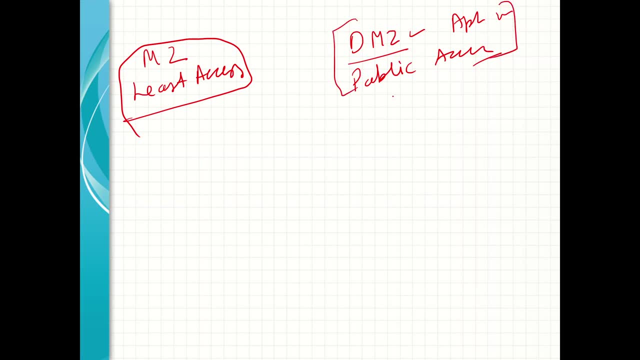 websites on this DMZ zone. Is it fine? Yes, sir. Okay, Now I am going to introduce a new concept for you. Sir, are you saying this application server is DMZ and others are local access zones? that is MZ. 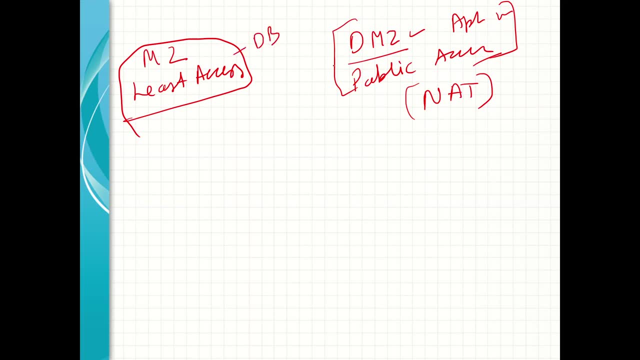 MZ usually contains DB servers, which is DMZ. These applications need to talk to the DB. Okay, Just tell me one thing Which is most precious thing for you: Your DB, or application Database. Your DB is most precious database, So maximum efforts. 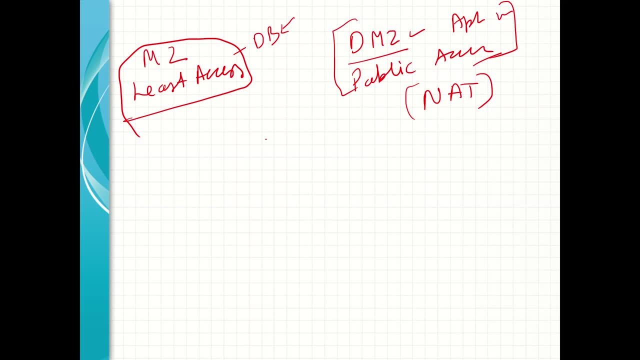 you people do for DB or application DB. Okay, Let us take one scenario: In a single server you can put application plus DB, and in a second scenario you put two servers: One is application and one is a DB server, Which is more secure. 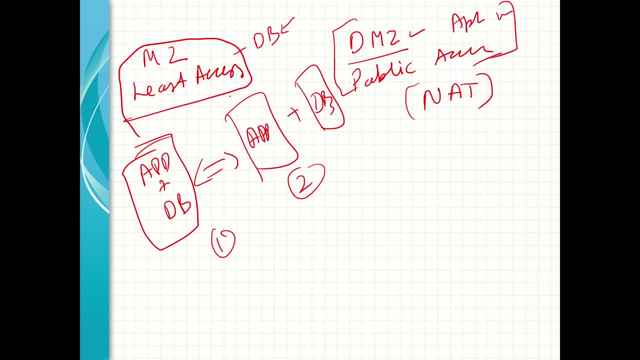 Second one, DB, Because in case this application server is being hacked, at least you have a DB server, You can restore the application, but in case, if this server is hacked, all the app and DB will be gone. Understood now, Yes, sir. 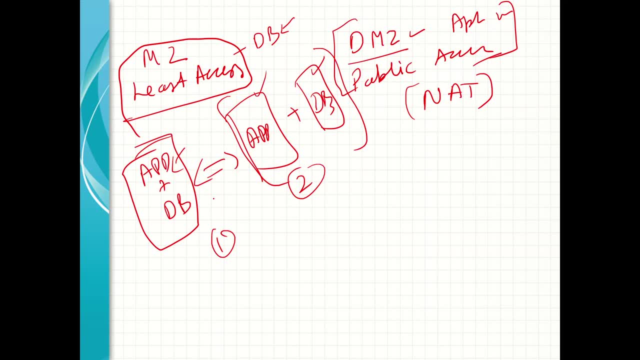 Everyone. Yes, very much, Yes, yes, One question is there? please Please repeat once again Which one. Just this slide, Just this slide, Okay, okay, I will repeat. No issues. I have said that you have two type of 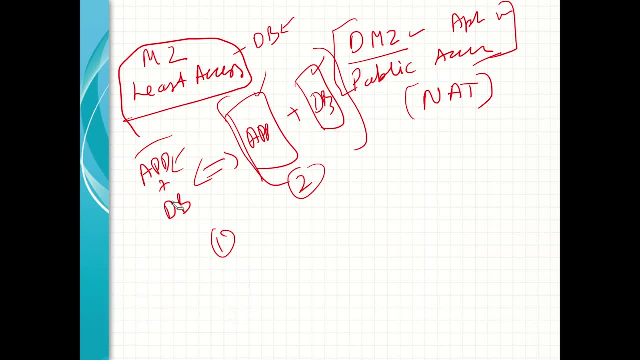 scenarios: Okay, Okay. You have basically two type of scenarios. You have a server one, and in which you have an application and you have a database also. It means you have deployed two type of services, or application services and database services, on a single machine. Okay, On a single. 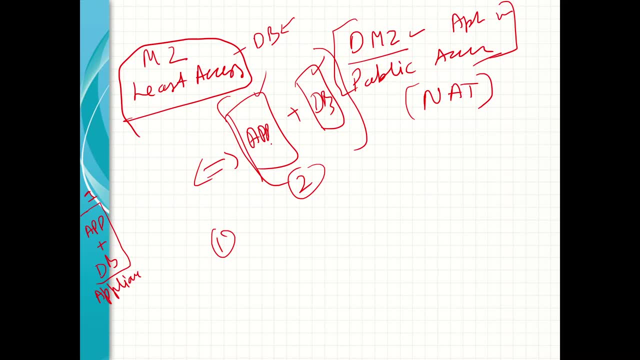 appliance. I would say, On a contrary side, you have used two different server, one for application and one for database, in the second scenario- This is the first scenario, This is the second scenario and in case I am asking you that which is a more secure first, 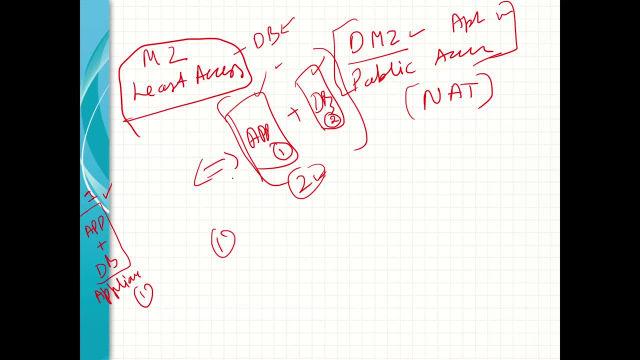 scenario or second scenario. You tell me Second scenario. Second scenario Why? Because we have a segregation of information. We have an application on a different side and database on a different side, So in case we have a ransomware on an application, 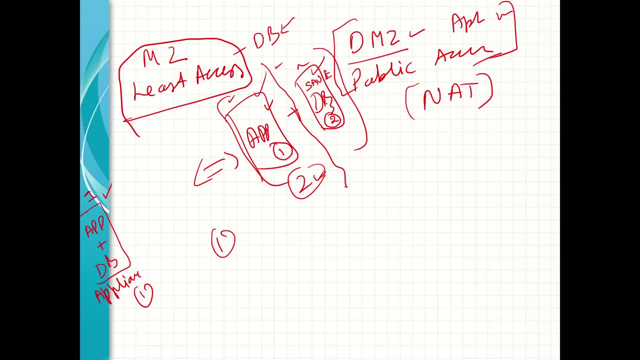 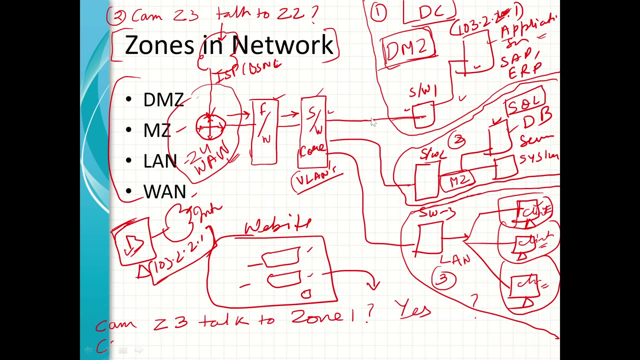 server. at least we can save our database server. Yes, sir, Yes, Okay, So this is the basic concept why the zoning are required. because now, tell me, in this previous network, in this previous example we have talked. let me ask a simple question from you that 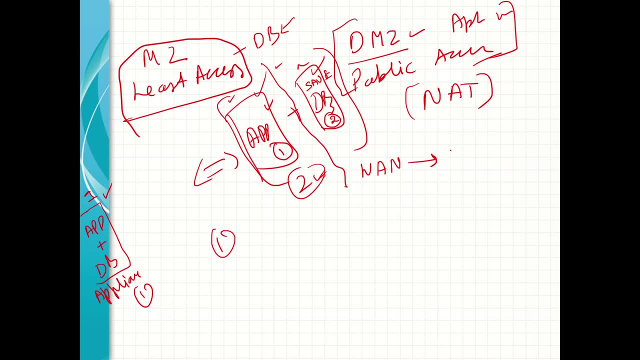 from when zone zone. okay, now we- I am talking in the name, not zone one, two, three or three, because now you people know that what are the MZ and these zones? Okay, from when to MZ. MZ to when: okay. DMZ to when LAN. 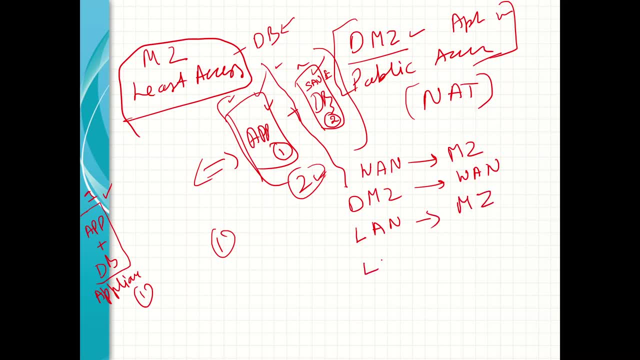 to MZ and LAN to DMZ: okay, tell me, in previous scenario, is it allowed from when to MZ? not allowed, not allowed, not allowed. okay, DMZ to when allowed: allowed. from LAN to MZ not allowed. not allowed. from LAN to DMZ: allowed. so now you know. 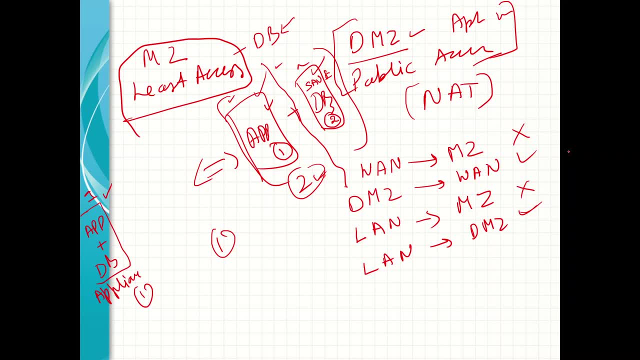 basic zoning functionality and now you can create a rules in firewall. I would say that what are the different zones and what are the rules to make them allow? now is it now it is clear to you people? I think now you have a better visibility. yes, yes, it is clear. 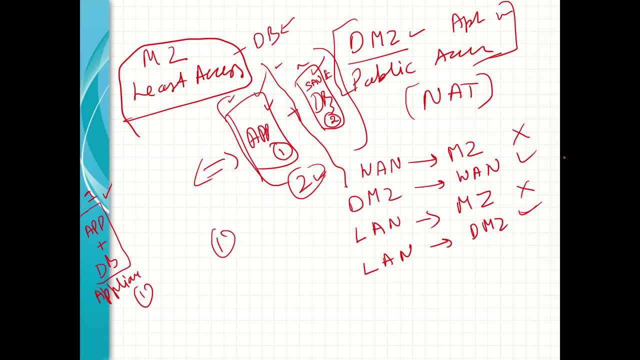 still have. LAN is actually connected. LAN is the- I mean zones connected using core switch, right? yes, so in that case from the application server we can talk to DB server. it is connected. yes, so DB server is the militarized zone. yes, and from LAN or via the switch. 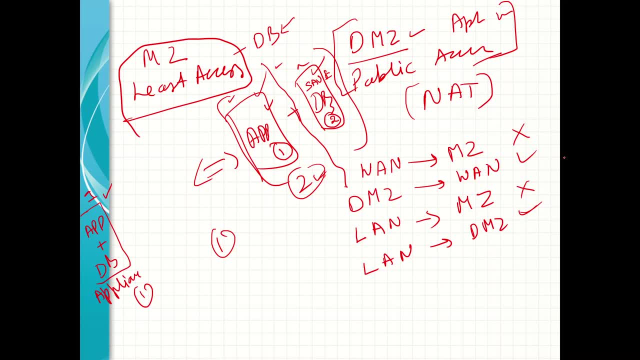 I can contact the militarized zone, right? no, no, it is actually blocked now by using the. when you have configured the VLANs, you have not passed that VLAN to the MZ zone and we configure only the application server. in that way, we set the rule. that's what you meant to say. 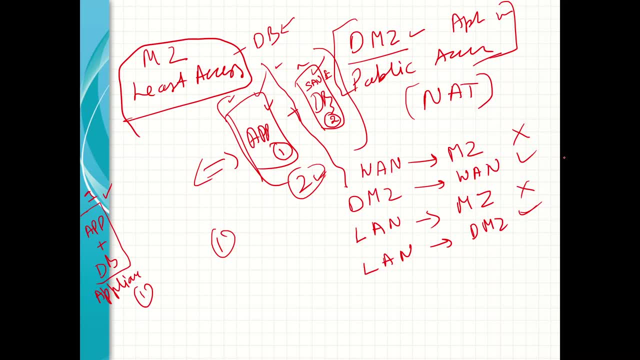 yeah, yeah, yeah, sir, one more main LAN also required. yes, one more rule is required. definitely, rules are required, but I am just asking on these four rules, that is it. this is happening in the previous scenario or not? ok, sir, are we going to learn how to configure this on? 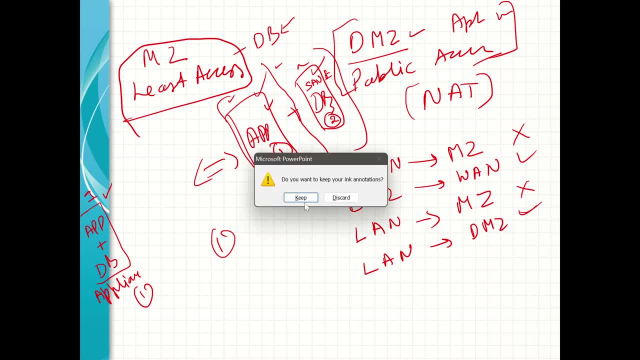 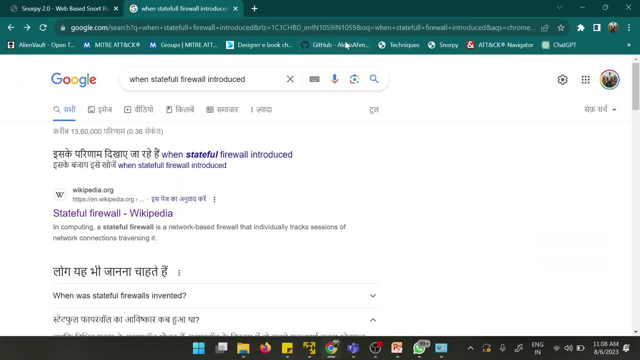 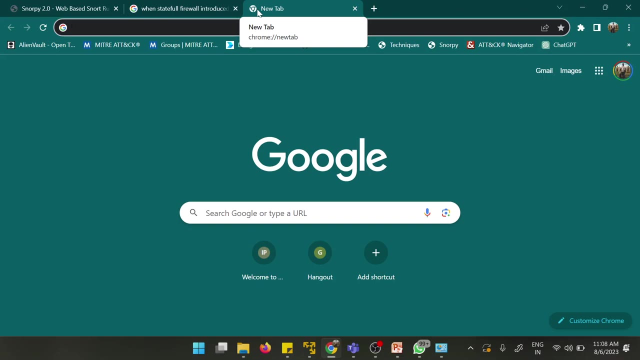 core 3 switch. yes, we are going to do it. right now. we are going to see a live firewall. I have just bought for you people. only, sir, there is one question: under what condition you will access this militarized zone, MZ? under what condition, who will access? 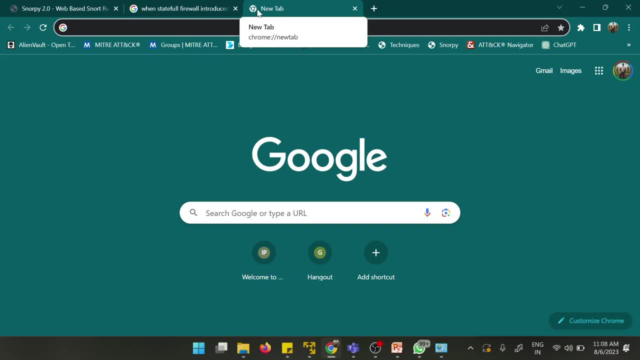 all this combination, in this combination, we are not able to access this MZ zone that is militarized zone. so under what condition? yeah, under what condition you will allow, the MZ zone will be accessed. actually, in this network architecture that we have described right now, we have configured in such a way. 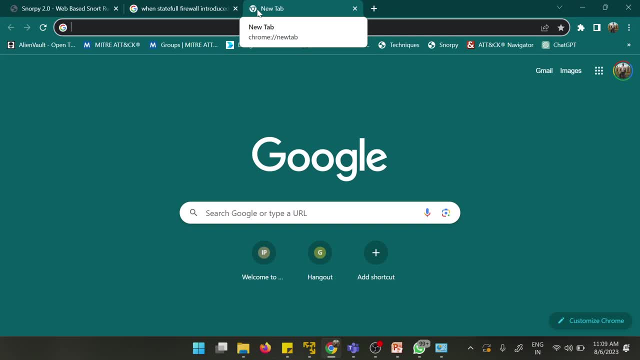 so that only DMZ can talk to MZ. ok, other than DMZ, nobody can talk to MZ, because MZ is the most secure part of my organization. I am keeping under the layer to layer mechanism. ok, got it, got it, sir. one request, sir. I was out of the 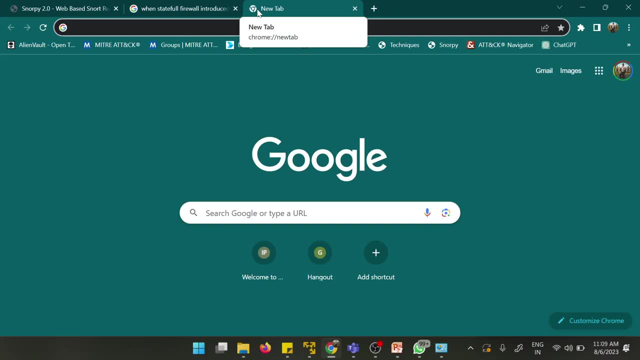 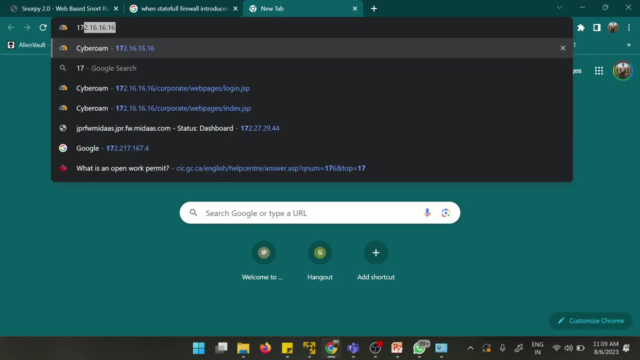 network for 5 minutes, like so I understood, till there were 4 zones. 4 was the internet zone and after that. could you please just explain? yeah, ok, I will. I am going to show you a live firewall so that things are getting more clear to you, ok. 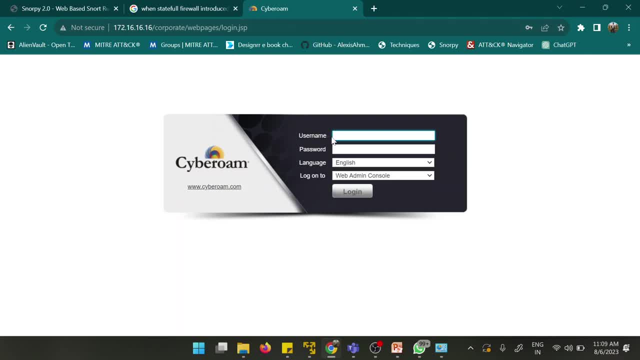 ok, adjust. what was zone 1, 2 and 3? what was DMZ, whether it was zone 1 or 2 or 3, just I want to can any participant can write in chat box, sir, I have got one query, sir, related one. sir. there have been 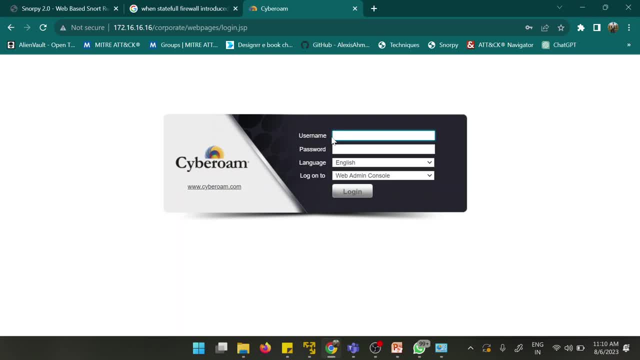 cases wherein the VLAN- since VLAN works at layer 2 of the OSI model, and there have been cases then that VLAN rules because of the misconfiguration or because of the spoofing and other attacks, it has been compromised. so don't you recommend an internal firewall for such a? 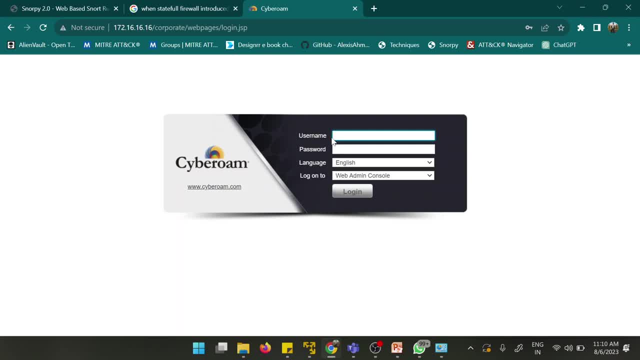 architecture in. nowadays, in practical scenario, firewalls are keeping in place for all these VLANs. even UTM's are the perfect devices. you can use them as a code switch, ok? ma'am Rohit ji has stated about the different zones. you can check out there, ok, thanks sir. 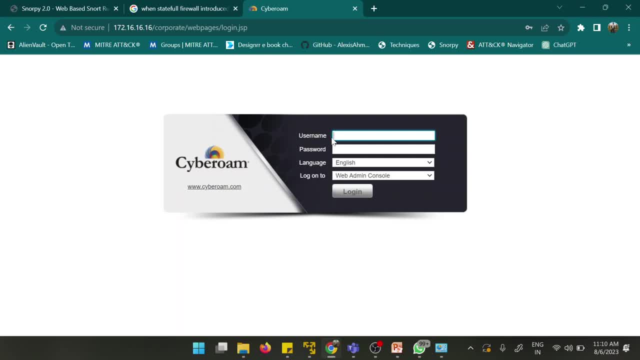 ok, so now we will be focusing on a firewall I have put down, I have installed a firewall in my network, in my home network, and I am going to tell you that, what are the different zones and how the rules are created for a zone. ok, so can we start? 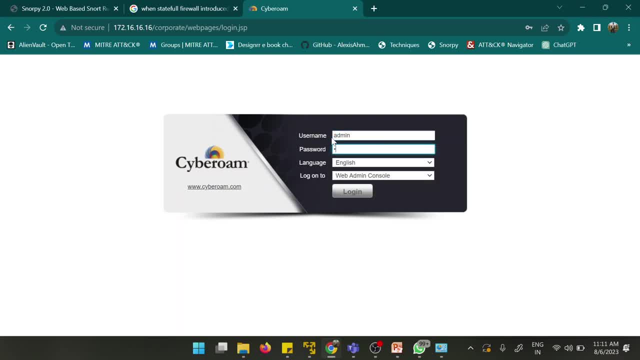 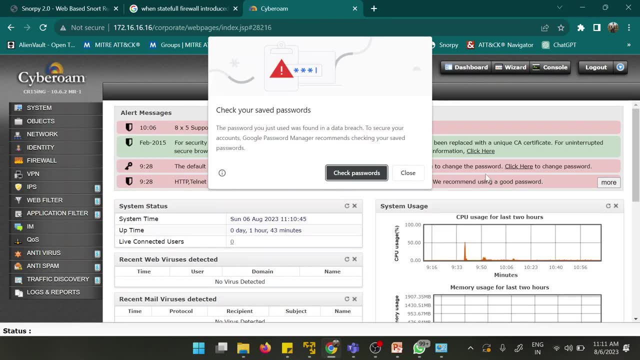 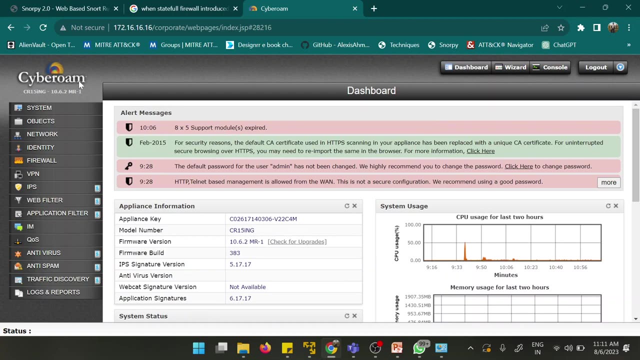 yes, sir, yes sir. ok, so this is a basic interface of a firewall I have put down in my network. this is a cyber home firewall, and now it is discontinued, actually, and cyber home is being take over by sofos. ok, so now you are not able to. 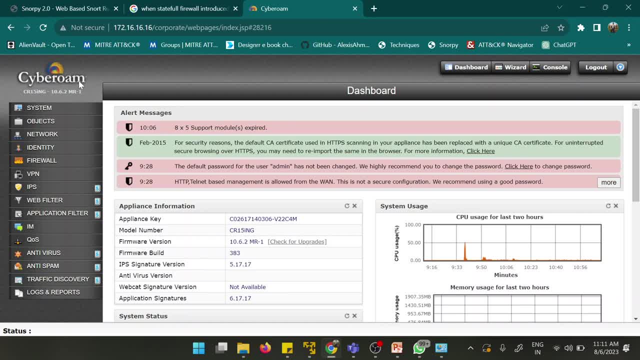 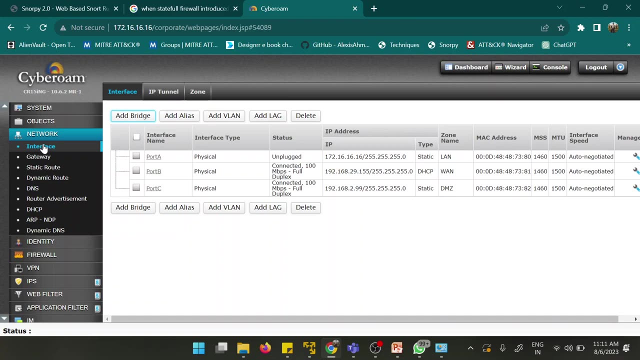 see some cyber home or something. now you are going to see this sofos firewall. ok, so what I am going to deck? then, whenever you check a firewall, you need to go to the networks and to check the interfaces. ok, you need to go to networks and check the interfaces. 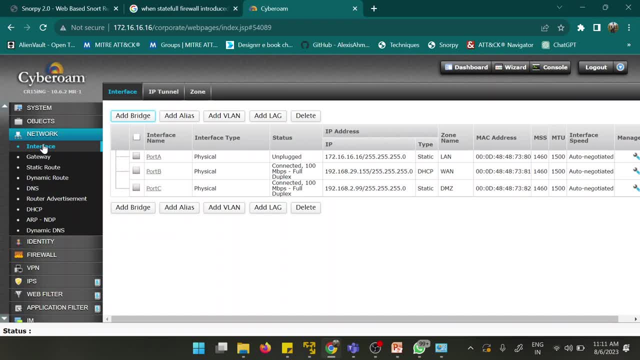 because every firewall has a number of ports, like 4 port, 8 port, and I would say there are very costly firewalls are having 8 ports or something. mostly normal firewall of 5-6 lakh rupees having 5 or 6 ports usually. 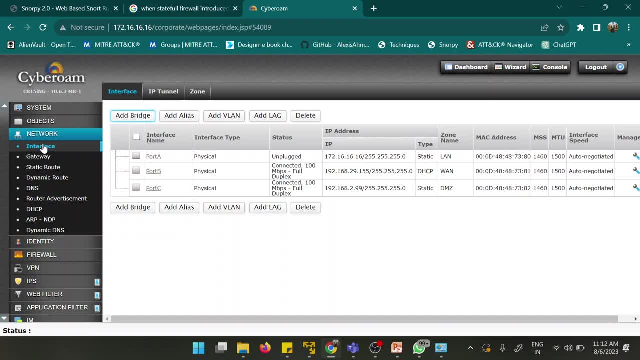 ok, because number of ports will increase the complexity of a firewall and complexity of a firewall will require a higher machine power, a higher processing power, so it will increase the cost. ok, so in this firewall I am having 3 ports where port A, B and C are defined. ok. 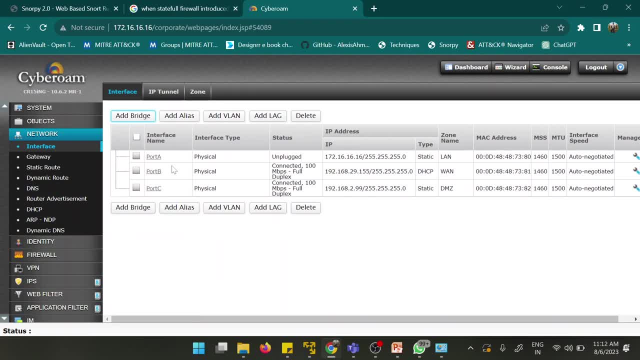 if you configure a firewall, there is no definition for port A is MZ, port B is WAN or port C is DMZ. it is all depend on us that how we are going to configure that firewall. ok, so in this case, on port A, I have configured my LAN. 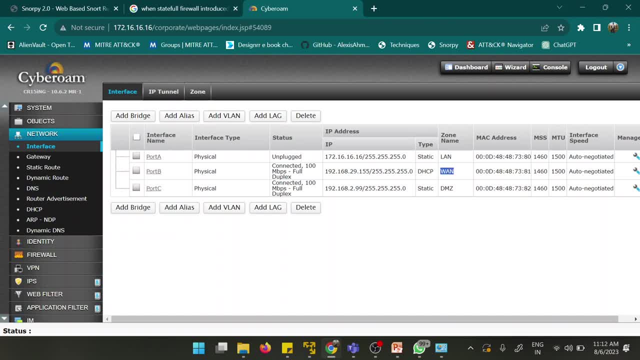 section. on port B, I have configured my WAN section and on port C, I have configured my DMZ section. ok, I have not configured any MZ section because I am not having any servers or something, but I have configured only these 3 LAN sections. ok, now you can see that this 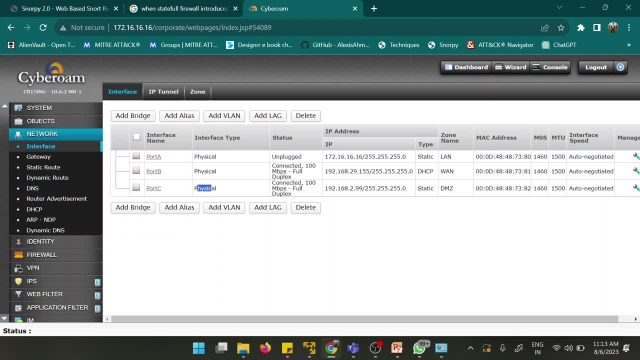 interface is physical. ok, one physical interface and only 2 connections are currently up. port A is unplugged, actually, because I have just connected my Jio router with this firewall and it is taking the IP automatically. you can see there is a DSCP, yes or no? 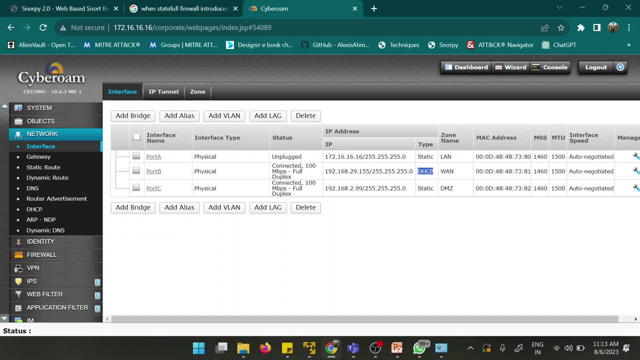 yes, yes, this is a DSCP and Jio is assigning me an IP. ok, so Jio router is assigning me an IP and this name is zone name, is WAN zone and this is the IP that I have assigned, because, you can see, this is static IP, so it is. 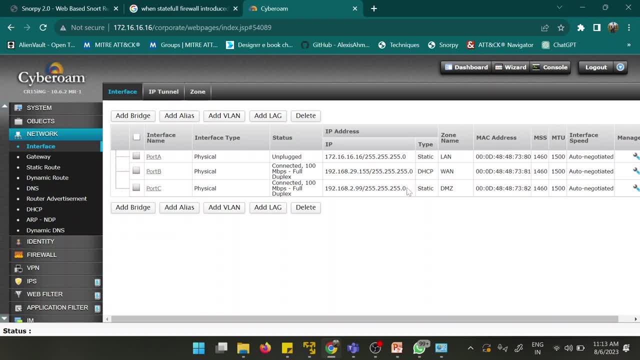 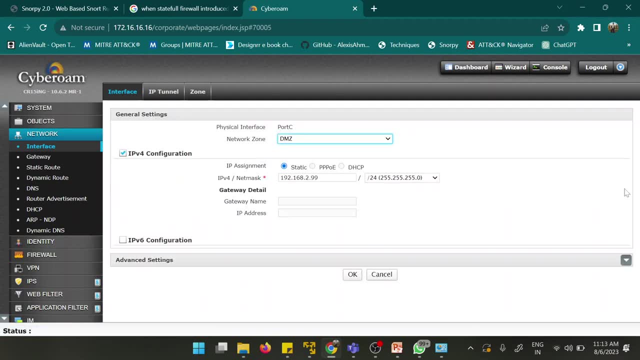 very much clear by looking to this configuration that the person who has configured the firewall has assigned the IP to this. ok, so let us check what is inside the manage section. ok, so whenever you configure a firewall, it will give you an option on which zone you want to take it. ok, 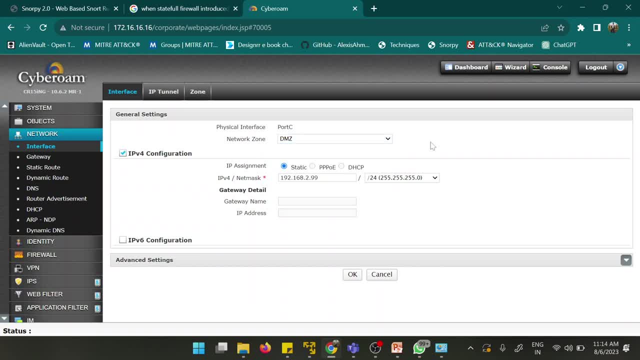 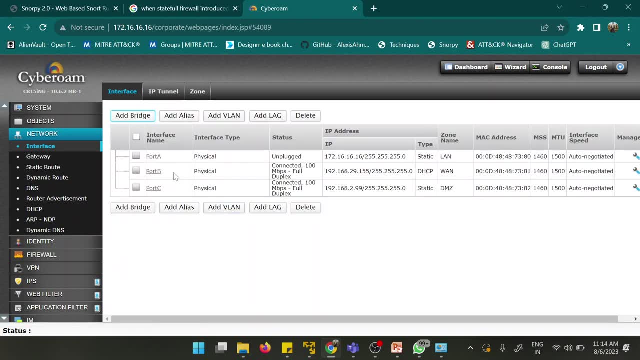 so port C, you can put it on a LAN zone, WAN zone or DMZ, so it is your choice, because when you create a network architecture, you can do it at your own. ok, so this is a simple configuration where one WAN zone is there and one DMZ. 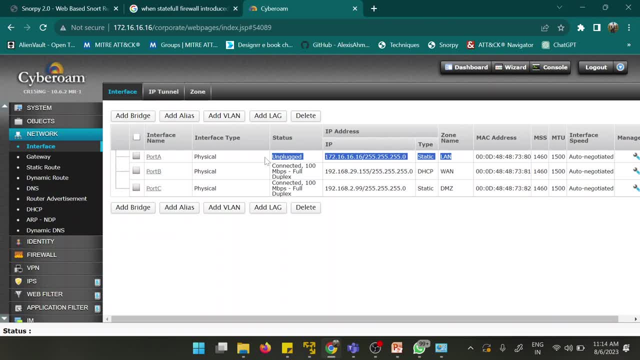 is there, ok. LAN is disconnected because I have disconnected my LAN zone, so these two zones are currently working. so any questions, Sir, what is the difference between static and DSCP? Sir? static IP is I am going to select IP for me, ok, and in the DSCP, 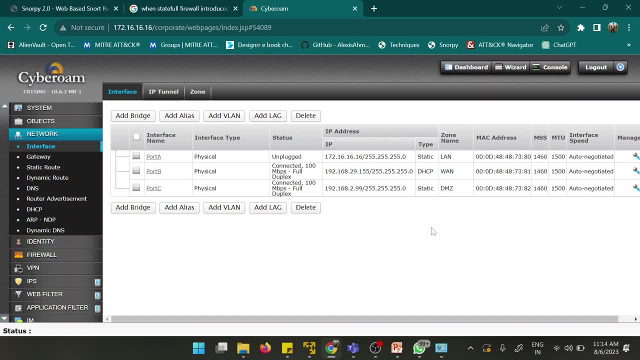 the router is going to assign IP for you. usually when you use the Jio router or some broadband connections to you, they will assign you a DSCP IP, and when you are creating an internal network, you need to create a static IP also. I would like to 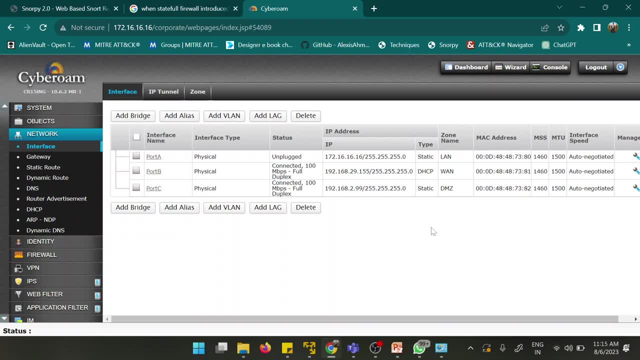 mention in case of an internal network. if you have a very large number of computers- workstations like 4000, 5000- you can put down a DSCP server and that DSCP server will assign IP, because manual IP configuration is very hard for a long. 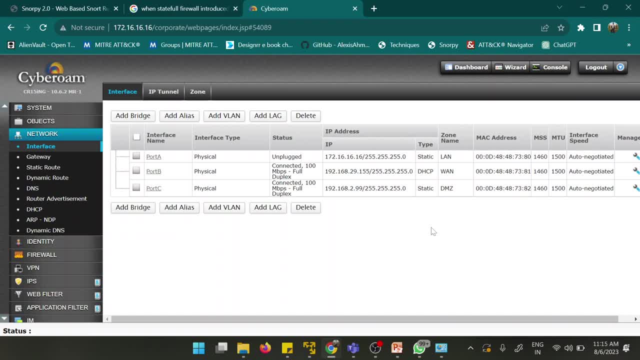 networks, for very large networks. ok, ok, sir. what is the form of DSCP, sir? what is full form of DSCP? dynamic host control protocol: ok, dynamic host configuration protocol is there and it is a separate service. it is a separate service and this service can be activated on a windows. 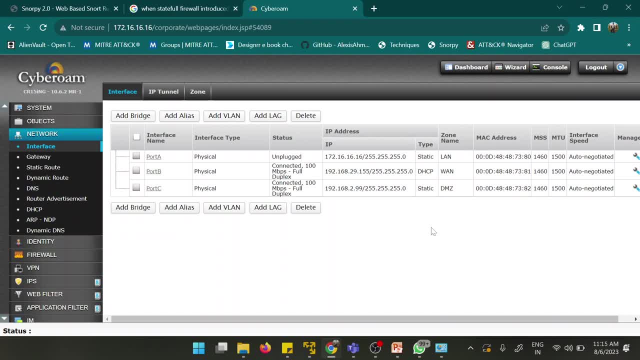 machine and this windows machine will acting as a, as a provider for IP for your upcoming network clients underneath the DSCP server. is it downstream, downstream side? you mean to say it will provide IPs to downstream, downstream side device? yes, yes, yes, ok, ok, somebody is asking here, please. 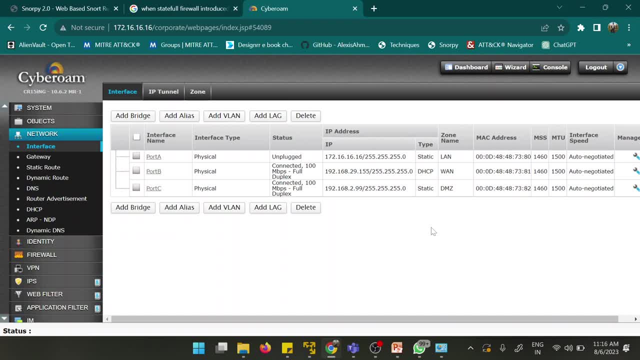 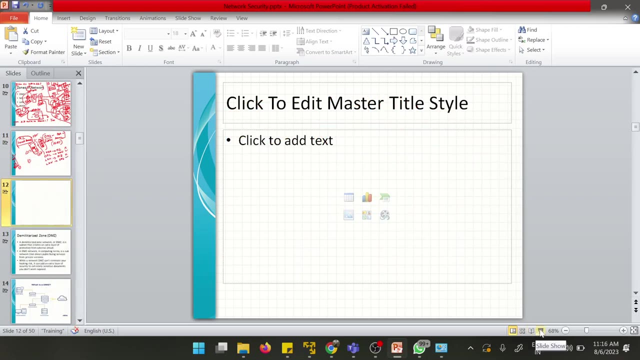 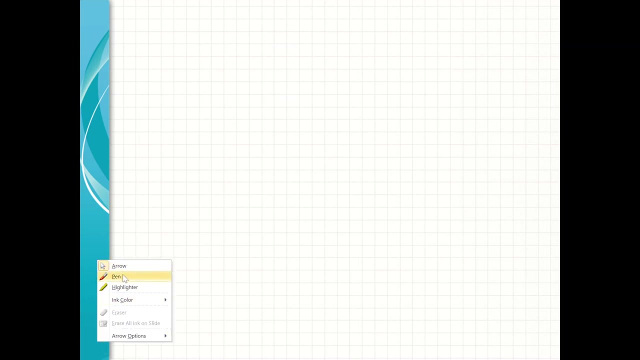 the static IP and public IP. both are same. no, no, static IP and public IP are different. ok, let me, let me talk on this thing. this is a very confusing question, I think, so I need to speak a little bit on it. is my screen visible? yes, ok. 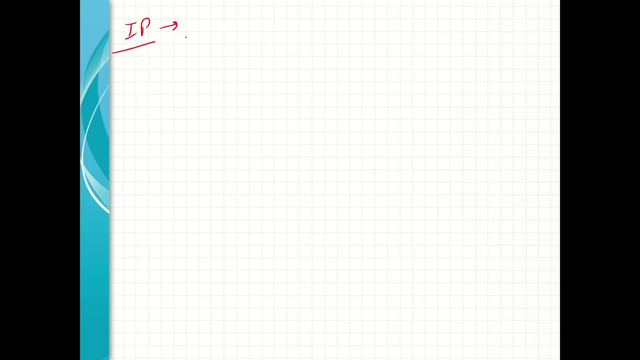 look, when we talk about IP, what is the full form of IP? internet protocol, internet protocol. basically, it is a address. it is a address, yes or no? yes, ok, ok. just think of a scenario: this is your home, this is your home and this is your bedroom one. 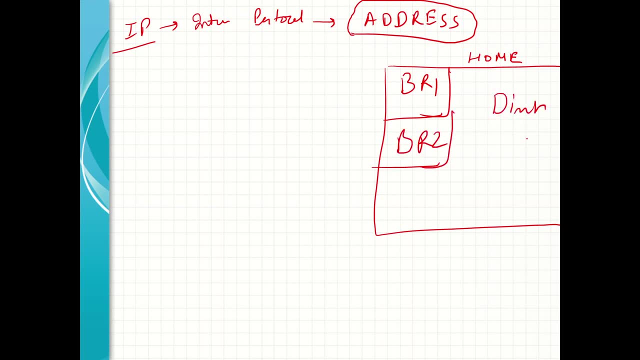 this is your bedroom two, this is your dining and this is your kitchen. ok, and this is a rest area, is it fine? and this is a study room? yes, sir, now your father is standing here and asking a person here. ok, that that Ram Ram is the name of the person. 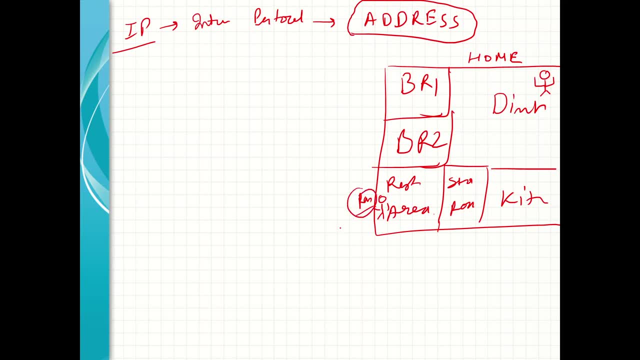 Ram come to dining room. so where the Ram will go in dining room, he will go to dining room. ok, is it fine or not? yes, ok. now think of a scenario that there are lot of dining rooms in a. there is a dining room in every home, so how to identify? 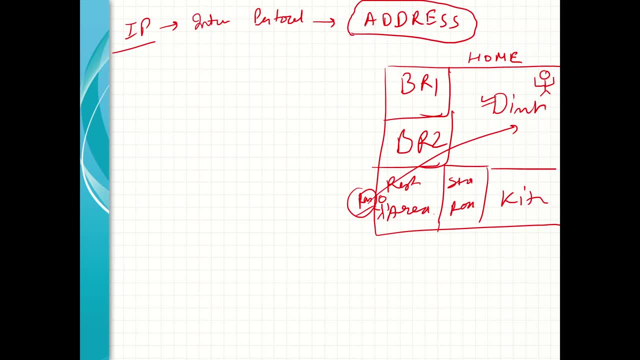 how to identify a particular dining room of a particular home. you need a address for that. if i say that this home address is 112 alok vihar delhi, ok. if i say, go to the dining of 112 alok vihar delhi, then you able to go. 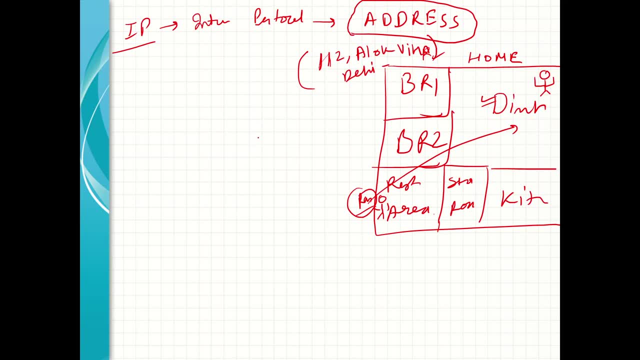 yes or no? yes, and if i say, go to dining room now, single statement, go to dining room, you will ask, sir, what is the address of the home in which dining room is now? understand you this address? this is a address which is publicly exposed. this is a address which is publicly exposed. 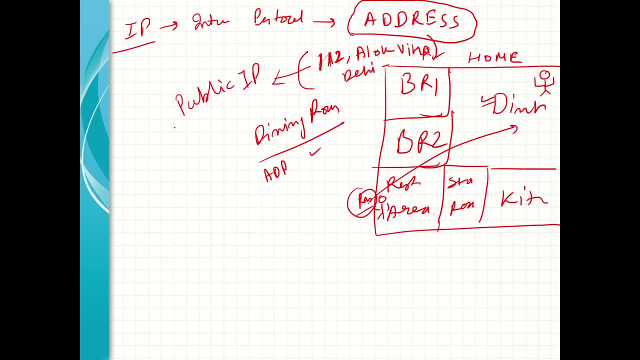 so this is we called it as a public IP. if you send a letter from USA to this address, is it deliverable or not? yes, yes, sir, yes. but if you send a letter from USA to this address, dining room, is it deliverable? no, no, because it is a. 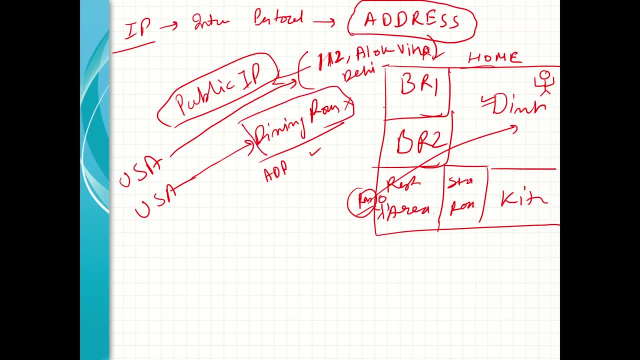 it is a localized address of a particular home. ok, ok, now think of a scenario. you have a, you have a organization of 1000 pc. ok, so every pc you give a IP address, so that, so that that IP address to 1000 pc is basically a local address. 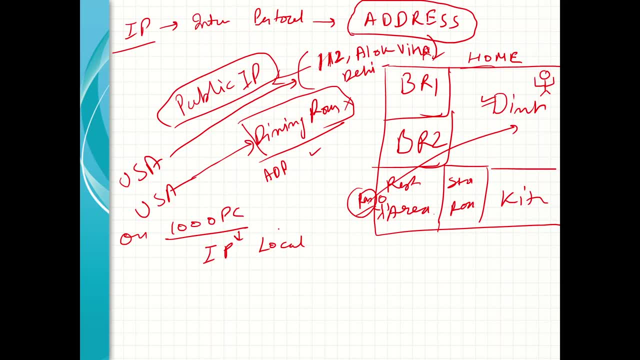 I am not talking on static or dynamic. I am talking about public IP and local IP. ok, so local IP is something that make you restrict to that network only. if I talking about study room, so this study room is of this home only, ok. ok, let us take one more example that you have: a 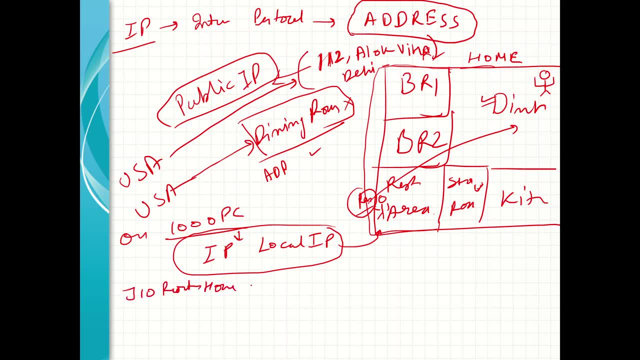 Jio router at your home. ok, and you have connected a switch to it at your home and you connected 8 pc's- 8 pc's to it. ok, now Jio has assigned a public IP to you, let us suppose 103, 22, 22.1- ok. 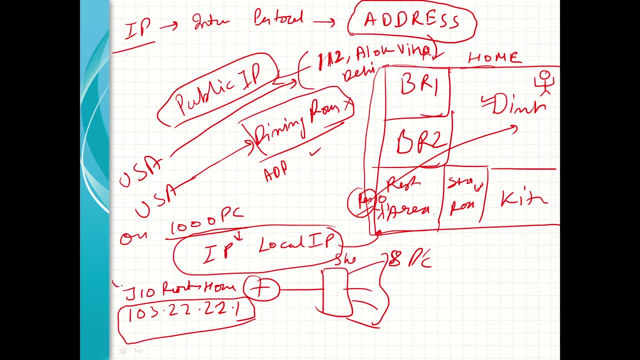 so this is a public IP. your internet is accessible through this Jio router, which is having a public IP, but the internal 8 IP's are not public IP. they are basically your LAN IP's. it is called, I think, private IP. yeah, private IP, you can. 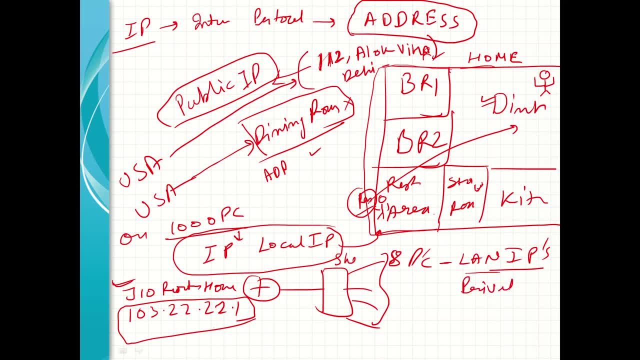 say it: local IP, private IP, not an issue. private IP is also same word. private IP is there, local IP is there, so this is a difference. so if somebody wants to talk to this pc from internet, let us suppose this is your pc and you host the application on this. 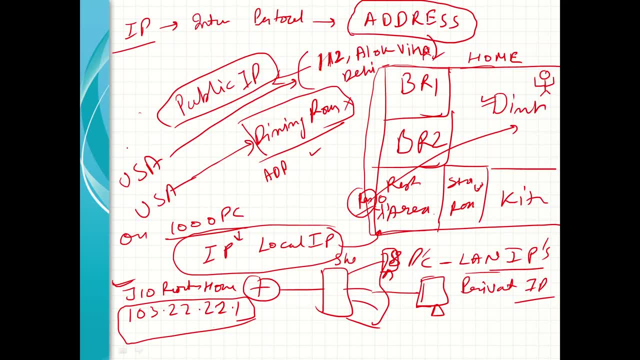 pc. can somebody from USA can access this on this local IP. no, no, no, why? because he is able to land to this only. he is able to land to this only, but you have not directed from this router to talk to this, to create a NAT rule, NAT rule. 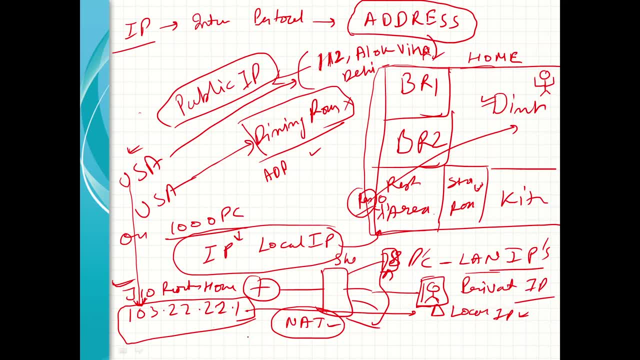 NATing. using the technology of NATing, it can be done, okay. how many people know about NATing? I know that, okay, and what about others? no, sir, okay, so let me. who has asked this question about public IP and local IP? is it clear now? yeah, clear. 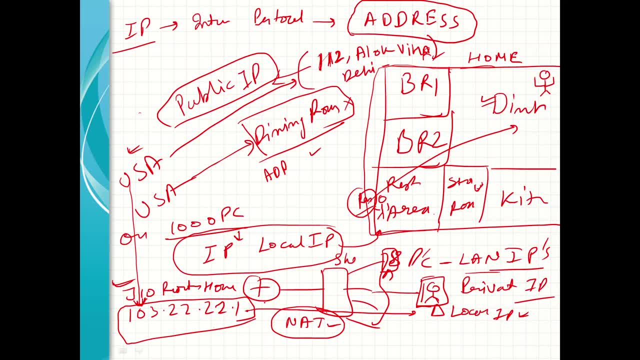 yeah, so the public IP essentially will be the static IP means that is talking about the dynamicity of the IP assigned by the external ISP. yeah, yeah, perfect, now you know about the point. yeah, okay, let me talk a little bit about NATing, then we will go to firewall part. 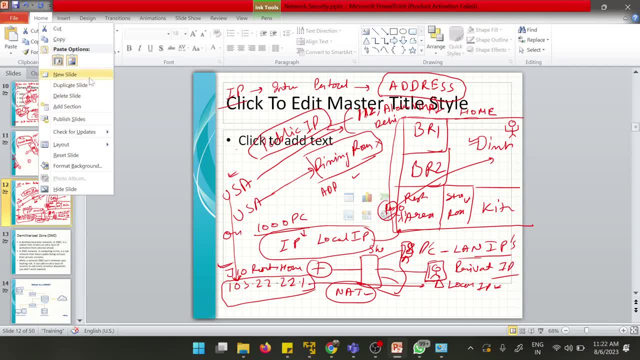 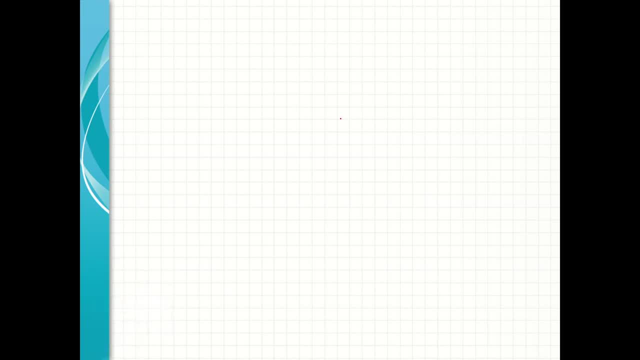 again, okay, NATing. NATing means network address translation. okay, let me take as a scenario that this is a router and you given IP 103.2.2.9 and this is your web server and you given IP 10.1.1.3. 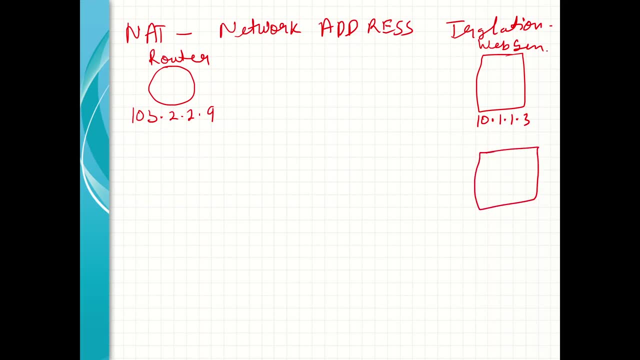 and this is a web server 1 and your web server 2, and you given IP 10.1.1.4. okay, now tell me. this is Mr A, with a smiling face. you want to access this web server? okay, and there is a switch between. 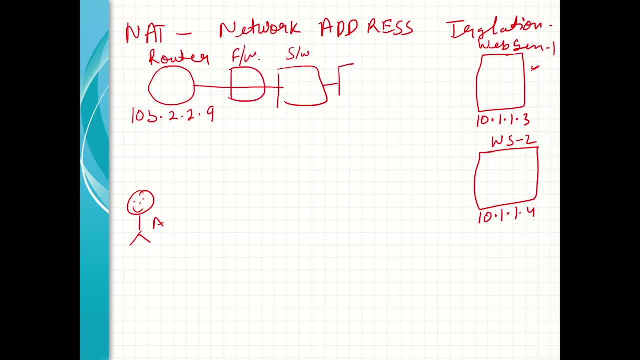 and a okay firewall in between. then there is a switch and then there is a connectivity to these servers. now, Mr A want to access the web server 1. A want to access web server 1. is it accessible, yes or no? no, no, because A know only. 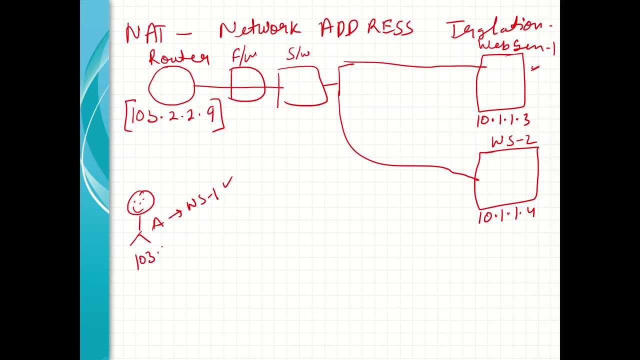 this IP, A know only this IP and the IP of web server is different. yes or no? yes, sir. so what we can do is we can ask a pool of IP, pool of IP from ISP that give me 5 public IP, or I can say 2 public IP. 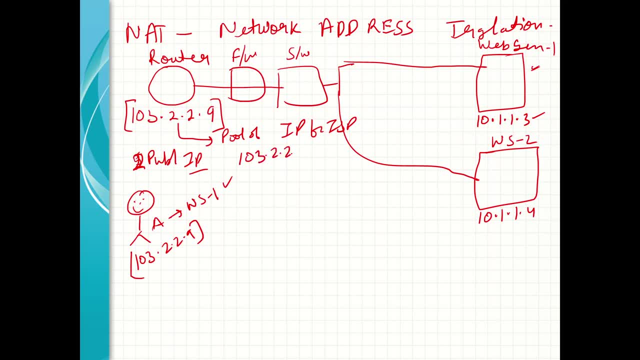 for my network, like 103.2.2.10 and 2.11. okay, now I will create a net table in my firewall where I can map 103.2.2.10 to 10.1.1.3 and 103.2.2.11. 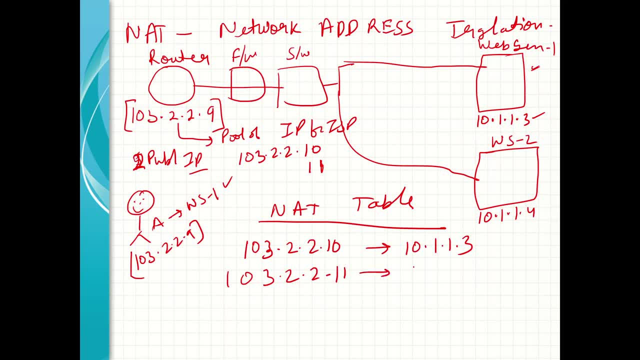 to 10.1.1.4 and 103.2.2.11 to 10.1.1.4. okay, now, whenever Mr A will access the IP, this 103.2.2.11. can anybody tell which web server will be replying? 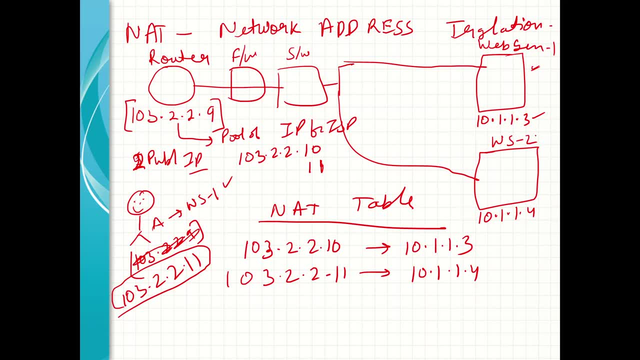 web server 2. web server 2 will be replying okay, and when this 10 is, and when he will trying to access this 10, which web server will be requiring one number? so this is basically network address translation and why it is done so, so that your web server 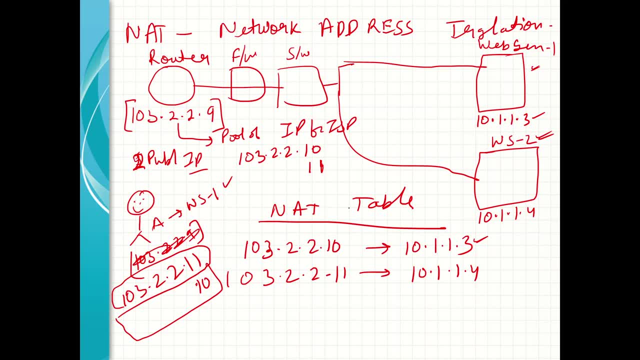 IP is not exposed to internet. this can only also be done if I put this IP directly into the server. if I put IP directly into this server, so the Mr A can directly have access to this server and he can start the NMAP and other. just hold for a moment. 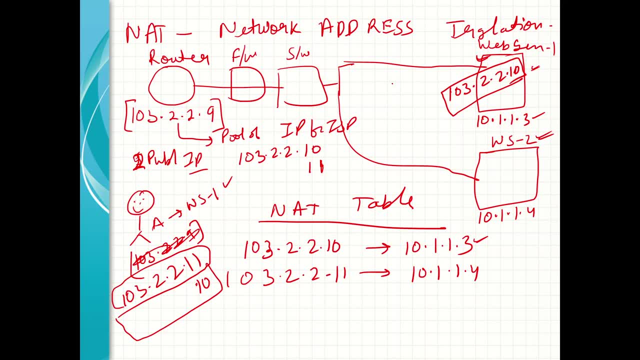 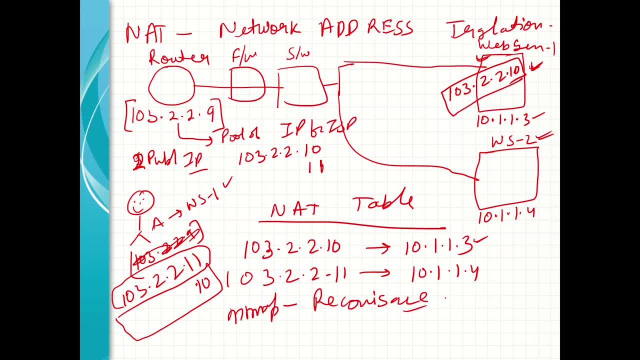 nmap is a tool for reconnaissance when you are trying to find the artifacts. artifacts about the server, that what is the, how many ports are open and how many services are running, which operating system the server is using. so these all the things that is coming in the reconnaissance part. 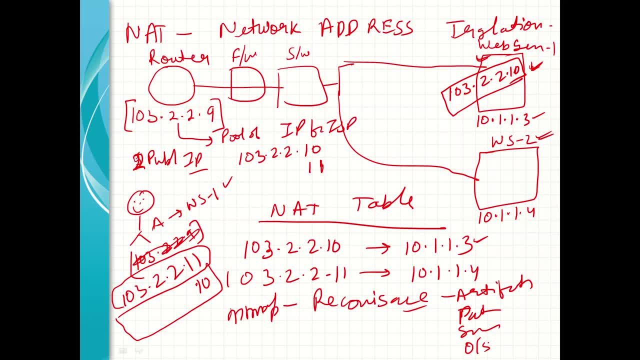 so what do people think? uh, this netting will i have one question? yeah, please. uh, mr pesar, i have one question. yeah, please see the router. you have assigned 103.2.2.9. okay, and additionally, you have taken two more addresses ending with 11 and 10 and 11.. yeah, now you have assigned to web server. 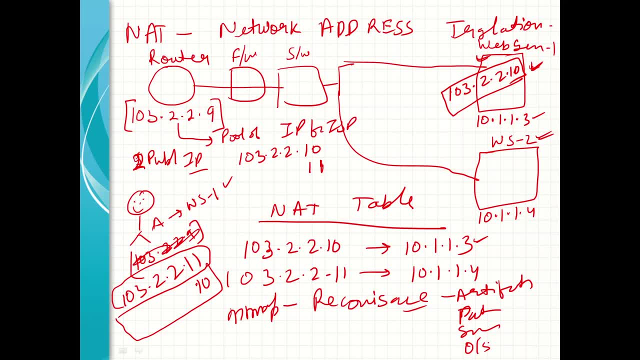 that server 2.. and when the a wants to access 10 without going to the router a 2.2.9. no, it cannot. it is going to the router only. sir, the traffic is going to the van only. this is the van only. it is not going to do that, go directly. but the. but the user a is going to type this: 2.2.11, no. 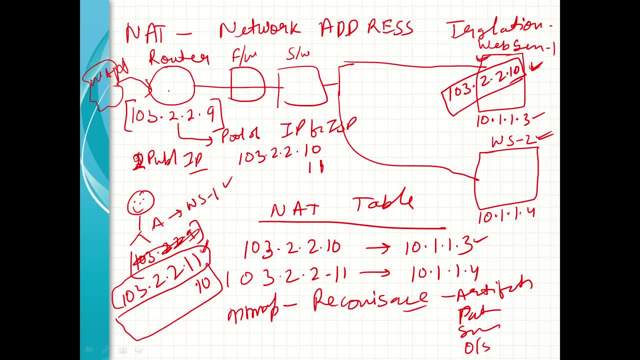 it will type this, but it will land on this, because the gateway for all these, now all the 10, 11, the gateway is 9.. so he, when he will enter this 103.2.9 in this example, he should enter first, then he should enter 10 or 11, right? no, i'm not getting your question. can you repeat? no, no. 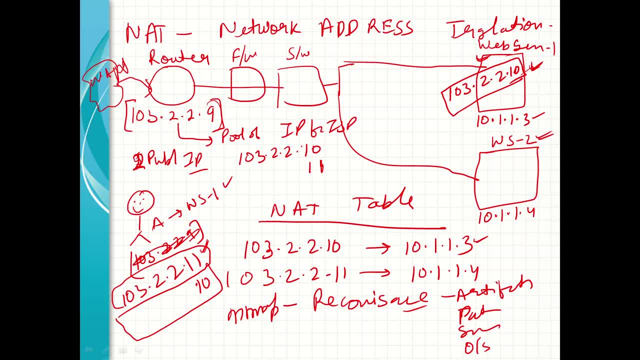 there are three addresses you are provided to, ending with 2.9, 2.10 and 2.11. so when you said to access the land on this main router, he should type this address. yes, so without the main router, he cannot get into this web server one or the server two. okay, okay. okay, now i got. 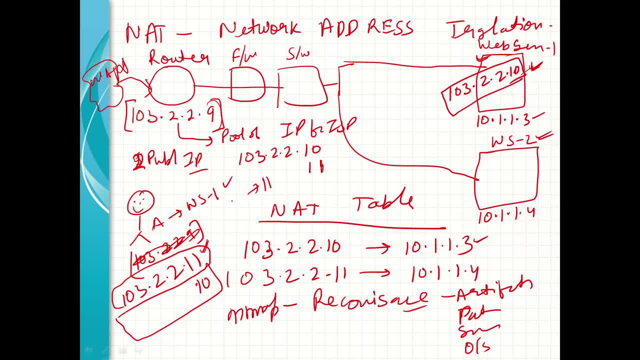 your question. you want to say, yeah, that to access the 11 he need to go to nine first. exactly, yes, so this is happening. actually, this is only happening if he want to access 11, he going to nine first. when you do the tracer, when you find the trace route for this particular, then you will find a. 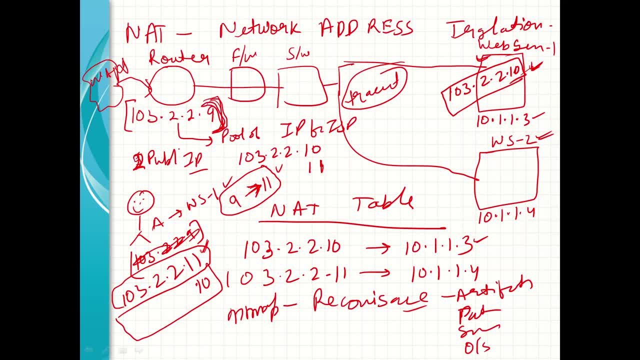 router. this router is all is always there, okay, okay, okay, this outer is always there and the traffic is going to this router only. but when this router traffic go inside the firewall, there is a netting table inside the firewall. okay, and that netting table will decide that this packet is going to be sent to which server. 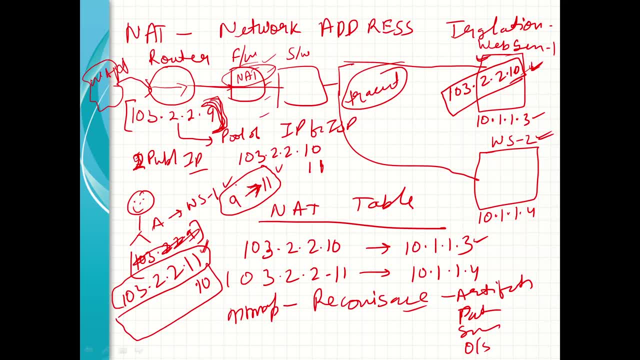 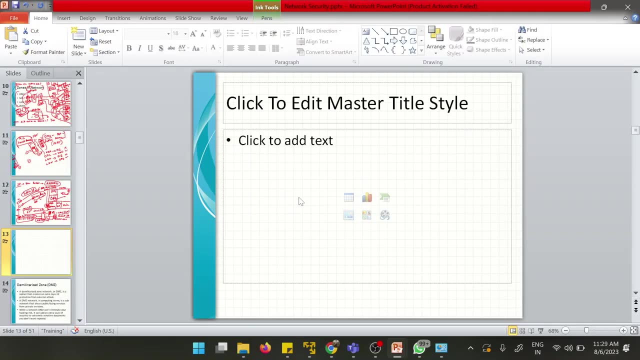 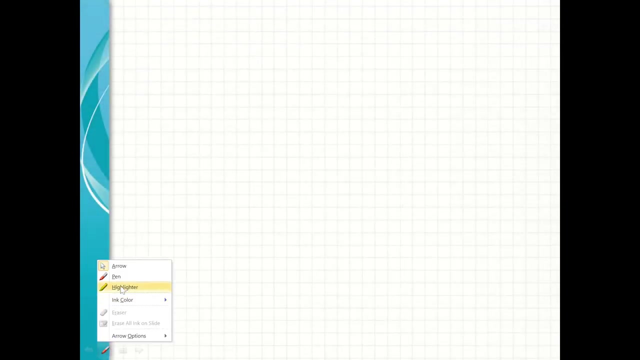 okay, understood. yeah, yeah, sir, please elaborate on this issue. okay, what is the address of this? uh, mr a. okay, let me take one more slide for this. okay, this is mr a, okay, yeah, yeah, and he is having a geo connection. do you broadband connection? okay, let us suppose geo has given him ip 23, 1.1.5. okay, 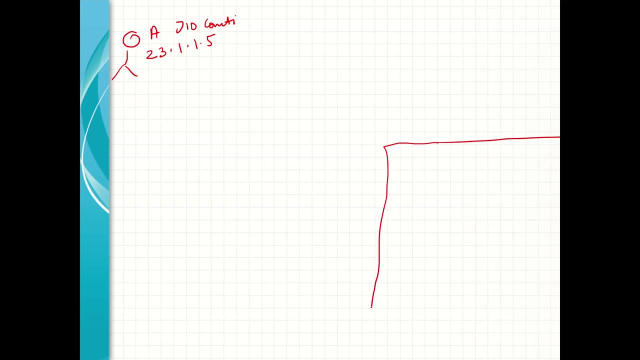 and this is our data center. this is our data center which is having a bsnl connection. okay, this bsnl has provided with a router, okay, okay, and we have configured a ip on fa- 0 by 1. there are two ports, basically 0 by 1 and 0 by 2. on fa, 0 by 1. okay, we have configured 117.23.2.2. okay, this is a lan ip of. 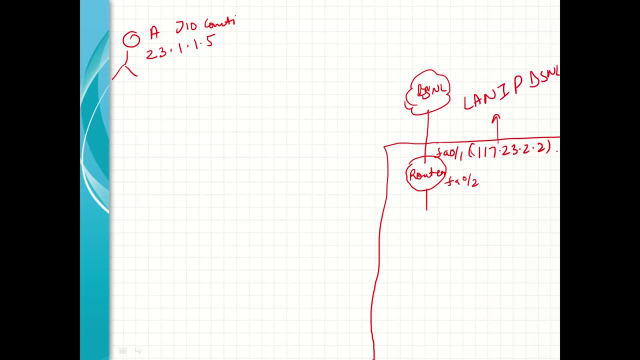 bsnl. okay, we, okay, it is given by bsnl, and on this we have configured 103.2.2.2. okay, so this is our public ip pool. okay, okay, both, both. both these ips are public. no, this is not public. a static root that transfer all fa 0 by one traffic to fa zero by two. okay, now after this. 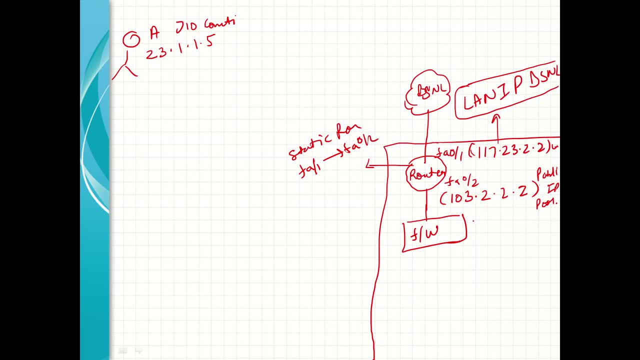 router. we have created a firewall and in this firewall we have write a net rule that for 103.2.2.3 go to this ip, ip1, for 2.4 go to ip2. so when where the firewall is situated after the router, router. okay, yeah. 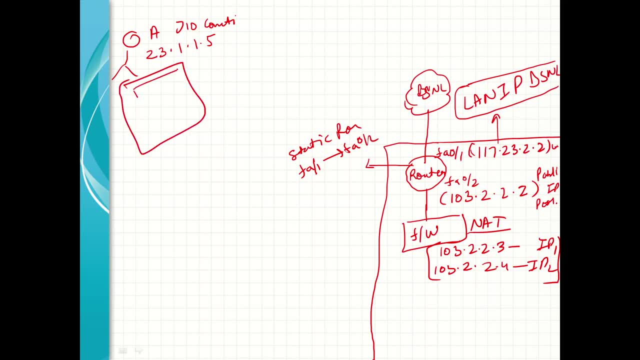 okay. so now when mr a on his browser type 103.2.3. okay, now this request will go to the main router of geo. okay, okay, and geo router will find the shortest virtual distance to this router. okay, search shortest virtual distance. okay, now talk one thing when one router. talk to different routers. 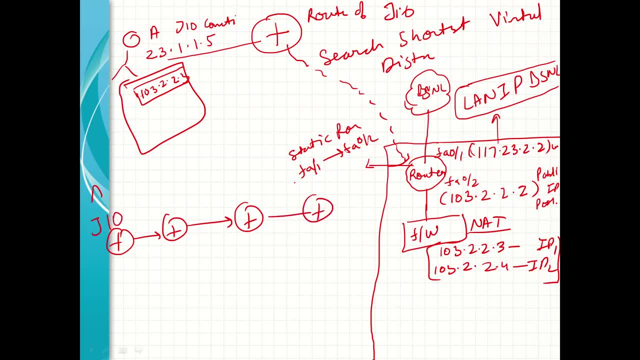 okay, so maybe this is a geo router of mr a and this is the bsnl router of our office. so every router when it is passed, it is called a hop. every router when it is called, it is called a hop. so if i say i have reached from. 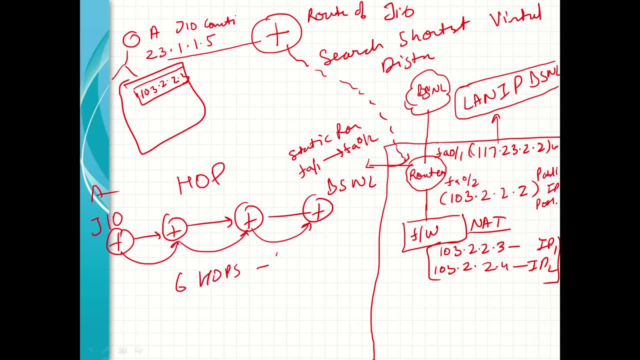 geo to bsnl in six hops. it means six routers came in between. okay, okay, so now when you type this ip address 10222, so it will land to this router, from this router to this firewall, and this firewall will, is having a routing and a netting table. 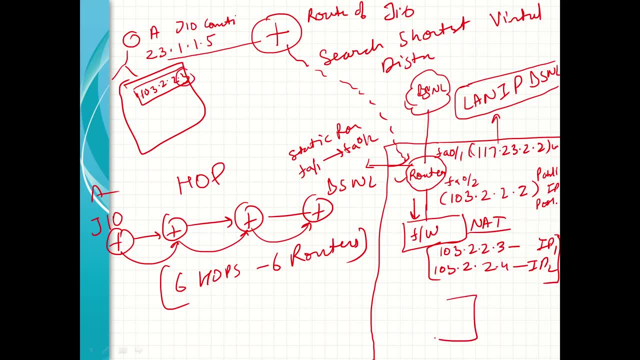 and that 2.3 is corresponding to ip1, which is having that ip1 serving service of web server 1 and the request is transferred to this. okay, understood that how exactly the things are happening, sir. does the role of DNS server come into picture over here? 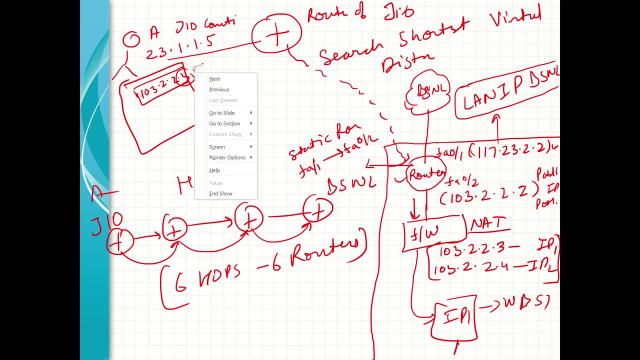 because we are not typing any domain name. here we are typing. we are typing what we are typing. we are typing the IP, IP address, public IP. now just take this scenario as a DNS service. okay, now take this scenario, thank you. what's your name? who asked this question? 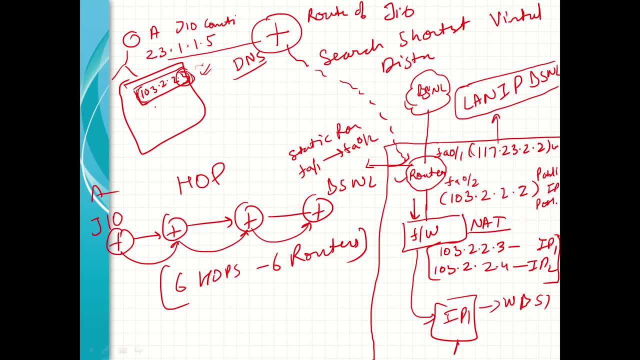 sir, this is Brahma here. Brahma, Kalyan Das hi Brahma. now. let us suppose now user will type wwwabccom. okay, now his computer will ask to DNS server: sir, what is the IP of ABC? now DNS will reply: the IP of ABC is 103.2. 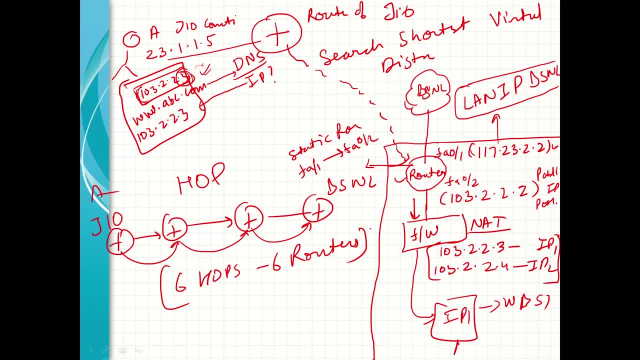 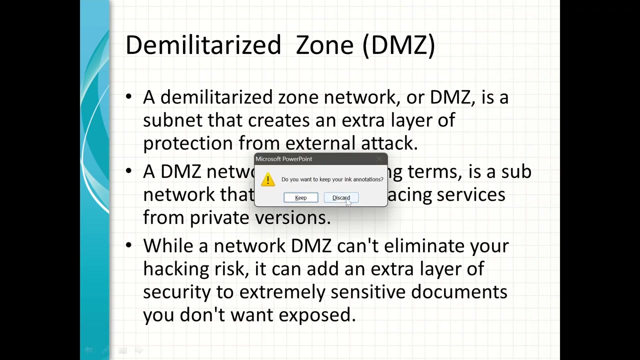 2.2.3. now the same thing will happen. understood now. yes, sir, got it. thank you, got it great. so this issue is clear. about the configuration part: yes, sir, yeah, so let's move it. net is also clear, DNS also clear. okay, so when do we require the airdrop in a particular server? 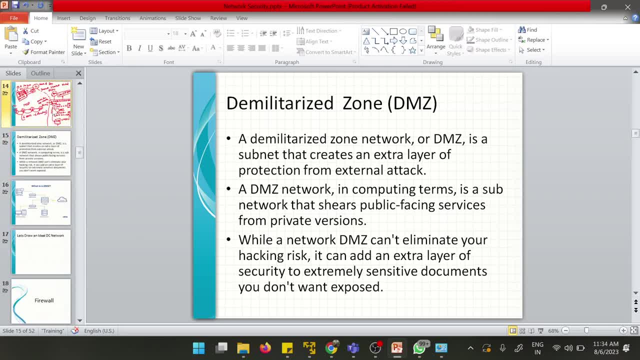 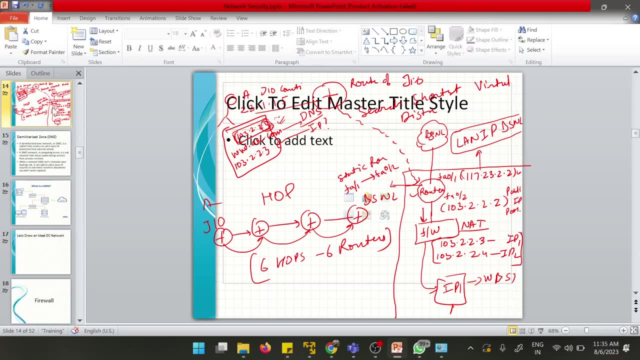 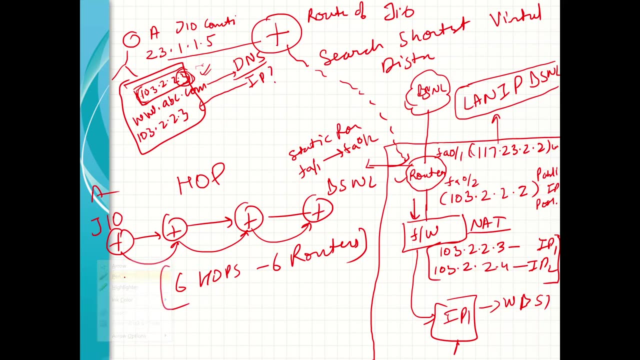 because many times we are using airdrop command in our IPC. which command, sir? sorry, I just airdrop command when we need to airdrop. okay, airdrop, airdrop. now see, I have given this statement here, this statement, this one, this is basically airdrop command. 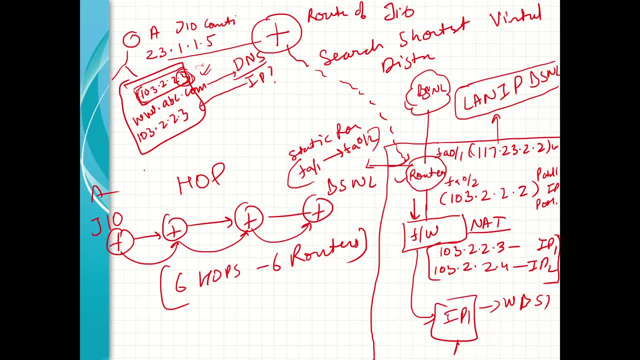 and I have created a new airdrop command. I will write this command. so, for example, I will write in router add, actually not add. it is root IP and F is 0 by 1. is this 117.23.2.2? then it is subnet. 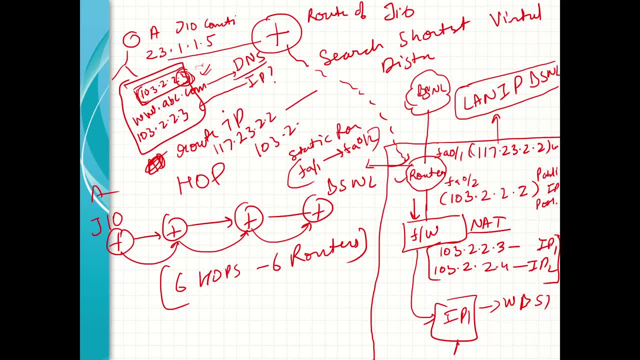 okay, okay, 2103.2.2.2. so this is a root command. static root command. this is a static root command. let me take this out route. okay, there are two type of routing: static routing and dynamic routing. but this is not a part of this session right now, so i'm not going to talk on that. but this is a simple static routing ip. 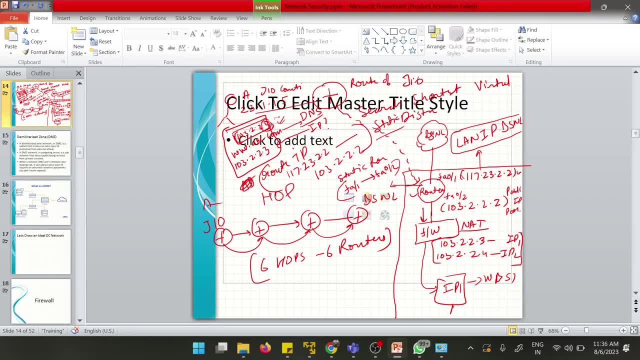 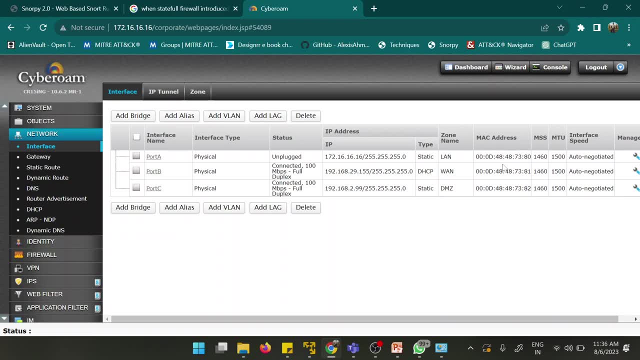 okay, is it clear, sir, who has asked this question? yes, sir, yes, sir. so now come back again to this firewall. uh, you have seen different type of zones, are there? okay, so now let me uh create some rules. so, can we? shall we create rules you want to see, or, uh, shall we skip? no, no, sir, create rules, yeah, yeah. 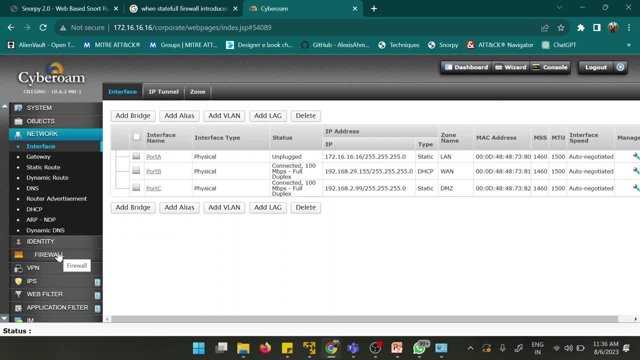 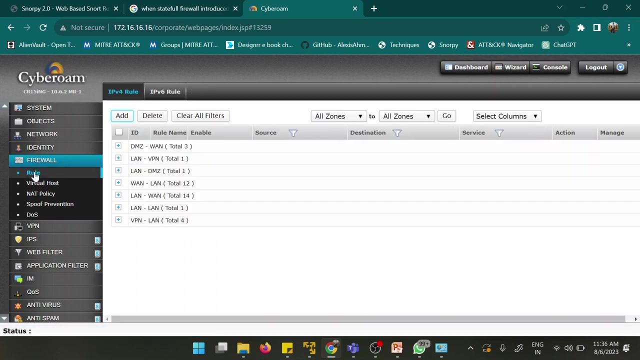 because this is the main: learning- talking theoretically and working on appliances totally different. sir, is this extreme protection or normal? this is a normal firewall. okay, i'll just bring this to make you people aware about rules and zoning, okay. okay, so you can see that there are different type of rules are already there. 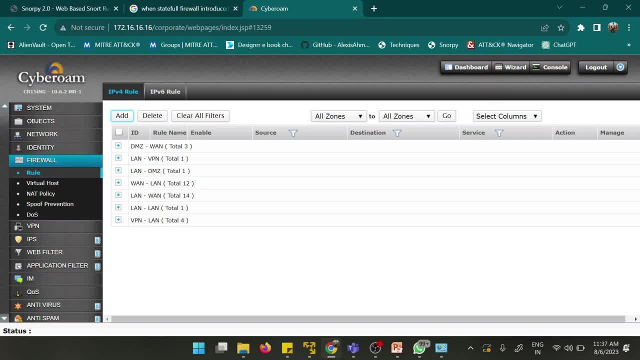 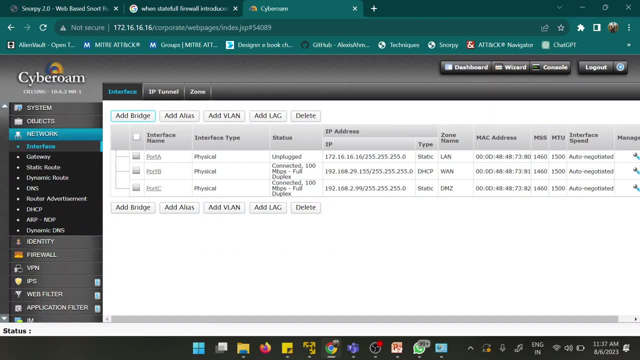 okay. so whenever you want to write a rules, you need to first make yourself very comfortable with the different type of zones, okay? so in this case, my internet is on with zone which zone- okay, and my uh users are on which zone- okay. so i want to create a rule. okay, let me uh type for you. let me type in chat box. 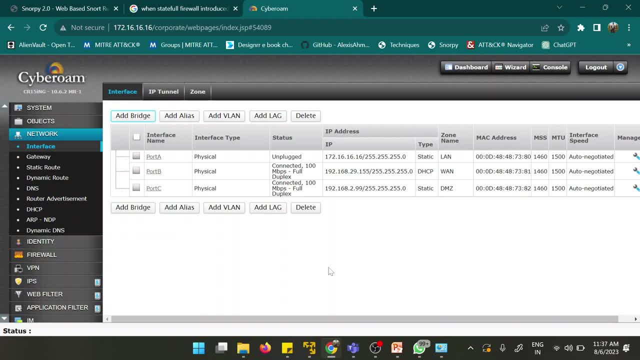 so that you can create a rule that block ip with this. okay, so there is a rule in chat box. create a rule that block ip this from accessing from lan to n. is it visible to everyone? visit my channel as well. there is a box. i will show you how is that. 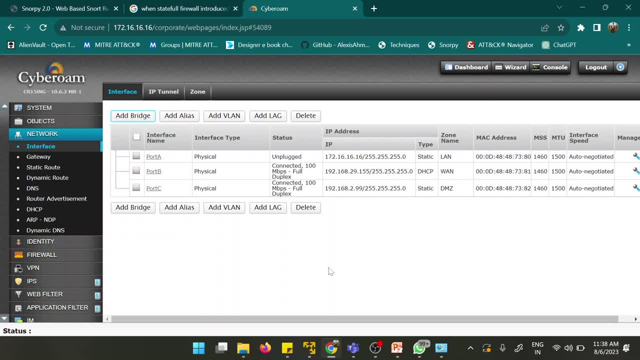 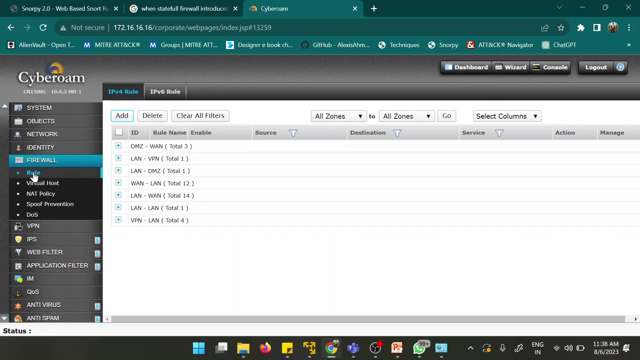 okay that. so there is a晚上 g league. a little bit log that is in ebook so this morning, so we need to everyone, okay, so now I will going to create a rule for this. so in every file all you have a functionality to add a rule. so let us go and add a rule, okay, so. 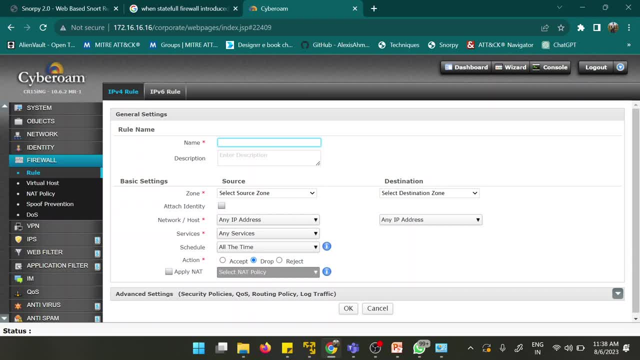 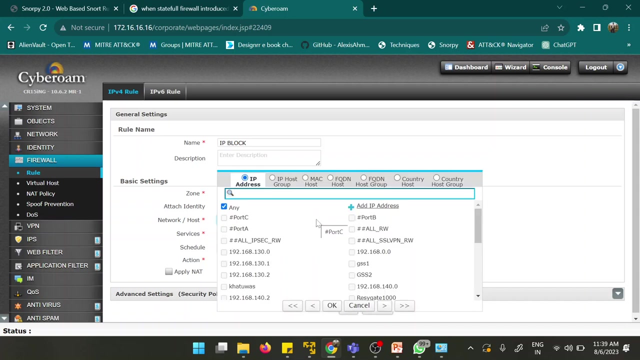 we need to give a name, so you can give a good name for this, like IP block. okay, now I will select a zone. what is the source zone? now I want whole land. I want to block this IP for the whole land. so what will I select? any IP address or a. 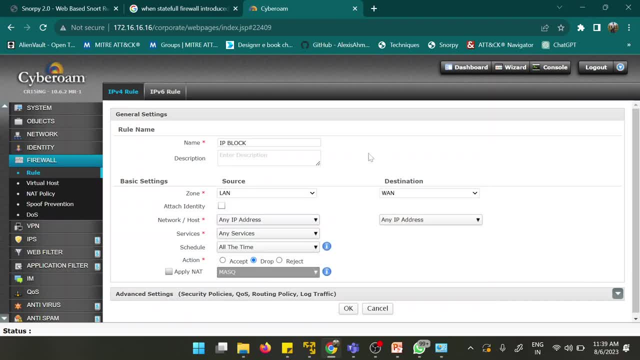 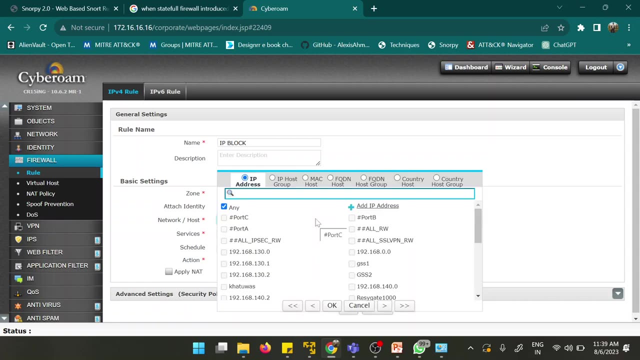 particular IP address, any IP address, whoever in my land is there is go, is this IP is going to block for everyone. okay, is it fine. that's why I am using any IP address, I or if I want to block for a particular IP address, okay, so let us modify the rule. 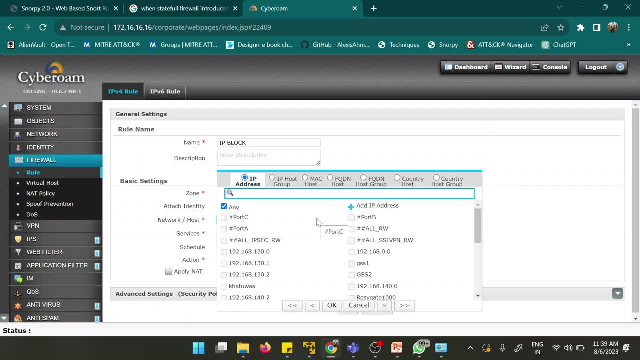 here, but it is still. yes. yeah, now I've right. different rule on chat box. now we will create a rule that will block IP this from LAN IP, this. ok, so now I will going to select a particular LAN IP, that from which the IP traffic is to be blocked. I will add IP now. it will showing you. 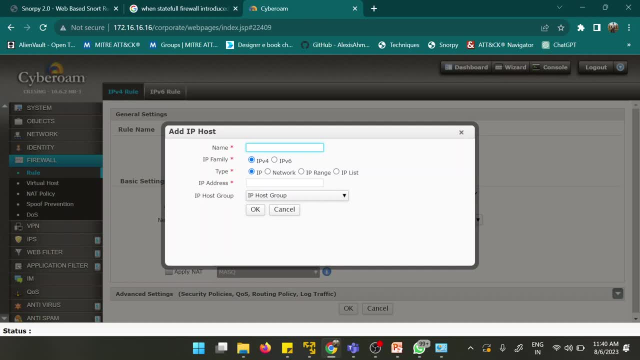 different type of options. okay, now it is showing different type of option: IPv4 and IPv6, which IP pool we are using right now. it is also giving you an option: IP network, IP range and IP list. okay, so if you talk about IP, you can. if there is a single IP, you can put. 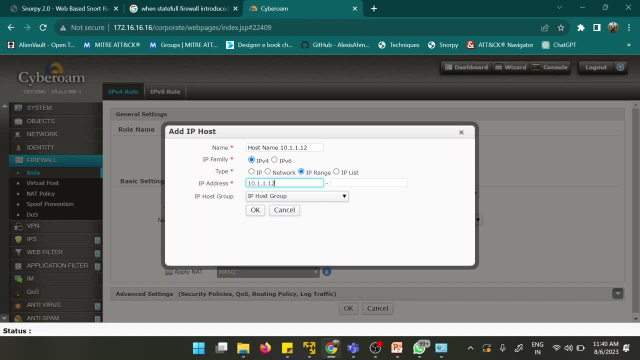 down IP here. if you have a IP range, you can put down a particular IP range here, that from 12 to 25 for all the IPs. this rule will apply. or you can type IP list. okay, you can add multiple IPs. okay, you can add multiple IPs, but I am going to do this for 10.1.1.12, okay, so, 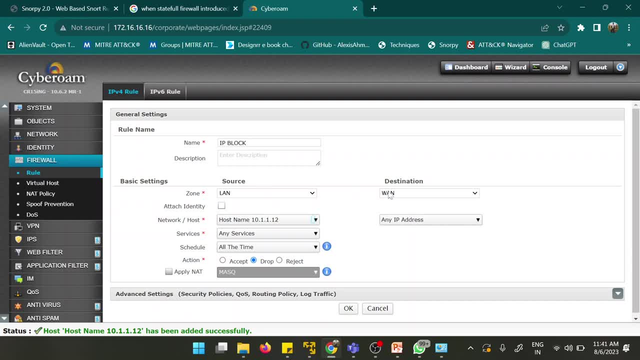 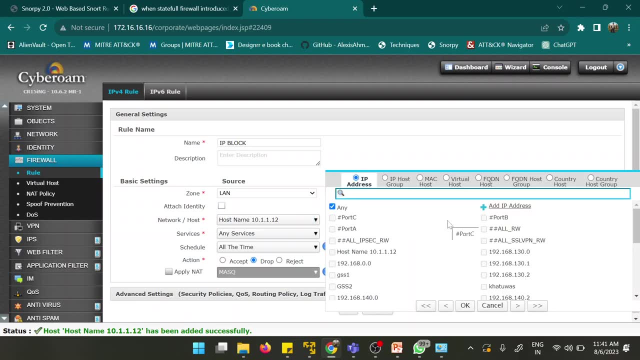 what I am going to do is I am going to block an IP from LAN to WAN zone for host name. this. now I am going to add the IP which need to be blocked. so for blocking the IP, we need to add an IP address. so what is our IP address? which? 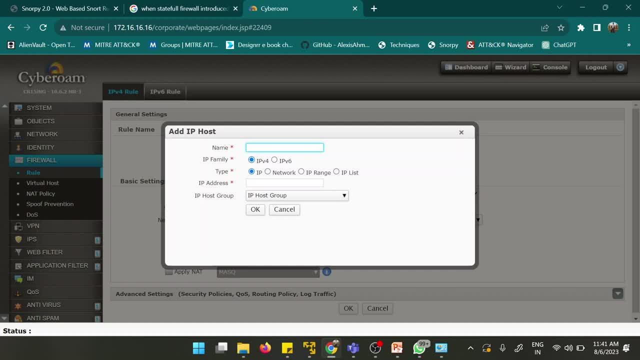 need to be blocked. tell me, just check the question then, fine, fine, 10.1.1.2, no, no, no, 1, 0, 3, 2, 2, 2, because this is a public IP. we need to go okay, okay, so we will block this okay. 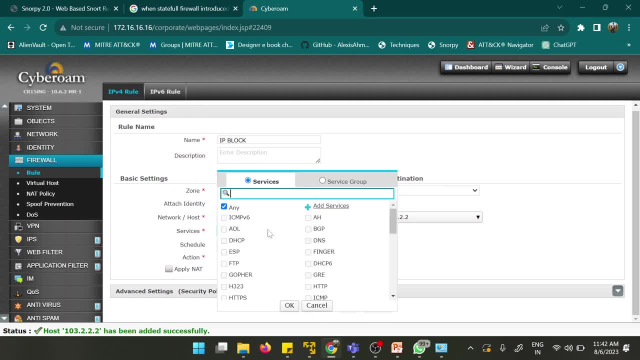 now you are having getting three options: that for services, that for all type of services you want to block, or for any ICMP. you want to block any DSCP. or you want to block in case. you want to block any DSCP you want to block in case you. 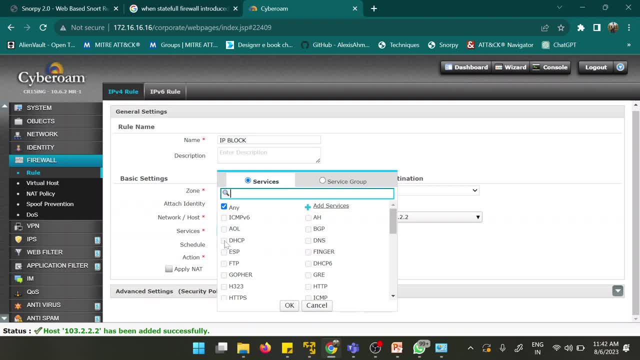 want to just block that nobody can ping you. you can block for the ICMP or if what? if you want that nobody can send you the s that emails, you can block the IMAP and pop through, though I am doing this for any services and also in the firewalls. 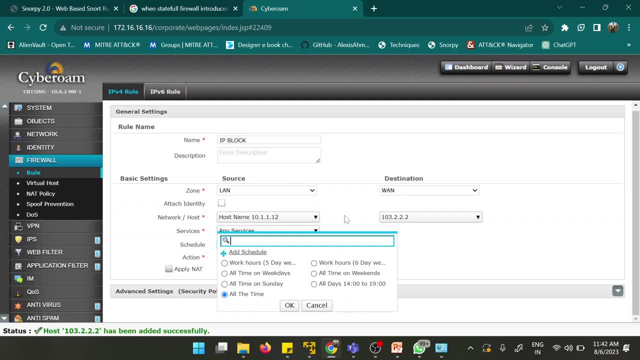 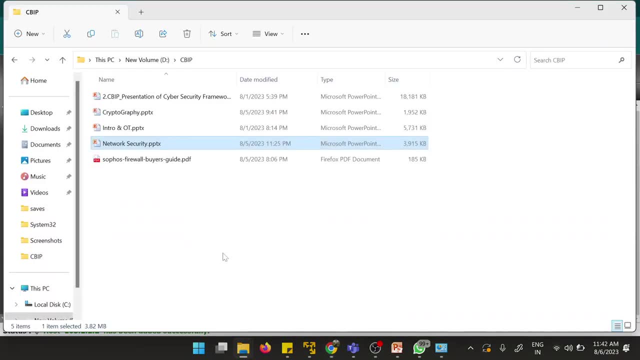 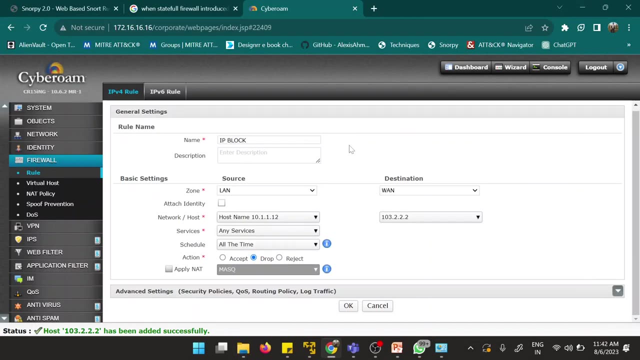 you will getting a time for schedule, like for all the day it is going to be blocked, or for some time it is going to be blocked now. the important thing is that there are three option. accept, it has gone. yeah, now you can see there are three option, are there? what is that? 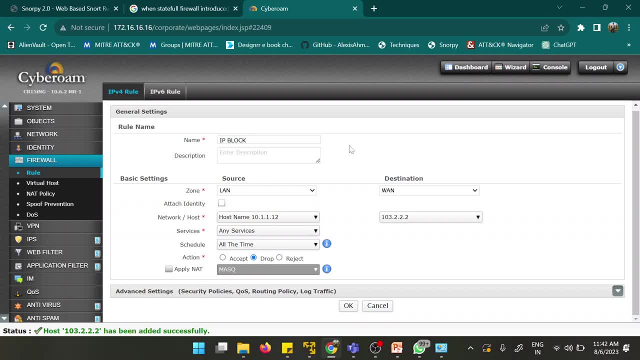 accept, drop and reject. okay, so what is the different between drop and reject rejection? send the message to the sender. yes, yes, yes, perfect, whenever. when you drop that message, it will not create an alert, but when you reject that message, it will create an alert. okay, so I will put a reject so that I can get an idea and 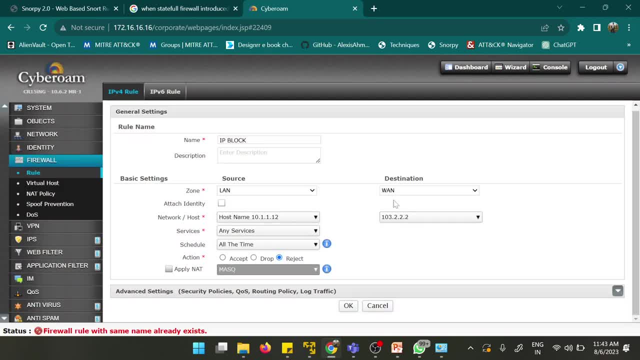 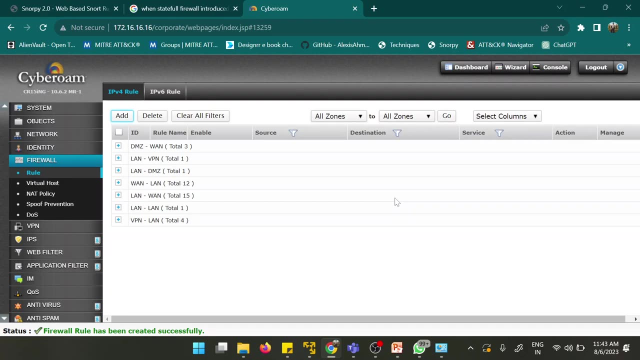 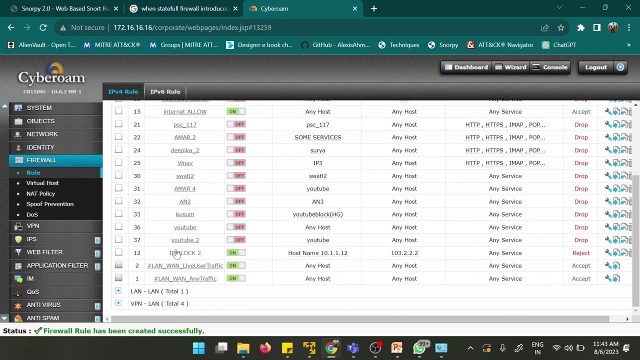 then I will save this one. okay, firewall rules and already name exist. okay, so when, on which zone? we have created the rule which only I've created: plan to end, when to end? when to one land to end, yes, land to end. now you can see there is a rule: IP block 2. 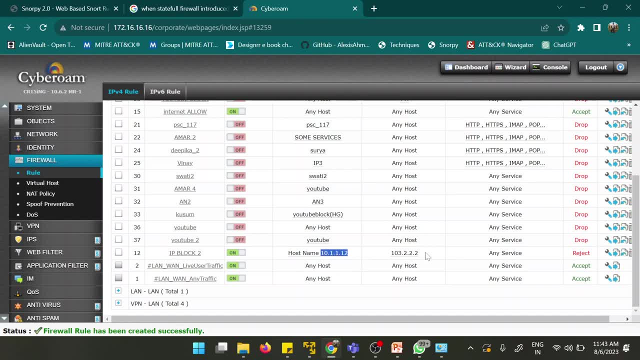 which is creating a block between this IP and this IP. this is a land IP and this is a public IP. now, this LAN IP of your network is not able to talk with this public IP. okay, is it fine? till now, you don't know. yes, but yes, sir. 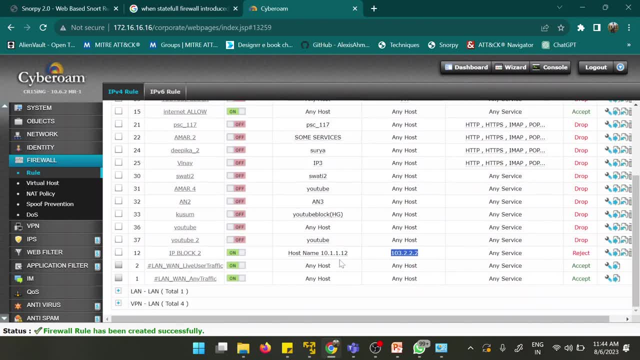 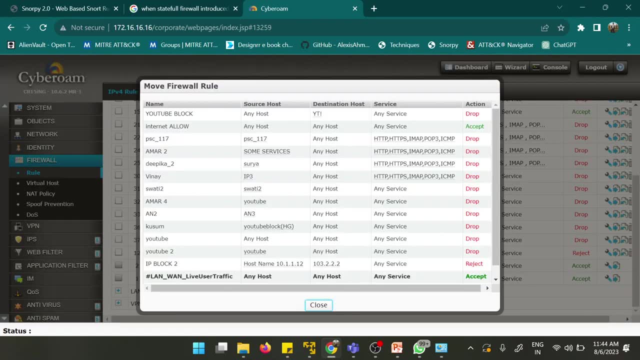 but there is a still a problem, and problem will exist. why? because on rules there is a concept of priority. works okay, the rule, the firewall will first take this rule, then this rule, then this rule. you are able to see move firewall rules. the internet allowed. well, sir, except okay. are you able to see this picture? 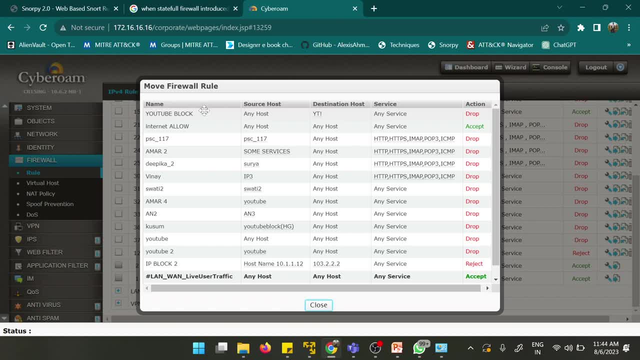 this window move firewall. yes, yes, yes. so actually the thing is, the firewall will take youtube block rule first, our internet allow rule second. so this is a priority. so if you want to block this ip, we need to make it on a top okay. otherwise this internet allow rule allow any host to any host to any. 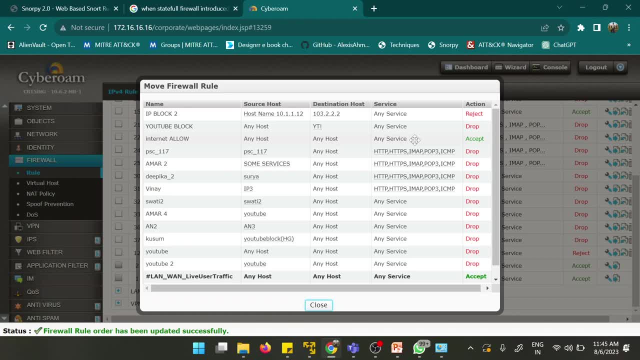 services. okay. so if this rule prevail first, do you think this rule is of any use? no, if, if internet allow rule is there, so ip block 2 rule is of is of no use. yes or no? yes, yes, yes, yes, so we need to prioritize the rule okay. 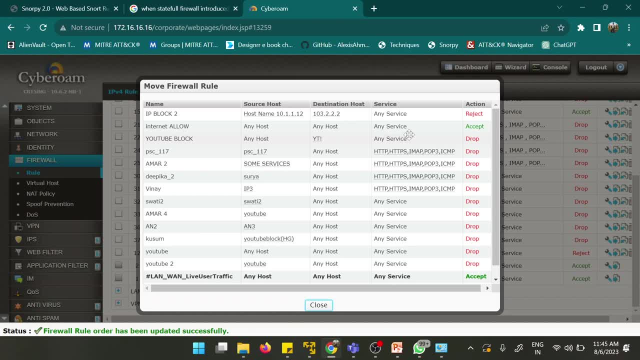 so when we are checking our firewalls, when we are checking our firewalls in a our network, in our offices, in the ot environment, we need to check. that is, if it, if it is any rule which is any to any, any host to any host and with any services. 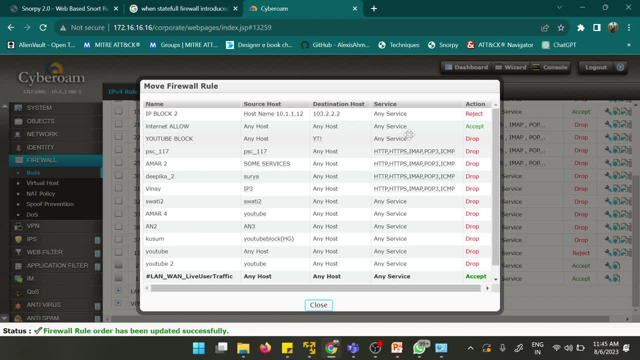 so it is not a good security practice. okay, so configuring a firewall is different, but configuring a firewall with security paradigm is totally different, okay. so in this case you need to prioritize the thing. so the other thing you need to do here is you need to use the 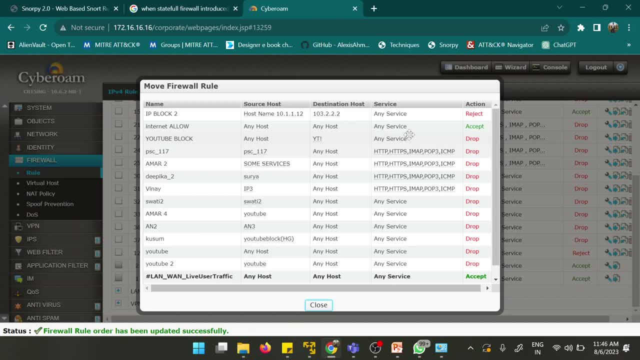 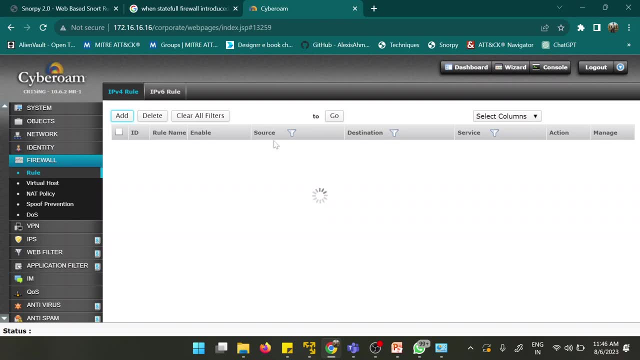 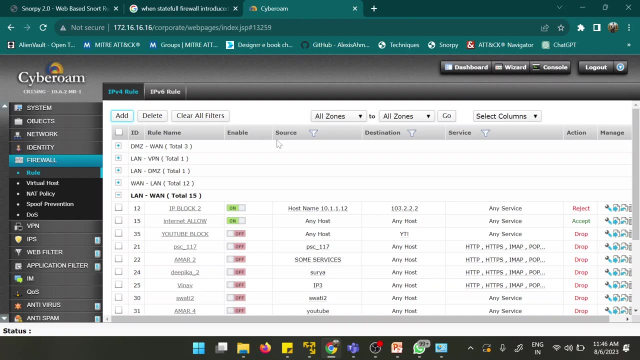 your, your also for top the, your, top ouais first. this is only thing we will so. so so look at this. yes, yes. first rule will be blocked on. no, no. this rule will only apply to this ip na. this rule will only apply to this ip 10: 1, 1. 12. first rule, and the second rule will apply to all ip. 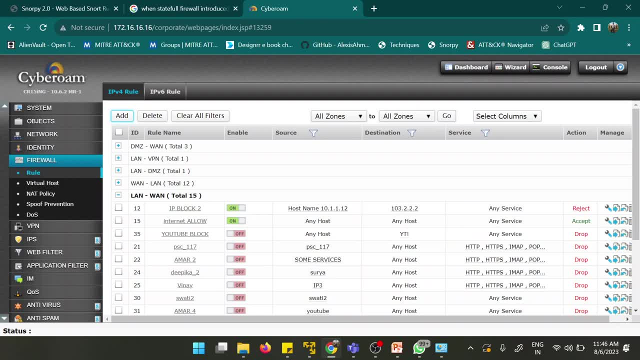 yes, sir, okay, the firewall. is the firewall is going to follow all the rules or only first? sir, it will going to follow all the rules, but on priority, yeah, rule one is subset of rule two. no, because there is no subset. every rule has a separate identity. but which rule you will follow first is on the. it should be on the priority. 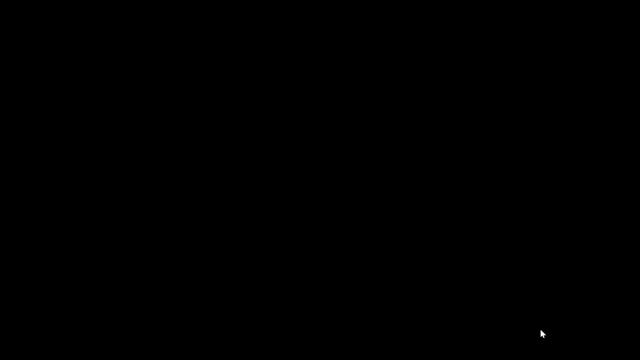 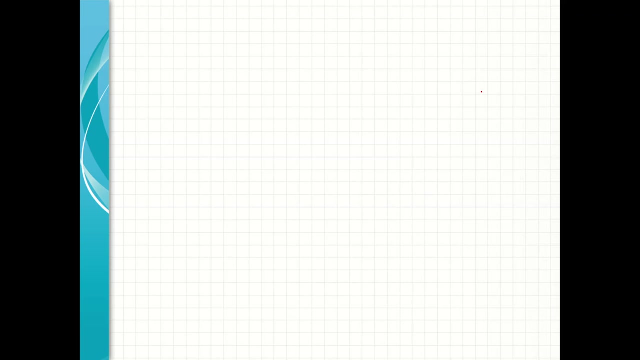 what's the difference? is there any guideline for this? moving this firewall? okay, let me give you a simple example. okay, then you will check. sir, can i also explain what is the difference between reject and drop? i will, i will tell you. okay, i let me write a simple rule for you. rule one is: 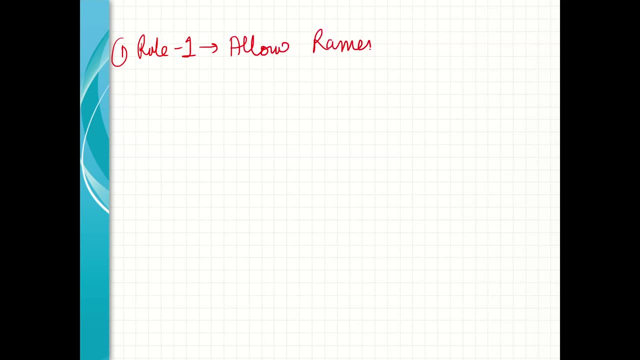 allow ramesh to go okay. rule two is: don't allow ramesh ramesh to go. okay. now, which is of higher priority rule? your first one, first one. so do you think that second rule will work? no, it will not work, because no, it will not already allow ramesh to go. 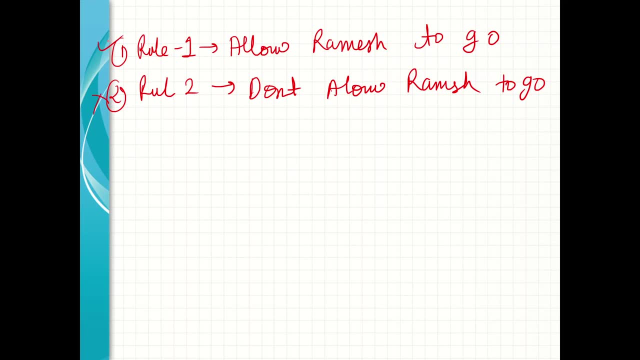 okay, even if that one was like this: don't allow anybody. even also: yeah, yeah, yeah, don't allow anybody. is there still? ramesh will let you go. don't allow anybody. is there still? ramesh will let you go. go because it is having, because it has superseded the rule. okay, understood. 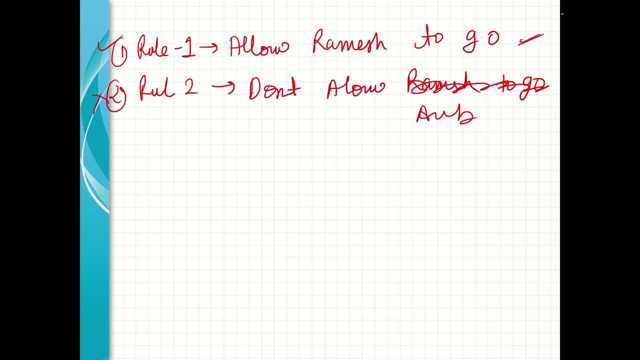 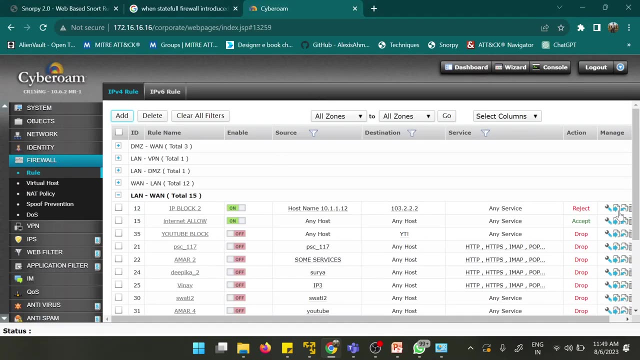 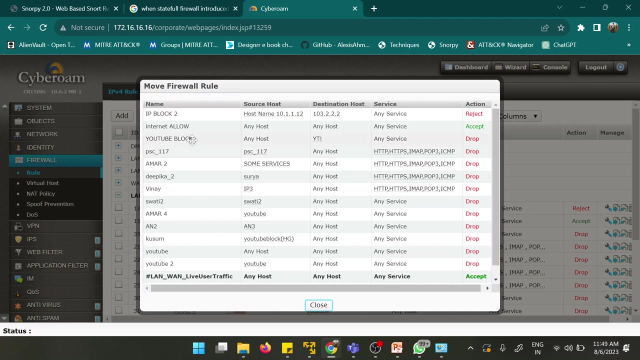 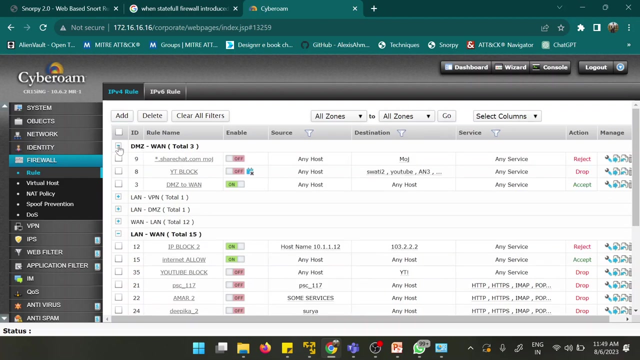 one, two, three are priorities of the rule. right, yeah, one, two, three are priorities of the rule, and you can see in this when i, when i shown with the firewall, there is no priority, number is given, there is no priority. whoever is on top is on priority. okay, like actually now. my children's are watching youtube these days, so i have created a. 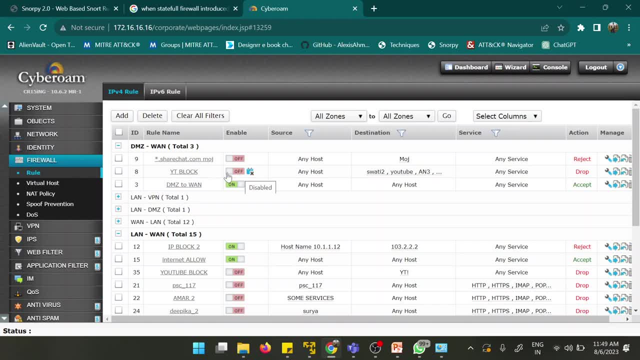 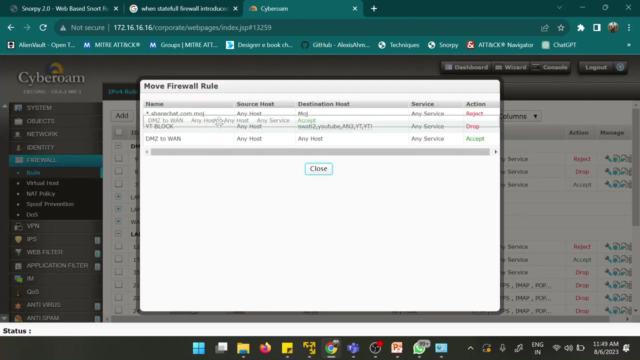 youtube block rule for them. okay, i have created a rule, dmz, to when to access the internet, but on top of that i have created a youtube block rule that youtube should be blocked, because first youtube will be blocked, then the internet will be unlocked, allowed. if i put this rule first, see if i rule this rule first, do you think youtube will be? 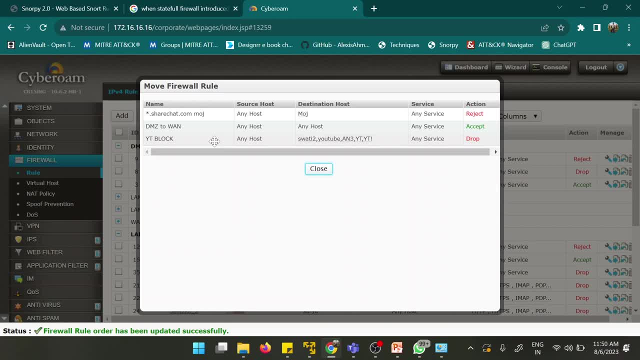 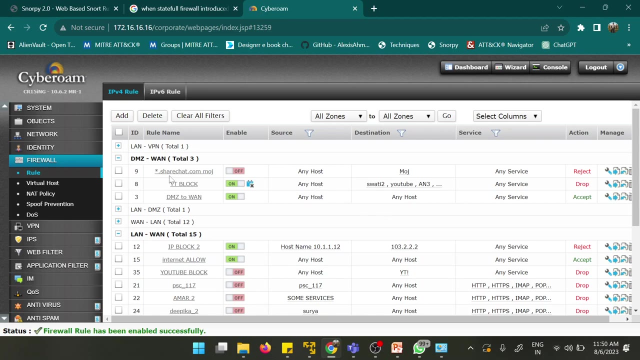 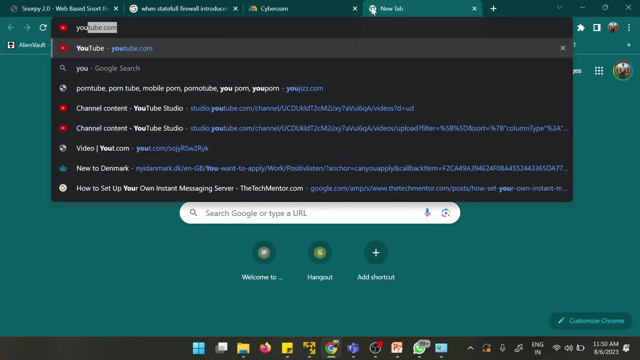 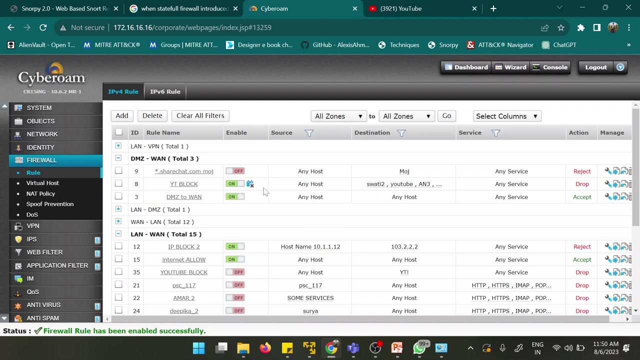 blocked. no, no, no. and now youtube will be blocked or not? yes, yes, yes, sir, can can inside youtube? can we block these reels? yes, sir, this is a share. see, in this i have blocked youtube. okay, let me open youtube. okay, because now youtube block is on, but the time is different. okay, the time is different. that's why. 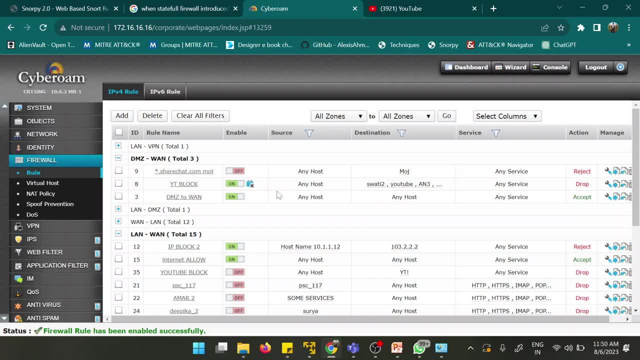 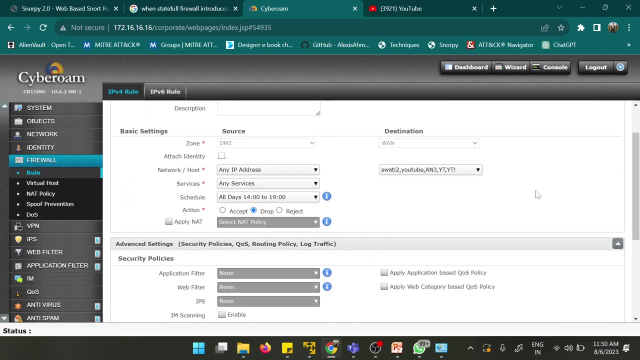 uh, what's your question, sir? such can inside youtube. suppose there are deals you can, you can block. now how you can do this? let us suppose a different creator, a different rule. uh, you want to block something? you can see video steaming, you can do so. these things you can block. you can block an ip address. you can block a ip host group. 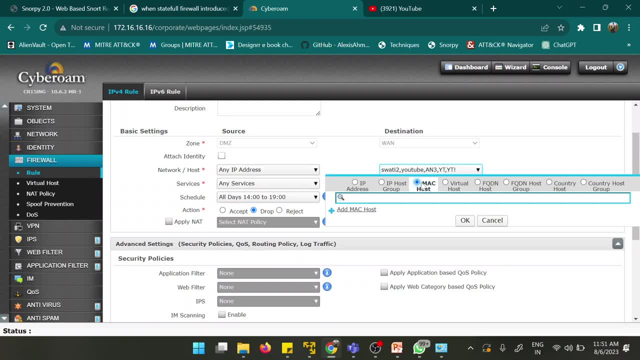 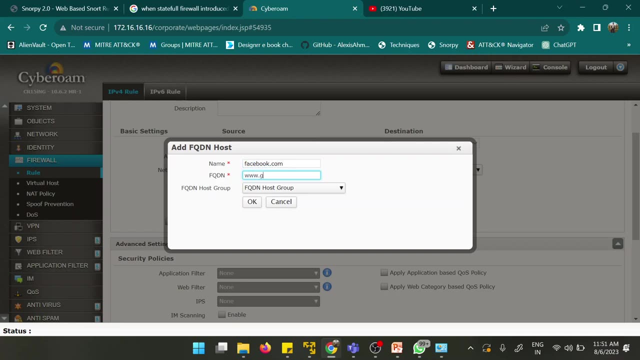 you can block a particular mac host if, if it is a l2 network in your environment, you can host a fqdn. fqdn means fully qualified domain name. you can add a domain name in this, like facebookcom, and write the facebookcom and just block now. 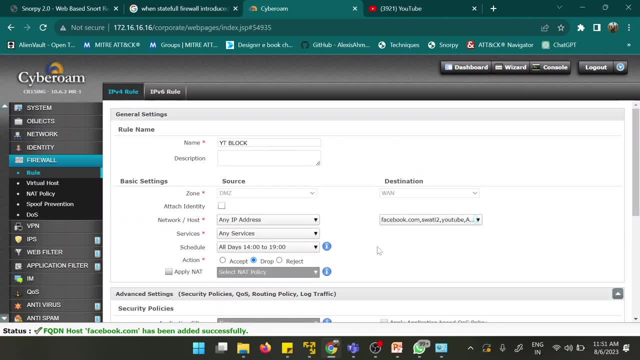 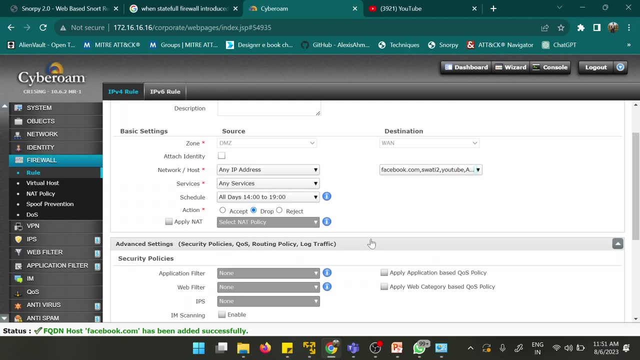 facebook is also blocked in this network. so what i am saying is, sir, youtube is allowed, but in youtube there are the reels. no, no, no, no, no. it cannot be blocked because basically it is running on domain youtubecom. yes, that's what i was asking. so that will require layer 7 firewall content. 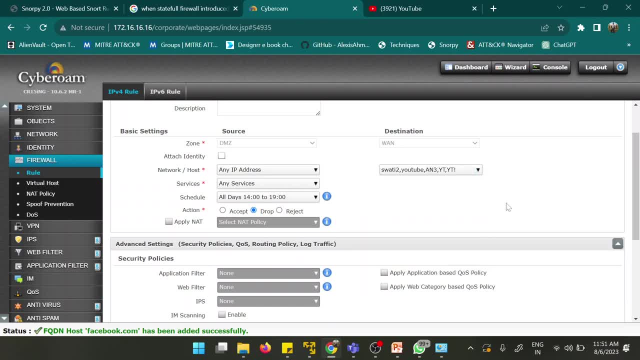 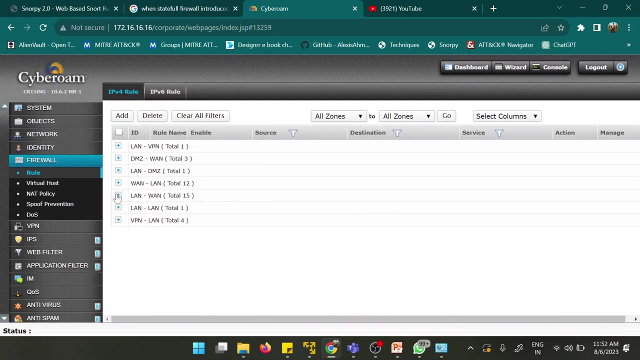 filter. yeah, yeah, yeah that, especially that ngfw next generation firewall. so any questions in this about zoning segmentation, about firewall firewall rule writing and all yes, yes, sorry, beginning with this inbound outbound, how you are segregating it. inbound outbound? yeah, definitely we can see, okay. okay, tell me you are on which network. 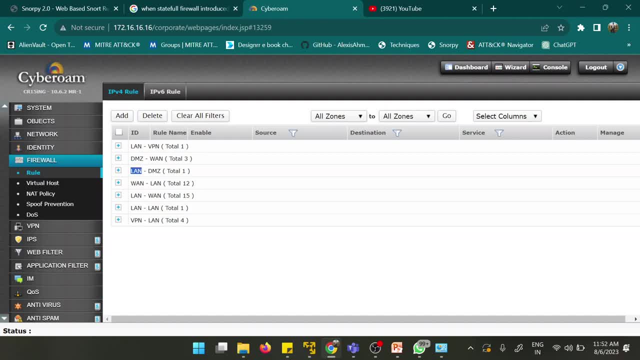 i am in land when this, this user users are in which network, lan, or when. so if i'm creating, if i am creating a rule from land to when this is an inbound or outbound, outbound, outbound, outbound. when i'm creating a rule from when to land, it is inbound or outbound: inbound, inbound. 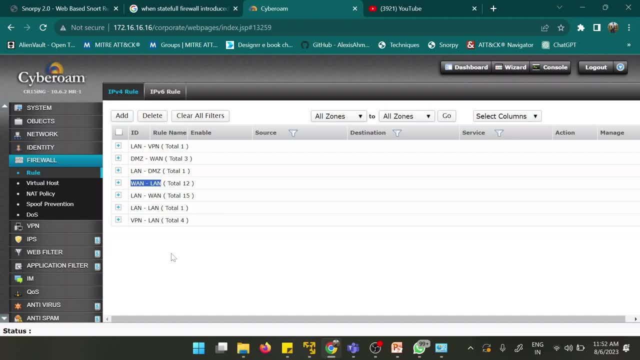 so clear. inbound, outbound rules, yes, yes. whenever we create any, uh, i mean, the first rule should always be: any. any block, right, it is not recommended. any is not recommended because when you write this, it means you are allowing any user to access any resource and any service. no, i'm saying sorry, any. 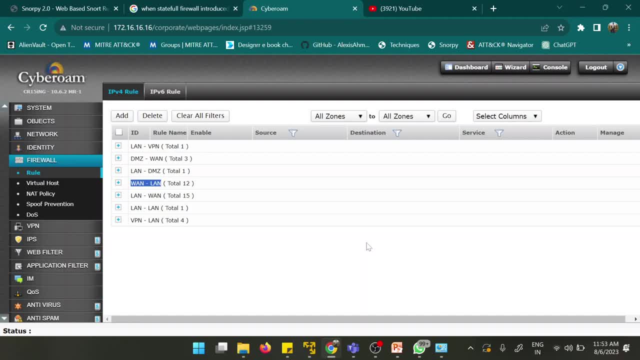 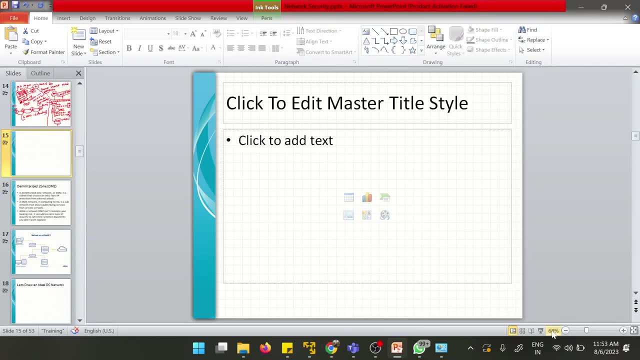 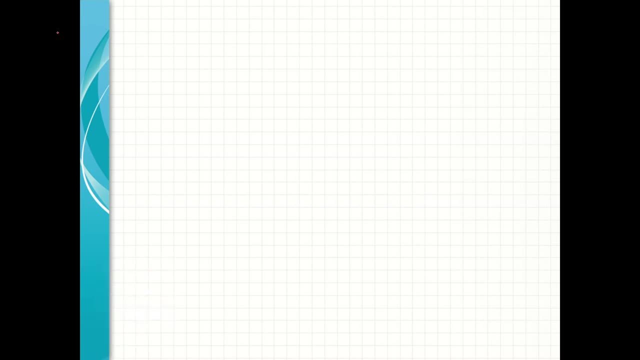 any block, i mean any network to any network- should always be blocked unless the rules gets created. yeah, actually they are two different concepts, that is, a white listing and blacklisting. so let me uh talk something about white listing and blacklisting, because that is a very important thing to discuss. 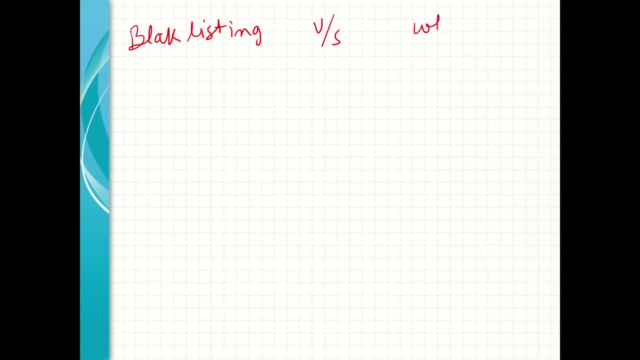 blacklisting versus yeah, yeah, nowadays you are asked to do for the blacklisting what the blacklisting is. this is mr a, okay, and he is doing a duty of a guard. he has a list of five, four people: a, b, c, d. whenever a person come inside he will ask: what is your name? he say my. 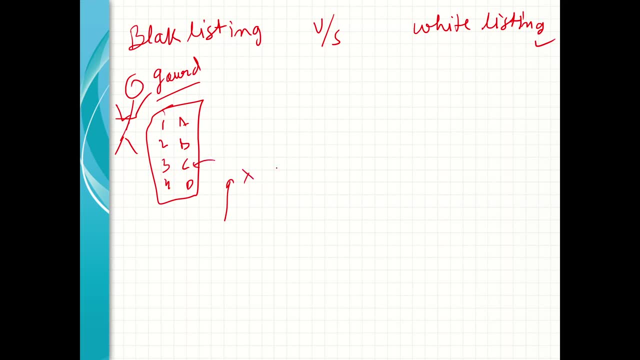 name is c. sir, you are blocked, you cannot go inside. so this is the concept of blacklisting in white listing, the guard will having a same list- a, b, c, d. if a person came and say my name is x, he will check. your name is not blacklisting. this is not a blacklisting for a person, you have to have. 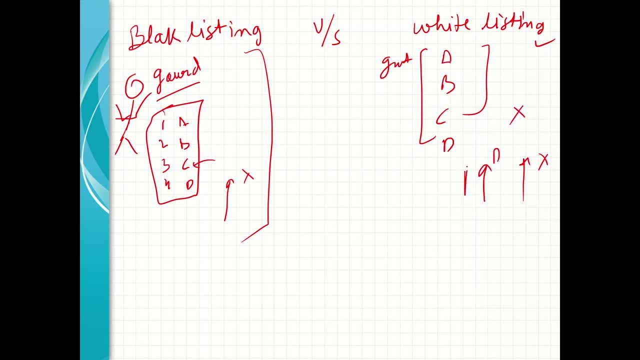 name is not in the list, you cannot go inside. only D will go, C will go, B will go and A will go. so this is the concept of blacklisting and whitelisting. earlier we are adopting this blacklisting concept, but now everyone is talking about whitelisting because this is a most 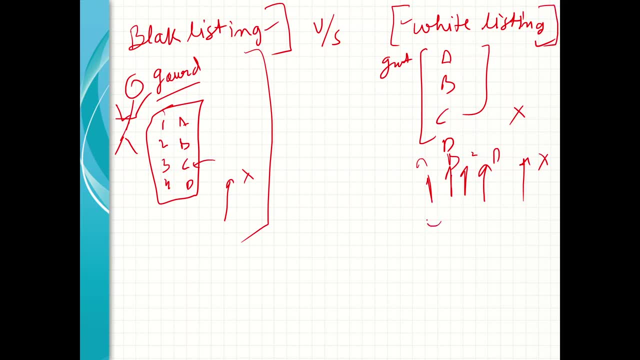 safer concept. but in case of your internet environment, in your LAN environment, this whitelisting concept usually fails because nobody knows that your user is going to access in the corporate network, which website may be he is going to access some income tax return or he need to. 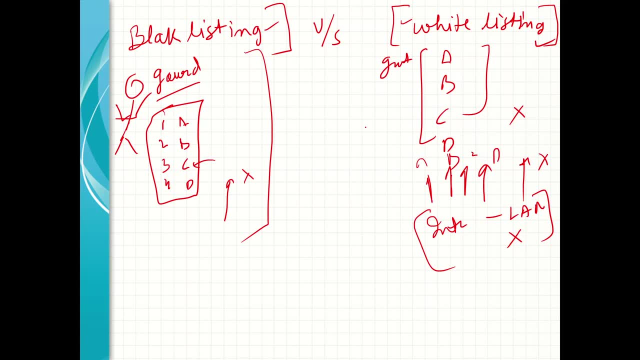 access some geological survey of India website. so usually whitelisting is applied in the OT environment and blacklisting is usually in the IT environment. so this is the basic difference between blacklisting and whitelisting. Sir, I think we know the difference in this A, B, C, D example. 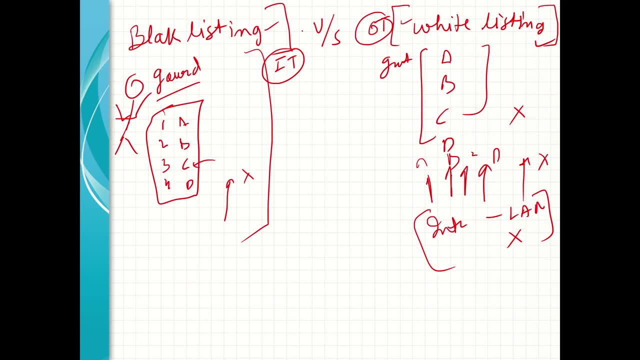 I didn't follow the difference you told, Ma'am, in this blacklisting, these four persons are blocked to go inside a building. okay, and this example, only these four- A, B, C, D- are allowed to go inside the building. Sir, I have one doubt: is there a chance that both rule will be applied? 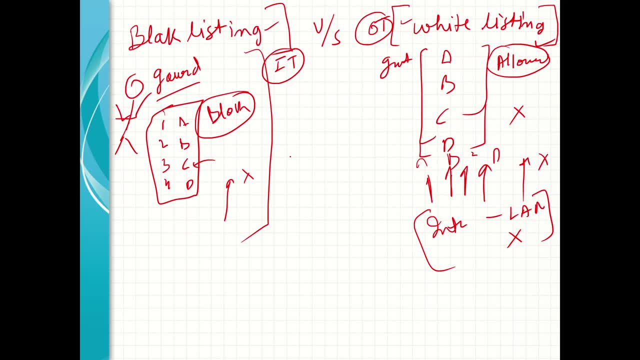 by A, B, C, D or whitelisting. yeah, in this blacklisting too, because- take it there- this is a two-step field where both rules apply on other marre rules. it can be applied either way, by blacklisting or after you, witchlisting and whitelisting, because if children code laws were applied before the blacklisting. 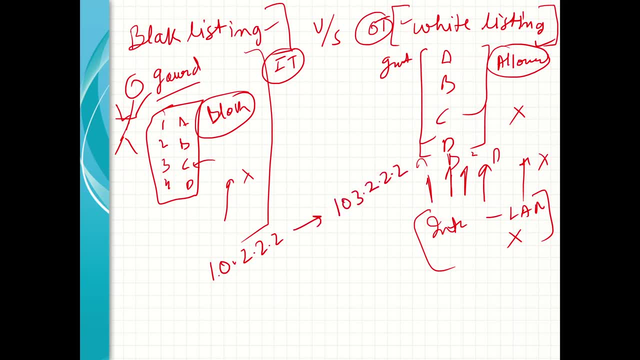 as well as blacklisting, becausel if children code doesn't apply to DH, network, allowed to talk to 103.2.2.2. this is the first rule and second rule is block all. so this is a white listing or a white black listing. the first one is white listing and the second 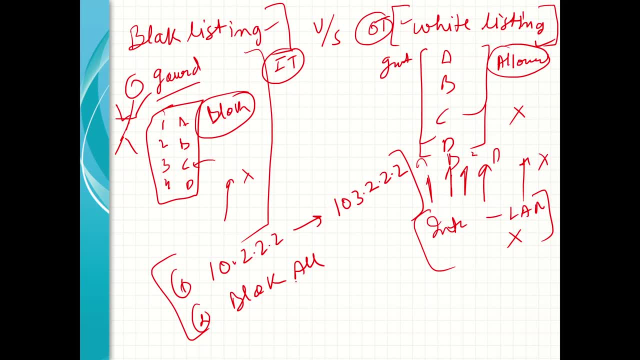 one is actually: this is: this whole is a white white listing, because you are blocking all but only allowing one. yes, yes, yes, this is a white listing concern. so, as you actually this concept will be implemented, how you are writing the rules in your network. that is more important. 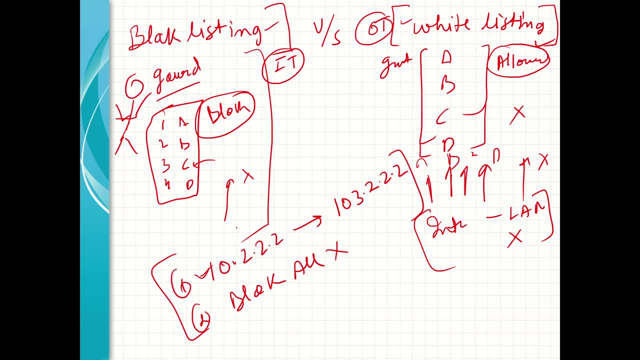 my question is like. my question is like whether both rule will be applied, like black testing and white listings for different networks. you can write not an issue, but for a single network you have to opt for a single. it is: either it is a white or a black. 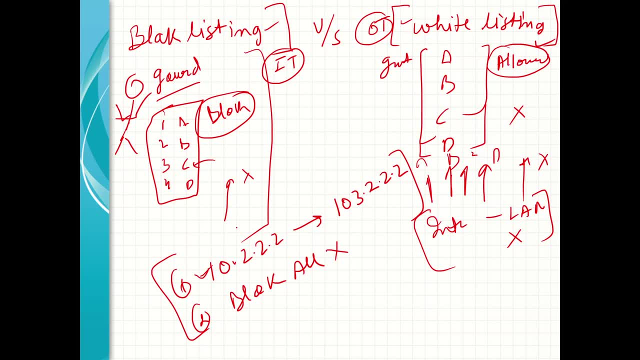 and not the second one, then, by default, what will happen to the rest of the traffic will work like 2.2.2. this first rule will work. and what about the rest? will it allow or not allow? defaultly, everything is blocked in firewall until unless you allow it. 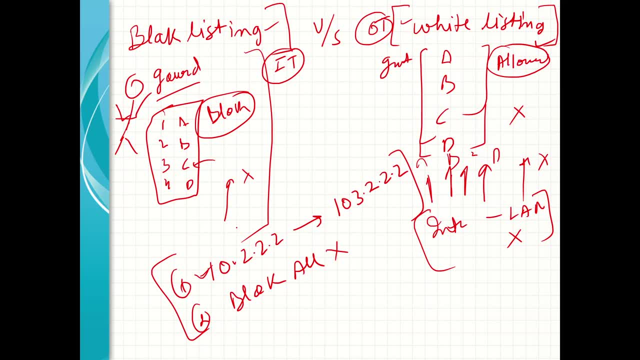 okay. yes, I have a question, sir. sir, we have a Wi-Fi from BSN ILI line and we have, suppose 2300, exe 2300. nowadays it is saying that your internet connection is not secure, sir. what can be the reason for that? previously it was not saying that. maybe some changes in firewall it is. 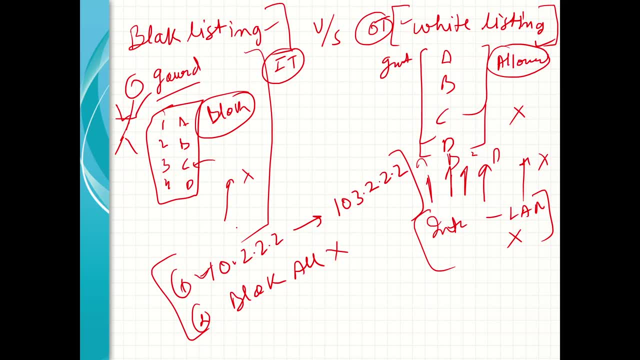 saying that your internet connection is not secure when we are connecting to ICICI. sir, we need to check it out, sir, we need to check it out remotely, sir, we need to check it out remotely by checking the firewall. actually, we cannot tell you. it is due to. 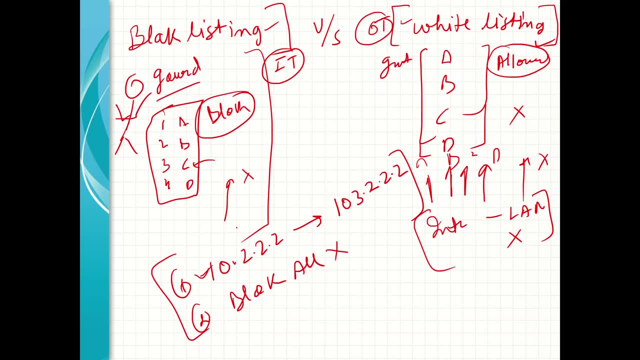 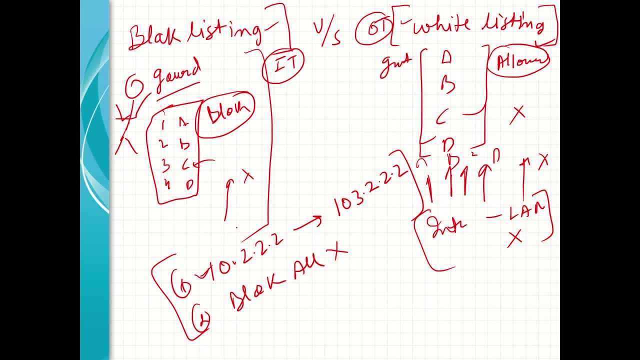 it can be the issue. question, sir: the date and timing of the firewall and drop esto is an issue, Jerry, such is the problem ago. this is the right thing to do. dropped, it is dropping not exactly, and paper, but law select when he is also arting. allowed same, honourable. 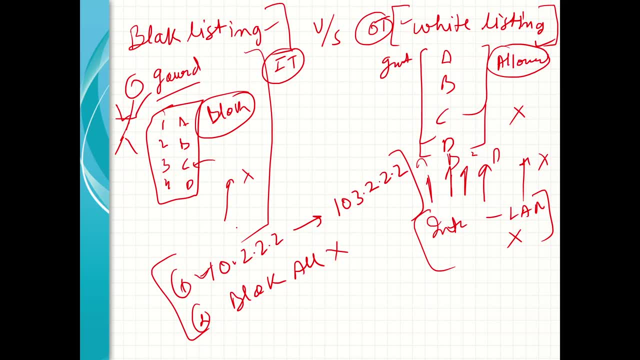 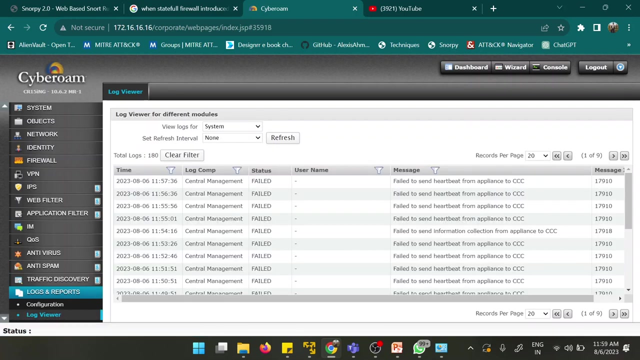 but in drop it is not creating an alert. sorry, in this example we are in packet filter- yes, you say dollar, dollar- where it will create a system alert system. that filter alert because you, what we are using, you are web filtering it, so it will create alert in this. this is: 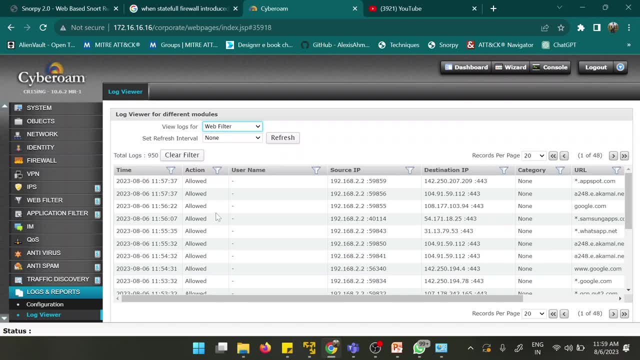 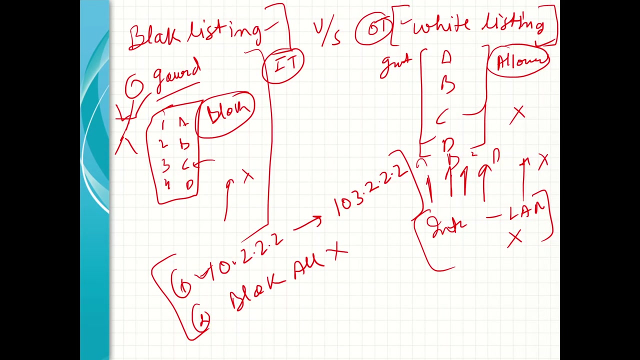 allowed now. so it will clear- to create a loud alert blocked. so I have not created any rule, but it is. it will be sold here. okay, this is a physical firewall. cyber home is a physical firewall. this is a physical fire alive I have in my house because in 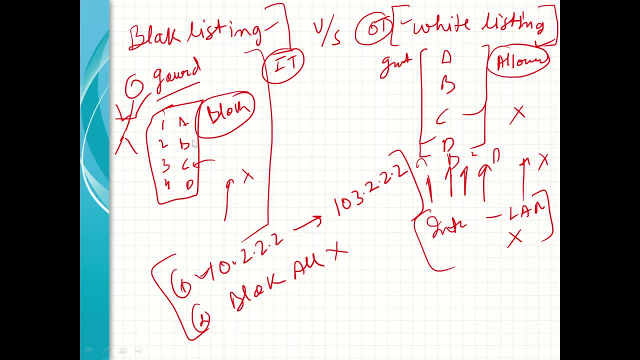 blacklisting, it is only block number of ips. and number of ips are increasing day by day. okay, now let us give- let me give you a scenario that on day one, okay, you have 100 ips to Block, okay, and on day 10, you got an advisory. 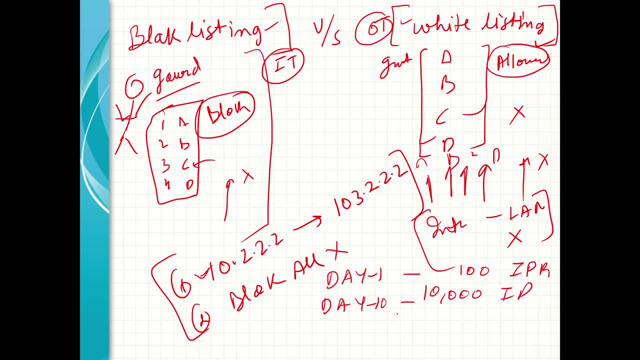 from seasoned that these are the 10 000 ip you need to block. on day 30, some 30 000 more ips came. Now, how many IPs are there after day 31? 40,001 IP, Okay, something like this. 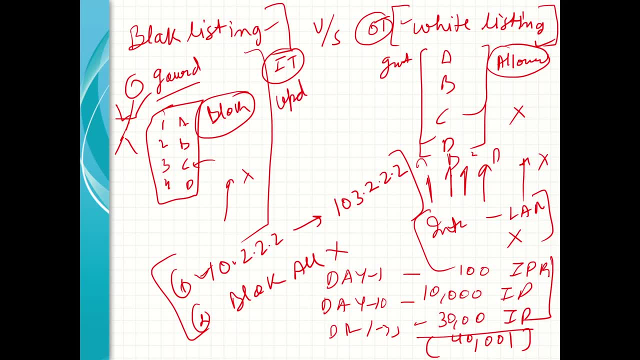 So every time you need to update your firewall, Update your firewall. Also, it will increase the latency in the firewall Because for every incoming connection, your firewall is going to check the list. Is it in the list? Is it in the list? 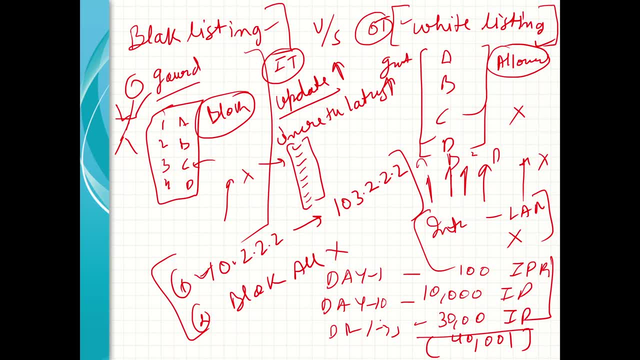 Is it in the list. So every time it is checking the list, Because this list is going to be increased day by day. Okay, sir, Exactly okay, I understand, But there is any limitation of this address in firewall? Sir, actually there is no limit of this address in the firewall. 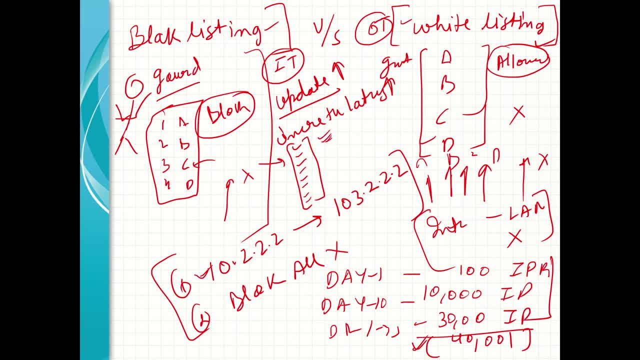 But you can see, if this is continuously increasing, then definitely your latency will increase. Actually, your firewall will be getting slower and slower. Yes, sir, So do you. So the latency increases And definitely the CPU heat will increase. 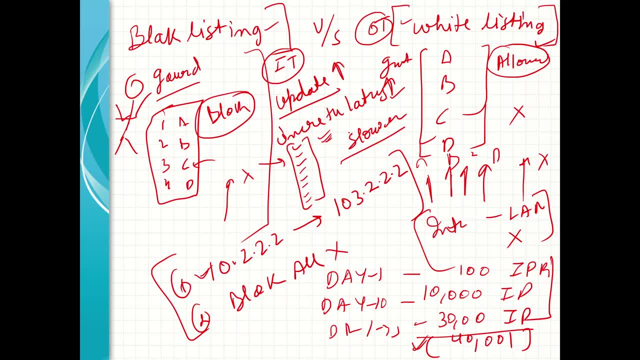 Lot of the things are there, So memory will get exhausted. Swarupji Sir, yeah, I wanted to ask that the only IP communication that we have allowed is 10.2.2.2.103.22.. What if, sir, already 10.2.2.2 already has a malware or something? 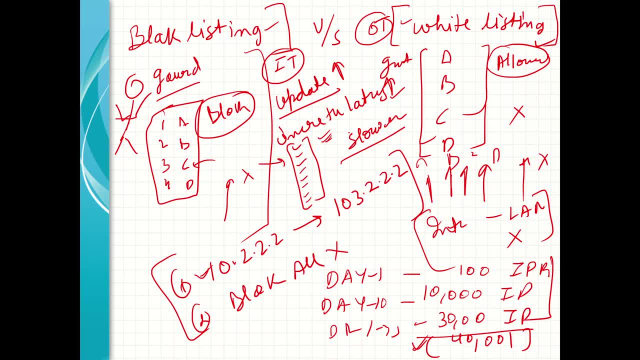 Won't it transmit to the 10.2.2.2? already has a malware or something. Won't it transmit to the 10.2.2.2? already has a malware or something? Won't it transmit to the other side? 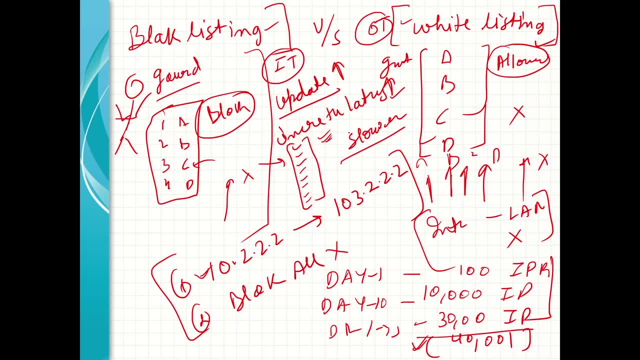 I've not got your question. Can you tell again, Sir? do we have put a firewall allowing only one communication and rest? all have been blocked. One rule has been put in the example. What if the communication that we have allowed already has a malware? 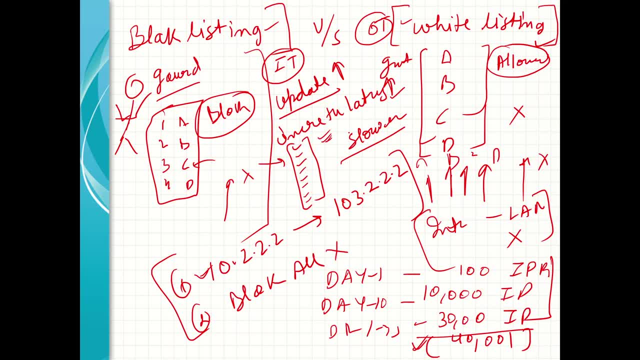 It will transfer One time. So, sir, in that way, When the last example, when you showed that uh van is connected to dmz and dmz is communicating with the database side as a mz, so if the malware is on the internet side it may go to application. 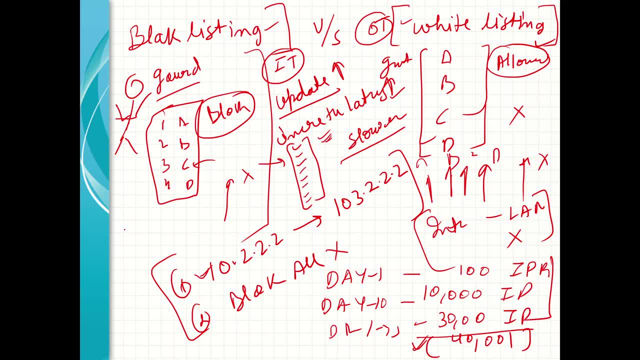 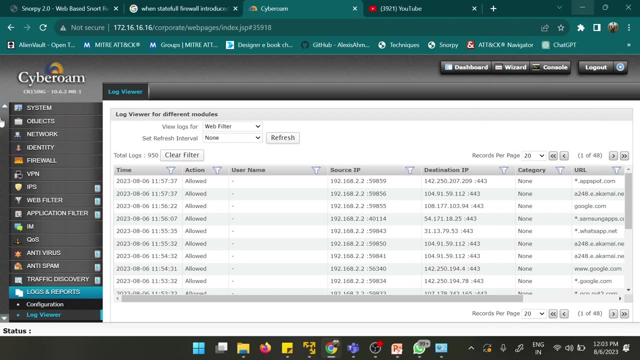 side and from application side it may again go to. definitely. i got a question. that's why the concept of ips and ids came and inbuilt ips and ids are nowadays are a part of firewall. you can see that if i see in my firewall there is an inbuilt ips, is there? 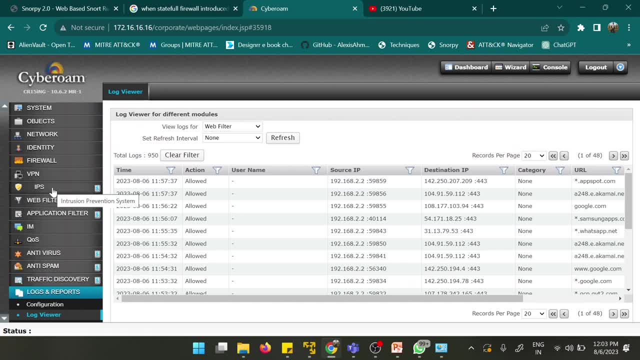 see ips? yes, and there is a firewall. is also there? antivirus? is there? anti-spam is there? okay, sir, but uh, most of the time those malware keep updating. but firewall is generally not connected to the internet, so how does it recognize whether it has to interrupt this or? 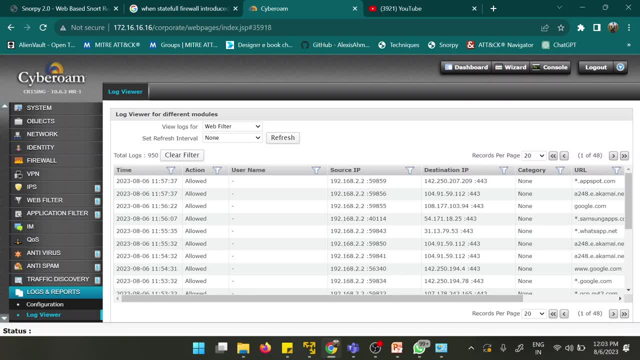 you not. a particular firewall is not connected to internet, so it is recommended to download the patches for the firewall and update it on the offline mode. it is recommended, but okay. okay because you need to update the firewall, because if you are not updating the signatures, then the anti-spam and anti-malware features are of no are of no use. 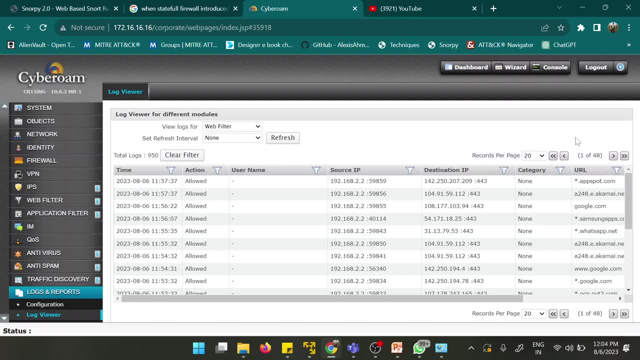 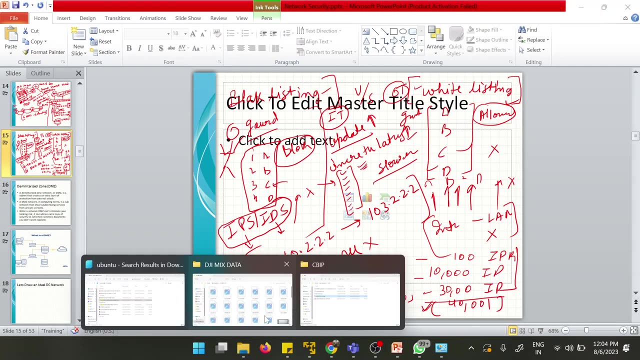 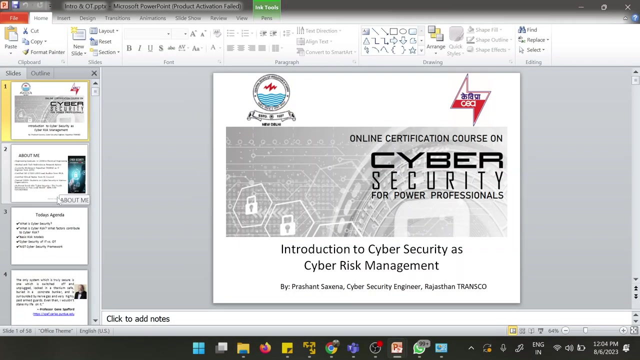 so after using all these uh protections, uh of dmz and mz, uh, a skilled hacker may uh somehow get through all the indirectly it may come to the critical assets. so how do we go about that? if you could elaborate on that, just see this slide, you will get an answer. 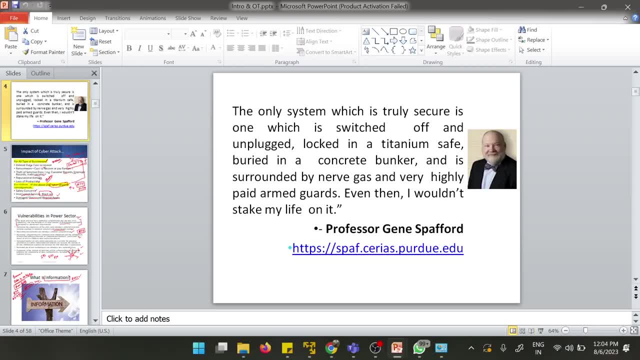 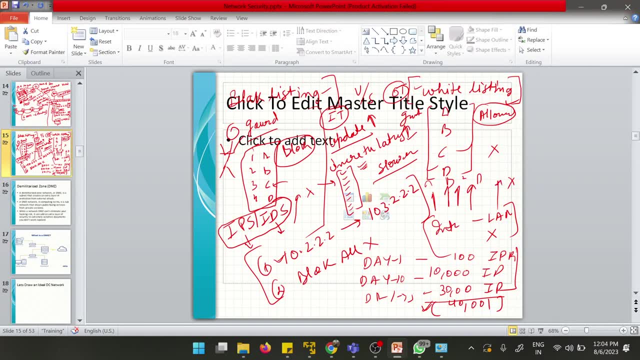 this is a fact. you are talking up on a very perfect uh thing. that's why security is not something that we rely on firewall. to be very frank, security is something you have to take care of. your end host, all of the host, all of the workstation in your network are to be scanned. 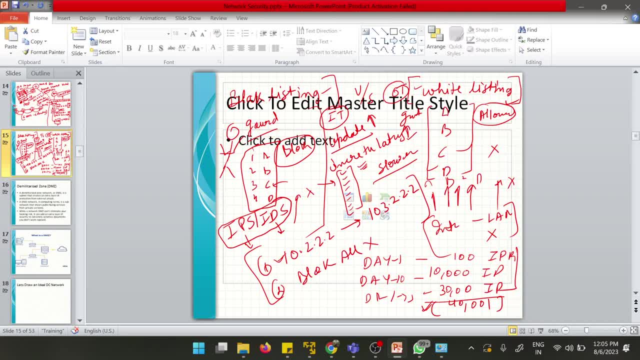 properly and their network traffic is logged and monitored on a regular interval so that, in case it is not, you have to go through the code and verify that your network is not being detected and you can put down. some n-bed devices are there. i'm talking, i'm going to talk. 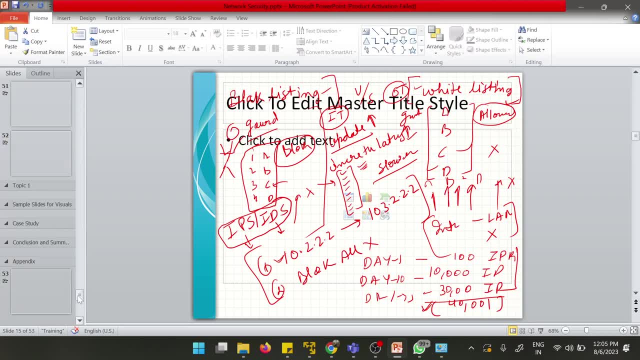 future on this, uh, in these coming slides, because now only 15 slides are completed and i have 52 slides because someone from inside might have knowledge of all the ideas, all these questions. definitely you have a valid questions and i would say, uh, you will get all your answers in this, in this program. 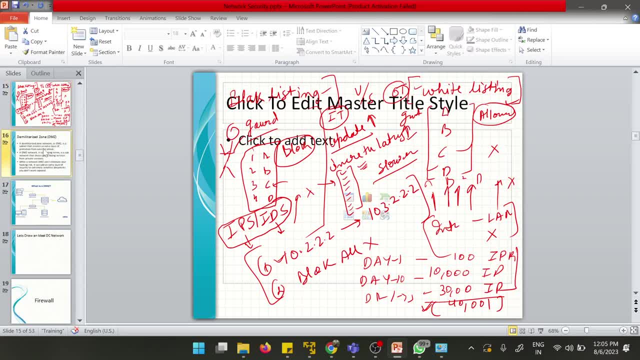 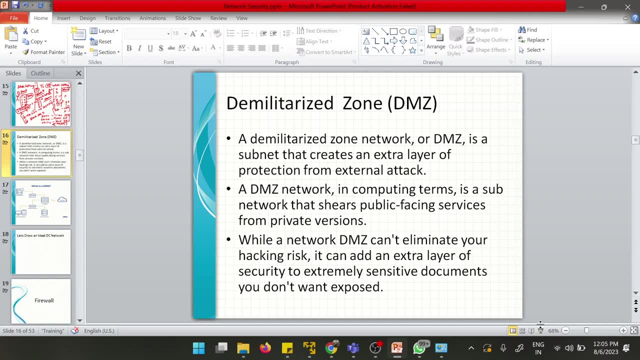 that i would say: okay, so you can go for anomaly detection as a ueba and all solutions. lot of devices are there. when we will talk about soc and all these, all devices will came into picture, but this entire zone. so, moreover, internal communication can be filtered, okay, so 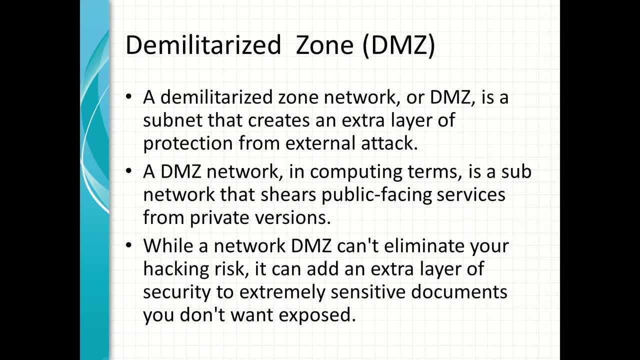 but if you are, if you are accessing a website or something, then in case- in that case, definitely it is a static ip- how it is going to a dynamic ip? google will provide you a dynamic or a static ip, static, static. so always we need to block a static ip. how we can block a dynamic ip? 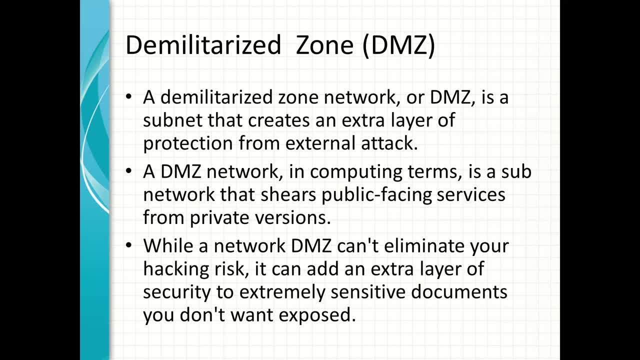 can you demonstrate like ips and ids configuration? definitely, we are going to do that. so shall we move it? yes, can i take a two minutes break? i will just have a water because the continuous two rms speaking my throat is getting dry. yeah, we have spent it two hours continuously and still i am not feeling tired with all such. 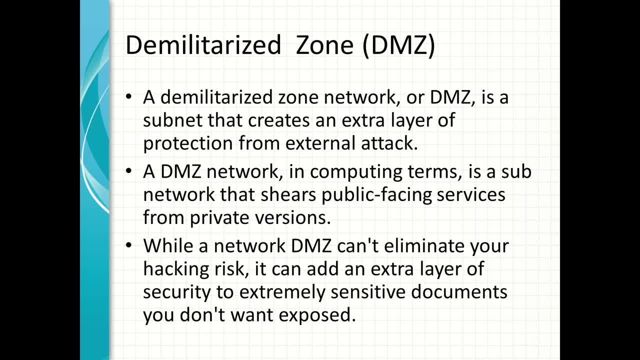 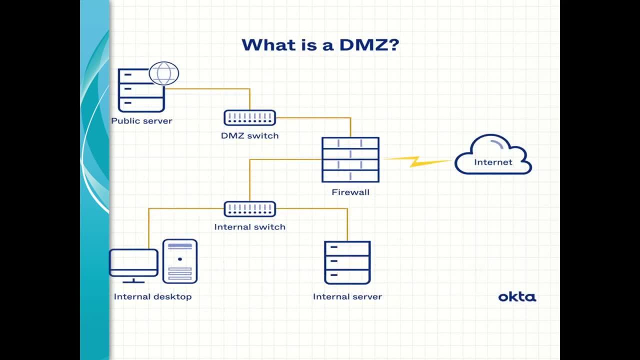 wonderful, enthusiastic participants. okay, so we have understood about demilitarized zone, so i don't need to explain this thing again because we have detailed discussion on that. this is a typical architecture of a dmz, where a public server is put behind a dmz switch. 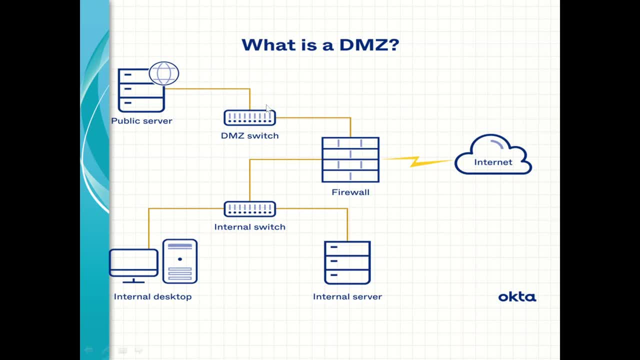 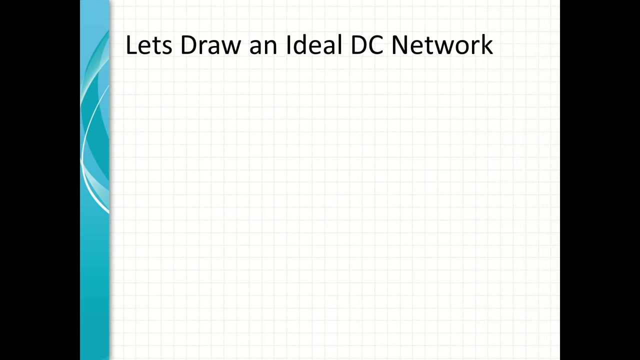 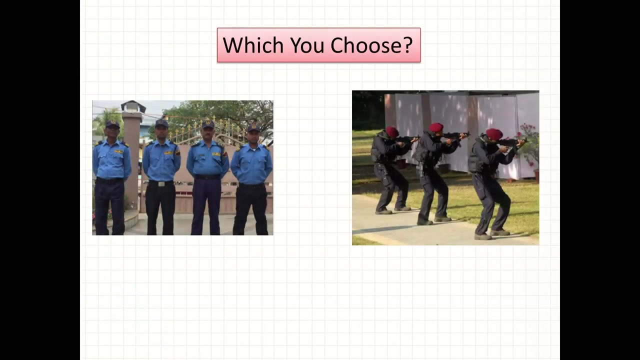 can you relate this gmz switch with that switch? i have drawn on the figure behind the core switch. can you relate? yes, yes, yeah, we have already drawn an ideal dc network. now let's go to the firewall. okay, which one you choose? if you want to secure your building, which one you choose? 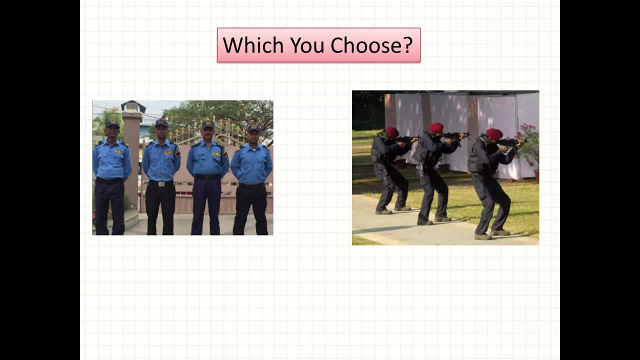 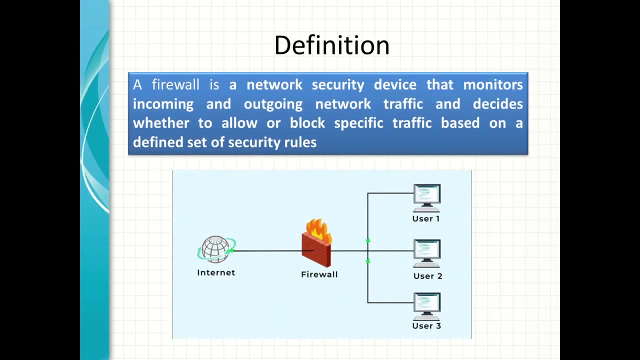 first one or second one, second, second one. why? because they are armed. that's why, yes. so let us define firewall. a firewall is a network security device that monitors incoming and outgoing network traffic and decides whether to allow or block. One small question: You talked about physical firewall. 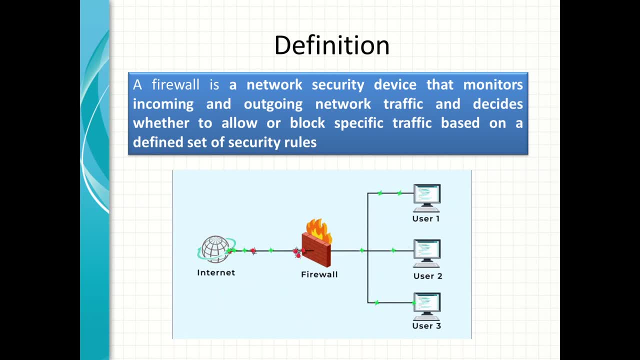 You told that your firewall is physical. Is there any other kind of firewall? Yes, it's coming. after two or three slides It is coming. Okay, thank you. So a firewall is a network security device that will tell you and monitor what is allowed and what is not allowed. 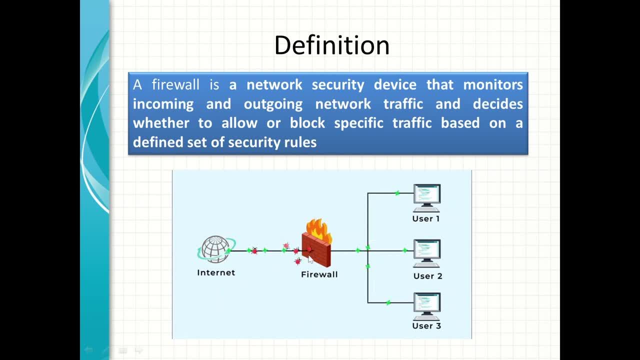 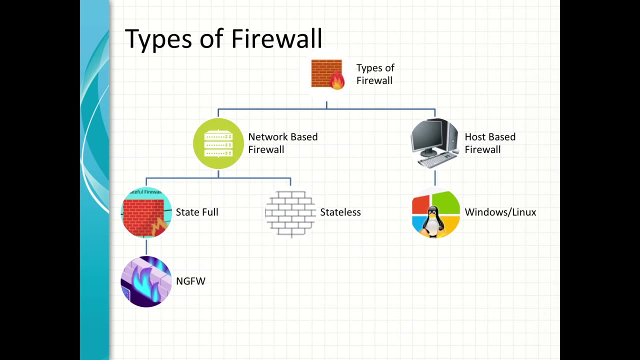 In this diagram you can see the red that malicious traffic is not allowed in the firewall. The firewall is blocking this. Is it visible? That animation? Yes, sir, So this is a simple firewall. Okay, So now we will be talking about types of firewall. 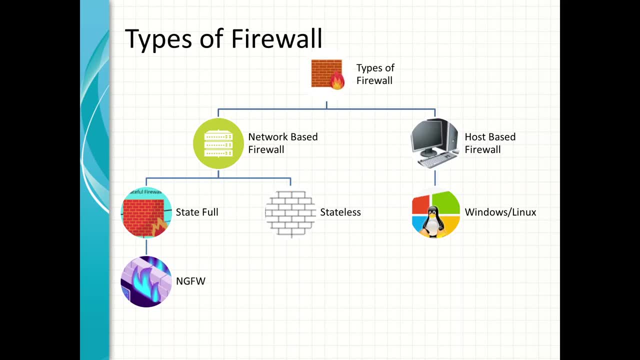 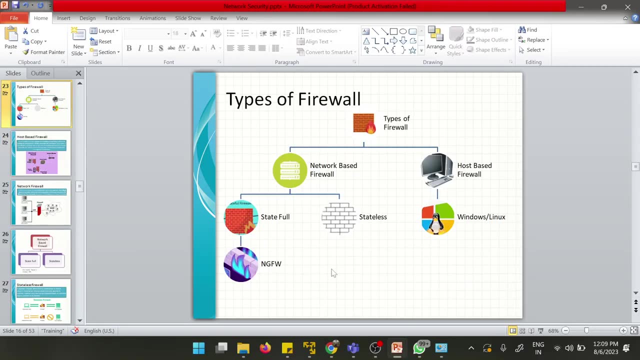 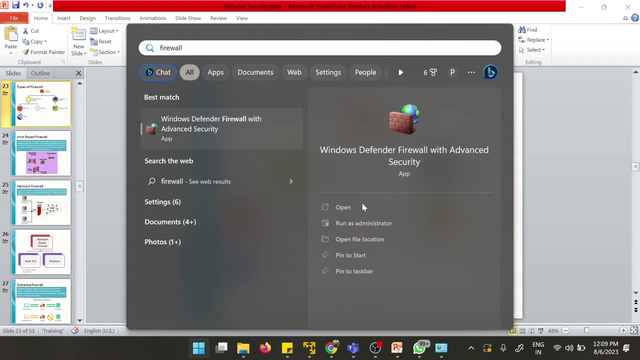 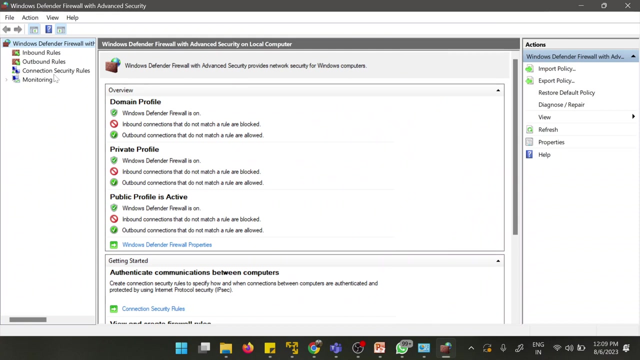 So, basically, we have two types of firewall: network-based firewall and host-based firewall. Okay, What is a host-based firewall? The firewall which is inside your PC? Okay, Because every system, every system itself having a firewall. Okay, So this is your inbound, this is your inbuilt firewall. 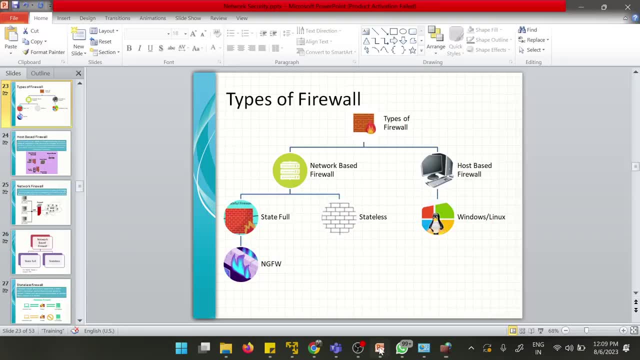 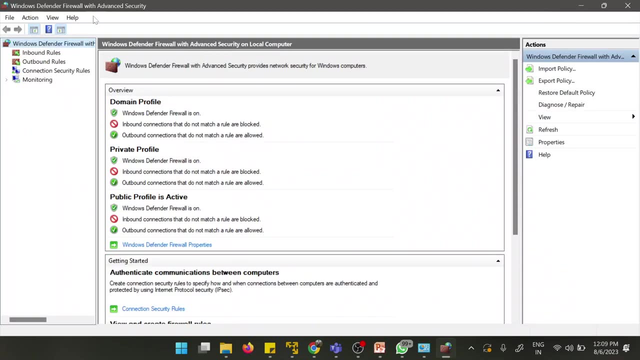 What we called it as a host-based firewall. What it is: Host-based firewall. Okay, So this is a host-based firewall. Are you able to see this? inbound rules and outbound rules: Yes, And these are the same rules we are able to see in that physical firewall. 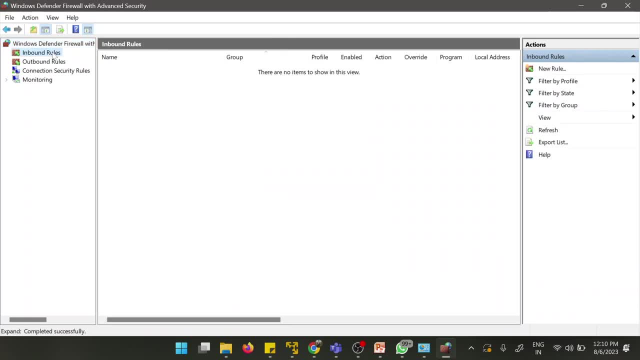 Yes, Yes, in different mode. Yeah, in different mode, definitely, But these are the inbound rules. So system has created all these rules at its own. Okay, And this outbound rule, all these rules are created Like I have created this particular rule for my system. 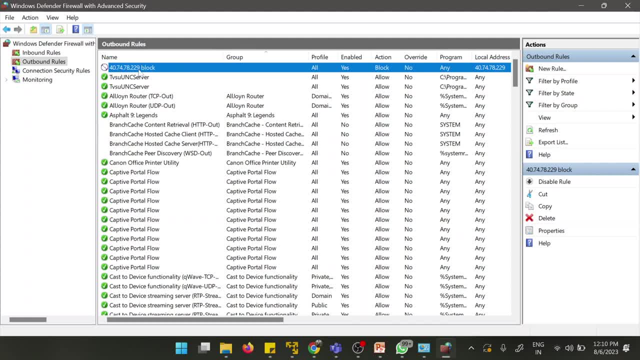 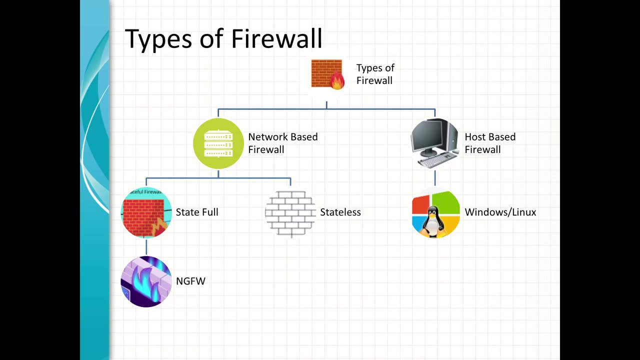 because I found that one malware is talking to this IP, So I have created a block rule for this system. Okay, So you can use your inbuilt firewall, which is called it as a host-based firewall, to configure the same Now, second, we have a network-based firewall. 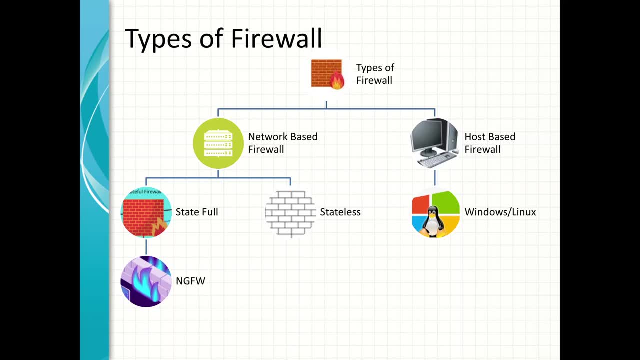 In network-based firewall we have a stateful firewall and we have a stateless firewall, And nowadays there are no stateless firewall exist. Okay, After 1995, all the firewalls are stateful firewall and the advanced feature of stateless firewall for network-based firewall is the stateful firewall. 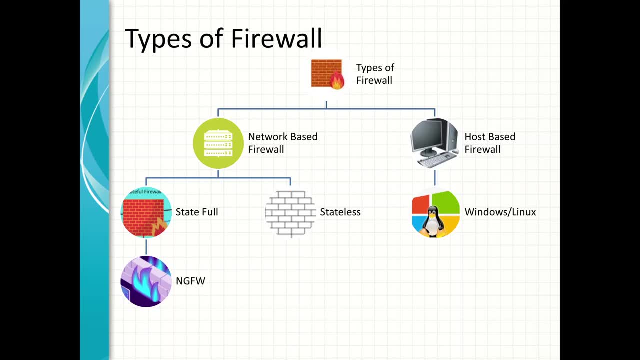 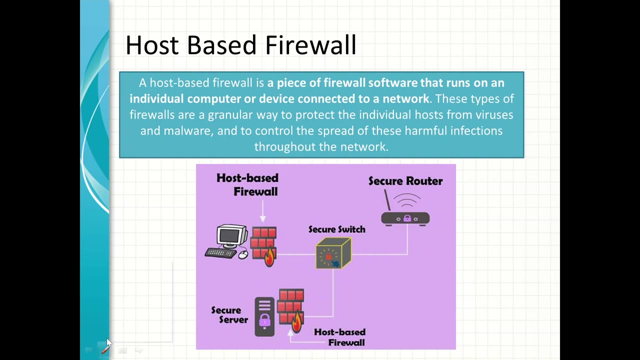 straightforward firewall is ngfw, that we called as a next generation firewall. okay, so we will talk each and everything about it, and then we will be going to talk about the ips and then we will be talking about the ids. okay, so this, this is a host-based firewall where you can see you have a 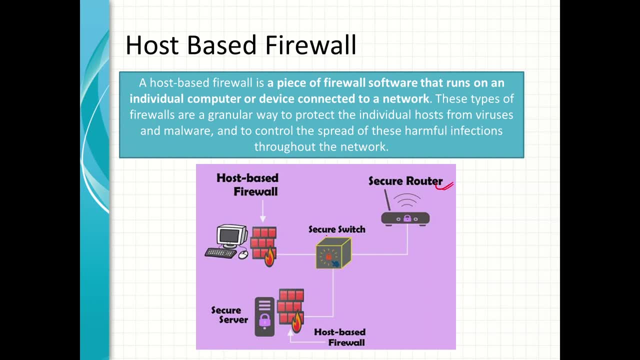 secure router at your home and then you have a secure switch. generally these two things are combined at your home. switch and router are on in a single device. then you have a different computers attached and you have a firewall that is called a host-based firewall. i have just shown you. 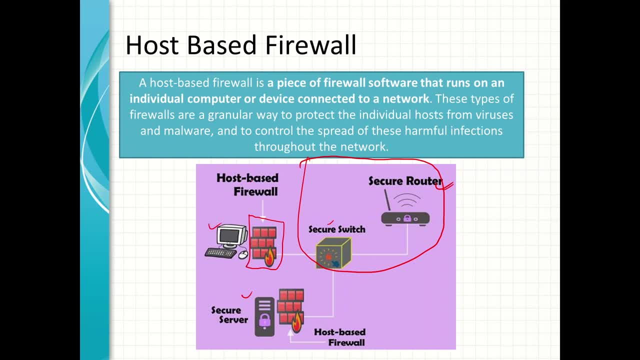 which is on your system and in linux also, you have a acls access control list that can be treated as a firewall in your system. this is a host-based firewall. so a host-based firewall is a piece of firewall software that run on an individual computer or device connected to a. 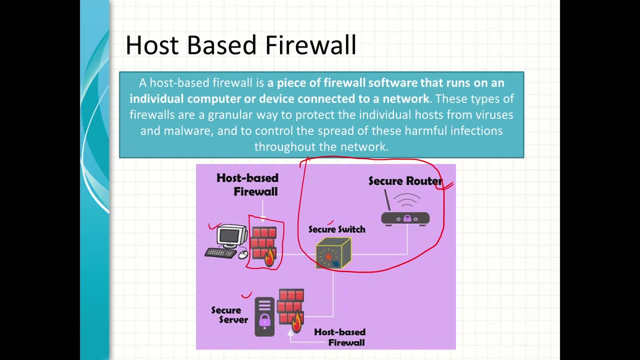 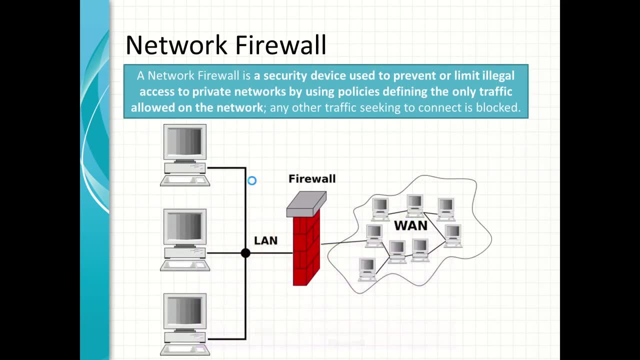 network. these type of firewalls are a granular way to protect the individual host from viruses and malware and to control the spread of these harmful infections throughout the network. so this is a host-based firewall. then we have a network firewall. when we have a very large network, we required to uh protect it, so we required a firewall. 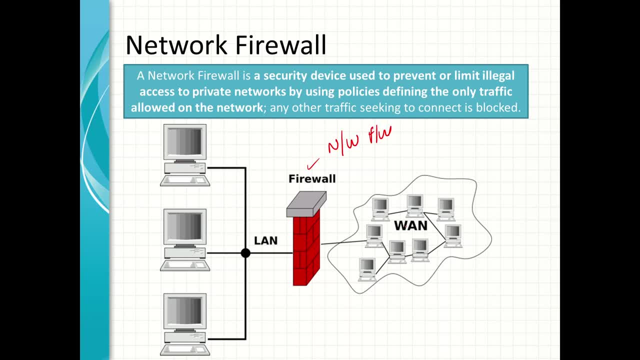 so this is called a network firewall. so this is the internet, this all is internet and this is a workstation inside my network, so we need a firewall to. when a firewall is put down into a network, it is called a network firewall. A network firewall is a security device used to prevent or limit illegal access to private 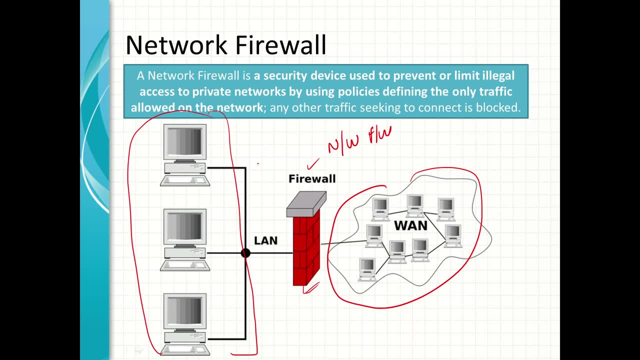 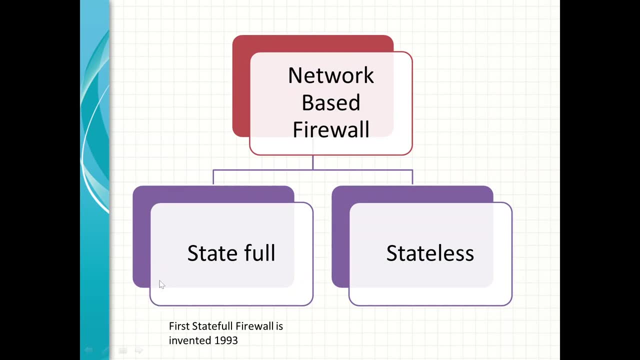 networks by causing policies defining the only traffic allowed on the network. So when we talk about network based firewall, there are basically two firewalls: stateful firewall and stateless firewall. Stateful firewalls are invented in year 1993 and from 1997 or forward, all the firewalls. 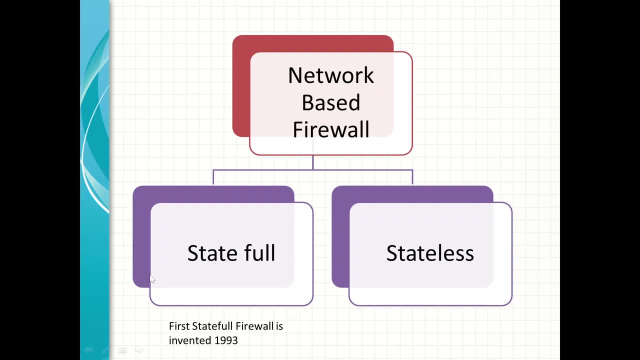 are replaced to the stateful firewall. So there is a very big difference between a stateful and a stateless also, although stateless firewalls are not used now. but I would like to tell the basic difference between a stateless and a stateful, because this is a very big confusion. even I have taken with my lot of 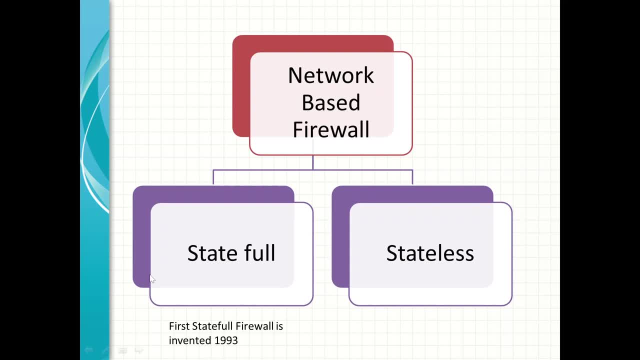 experience. what is the basic difference between the stateful and stateless? because now most of the books are talking, most of the resources that we are available are talking on a different paradigm about stateful and stateless. So let us talk about stateless firewall. 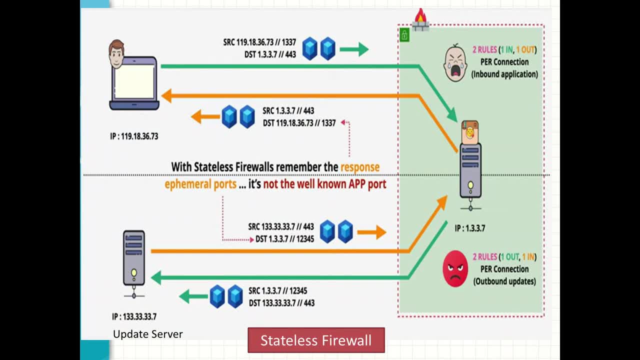 Okay. so before this, just go to this example. okay, is it visible to you? yes, okay, okay, if you see, this is the same example we have talked in the very initial of our session. you know when, when, when I have talked about request and response. remember, Remember this. yes, yes, okay, so in state. so in a stateless firewall, for every request you. 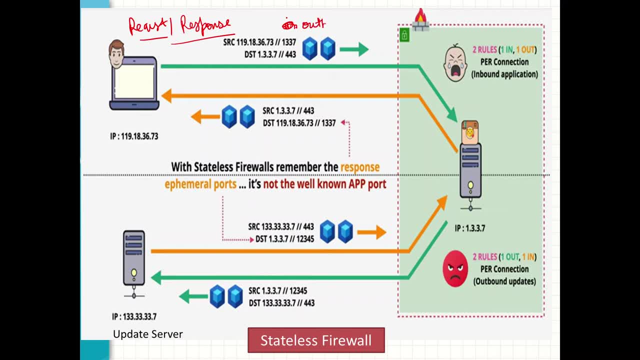 need to create an outbound rule, okay, yes, and at server side, you need to create a inbound rule. inbound rule- okay, I am talking about stateless firewall. so now tell me if this server need to respond back. If this server need to respond back, It is also required a outbound rule. that I have said, yes, and it required a inbound rule. 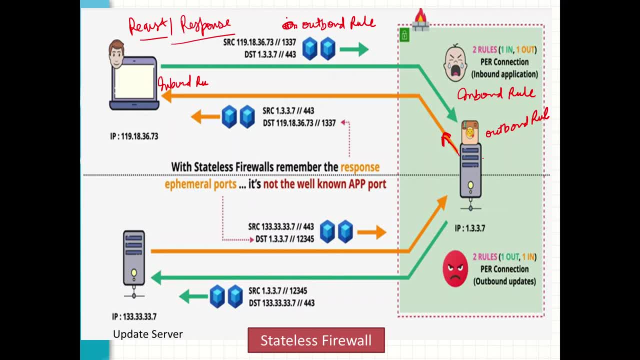 so okay, so actually the thing is happening. the server, the communication between the two, is not understanding the state of communication. it is not understanding the state of communication that if there is a request, It is expected to send a request. now let us suppose a situation: there is an output outbound. 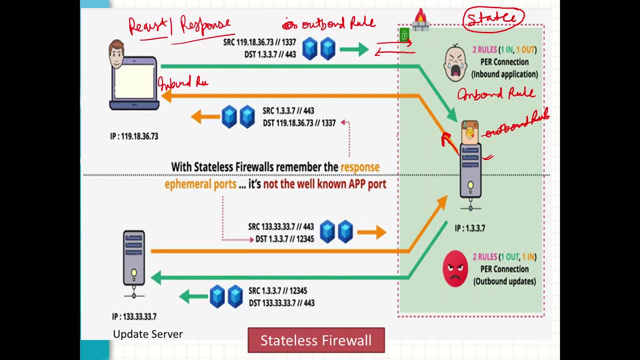 rule is not defined, then do the server able to communicate and reply back? Tell me yes, yes, no, it will. it will not allow to in stateless. in stateless, it is not allowed. what's the issue? is in stateless, two rules are required per connection. please repeat. 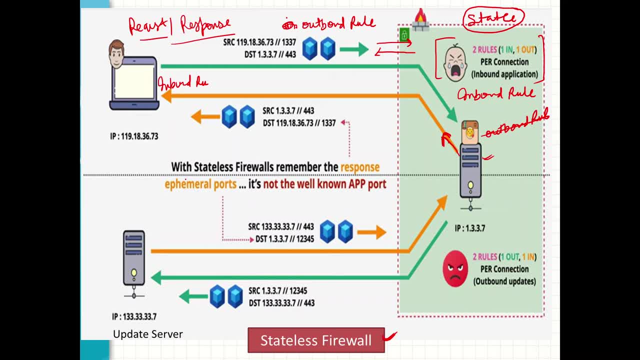 this. Yeah, This is just something very tricky, so I am going to talk on this, not an issue. Okay, what I am saying is, when request came, one rule is required as our inbound outbound and on other side, Now to reply back. I have said that there is a request and reply now on the other side. 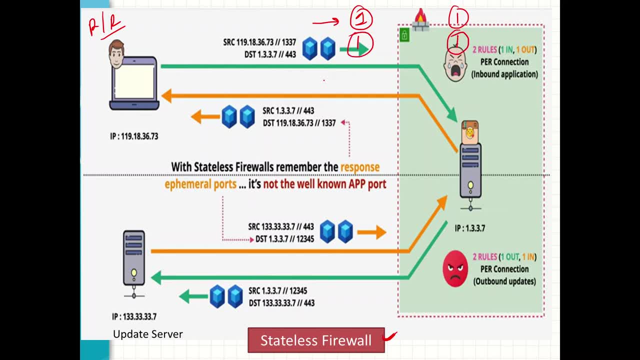 again, one outbound rule is required and again one our inbound rule is required. yes, okay. so this is the problem with the stateless connection. they are not able to understand the state of a connection. State of the connection is When we have Send a dns query. let us suppose when we have send a dns query, this: a person send a dns. 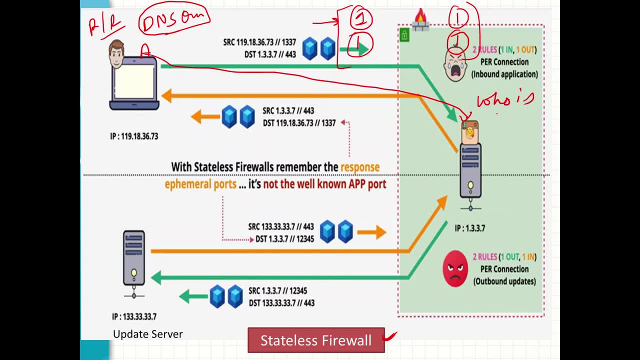 query to this server. who is google okay dot com now? do you think any rule is existing in this server which is allowing you to, which is allowing this server to connect back to you? do you think it is there? it is not there actually. Yes, Yes. 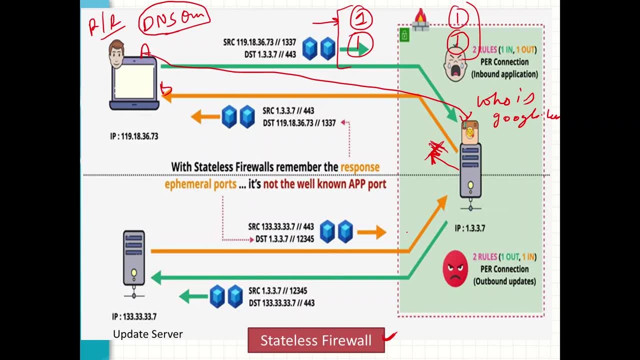 It is not there in the remote server. It is not there in the remote server which is replying back to you. that, okay, go to this server. okay, let us suppose this ip is this: 119, 18, 36 dot 73.. So this server need to have this, this rule. okay, allow one one. okay, allow one dot three. 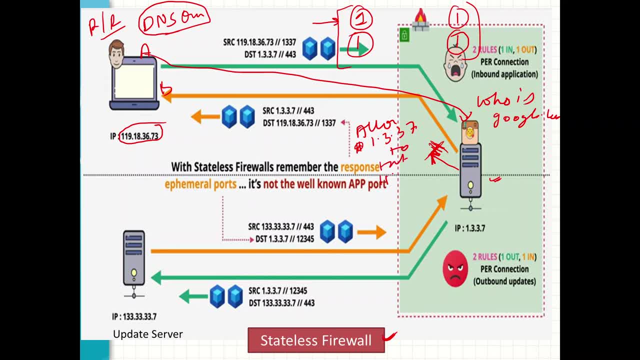 dot three, dot seven, to talk one one: nine ton dot eighteen, dot thirty six, dot seventy three. do you think this rule is available in this? no, it is not available, because in real life scenario this is not available. in real life scenario this is not available, but in stateless. 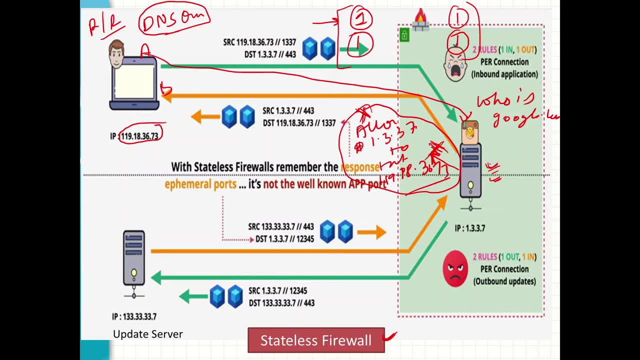 communication. it should be there, otherwise this dns reply is not able to reach to mr a. So what is the problem in stateless communication? Two rules are required, One is the outbound rule and one is the inbound rule. and then again, to reply back, there is: 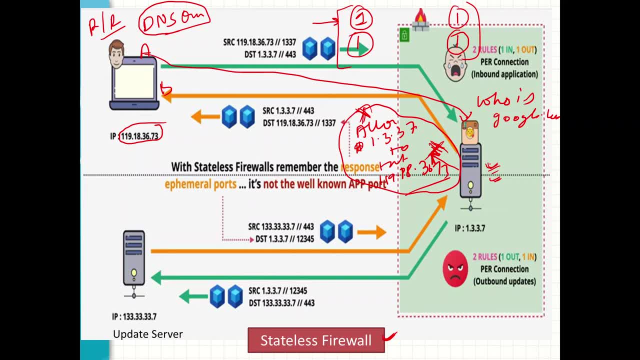 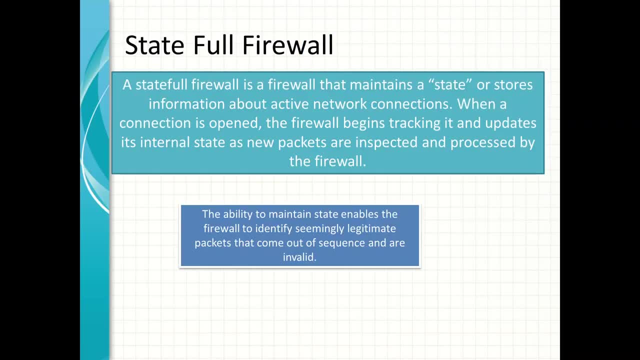 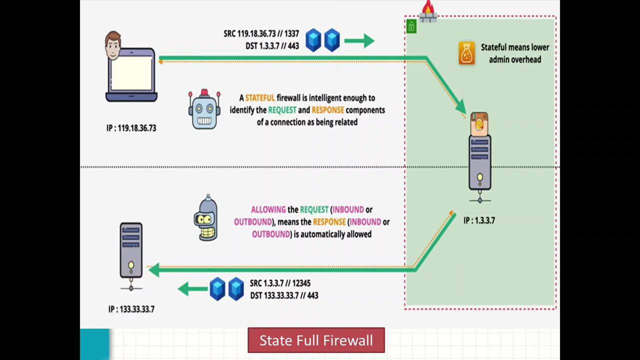 outbound rule from server side and one is a inbound rule from client side, which is actually not feasible. So what they have done? they have created a stateful firewall. what in the state for firewall? as i have already said, after 1998 or 2000, all the firewalls are not stateful firewall whenever. 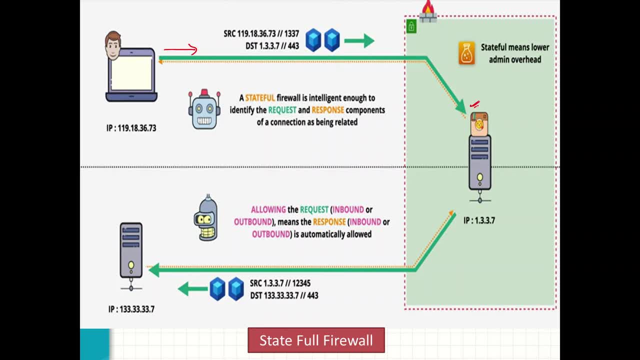 you send A request to this, okay, this firewall doesn't don't need an inbound rule. they don't need an inbound rule. okay, they don't need an inbound rule. they just check the communication and reply back. if it is a tcp request, then let us suppose this is a tcp and this is a client. 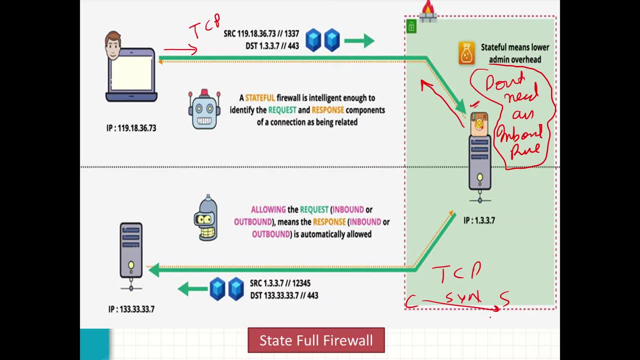 and this is our. client is sending us in request. So It is a. it is a state of communication. client is sending us in request. the server will also send a synac request. So this is a state of communication. this is maintained in a state full firewall. but if 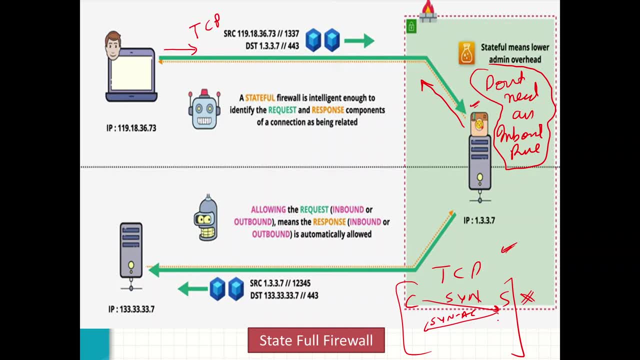 it is a stateless firewall, so this type of communication is not possible. Every time you need to allow and disallow both side to communicate in between. Understood, For stateless, stateless communication. every device will have a inbound rule. Okay, Every device will have two types of rule. yes, one for inbound and other for outbound, outbound. 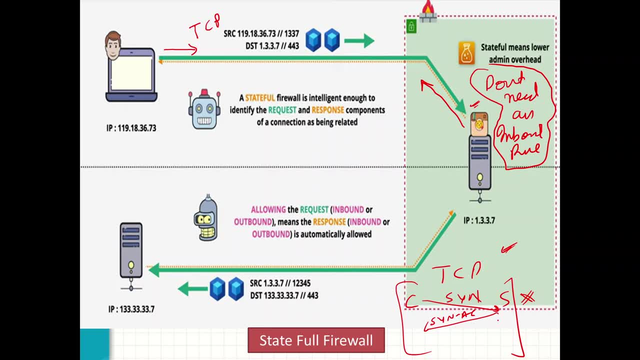 but that actually that is not possible because we are accessing number of website in year 93, when this type of devices are increased. then internet is on very, very early phase. so there are very limited number of domains, maybe 1000 or 2000, and a person using two. 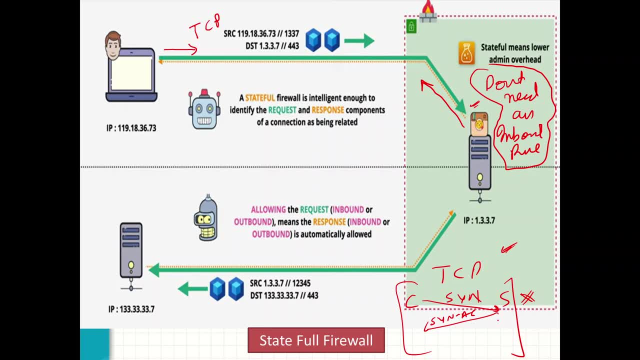 or three, five websites, So You can enter it into their inbound outbound rule. But in current scenario you are having a n number of websites, even countless websites are there. So how can you make a rule set for inbound and outbound? So that is the main difference between stateful and stateless stateful- consider the state. 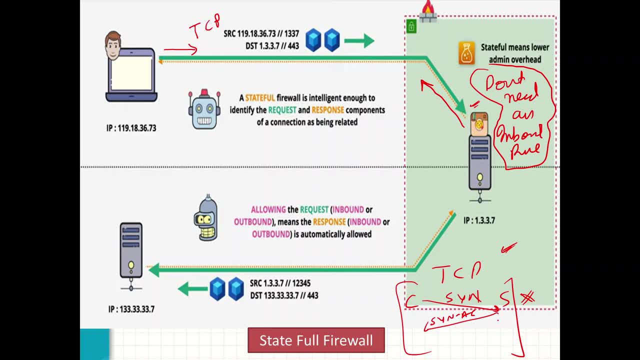 of connection, that this state of connection is require a reply from the server, So a dedicated outbound rule is not required. Understood, Sir, can I ask you? Yes, Yes, Sir, actually most of the OT systems. we have a very few websites like WRLDC website from 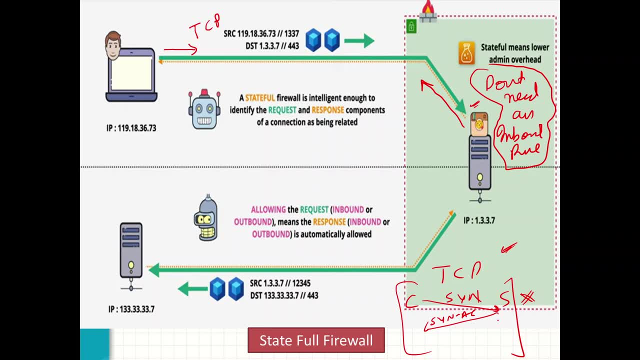 which we have to communicate. so limited number of websites are allowed. so in such cases, won't stateless would be a better alternative, because for all the other incoming we won't be able to reply? Yes, But for definitely for OT. stateless is a wonderful, but stateless are not available in market. 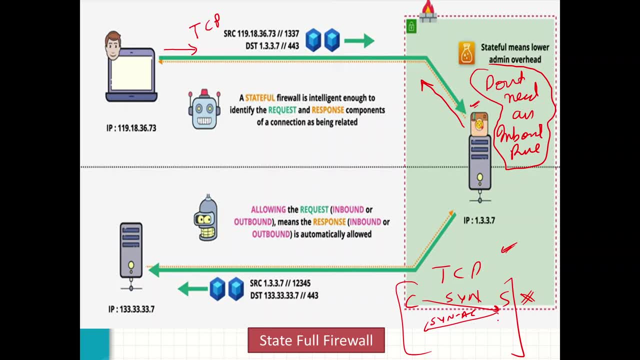 now, But Technically it is good. definitely technically it is good. stateless is a wonderful option for OT environment, but nowadays they are not available. we can. what we can do is we can deploy open source firewall on a separate workstation and then we can use this as a 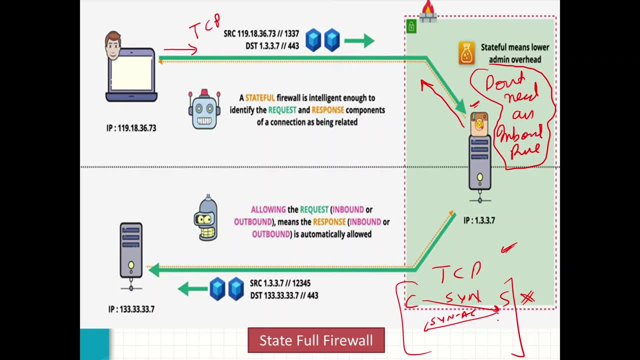 stateless? Yes, Great. And if you are using that whitelisting approach so that the concept of stateless can be adopted using the whitelisting approach? Sir, can you demonstrate Data diode? we can put up. Data diode is something different. Data diode is just allowing a traffic in one way only. That is a different thing. 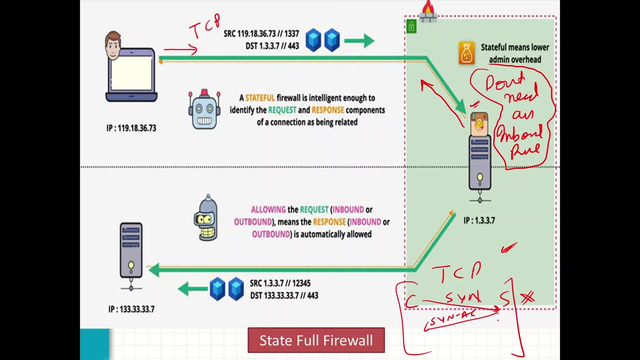 Sir, this is Anil Sir, but any hacker may masquerade through the IP that we have allowed and can get access to our thing. But in stateless, unless we specifically don't give an outbound thing, nothing would happen. Definitely, it is true, Stateless are more secure than stateful. It is a fact. 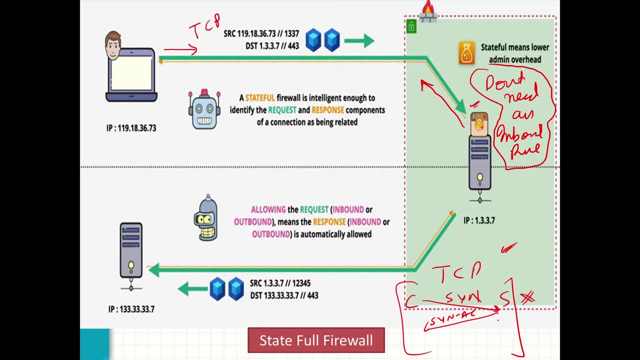 Why did we go for this thing? Because, on a mass level, how many? what do you think in this world? what is the percentage of share between IT and OT? Yeah, that I understand, But still for us… Technology is growing. Actually, the thing is that technology is growing and it is our wish that, which technology we are going to adopt for our solution. 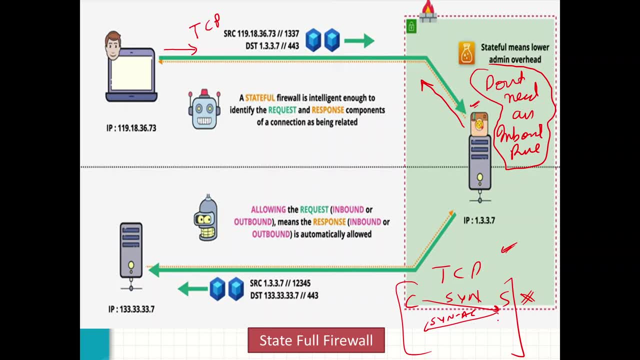 So if we need to go for a stateless, definitely we will go for stateless. We can build our own firewall on an open source environment by putting it on the server and on Linux or something. So I am just talking about the logic. What is the logic between a stateful and a stateless? 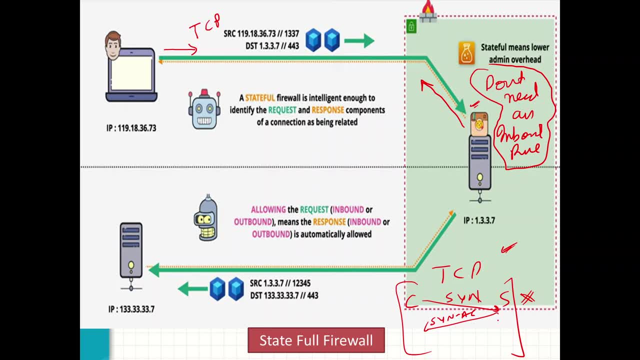 Okay, Any more questions? somebody is asking. Yes, sir, I have a question. Yeah, Sir, I have one question. In a stateful firewall, if communication is blocked, then there will no request will be exchanged and it will not be accepted. 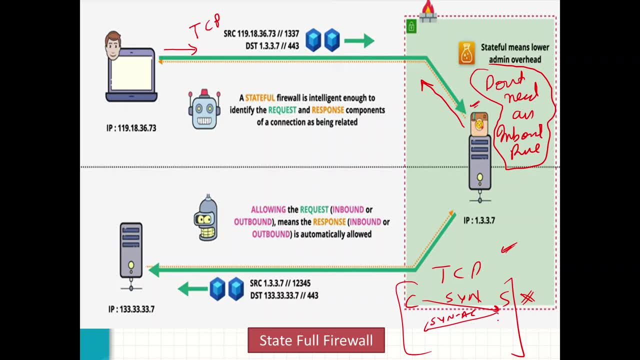 Yes, but if the block is not there, then the firewall will communicate at his own to complete that request. Like if I say there is a SYN request, a client send a SYN request to the firewall, then the firewall will automatically send a SYN request. 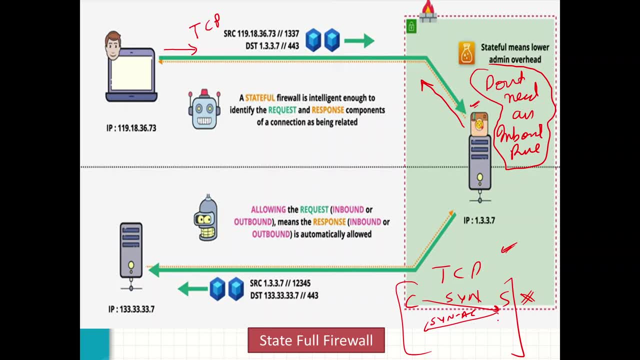 And then if client again send a SYN request, then a connection will be established until and unless it is blocked. Okay, Yeah, Sir, is it possible…? Yeah, please go ahead, sir. Sir, is it possible to explain this terminology with a 104 communication? Is it relevant or not? 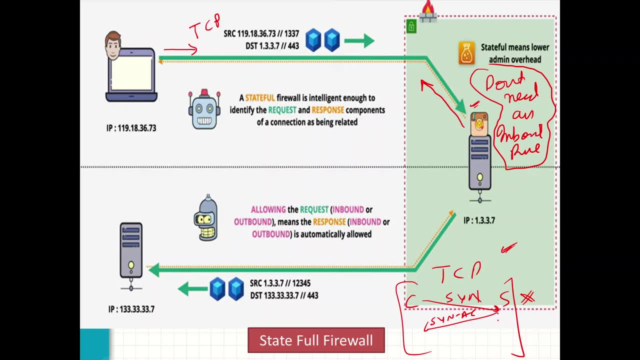 Sir, in 104 communication for stateful and stateless, 104 is already a serialized communication. 101 is a serialized communication. Yeah, 104.. In that case I think it is already a stateless communication. We are not taking care of the other party's state. 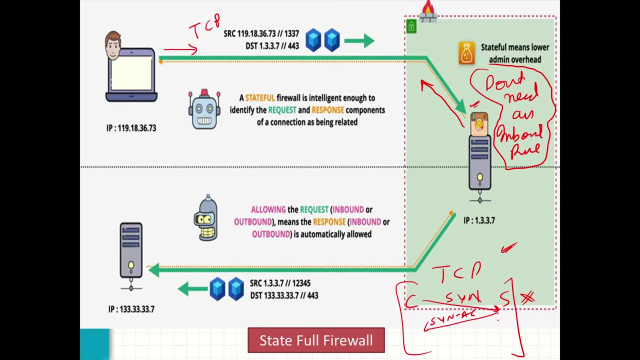 We are just sending the bits to our data historian and all, So it is already stateless, But it is a master-slave communication, right, So there is a communication between a master and a slave, But there is an identity definition between. there should be an authorization between the two. 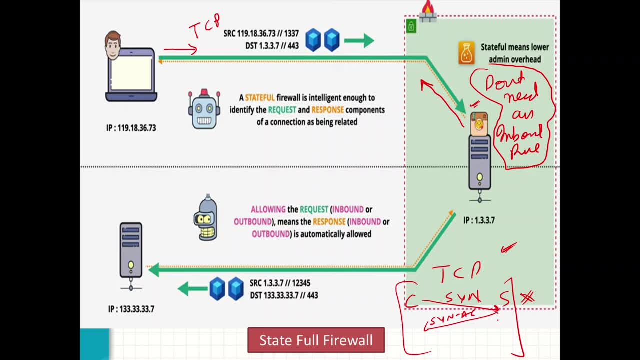 So it is a stateless communication because they are not replying at his own. If communication is between the client to master, then the master is only replying when it is in the list of approved IPs or something. Okay, Okay, Thank you. 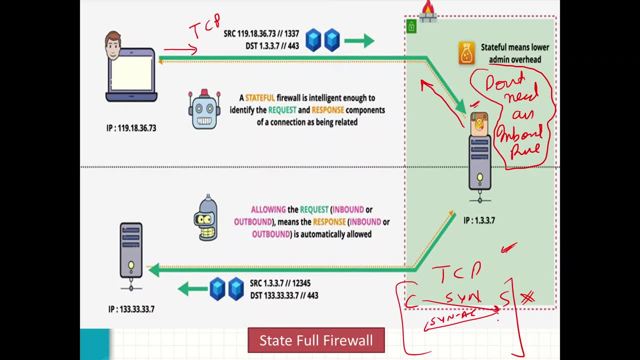 Thank you. One person is asking a question. Yes, Prashanthi, Yeah, Prashanthi Anil here. Yeah, I have two questions. First is that: can we configure the stateful firewall- nowadays firewall- as a stateless? 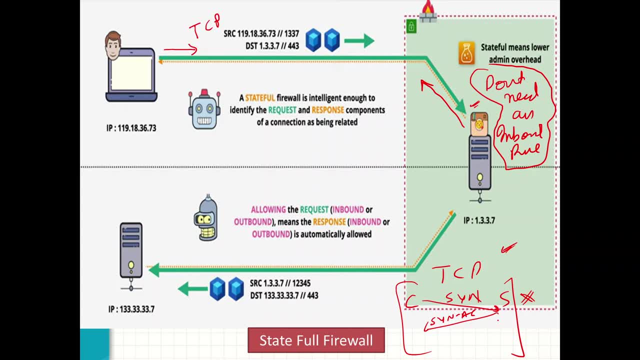 That is configurable? I think so, right, Yeah, it is configurable. So that is why nowadays, stateless firewall is not available. Yes, Point number one. Now, point number two is that you can correct me. One of the major reason is that the DDoS attack, or stateless firewall, is more vulnerable to DDoS attack. 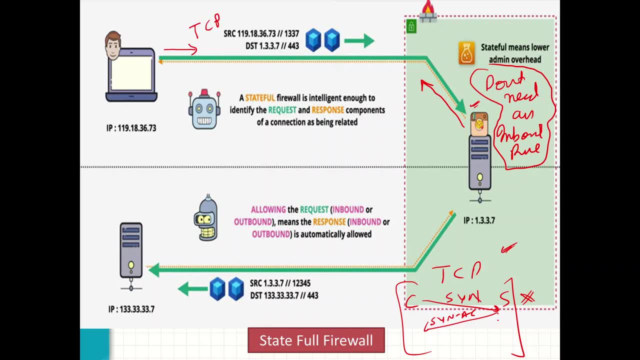 And your firewall will be down by unnecessary- you can say ping- or unnecessary at. you can say acceptance, network, right, Yes, yes, That is one of the major reason. That is why stateless is now not coming and now more intelligent. you can say yeah. 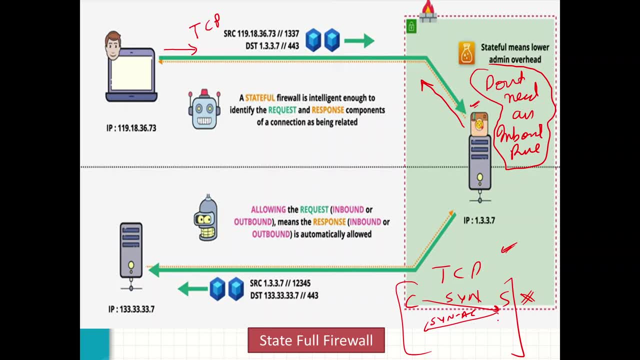 It cannot be the major reason. It cannot be the major reason- Actually major reason- for migrating from stateless to stateful, because the technology need to be fast. to be very frank, Technology need to be fast. You want a high speed of internet. 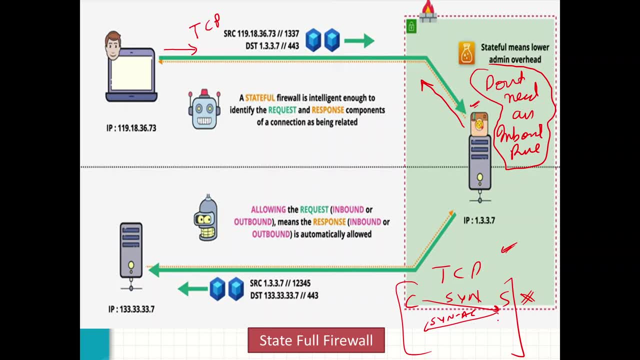 And for high speed of internet. you want to exchange a communication with the least amount of authenticity, Because every time if you trying to send a message- Yes- And trying to search yourself in a, in a rule Like if I tell you, I tell you that in 30 days you blocked 40,000 IPs. 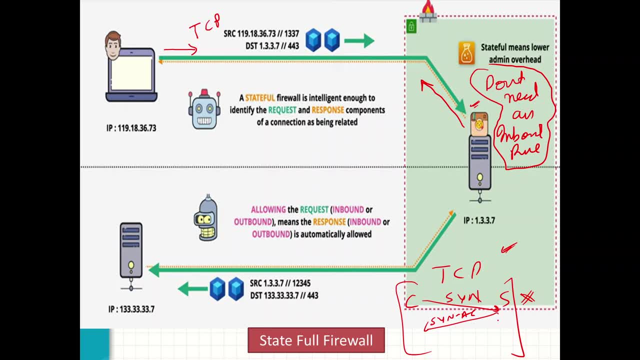 So in that case, if it is going to increase day by day, day by day, definitely DDoS attack is a major reason, Definitely it is there. But technology growing, which includes a faster communication, speedy communication- Now I will say that SD-WAN concept is also came. 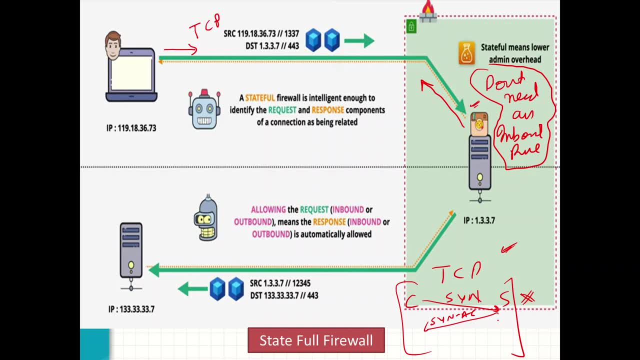 You people are knowing about SD-WAN. Yeah, right, Yeah, SD-WAN, Right, SD-WAN is basically a concept of this, Because we have entered into the stateless and that stateless communication between the routers, when, when we have a control plane and a data plane. 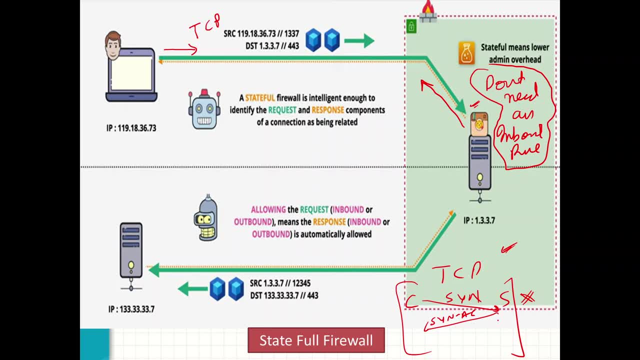 Earlier all the router. on a physical level they have a separate control plane and a data plane And they required a high amount of capacity to to configure the data. But now in the SD-WAN, on the upper layer, we have a single control plane. 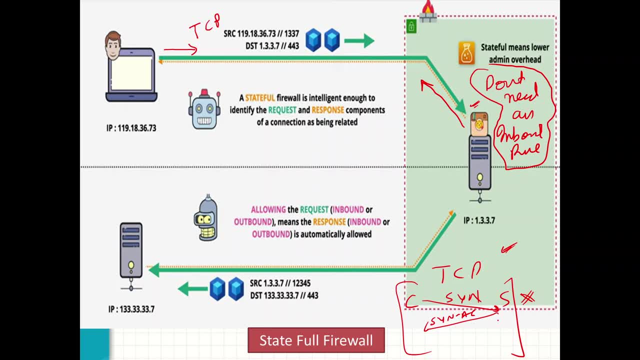 And from that single control plane we are configuring the same. So this is a technological requirement. Actually, Yes, right. One more example: we can say that the managed switches and non-managed switches. Earlier we used to have non-managed switches which are broadcasting only. 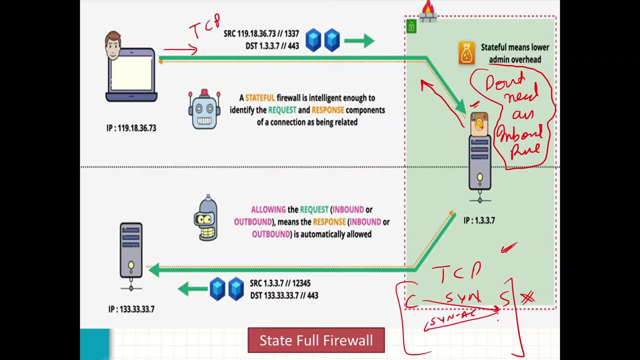 Right Broadcaster: only Yes, Yes, Hub. That is one of the same example. Yeah, Yeah, Hub. only Yeah, Right, Okay, Thank you. Thank you, Sanjeev. I have a question, Anjan, here. 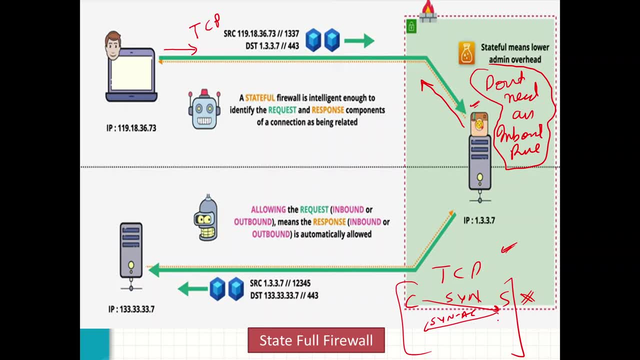 Yes, sir, Please. Good afternoon, Sir. in control center environment we use to use, we use external and internal, both kind of, But there are different make Sometimes. So why you use different make of control firewall? Actually, I don't think that there is any guideline or any requirement to use a different. 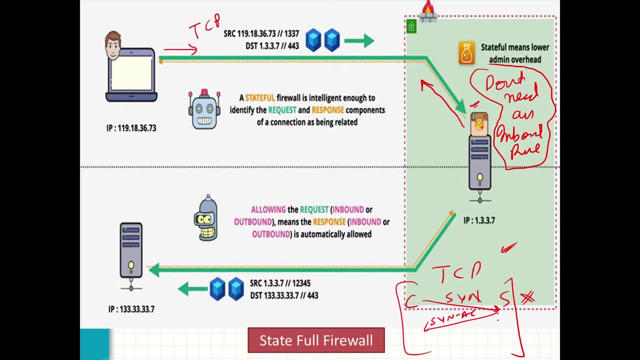 make. Even in my environment I have a same make firewall, So I don't think this. there is a requirement or having a different make, But if there is a deployment from the vendor is like this. So I don't think so. 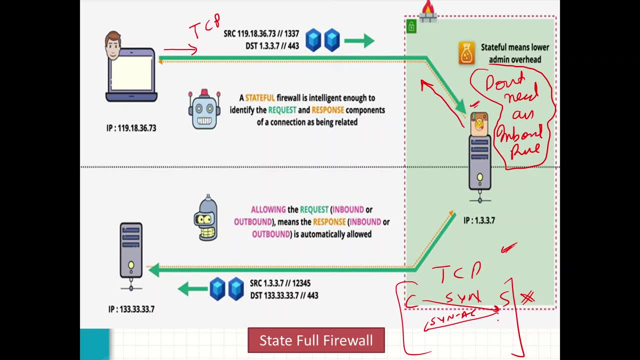 There is a issue. So it will make any advantage. So it will make any advantage. No, No, It will not make any. No, No, No, In many, Sir, any One advantage is there. One advantage is there. 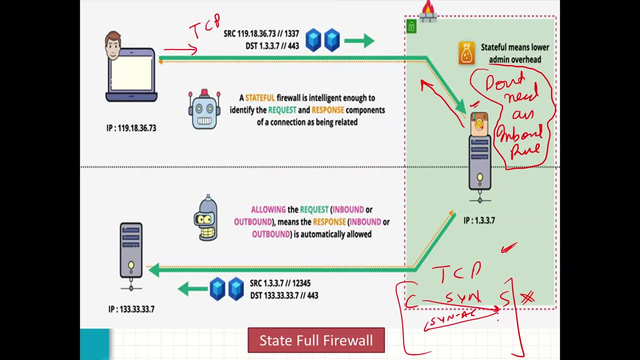 If you have a same make and same model inside your environment. So if your external firewall is exposed and if their vulnerability is disclosed, So automatically your internal firewall is vulnerability is also disclosed. Sir, I am talking about this WBDCL, or most of these utilities and power plants. 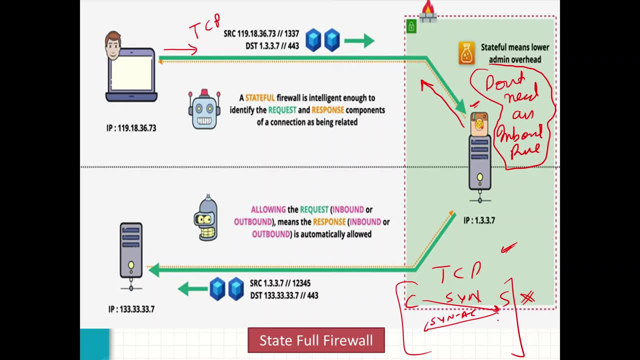 Yes, Utilities and power grids are asking for different make of firewall for their. That may be the one of the reason, Because if external firewall is disclosed and its vulnerabilities are disclosed, So if the same firewall is inside the network, then there is a chance that hacker can use. 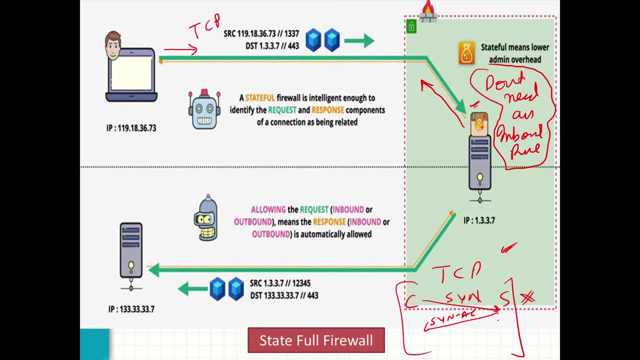 this same technique to intrude the insider firewall. So maybe this can be the reason that why they have given you the guideline. But on the CA guideline I don't think so that there is written anywhere to have a different make in CA guidelines. 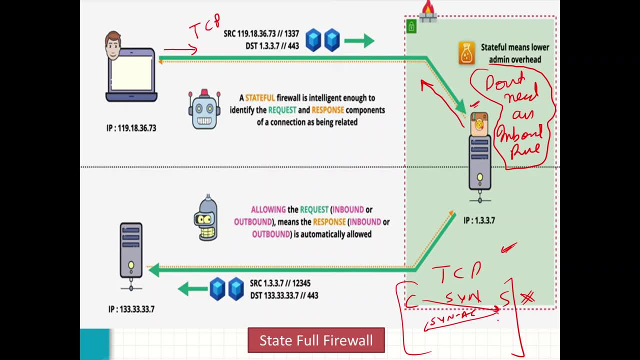 Is anybody from CA here? Yes, sir, From CSET power. Yeah, There is no SS guideline. Yeah, No, sir, Yeah Yeah. Moreover, different makes increases the effort level of the adversity. It will increase the effort level. 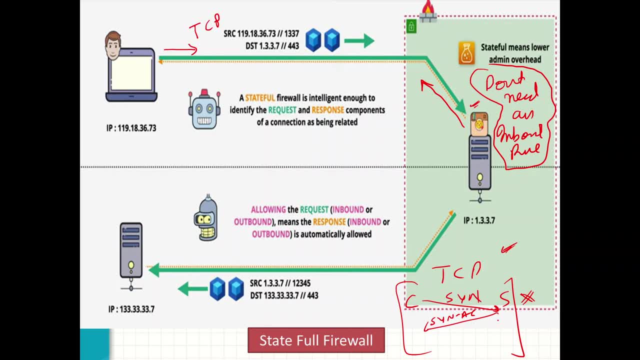 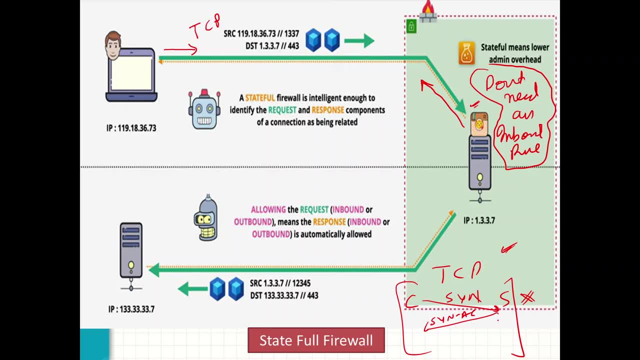 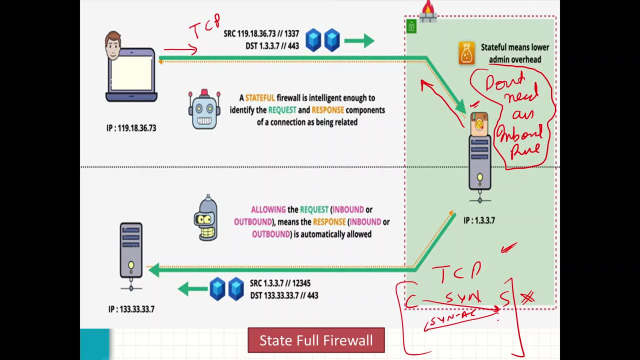 Exactly the reason you are telling. nowadays they are saying to have different vendors so that if one is in, Yeah, I'm probably. I'm just saying a word from that. Definitely, Yeah, probably, probably. they have thought like this, probably. they have thought like this and we: 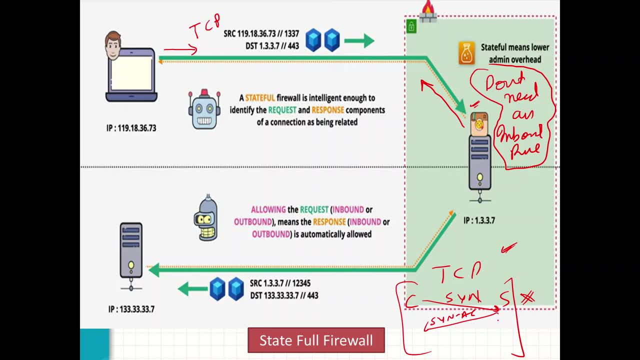 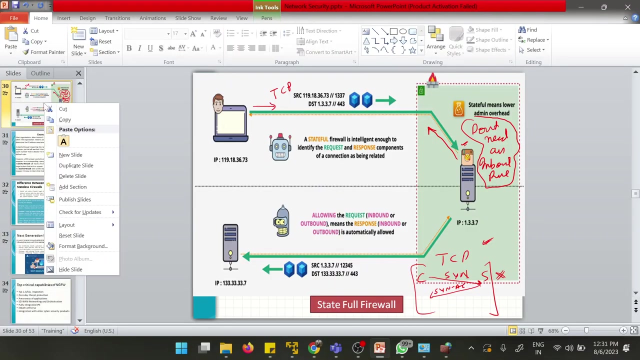 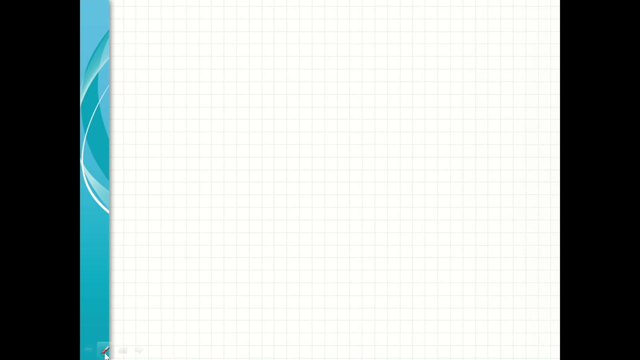 appreciate each and everyone's effort, because everybody has a different, uh, set of security feeling. yeah, so yeah, personally, my question is: is foreign. just give me a minute, sir. one more point you can add in desk once you bought a firework: what is the? is there any best practice analyzer that the configuration of the firewall is? as for 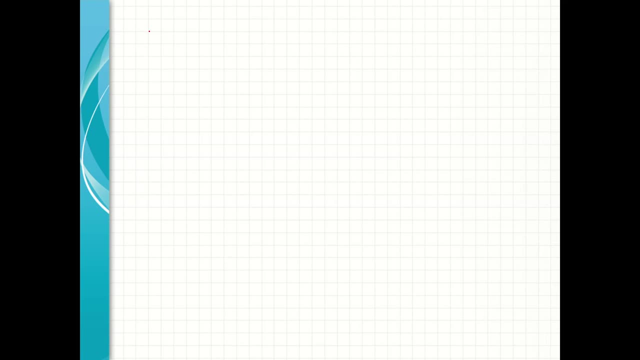 the best because because see, nowadays, but it is not up to the best practice. so if it is gaps are there, then we can check out. what i can recommend is actually: all the firewalls came into the block all mode. okay, so all the services are defaultly blocked in the firewall in a fresh firewall. so when you configure, 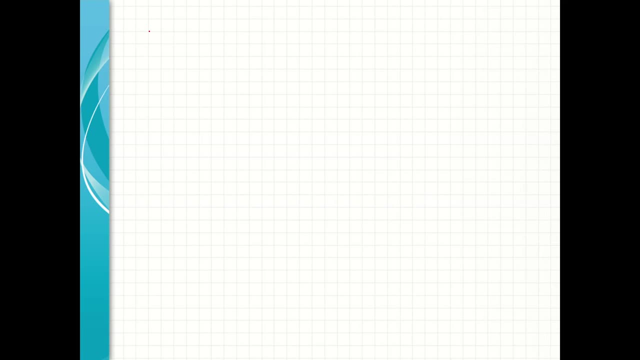 a firewall so you actually allow the services. all the services are already disallowed. okay, and definitely breakfasts are there, lot of, i think. so government organization are working hard to release these. posoko has also worked hard to create the guidelines in the fold meetings and all to have. 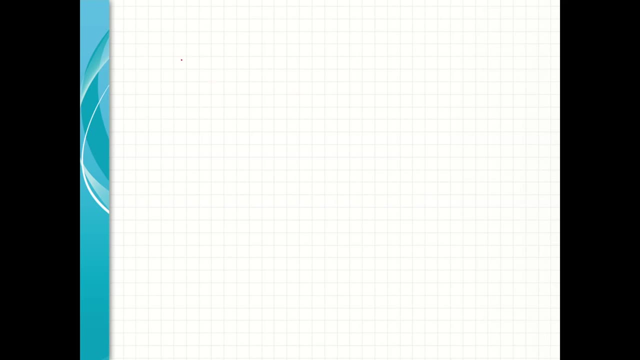 that guidelines for firewall and what so what's the question asked before this? what's the question, sir? sir? calculation of firewall, actually not the calculation. firewall is all depend upon how much throughput you're required. okay, let us, let me give you a one second right now. right now, you, now we can go for that one second. 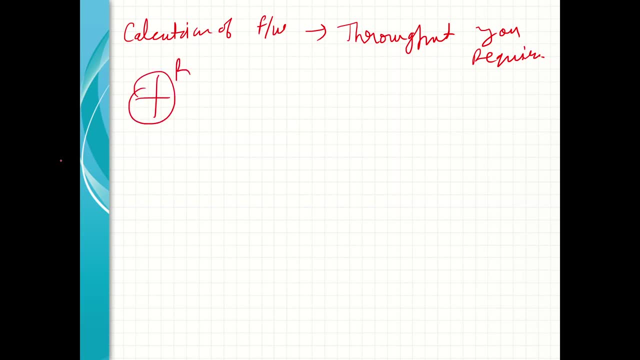 solution. this is okay. you have a router and here you have a firewall. here you have a core switch and here you have a separate DMZ switch, AMZ switch, LAN switch. in LAN you have a hundred PC in AMZ. you have a 10 server in DFZ. you. 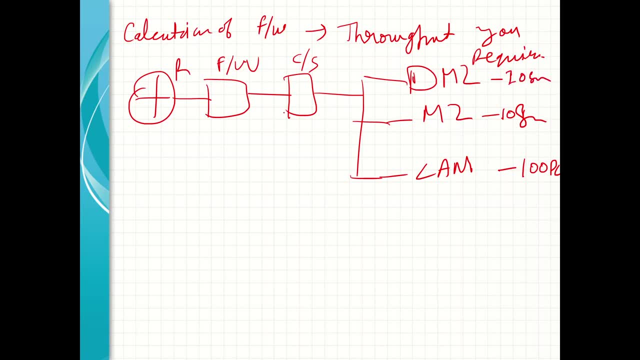 have a 20 server. okay, now to calculate this, you have to understand what is the ISP bandwidth. okay, bandwidth. let us suppose the bandwidth of ISP is 500 Mbps. okay, now let us suppose about a core switch. your core switch is off. 2 gig, 2 Gbps, okay, what is your core switch capacity? 2 gig means throughput. let us. 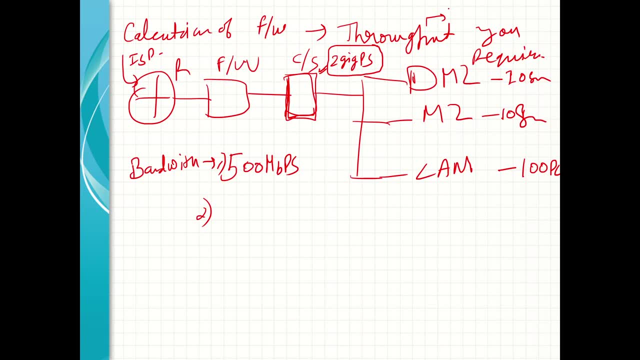 underscore. let me tell you one thing: what is throughput? throughput means the maximum data that can be handled by a server is called a throughput. if the packet is start dropping at 3000 Mbps, it means the throughput of a firewall is 3 Gbps. understood this thing? what is throughput means yes or no? yeah, 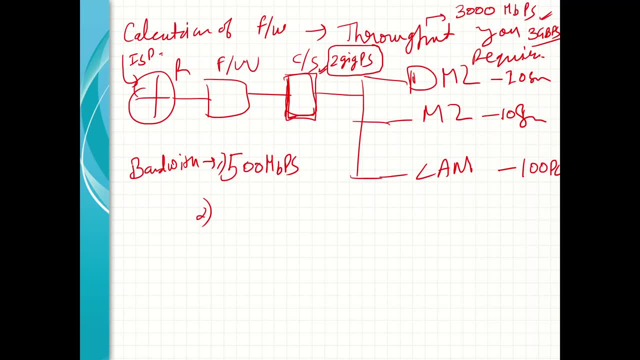 so now, coming back to the question, let us suppose the ISP is of 500 Mbps, your core switch is off, 2 gig, okay. okay, the SFP is connected. and for DMZ, you have a 20 server and for each server you have a bandwidth of 1 Gbps. okay, and for AMZ, you. 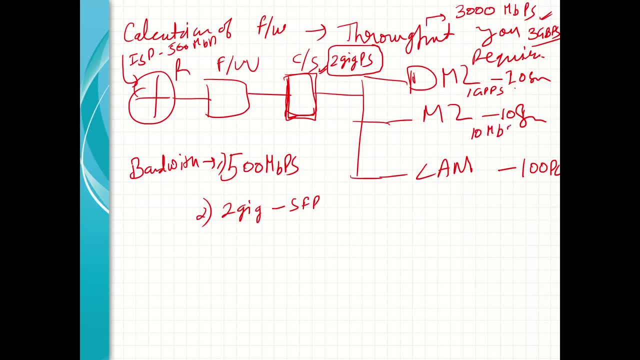 have a 10 server of 10 Mbps switch. take it as a 1 Gbps more than 100 Mbps and in this you have again 10 Mbps. so 2 gig: 10 Mbps into 20, 10 Mbps into 10 and 10 Mbps into 100. so this shall be. 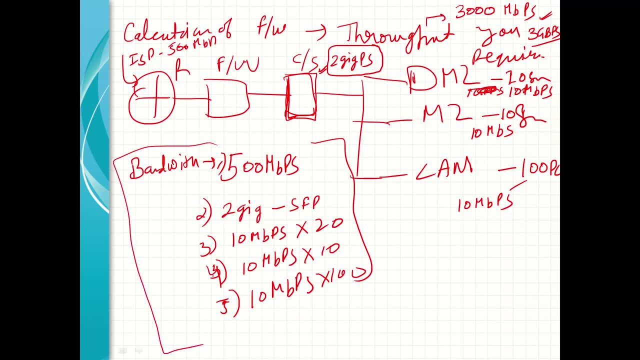 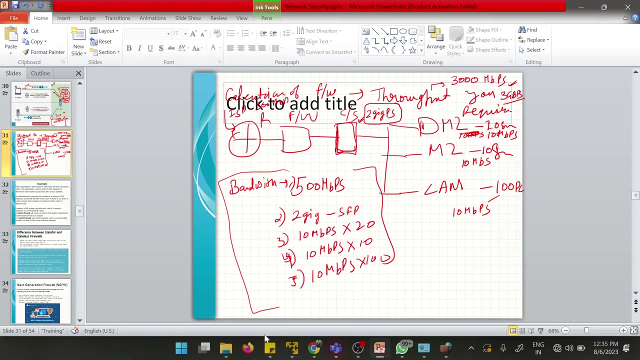 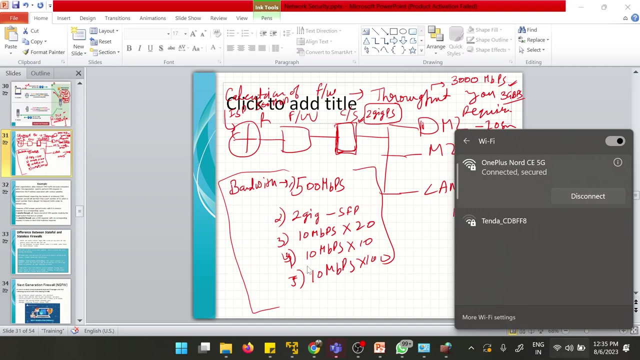 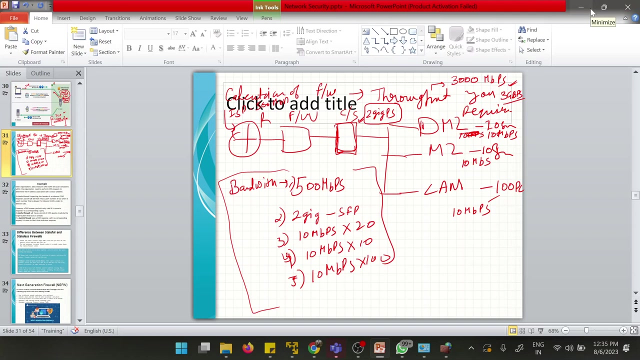 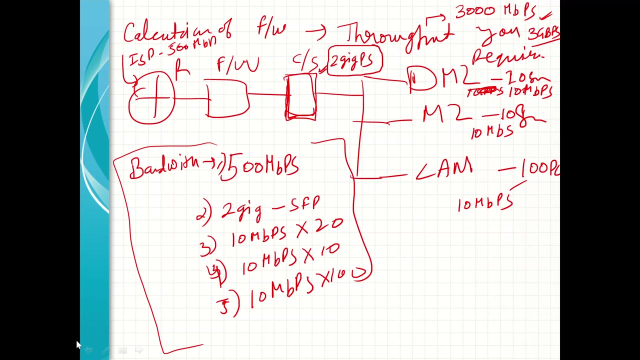 your ideal bandwidth. you required to cater your issues. understood, tuu? yeah, what are you doing? yeah, what are you doing? ok, so i am waiting, sir. yeah, is it fine? ok, So is it visible now? yes, yes, yeah, so we have calculated. this is like my ASP bandwidth. 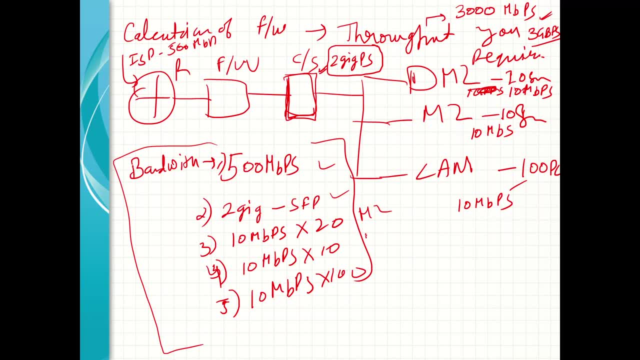 my code switch bandwidth, then I have a MZ, DMZ and length. so this is the ideal bandwidth I required for the hole. this is the ideal bandwidth I required. okay, so this bandwidth can be treated as a throughput when we calculate this. let us suppose it is coming to be 20. 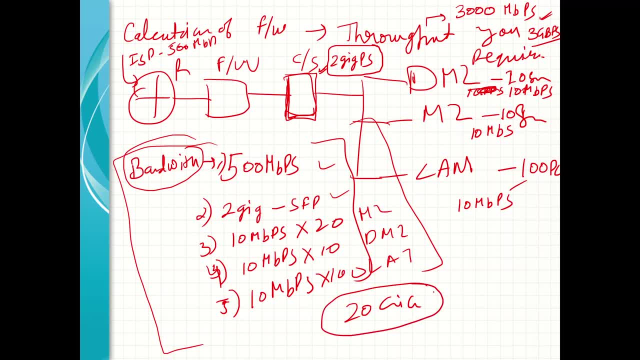 gig. okay, this is coming to be 20 gig. it means that your firewall should be of minimum 20 gig. Okay, 20 gig. your firewall should be of minimum 20 gig, so you can ask your vendor to provide you a firewall with a 20 Gbps to 20 gig capacity. understood any question in this. so it is. 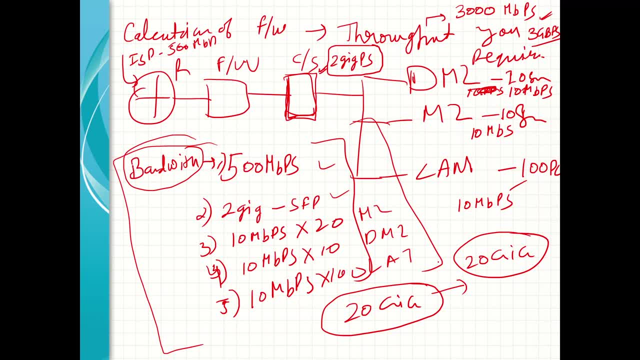 a simple calculation, not an issue, any question. Number of users. number of users depend on the number of users I have taken. I have taken 100 PC 100 users. Okay, okay, Yeah. So you need to say that when I purchase a firewall, I should be aware of the number. 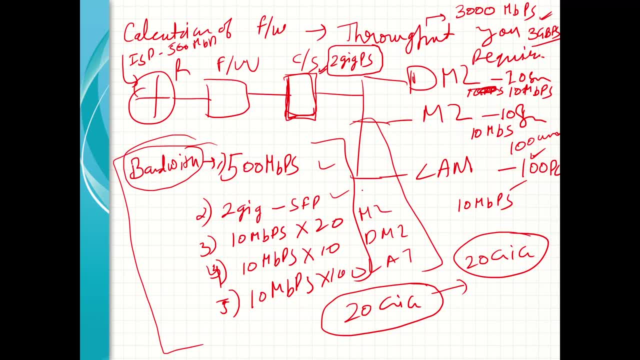 of machines to be connected Definitely, Even in future also, Definitely, definitely. and also you can take around 20% of overhead. You can also take 20% overhead The number of users or number of concurrent corrections per user. No, no, actually, how would you configure it? 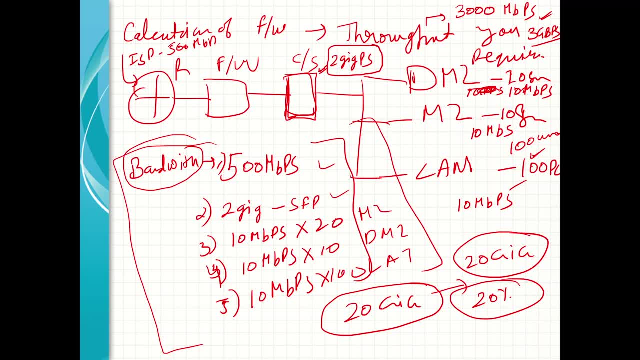 I don't know, I don't know, I don't know from the concurrent connection, because every time current corrections are different. you have to place a firewall and calculate with the maximum capacity you have. Okay, just think of a situation when you select and go to the electricity connection. how? 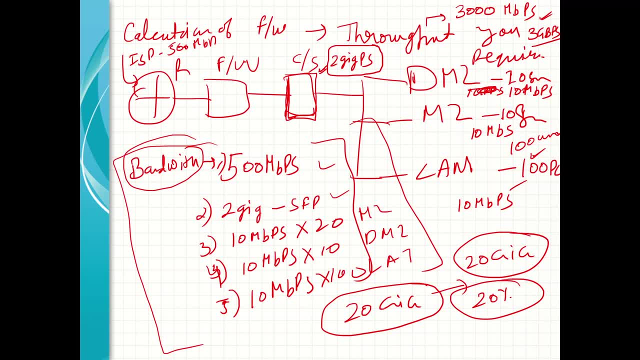 you can calculate a load or a connection. Number of devices connected, okay. The number of devices: Number of devices connected: okay. So if I have a connection connected, okay, let us suppose if they are. if you have a, five acs and, and each ac is approximately, 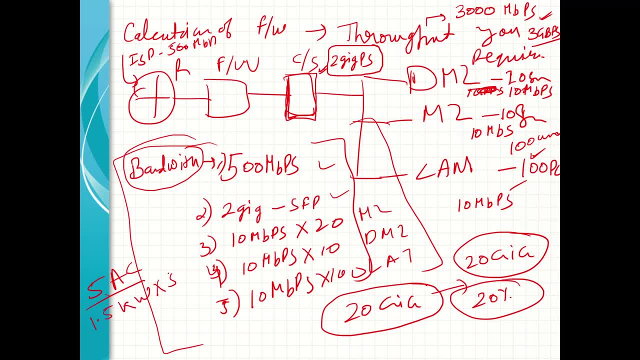 coming 1.5 kilowatt. so 1.5 into 5 is around 7.5 kilowatt. plus you have a 2 kilowatt separate connection, separate load. so how much connection load you will go? you will go for 12 kilowatt. 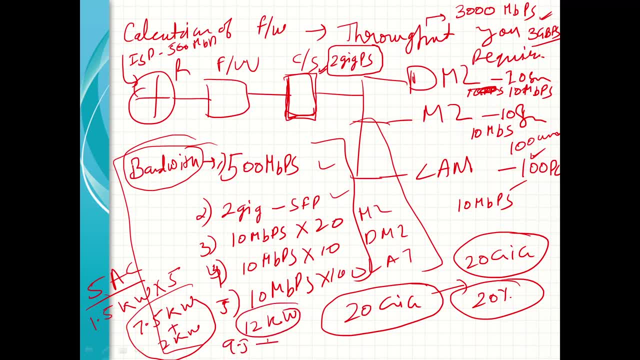 because although this is 9.5, but you will take 2.5 as a overhead, because in case you increase your ac to 7, then you must have an extended capacity, so the firewall is having different bandwidth. also, there is a firewall throughput, then ipsec, epn throughput, then threat protection. 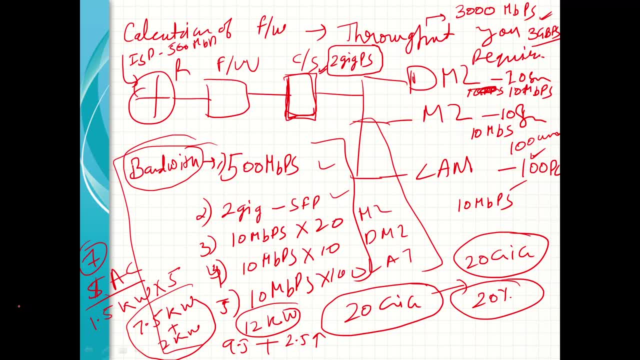 throughput also there. yes, yes. so because they go, the highest is firewall throughput and i would say the highest is firewall throughput. then we have ngf throughput, ngf throughput- when we talk about ngf now, then you will get a clear idea about ips and ids throughput. okay, i will cover it, no issue. 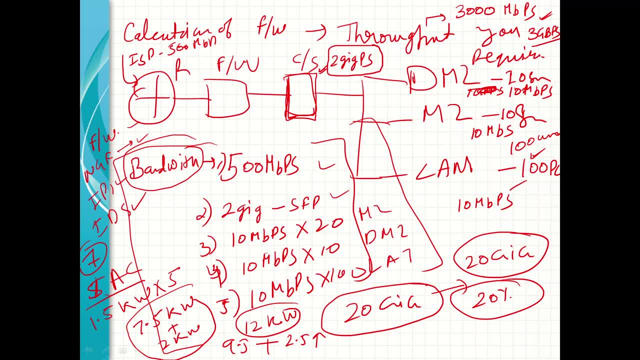 so let's go ahead. but uh, internet isp is a 500 mbps, which is lower than the capacity, because isp will be only able to talk with the 500 mbps capacity when simultaneously talk is going on. uh, then why do we need the internal will also talk, that we go through the cs, right? 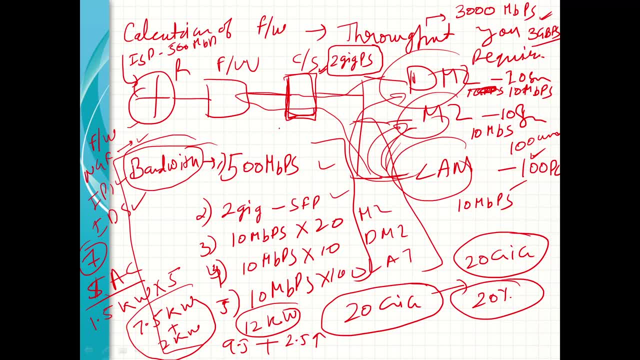 no, no, it is going to firewall only actually. in physically it is showing, but in actually it is going to firewall only because where you have created the rule, land to mz where, ah, yeah, in firewall, yeah, so these traffic are all going to be firewall only, sir, okay, okay. 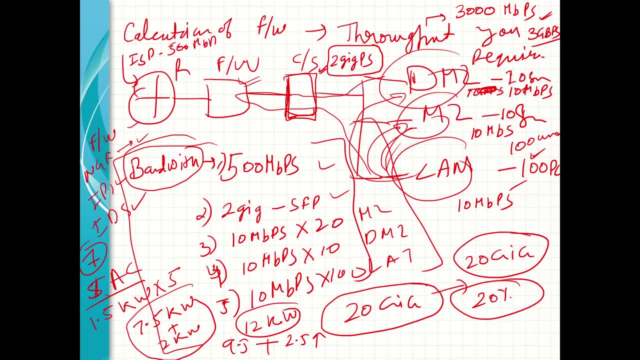 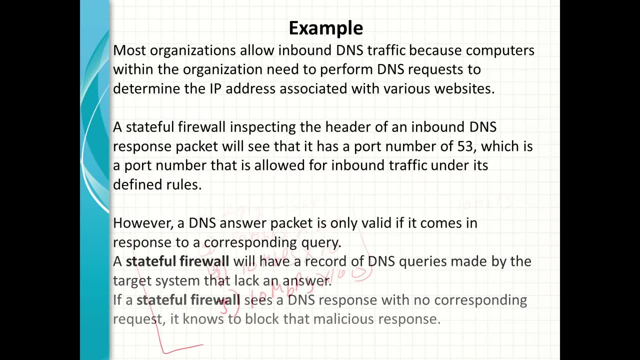 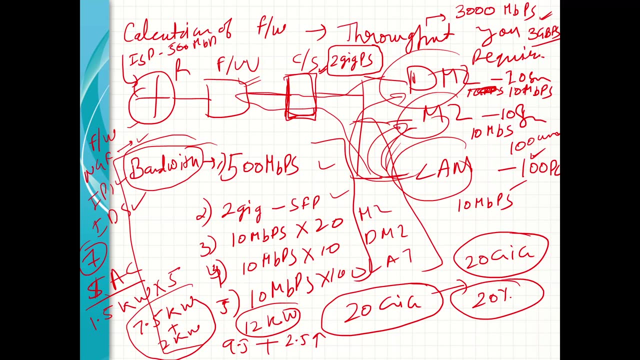 so shall we move it? uh, sir prasanji, on this side, i have just one question. uh, these firewalls and utms, these days we can actually restrict the traffic that is coming from outside the country. so, uh, can you explain, like, how can we do that? i mean suppose, if i want to, 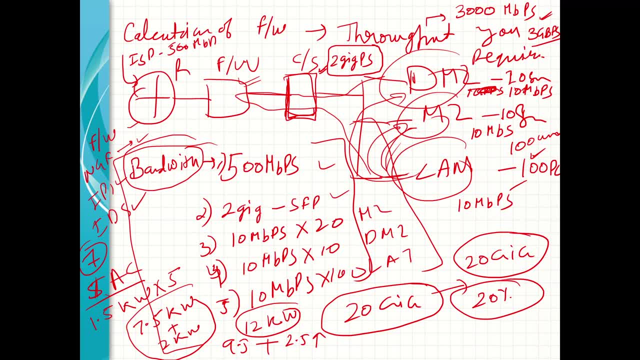 restrict all the traffic outside india. whatever option of geo fencing, geo fencing- there is option that is we call as a geo fencing, and you can activate the geo fencing feature. it will block all the mill, all the traffic from the particular country, or you can block all that outside traffic. 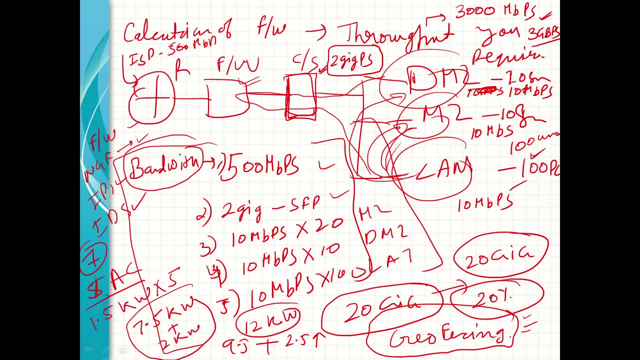 in your environment, so it comes by default in all these other environments. yeah, most of the firewalls having this feature nowadays. okay, good, good, okay, uh uh the way. uh this uh uh the way. chinese government has not allowed anything to work. can you do a case study? 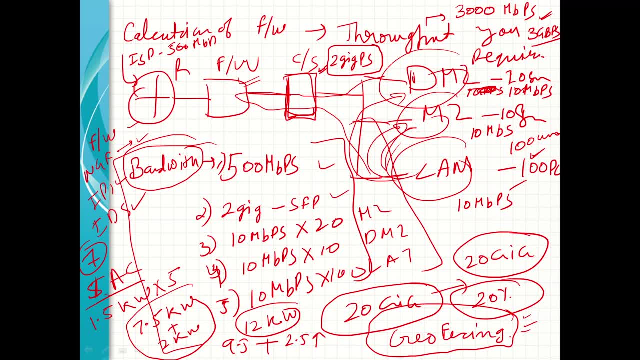 on that, sir, if possible. uh, okay, i will. many, i will do it sometime after this because we are running out of time. definitely i will take that. yeah, sure, sure, because we have a long journey to go. we have a long journey to go for three months. definitely, we will take that. okay, so shall we move. 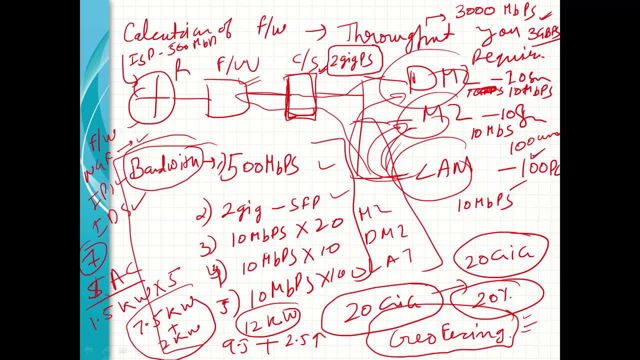 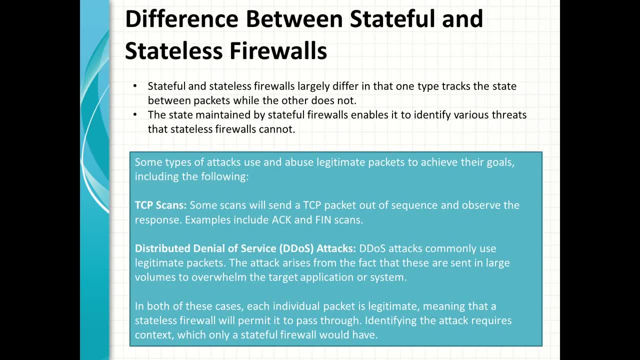 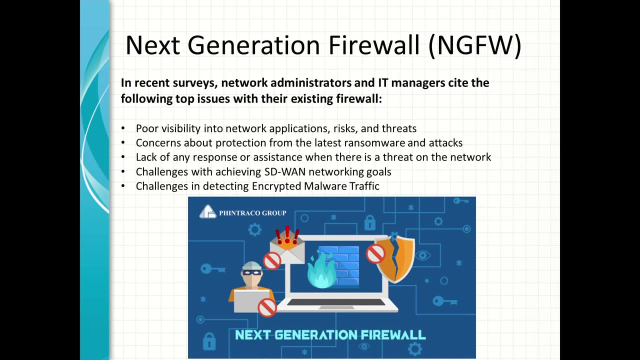 ahead. yes sir, yes, please, yes sir. so we have talked about difference between stateful and stateless firewall. so i think now you people have a better understanding about about this. now we have a next generation firewalls, okay, so what we can do to prevent it, sir, for its prevention, there are some options in your ngfw that, if it is, 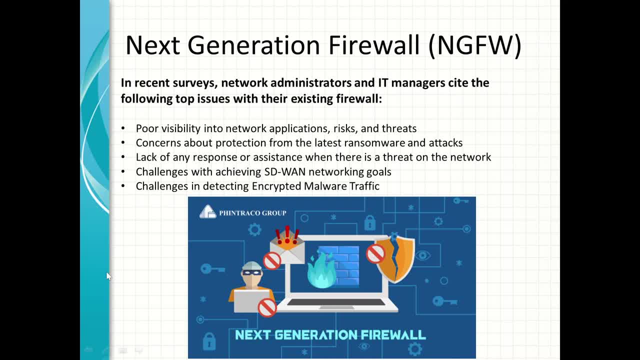 coming after masquerading, then definitely it will come somewhere. sir, it can be done. it is not a matter of block. it will not be done by geofencing, it will be done by the rule set you will make. okay, so let us talk about next generation firewall up. these are some issues that are being observed. 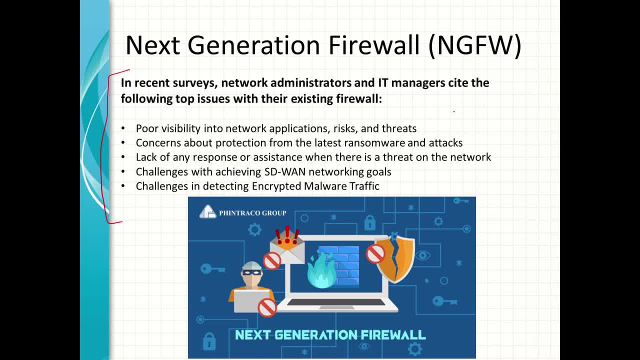 in the firewall, in the traditional firewall, so that are being catered in the next generation firewall. what are the issues? poor visibility into network application risk and threat. concerned about protection from latest ransomware and attacks. lack of any response or assistance when there is a threat on the network. 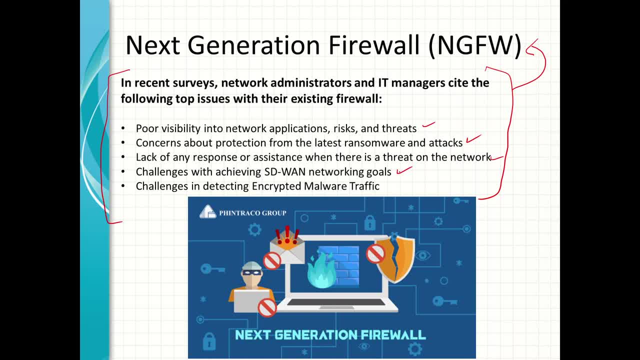 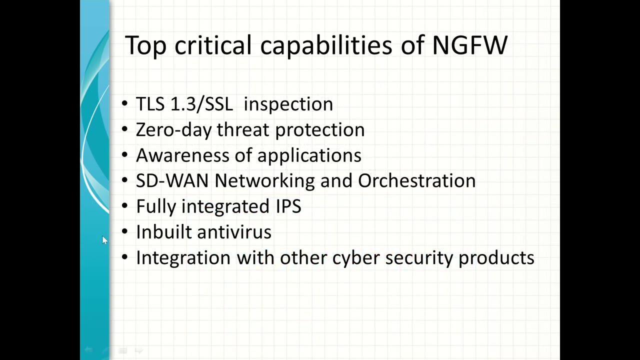 and challenges which are with achieving hd bank technology goals and challenging in detecting encrypted malware traffic. so this is the, i would say, the main usp of our next generation firewall. this is the main usb of a next generation firewall where the encrypted malware traffic is also scanned. okay, so let me uh talk on this, because this is a very important thing. now we have entered 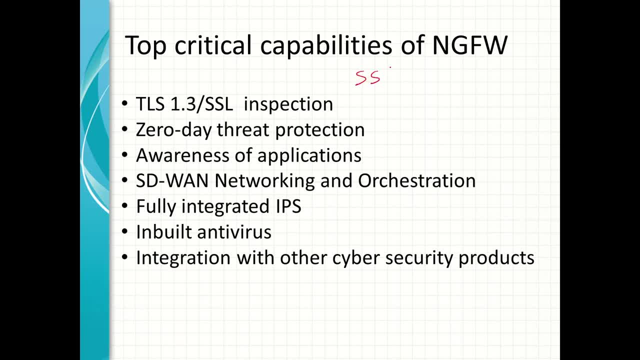 into the. we have started from where we started. we have started ssl and now we are on to the tls 1.3. what, what is this? these are the encryption layers. okay, these are the encryption tiles. so what are the top critical capabilities of ngfw? they can inspect. 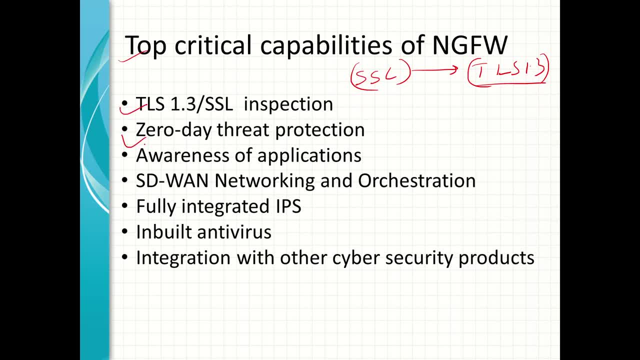 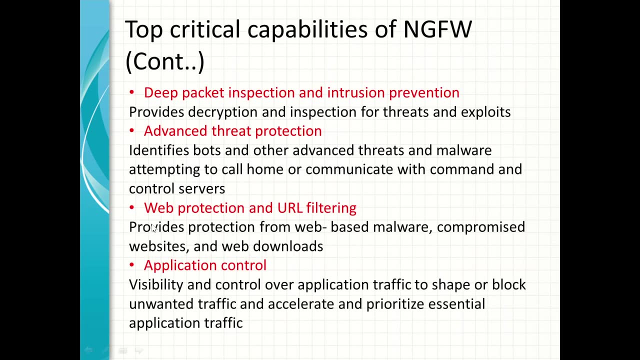 the packet, which is also encrypted. they can help you and zero their threat protection. they can help you in awareness of application hd when networking and orchestration. they have a fully integrated ips, inbuilt antivirus and integration with other cyber security products. okay, in continuation to this, uh, we have a deep packet inspection and intrusion prevention into. 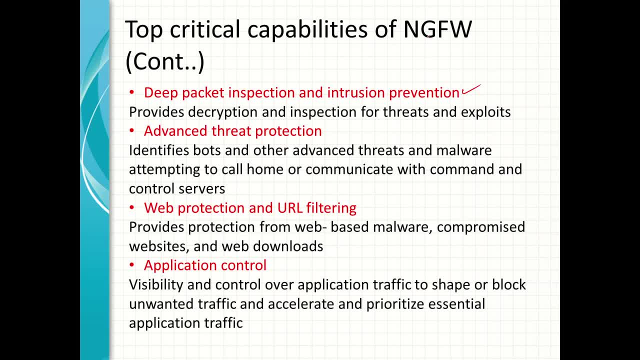 the next generation firewall. see, the normal firewall is talking on layer 2, layer 3 and layer 4.. in layer 2 we have a mac, in layer 2, in layer 3, we have ip and in layer 4 we have a port. okay, so most of the firewalls are in. traditional firewalls are just, uh, taking care of from l1 to 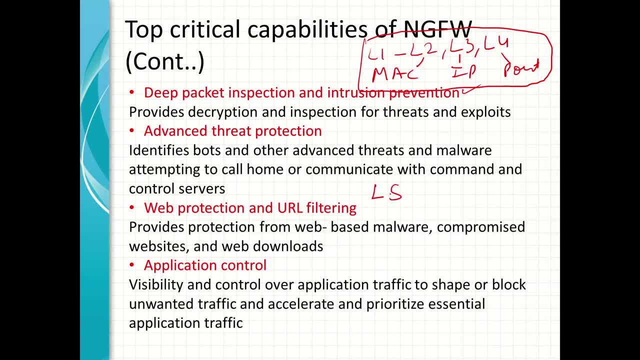 l4, but the upper layer fire. upper layers from l5 to l7- that is, a trans transport application and presentation layer- are also covered in the um in the next generation firewalls, okay. so deep packet inspection will help you to find out the malwares in layer 5, 6 and 7, also advanced threat protection. 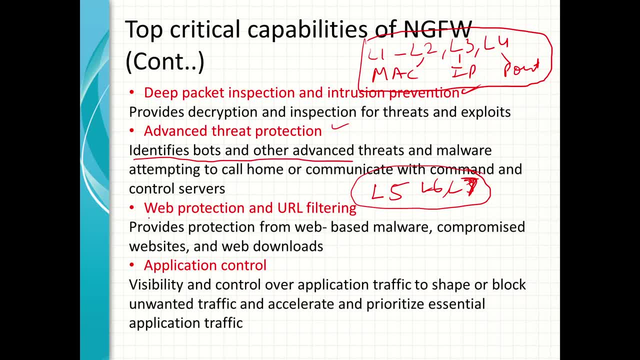 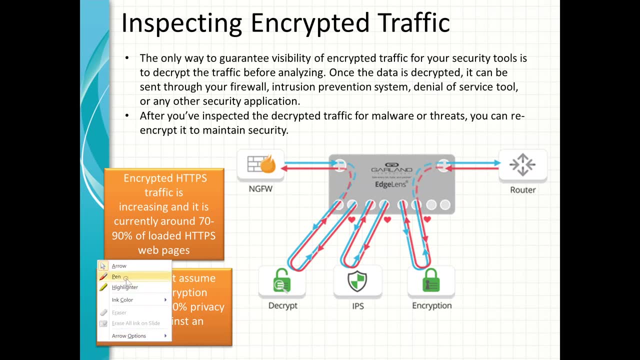 it can identify bots and advanced threats, web protection and url filtering. they have a good request and performance. website and web download can be blocked. then they have a better visibility over the application control. okay, now, this is very important and i think how many people know about this thing- that encrypted traffic is also being inspected these days? how many people know this? 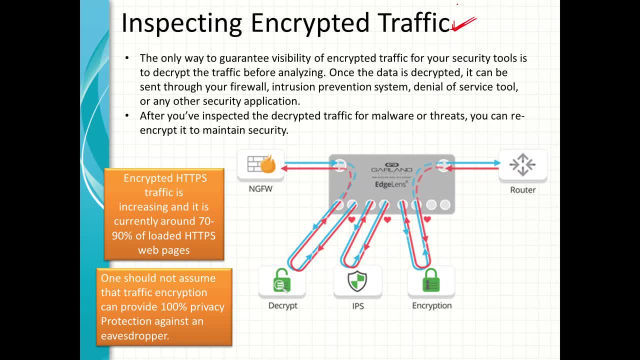 tell me. what about others, if you want to say something, please. Okay, so now the thing is that, after the evolution of TLS 1.3 and even TLS 1.1, 1.2, the encrypted traffic is also being inspected by the firewall. as you can see, this is a next generation firewall. 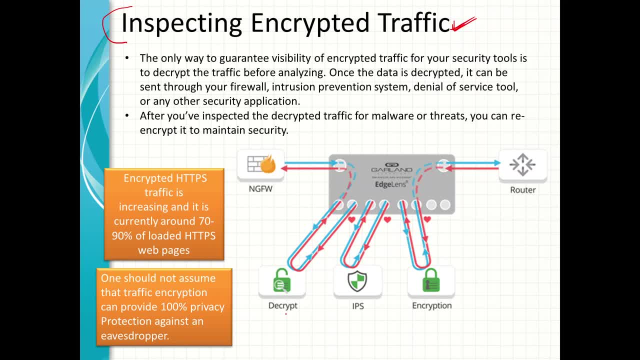 and in this next generation firewall the packet is firstly decrypted. okay, the packet is firstly decrypted, then it is checked in the IPS, then it is again encrypted and then it is again sent back to the router. okay, so they have a capability to decrypt your packet. so if you are thinking 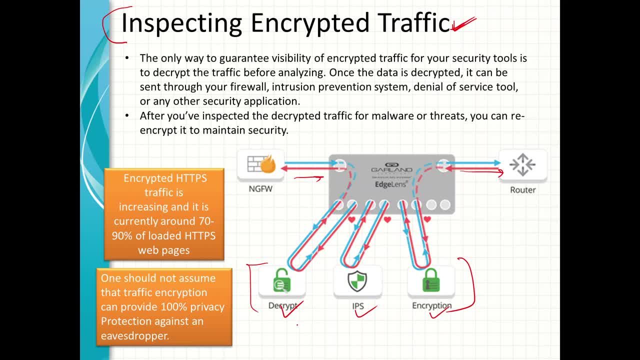 that your packet that you are sending from your home to your googlecom, so probably it is already being decrypted in the firewall in some- some of the ngfw firewall of your own, But usually they are. even the organization owners or network administrator do not have access to view the contents of the firewall because these firewall have a CA certificate. 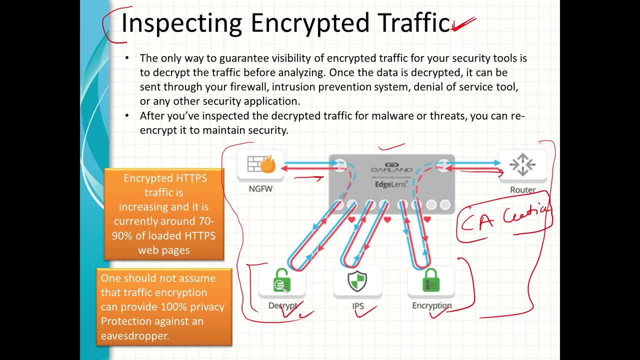 okay, certifying authorities certificate and these CA certificate ensure that this encryption and decryption is just for the scanning of the malicious traffic inside the packet. so what is exactly Is doing? the only way to guarantee visibility of encrypted traffic for a security tool is to decrypt the traffic before analyzing. once the data is decrypted, it can be sent through your firewall. 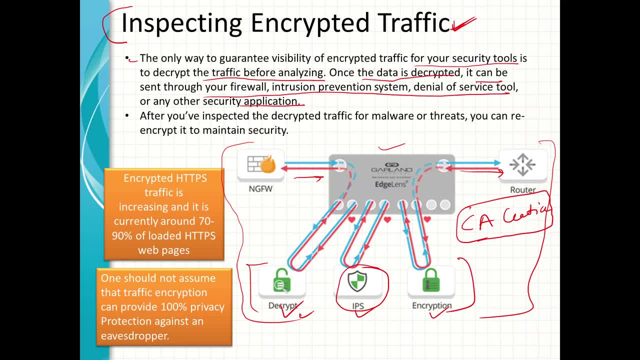 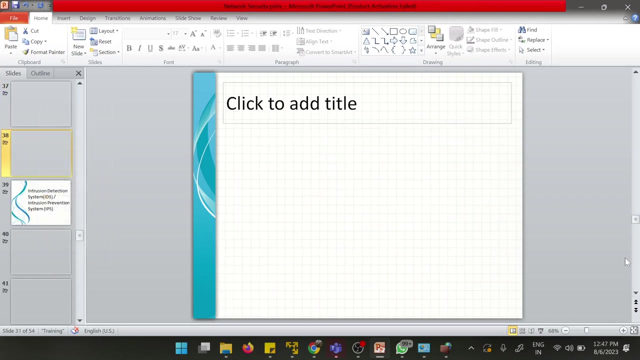 IDS denial of service tool or any other security application. after you have inspected the decrypted traffic for malware threats, you can re-encrypt it to maintain security. okay, so in this way, your traffic is also encrypted Now. now let me ask A simple question from you. 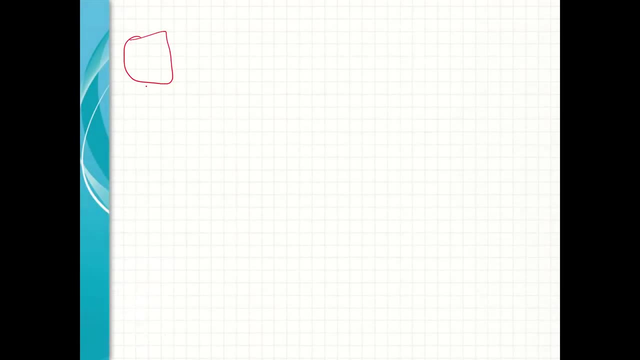 Okay, Okay, this is a PC of Mr A and he is accessing a server web server. okay, and this is a firewall in ngfw. is there? He has Tried to access a page of web server. he has received The web page user name and password. he just entered the user name and password and press the submit. 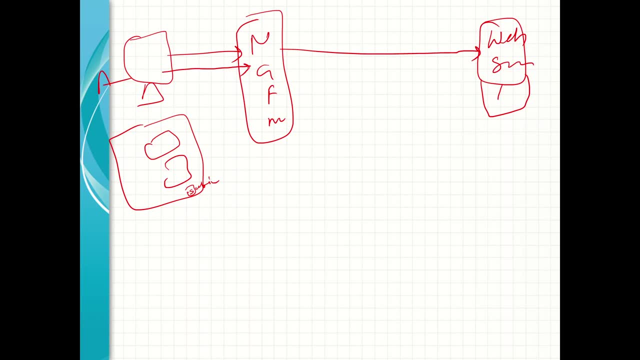 button now. thus, this submit button will bring that packet to the ngfw and that ngfw will open, check and then again close back and send to the web server. now tell me, is it hampering the integrity of a user? A When I when we have talked about the CA, CIA. 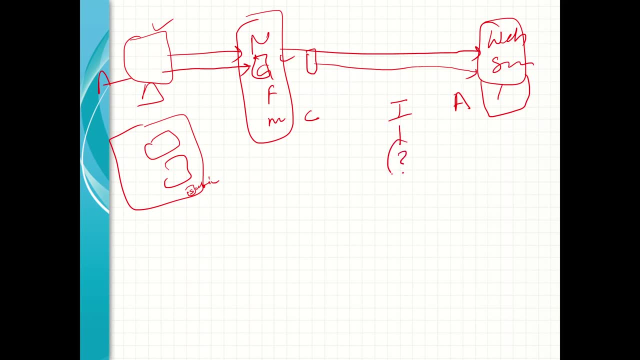 Now tell me: Integrity is hampered or not? Yes, sir, And confidentiality is hampered or not? Yes, sir, Definitely, confidentiality and integrity is hampered. so, and there is also a chance that if a CA certificate is expired, web server may be not replying back to this A because he find this communication as a malicious. it will treat this as malicious. 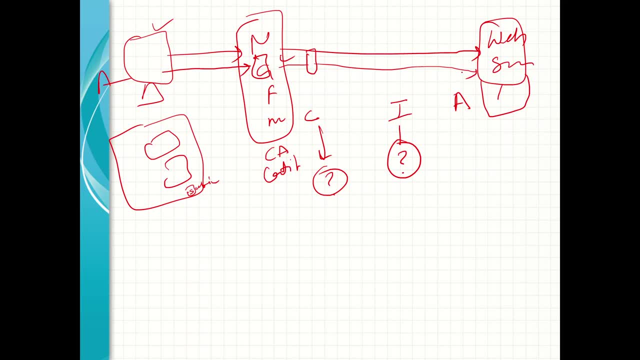 So A, A, A, A, A And the packet which is sent by a is open by someone else. But the thing is that when this packet is open in the ngfw is treated as a legitimate process because the c A. 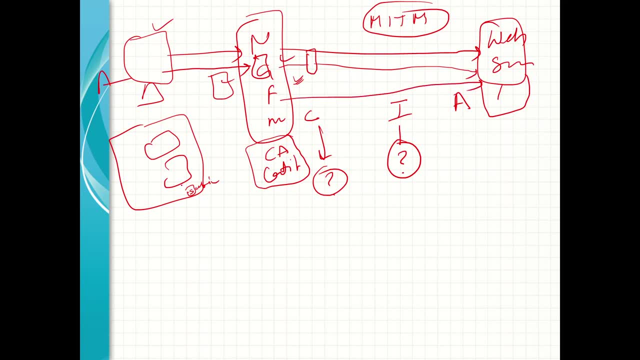 A, A. A Certificate is already evil and this is a threat ticket is also Share, Shareshared with this Web Server. This ngofw will add a c A. A received a packet from a, but we are the certifying agency to check the maliciousness, so we are. 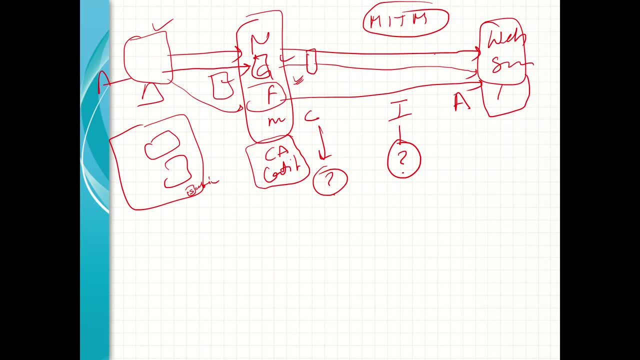 sending our certificate also to send you. someone has asked in around 10 minutes before that there they are showing an error. that isp issue is there. isp is not. service is not secure. who is there, sir? what's the good name? somebody has asked. so this probably the issue because the ca certificate is expired at their. 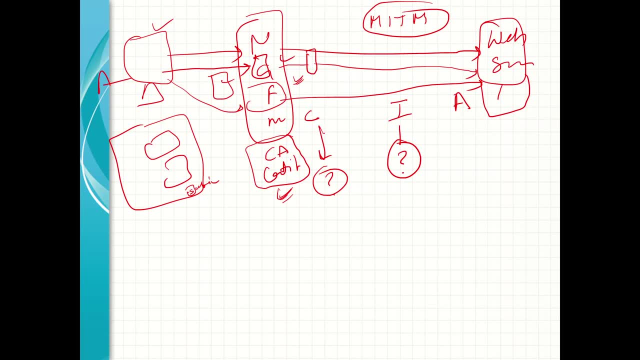 end. so you have you understand how the encrypted traffic is being analyzed, sir. i have a question here. so if it is encrypted and sent in wireless encrypted form, then in the other end receiving and say googlecom server, they should also have the ca certificate to decrypt, right? so you mean to say because there will be different vendors for this ngi? 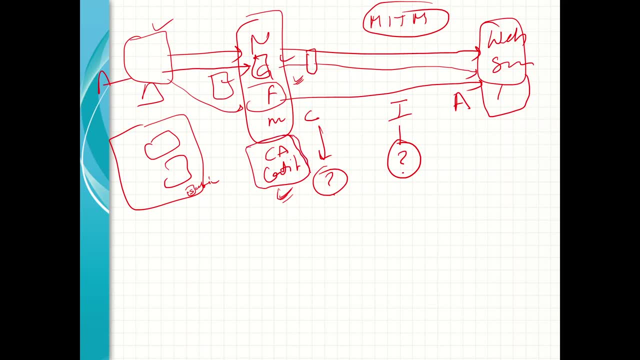 ngi from. but ca certificate is provided by the certification authority. okay, like verisign, verisign is a company who is sharing certificate. ca certificate is certifying authority certificate. is it shared with the? okay, is it shared with the other end also? because, yeah, they are shared, otherwise how would you ensure the proper? 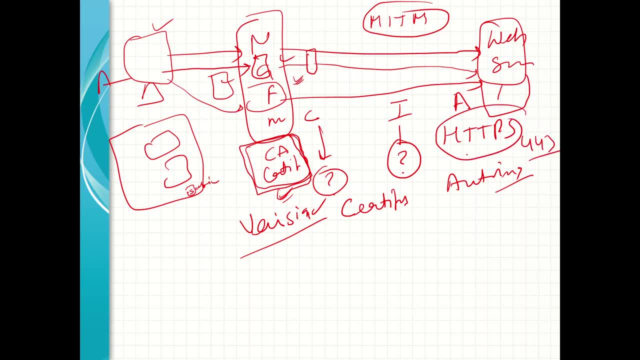 https communication over a 443. it is not possible if you are not sharing the certificate, as you, as you told earlier during communication. uh, symmetry. for this, encryption and decryption keys are exchanged. yes, so when firework opens one and uh decrypted and again encrypted to ensure its uh. 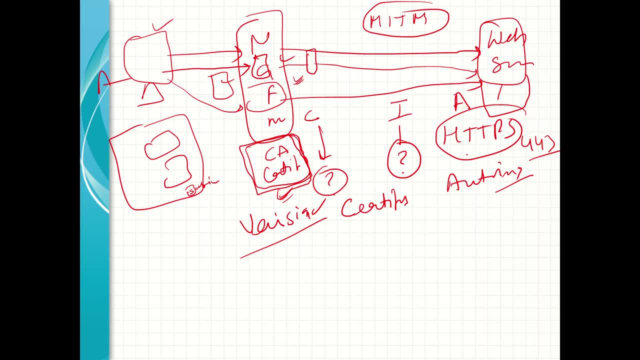 genininess and authenticity. they they use the same key or different keys, or also the same key. they are not using different keys, or also they use the same key or different keys, or also they are sharing with each other. so they are sharing, so they have to be careful. which those keys are in them is like when we are not using them. 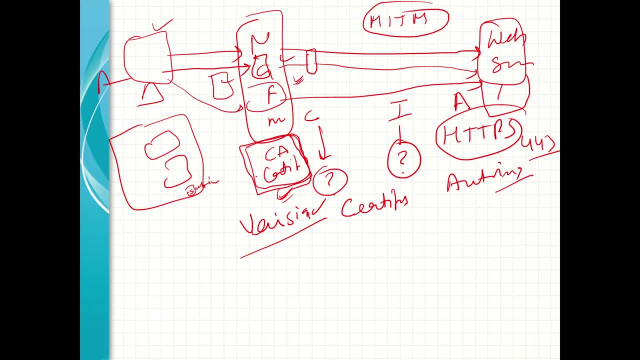 different keys or how the keys are exchanged. okay, okay, so let us suppose take this ca certificate as a key only. okay, this is a key only. let me tell you, with a small example, that this is a client and this is a server, and on the client end we have a ng of w. okay, so in initial communication, 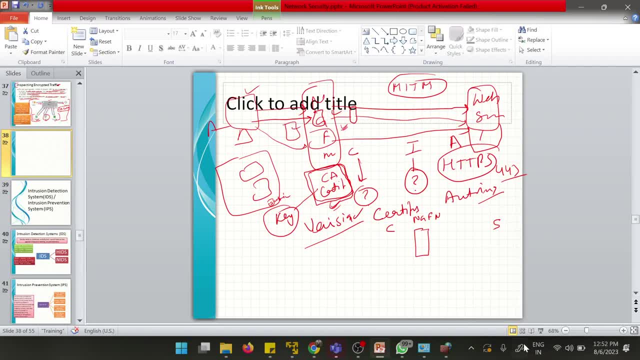 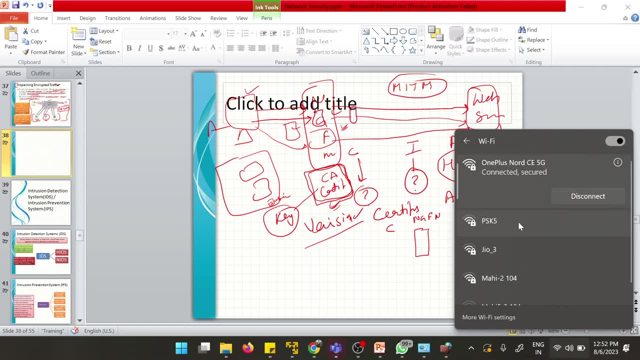 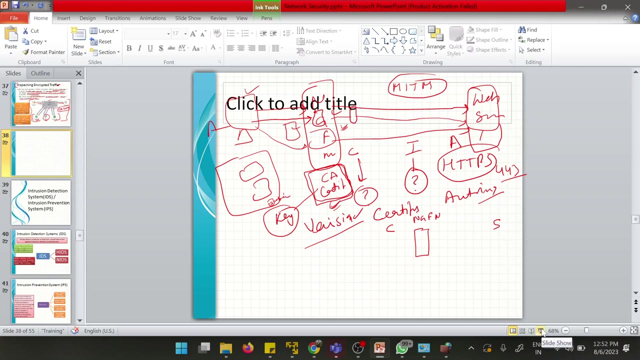 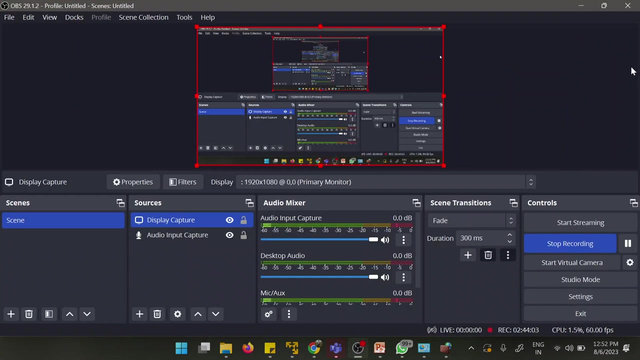 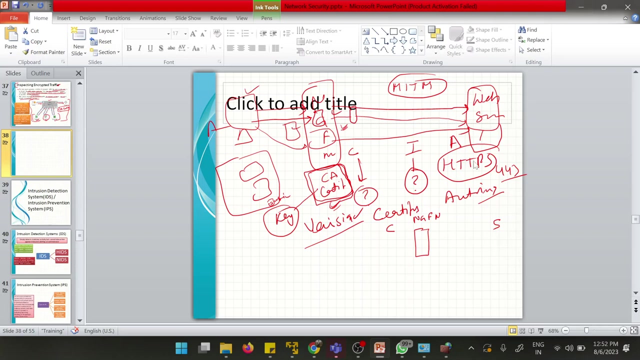 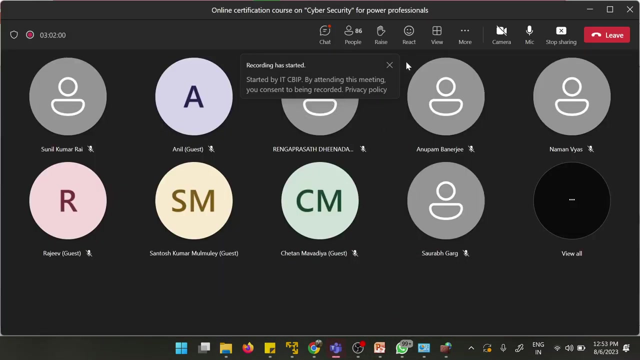 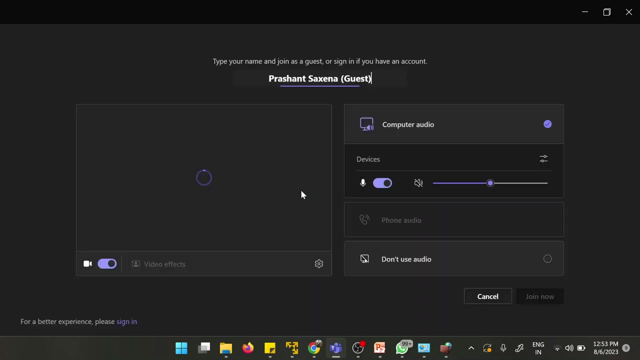 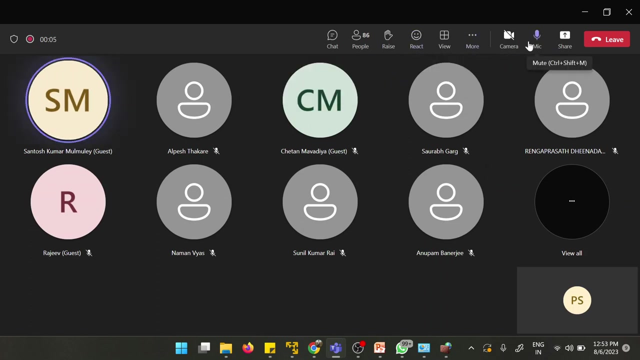 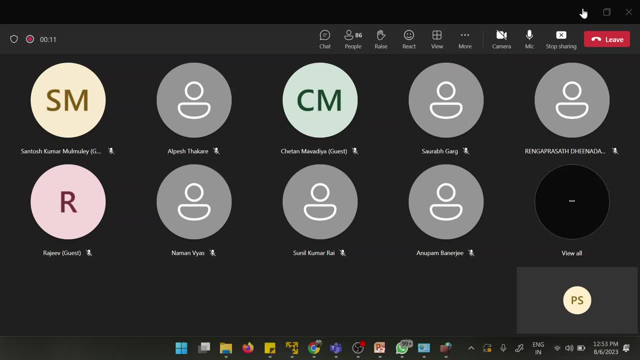 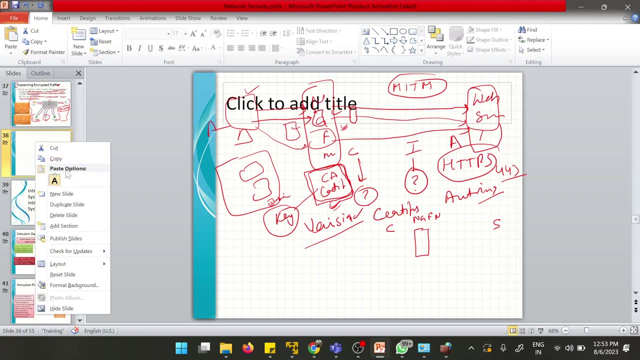 yeah, sorry, sorry for the. yeah sorry, sorry for the interruption. actually there is a power cut in my interruption. actually there is a power cut in my interruption. actually there is a power cut in my area, area area. so i'm putting on ups, that's why. okay, now it's perfectly. 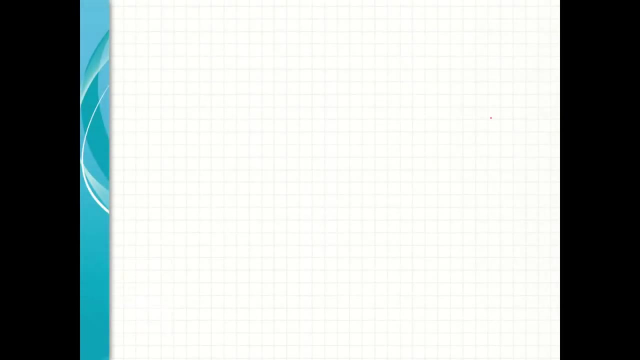 okay, now it's perfectly okay, now it's perfectly yeah, yeah, yeah, okay, okay, let us talk on this. okay okay, let us talk on this. okay okay, let us talk on this. we have a client and we have a server. we have a client and we have a server. 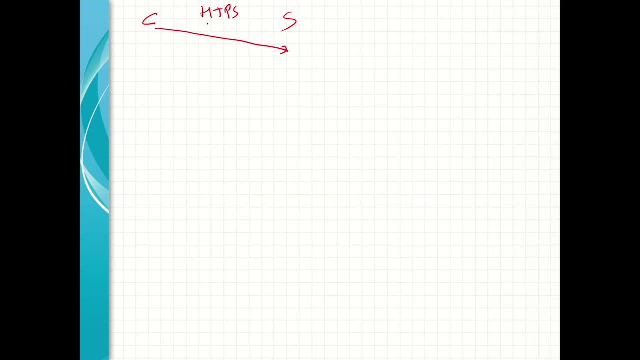 we have a client and we have a server to establish a https communication. to establish a https communication. to establish a https communication, we have to send a syn packet. we have to send a syn packet, we have to send a syn packet. then we have the client, the. 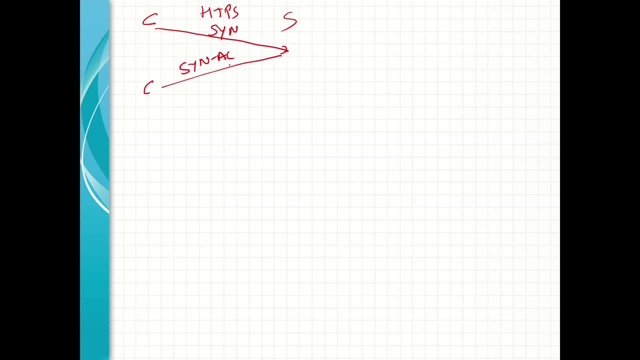 then we have the client, the, then we have the client. the server will send to server a syn server will send to server a syn server will send to server a syn packet, packet, packet, and the client will again send the act and the client will again send the act. 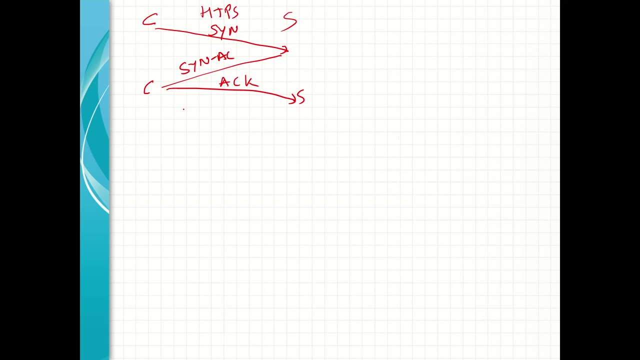 and the client will again send the act packet to confirm that packet, to confirm that packet, to confirm that we have a connection done because this we have a connection done because this we have a connection done because this is a tcp communication and tcp is a is a tcp communication and tcp is a. 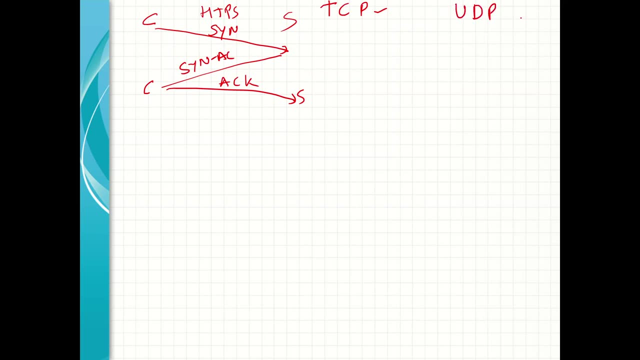 is a tcp communication and tcp is a connection oriented communication. connection oriented communication, connection oriented communication. this is not a udp communication. okay, udp. this is not a udp communication. okay, udp. this is not a udp communication. okay, udp is a connectionless protocol, is a connectionless protocol. 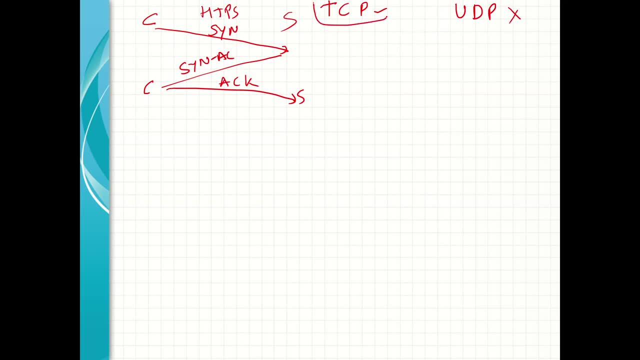 is a connectionless protocol. i think you have already studied about. i think you have already studied about. i think you have already studied about it. okay, we are focusing on tcp once the it. okay, we are focusing on tcp once the it. okay, we are focusing on tcp once the communication is established. 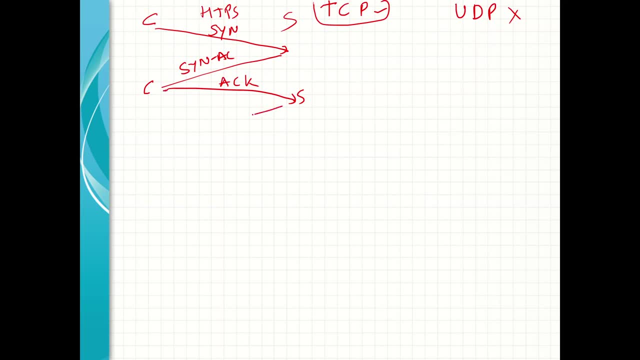 communication is established. communication is established. the server, the server, the server, during, during, during, will share. what type of encryption level will share? what type of encryption level will share? what type of encryption level? he is doing encryption level. he is doing encryption level. he is doing encryption level. let us suppose server is saying: i am. 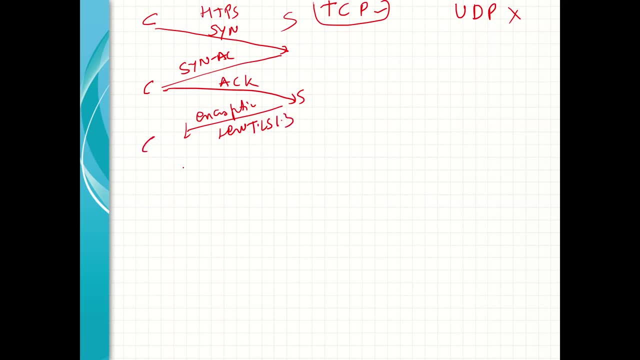 let us suppose server is saying i am. let us suppose server is saying i am using tls 1.3, using tls 1.3, using tls 1.3. okay, the client will receive the okay. the client will receive the okay. the client will receive the information that tls 1.3. 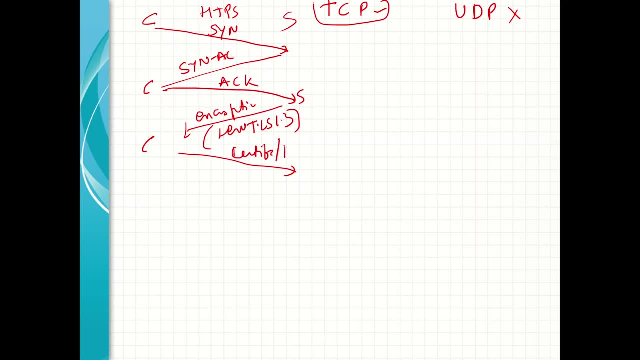 information that tls 1.3. information that tls 1.3. certificate: certificate, certificate. slash, key it one and the same thing. slash, key it one and the same thing. slash, key it one and the same thing. certificate and key to the server. certificate and key to the server. 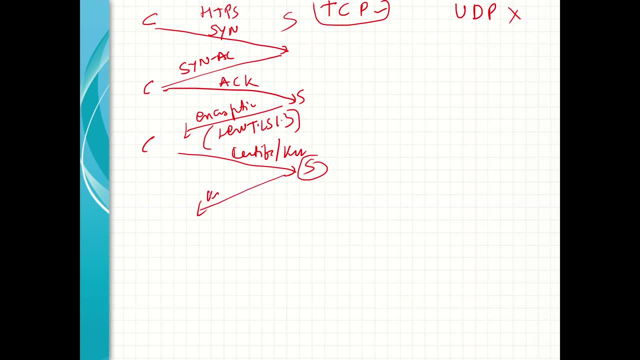 certificate and key to the server. okay, and the server will again send his okay, and the server will again send his okay, and the server will again send his key, key, key and certificate and certificate and certificate for communication. okay, these are the for communication. okay, these are the. 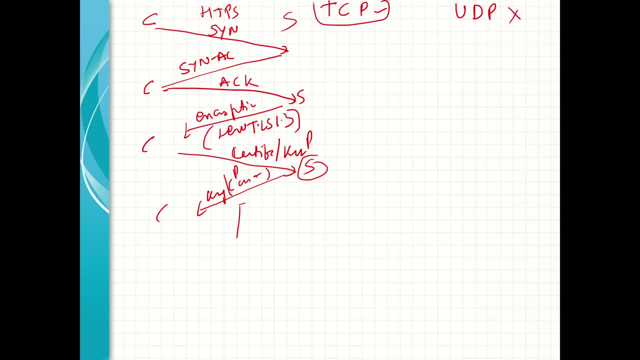 for communication. okay, these are the public keys, public keys, public keys. now, when the real com, now when the real com, now, when the real com, real transport of data will occur, this real transport of data will occur. this real transport of data will occur. this ng of the blue will came into the part. 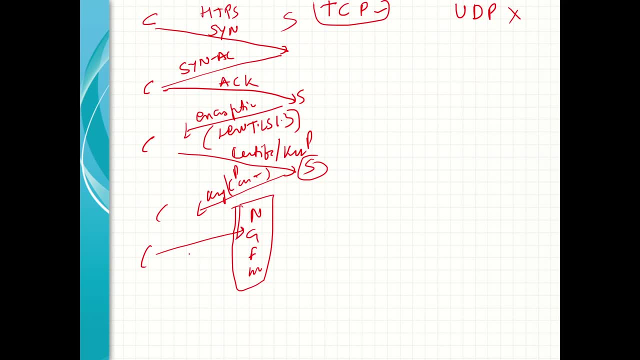 ng of the blue will came into the part. ng of the blue will came into the part and the client will send the data to ng and the client will send the data to ng and the client will send the data to ng of w and ng of w to data to the server. 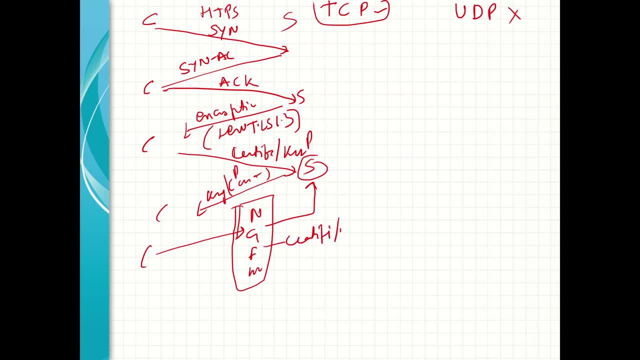 of w and ng of w to data to the server of w and ng of w to data to the server. but ng of w will also share his. but ng of w will also share his, but ng of w will also share his certificate, slash certificate, slash certificate, slash that. 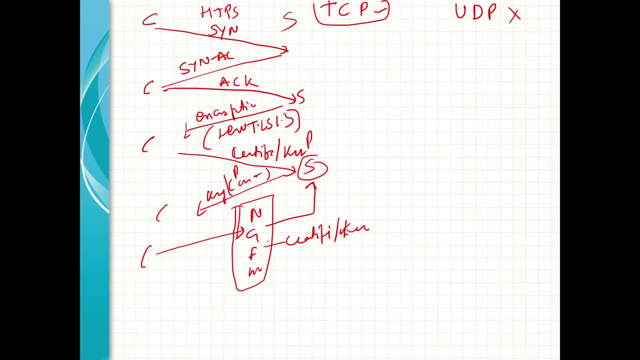 that that certificate slash key to the server, that i certificate slash key to the server, that i certificate slash key to the server, that i have decrypted, decrypted the data and again have decrypted, decrypted the data and again have decrypted, decrypted the data and again encrypted back and sending you the data. 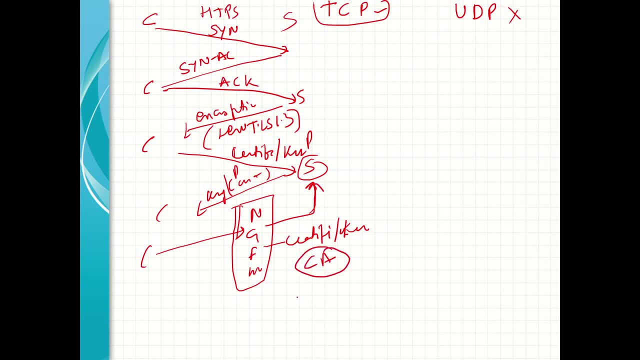 encrypted back and sending you the data encrypted back and sending you the data. so so, so, this ca certificate that is provided by this ca certificate, that is provided by this ca certificate that is provided by the very sign, very sign, and there are the very sign, very sign, and there are. 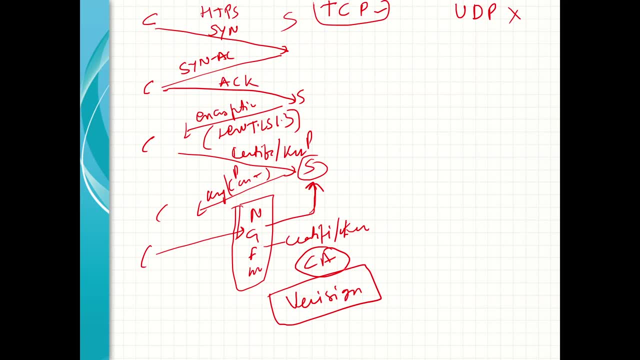 the very sign, very sign, and there are different, more companies, different, more companies, different, more companies uh which have assigned this uh duty to uh, which have assigned this uh duty to uh. which have assigned this uh duty to issue, they can issue the ca certificate issue. they can issue the ca certificate. 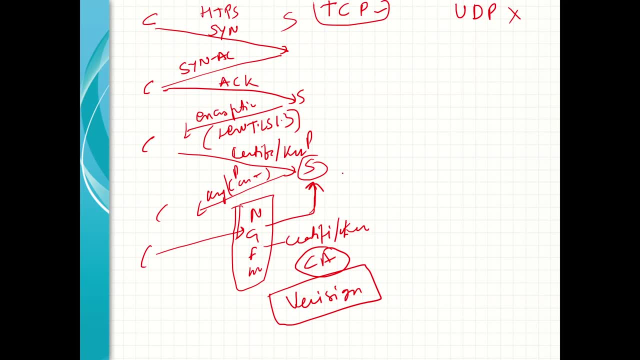 issue. they can issue the ca certificate. so this ca certificate is shared with. so this ca certificate is shared with. so this ca certificate is shared with that server, and then server will take that server, and then server will take that server and then server will take this uh. 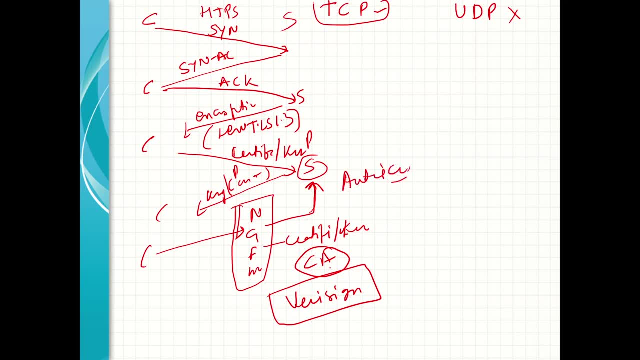 this uh. this uh: transfer of data as authenticated. transfer of data as authenticated. transfer of data as authenticated in case this ca certificate is expired, in case this ca certificate is expired, in case this ca certificate is expired, then your communication will not being. then your communication will not being. 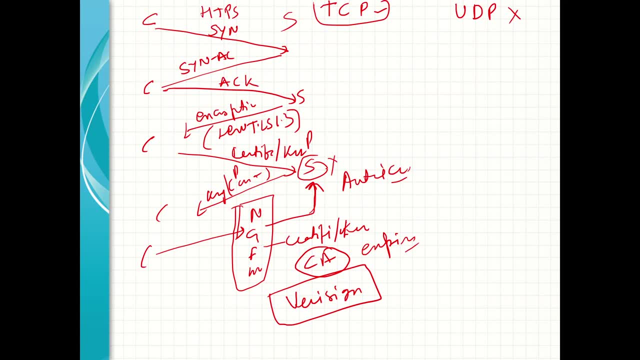 then your communication will not being established by the established by the established by the server end, because it will think that server end, because it will think that server end, because it will think that this is a mitm attack and this is a mitm attack and this is a mitm attack and it will not allow inside his environment. 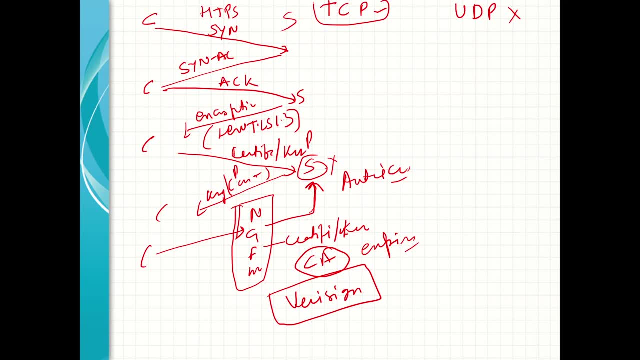 it will not allow inside his environment. it will not allow inside his environment. is it fine? is it fine? is it fine, okay, sir? thank you, okay, sir. thank you okay, sir. thank you okay. let's move on if the data is double. okay, let's move on if the data is double. 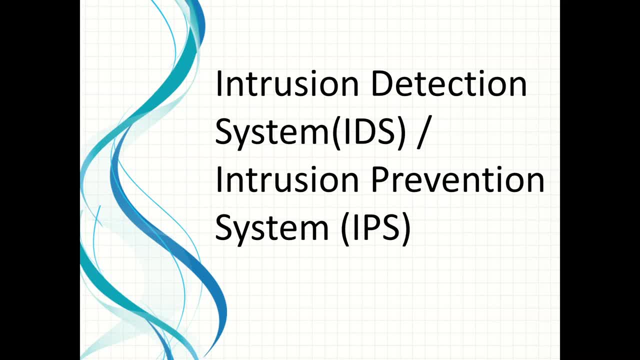 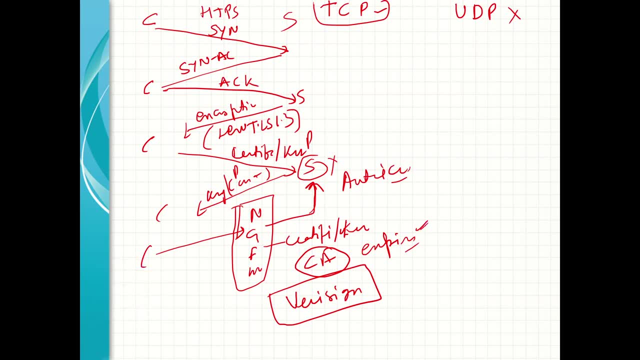 okay, let's move on. if the data is double encrypted, then how will it detect? encrypted, then how will it detect encrypted, then how will it detect, sir, because, sir, because, sir, because, because, when, the, because, when, the, when, the meaning is key, meaning is key, meaning is key. if malware is double encrypted, then 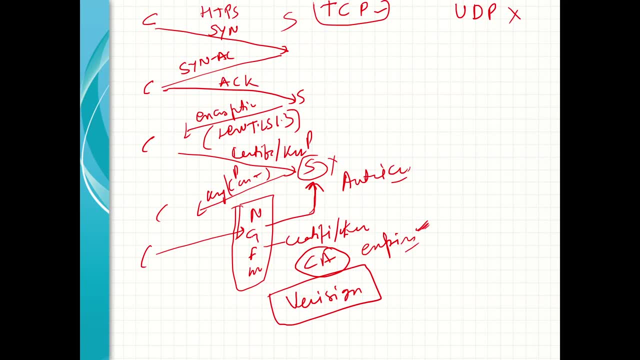 if malware is double encrypted, then if malware is double encrypted, then how will the ngf blue or the? how will the ngf blue or the? how will the ngf blue or the server side will detect? server side will detect, server side will detect. they have a capabilities inside, sir we. 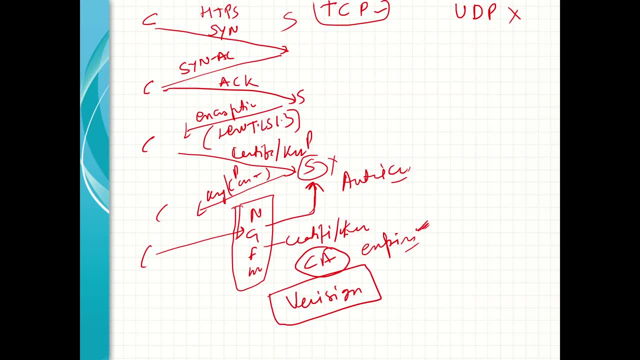 they have a capabilities inside, sir, we. they have a capabilities inside, sir. we cannot talk on that, cannot talk on that, cannot talk on that. they have capabilities. again, the all thing depend on that. my again, the all thing depend on that. my again, the all thing depend on that. my very first light titanium box. 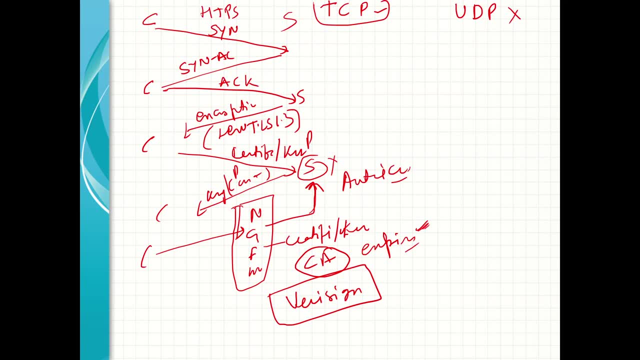 very first light titanium box. very first light titanium box. so there is always a vulnerability in so. there is always a vulnerability in so there is always a vulnerability in system, sir, system, sir, system, sir. okay, so this is about firewall, can we? okay, so this is about firewall, can we? 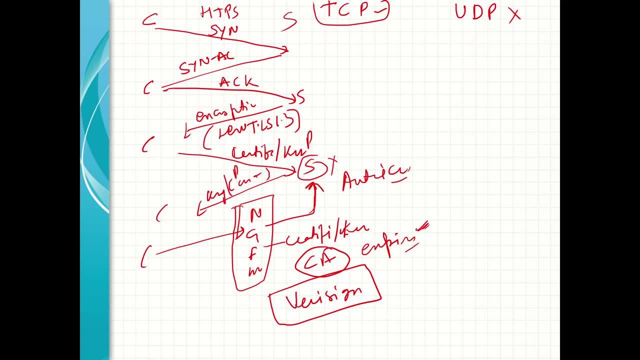 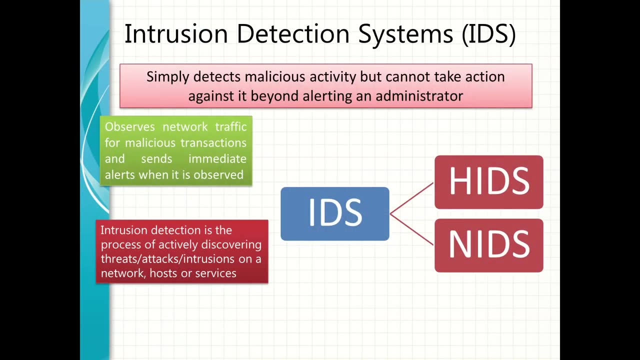 okay, so this is about firewall. can we move ahead now? yes, okay, so let's talk about ids and ips. yes, okay, so let's talk about ids and ips. yes, okay, so let's talk about ids and ips. so, what the ids is, i think you have. so, what the ids is, i think you have. 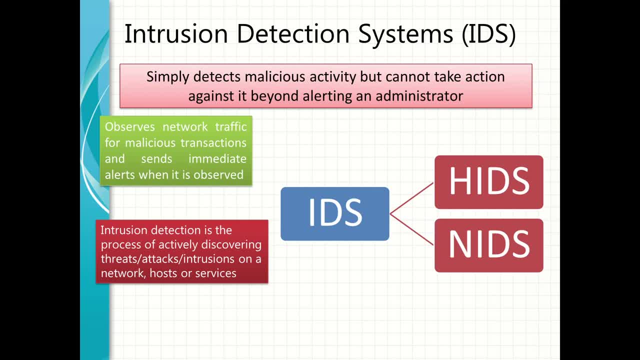 so what the ids is? i think you have already studied uh in yesterday's class. already studied uh in yesterday's class. already studied uh in yesterday's class. simply detect malicious activity. simply detect malicious activity. simply detect malicious activity, but cannot take action against again it. but cannot take action against again it. 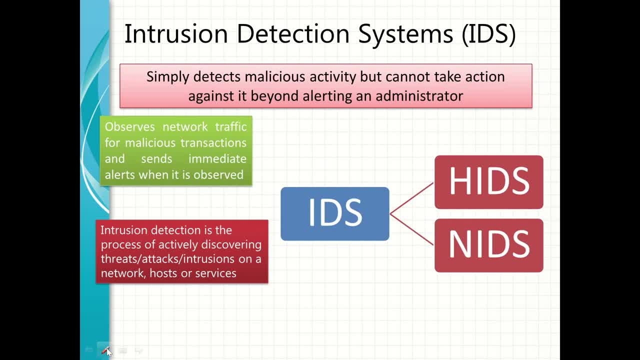 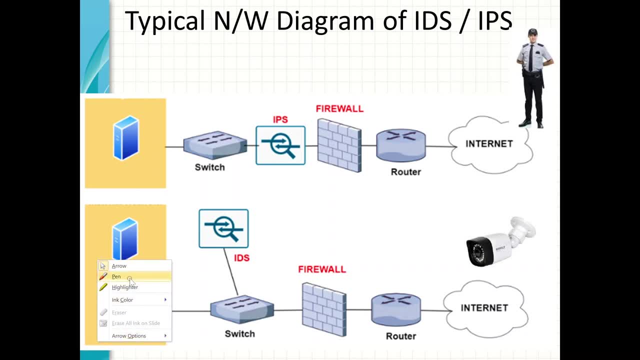 but cannot take action against. again it beyond alerting an administrator, beyond alerting an administrator, beyond alerting an administrator, so ids, so ids, so ids, so, so ids. so this slide is more clear to you. this slide is more clear to you. this slide is more clear to you. is the slide visible? 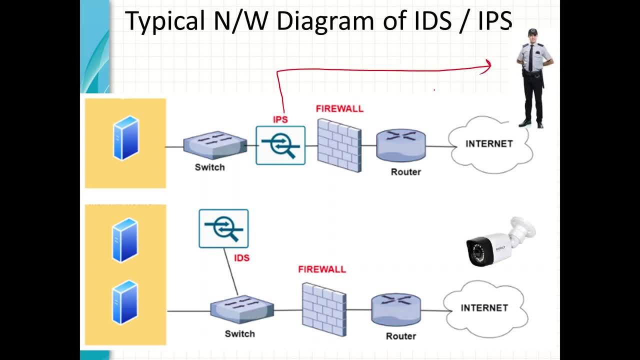 is the slide visible? is the slide visible? okay, yes, sir, okay, yes, sir, okay, yes, sir. always relate an ips with a guard and ids always relate an ips with a guard and ids always relate an ips with a guard and ids with the cctv camera, with the cctv camera. 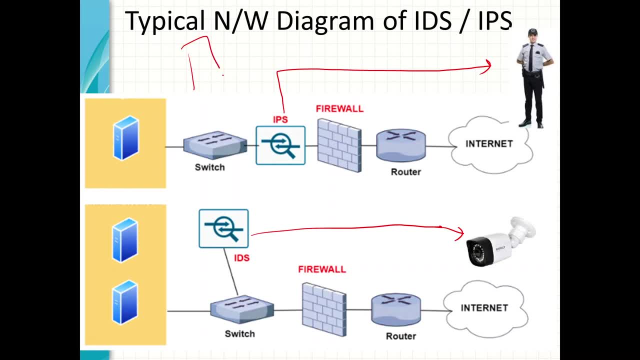 with the cctv camera. how, how, how? just think of a scenario. there is a just think of a scenario. there is a just think of a scenario. there is a building and guard is sitting outside building and guard is sitting outside building and guard is sitting outside. if some person who is looking like a 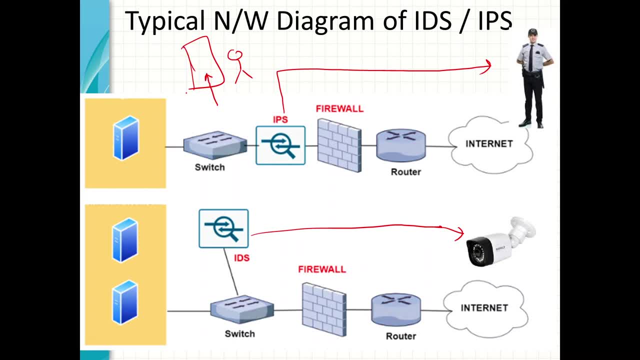 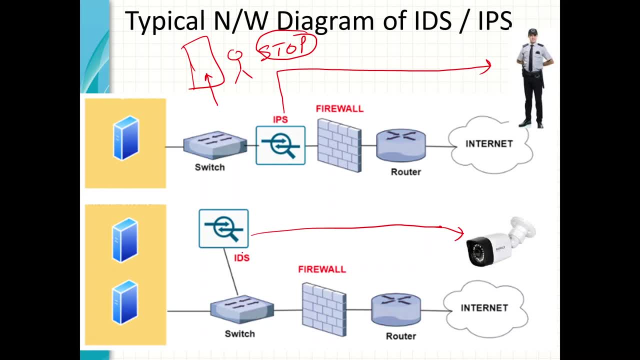 he will stop. he will stop, he will stop. okay. now think of a scenario where ids is okay. now think of a scenario where ids is okay. now think of a scenario where ids is there like a cctv in the building. you there like a cctv in the building, you. 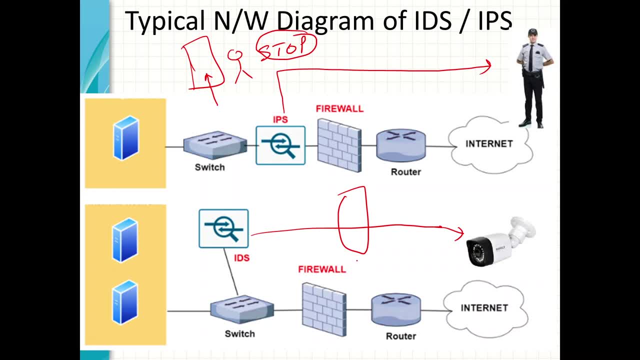 there, like a cctv in the building. you have a cctv, have a cctv, have a cctv and at night two some thieves are and at night two some thieves are and at night two some thieves are entering inside, entering inside. entering inside can cctv will do anything. 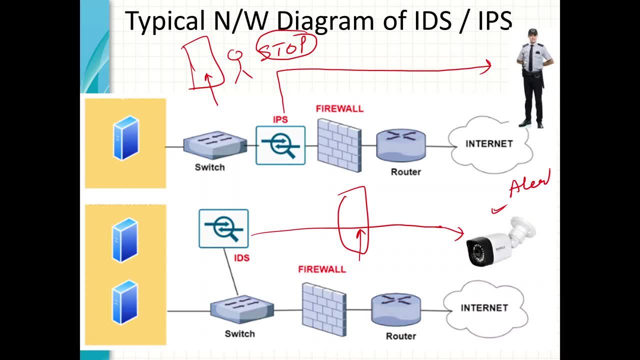 can cctv will do anything. can cctv will do anything: detect? it will create an alert, but it can't do. it will create an alert, but it can't do. it will create an alert, but it can't do anything at his own. and it is your luck that you are able to. 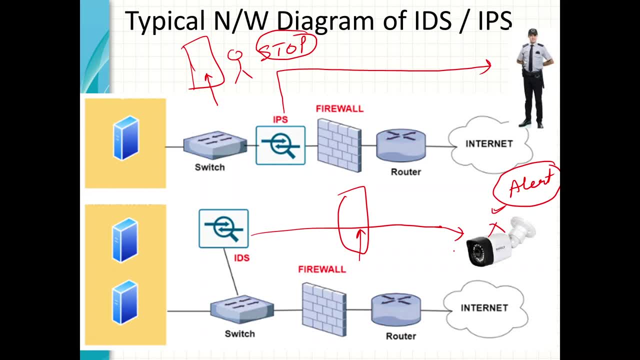 and it is your luck that you are able to, and it is your luck that you are able to see that alert or not, understood, understood, understood, yes, sir, yes, yes, yes, sir, yes, yes, yes, sir, yes, yes. this is a very simple analogy that i. this is a very simple analogy that i. 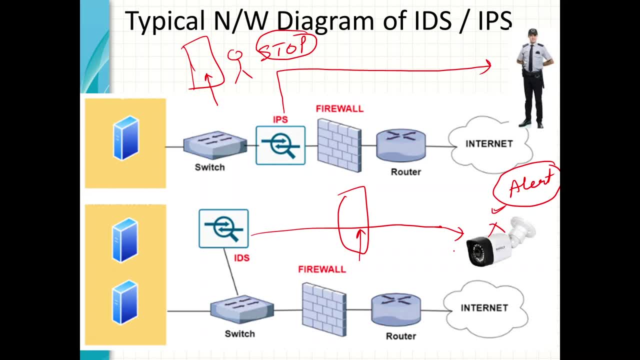 this is a very simple analogy that i have developed, have developed, have developed that ips is a, that ips is a, that ips is a security guard and ids is a security guard. and ids is a security guard and ids is a cctv camera. you have created and deployed an ids in. 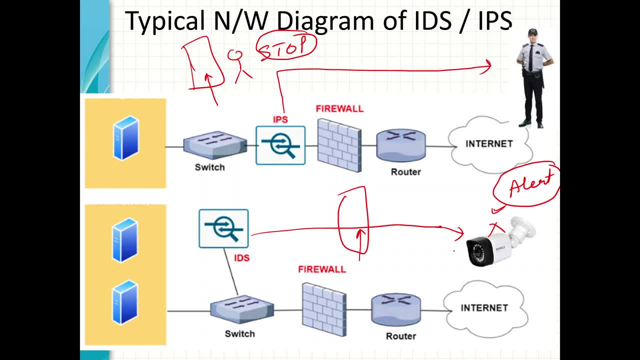 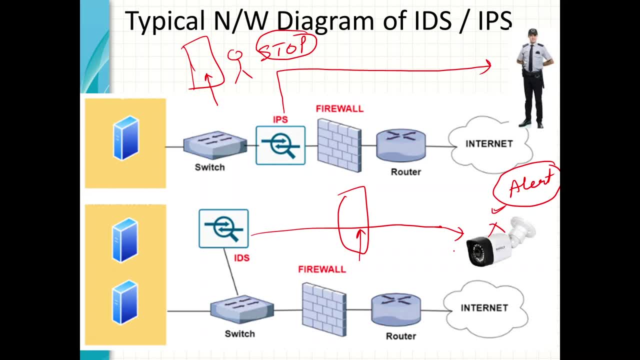 console, then do you think it is of any console, then do you think it is of any meaning? tell me, okay, so this is a basic that happened. okay, so this is a basic that happened. okay, so this is a basic that happened with, with, with. yeah, after theft happened, we can uh. 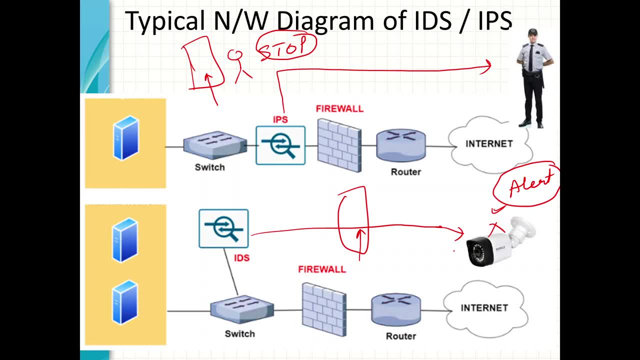 after theft happened. we can uh after theft happened, we can uh take the alert and uh take the alert, and uh take the alert and uh, we can prevent for next time. definitely, we can prevent for next time. definitely, we can prevent for next time, definitely, definitely, it is. 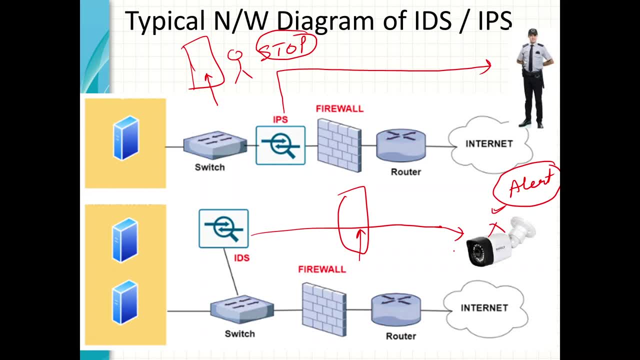 definitely, definitely, it is definitely, definitely, it is definitely. it is a mechanism to a mechanism, to a mechanism to protect, but at the time of moment. protect, but at the time of moment. protect, but at the time of moment. sometimes ids don't work properly, sometimes ids don't work properly. 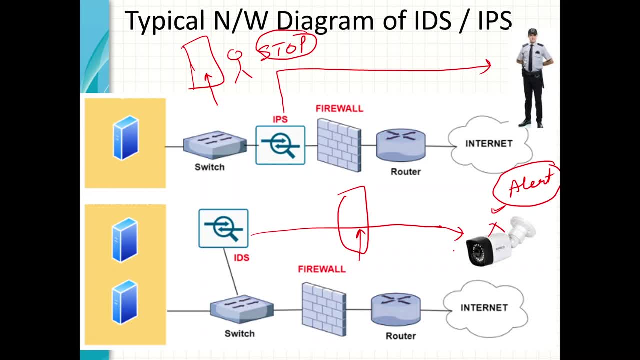 sometimes ids don't work properly. okay, okay, okay, okay. so this is a basic difference between: okay, so this is a basic difference between: okay, so this is a basic difference between ids and ips. i am not taking more of it. ids and ips. i am not taking more of it. 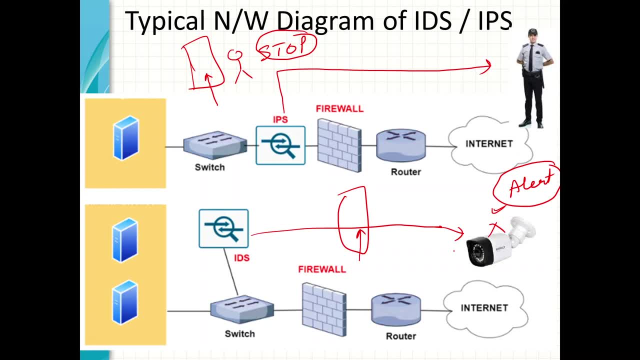 ids and ips. i am not taking more of it because you have already covered as you, because you have already covered as you, because you have already covered as you have told, have told, have told also, also, also. there is a very good ips ids that we. there is a very good ips ids that we. 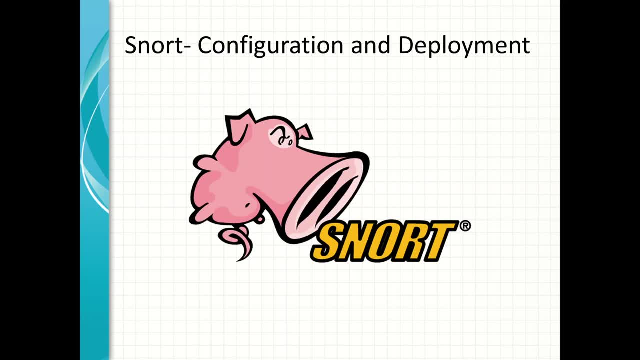 there is a very good ips ids that we call this as a snort. call this as a snort. call this as a snort. how many of you people know about snort? anybody know about snort? okay, yeah, it's not. is an ips ids combined? 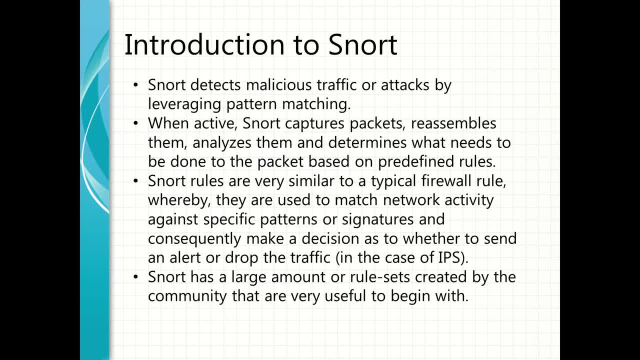 yeah, it's not. is an ips ids combined? yeah, it's not. is an ips ids combined and it's not? can and it's not. can and it's not. can- okay, so it's not. can detect malicious: okay, so it's not. can detect malicious: okay, so it's not. can detect malicious traffic or attacks by leveraging pattern? 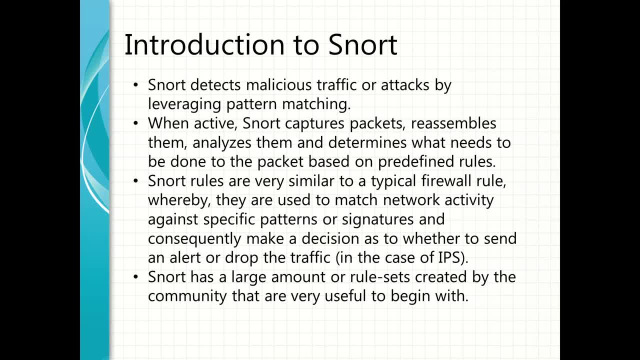 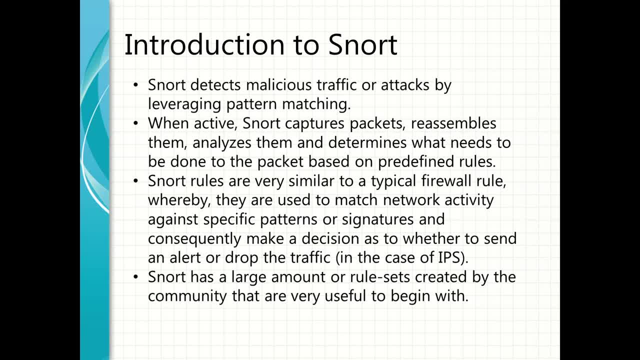 packet, reassembles them, analyze them and determines what need to be done to the. determines what need to be done to the. determines what need to be done to the packet based on predefined rule. packet based on predefined rule. packet based on predefined rule. it's not. rules are very similar to a. 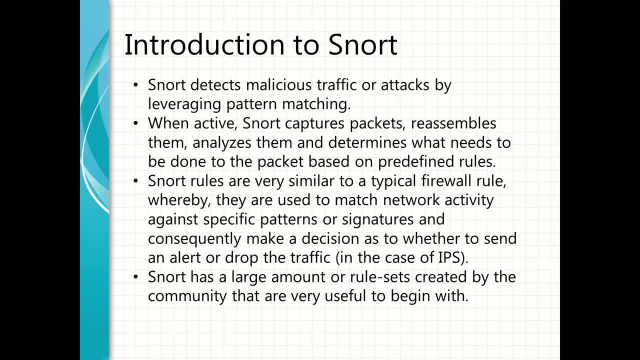 it's not rules are very similar to a it's not rules are very similar to a typical firewall rule, whereby they are typical firewall rule, whereby they are typical firewall rule, whereby they are used to match network activity against used to match network activity against used to match network activity against specific patterns or signatures. 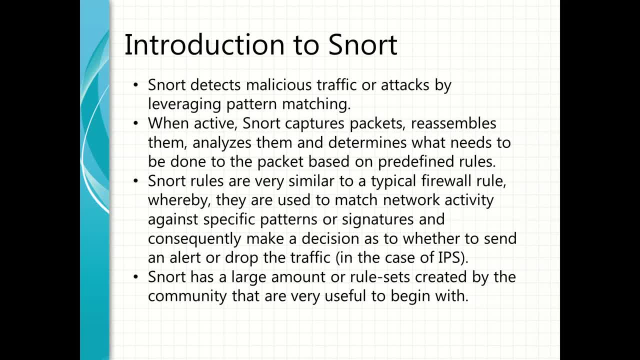 specific patterns or signatures. specific patterns or signatures: it's not has a large amount of rule set. it's not has a large amount of rule set. it's not has a large amount of rule set. created by which community that are very? created by which community that are very? 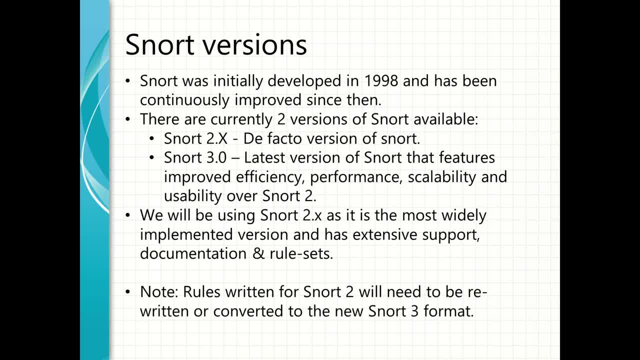 created by which community that are very useful to begin with ticket. it's not is useful to begin with ticket. it's not is useful to begin with ticket. it's not is basically having two versions. two point, basically having two versions. two point: basically having two versions. two point x and three point zero. but currently we 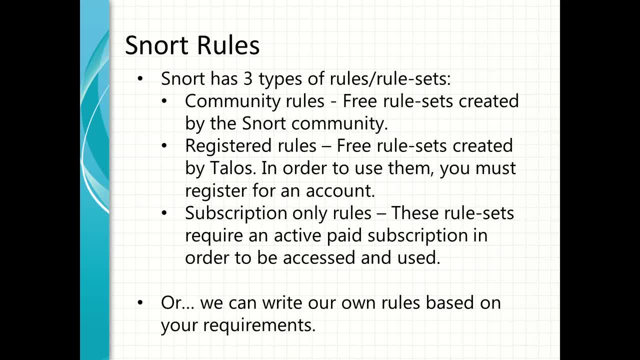 x and three point zero, but currently we x and three point zero, but currently we are using two point zero versions, are using two point zero versions, are using two point zero versions. okay, snort has three type of rules now. okay, snort has three type of rules now. 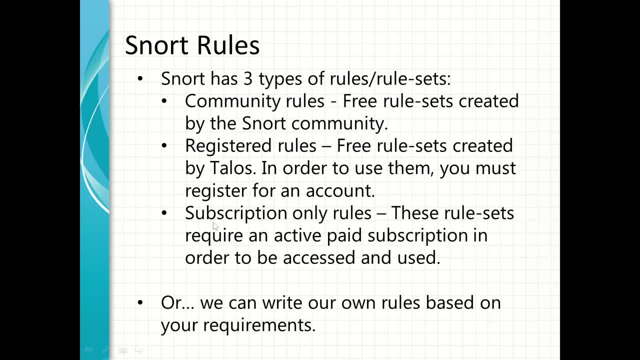 okay, snort has three type of rules. now, see, this is very important. see, this is very important. see, this is very important. this is very important. it's not has. this is very important. it's not has. this is very important, it's not. has basically, three type of rules. uh, what is? 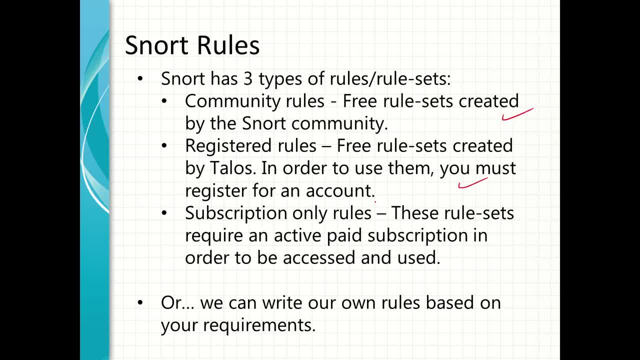 basically three type of rules. uh, what is basically three type of rules? uh, what is one is a community rules, then we have a one is a community rules, then we have a one is a community rules, then we have a registered rules, registered rules, registered rules, and then we have a subscription only. 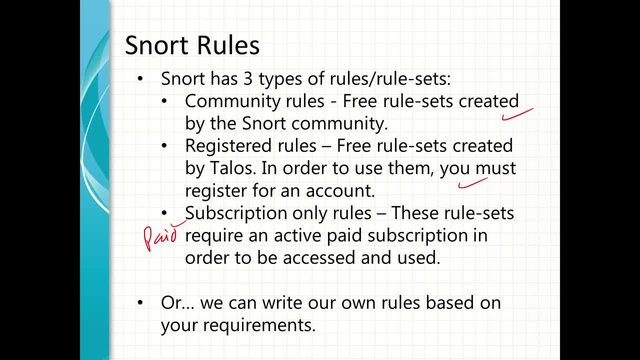 and then we have a subscription only, and then we have a subscription only rules okay. so these are the paid rules, rules okay. so these are the paid rules, rules okay. so these are the paid rules and these are the and these are the and these are the free rules. 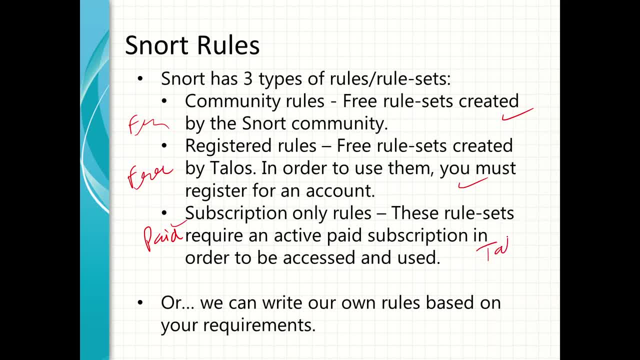 free rules, free rules: okay. telos is our organization. telos is okay. telos is our organization. telos is okay. telos is our organization. telos is our organization, which is very our organization, which is very our organization, which is very famous in security and famous in security and 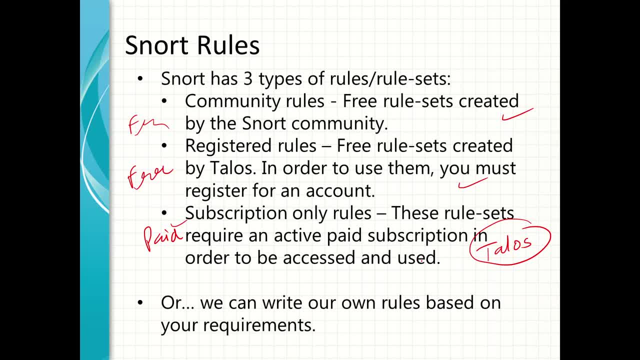 famous in security and they are providing rules for the safety. they are providing rules for the safety, they are providing rules for the safety and security of your organization and security of your organization and security of your organization, and also they have a community rules and and also they have a community rules and. 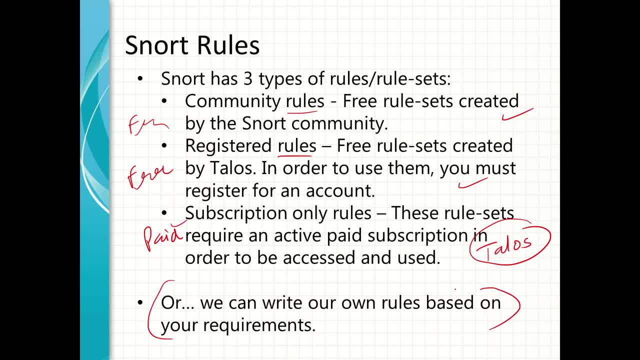 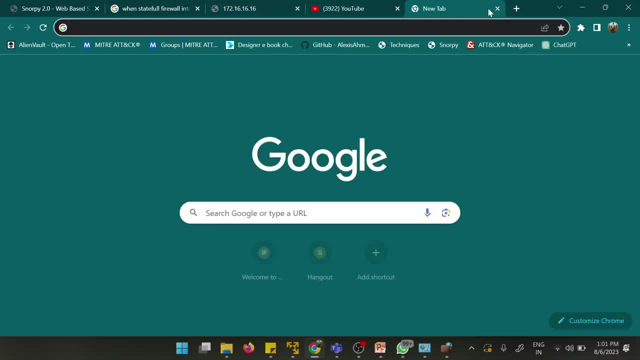 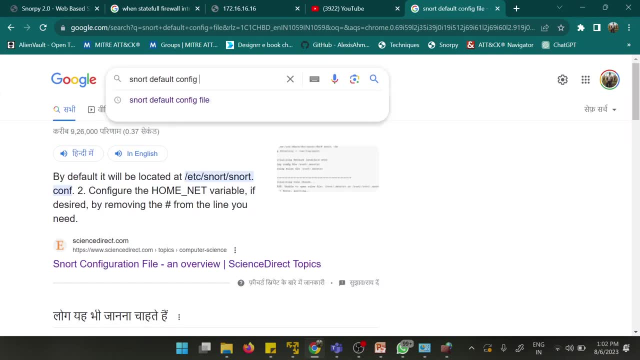 and also they have a community rules and register rules, register rules, register rules, and also we can write our own rules, so and also we can write our own rules, so, and also we can write our own rules. so let me, let me, let me tell you more about it. 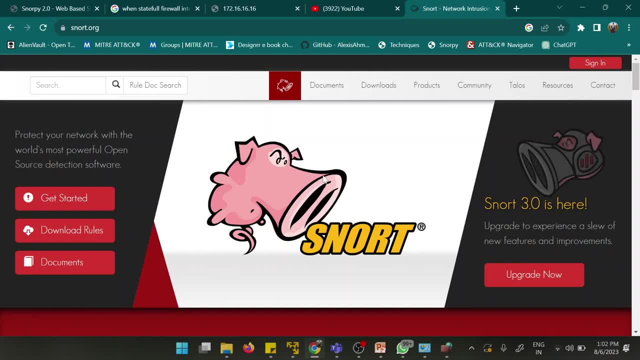 so this is a website of snort. so this is a website of snort. so this is a website of snort, snortorg, snortorg, snortorg, snortorg, and, and, and you can download snort from here. you can download snort from here. 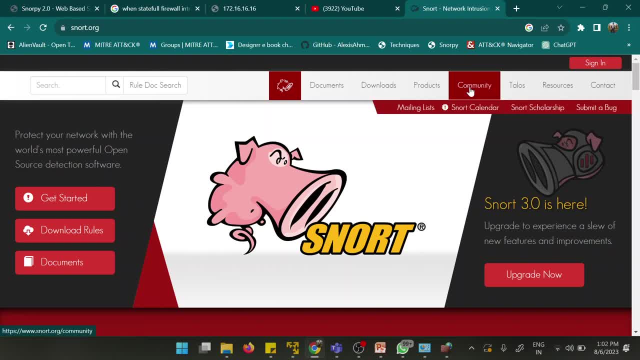 you can download snort from here, and the important thing that i want to, and the important thing that i want to, and the important thing that i want to share with you is share with you is share with you- is that is snort rules. that is snort rules. 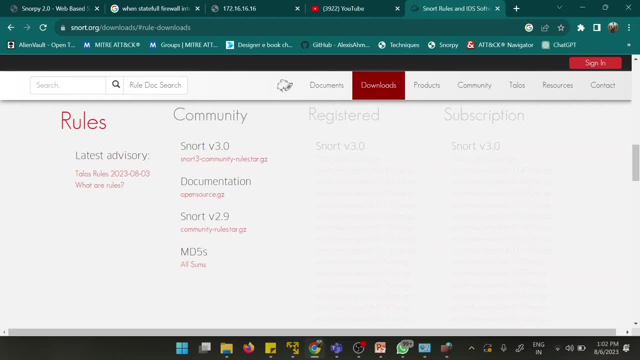 that is snort rules. okay, snort rules are very important. okay, snort rules are very important. okay, snort rules are very important. and one can and one can and one can download the community rules from here. download the community rules from here. download the community rules from here also. 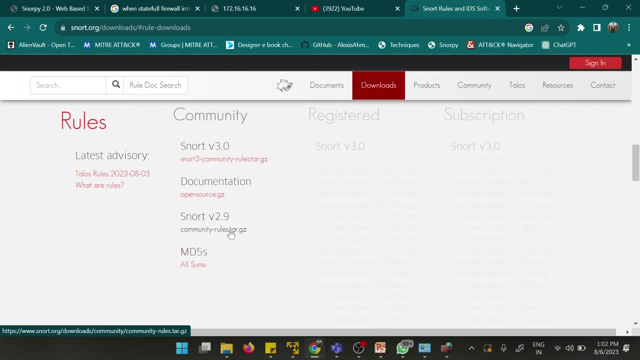 also also: okay, what are community rules? okay, what are community rules? okay, what are community rules? basically, lot of people, basically, lot of people, basically lot of people are working continuously to, are working continuously to, are working continuously to detect the attacks and detect the attacks and detect the attacks and extracting the signatures of that attack. 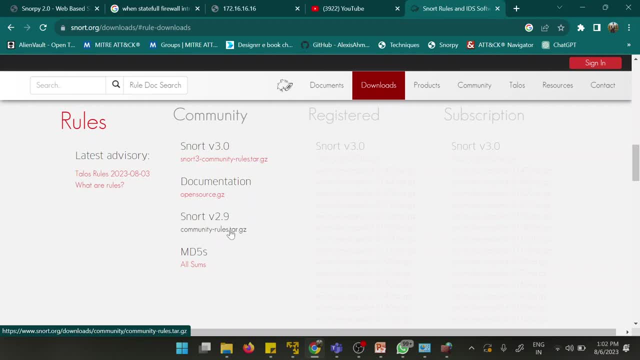 extracting the signatures of that attack, extracting the signatures of that attack and converting and converting and converting it into some rules so that these rules it into some rules, so that these rules it into some rules, so that these rules can be implemented into, can be implemented into, can be implemented into these not environments, so that they can. 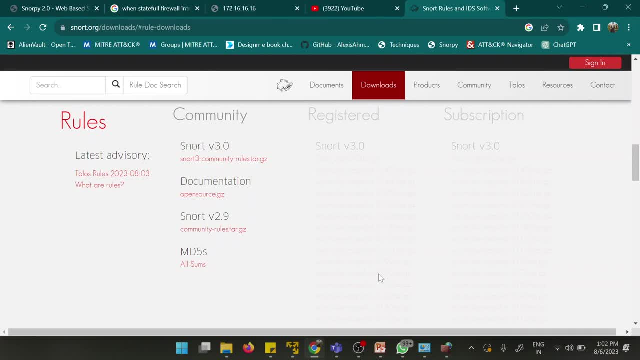 these, not environments so that they can. these not environments so that they can work okay, work okay, work okay. so it's not. is working on which, so it's not. is working on which. so it's not. is working on which environment, environment, environment. it's not is working on. 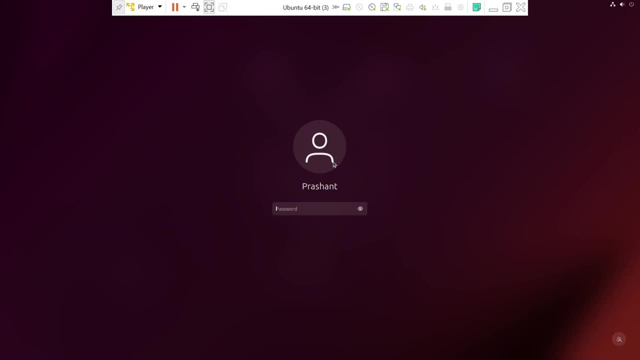 it's not is working on. it's not is working on linux, linux, linux, okay, okay, okay. so let me show you this, so let me show you this, so let me show you this: this is not an appliance. this is not an appliance. this is not an appliance. this is basically a software. 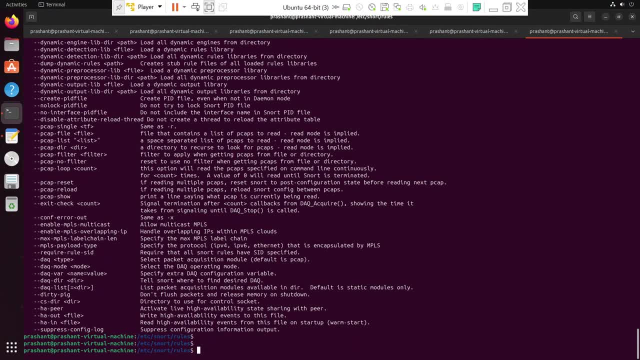 this is basically a software. this is basically a software appliance. it is a software you can appliance. it is a software you can appliance. it is a software you can deploy it on any anywhere. okay, so initially, uh, if you want to. okay, so initially, uh, if you want to. 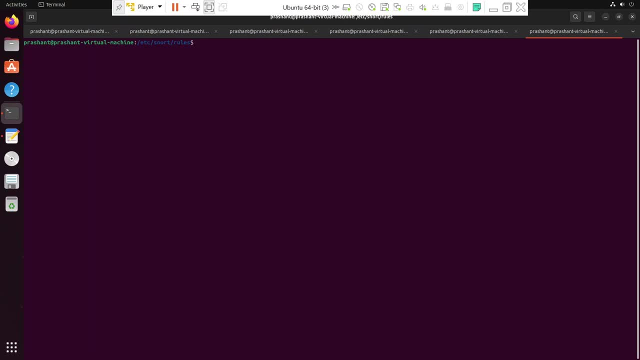 okay, so initially, uh, if you want to install this, not install this, not install this, not you can, you can. you can use a command: uh install. use a command: uh, install. use a command uh install. okay, okay, okay, apt, apt, apt, install, install, install. it's not okay, this is simple command. 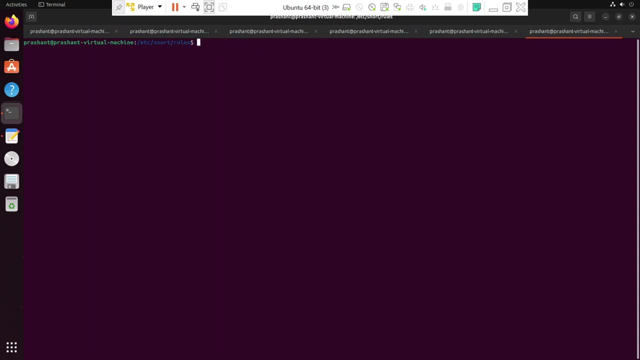 it's not okay. this is simple command. it's not okay. this is simple command: uh, through which you can uh, through which you can uh, through which you can uh uh, through which you can uh install your. now it is visible, i think so. is it visible now? 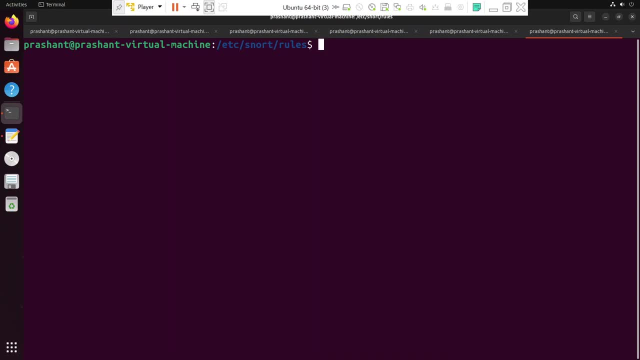 is it visible now? is it visible now? yes, sir, yeah, yeah, yes, yes, yes, so it's yes, sir, yeah, yeah, yes, yes, so it's yes, sir, yeah, yeah, yes, yes, so it's not. can be installed, uh, like i have not. can be installed, uh, like i have. 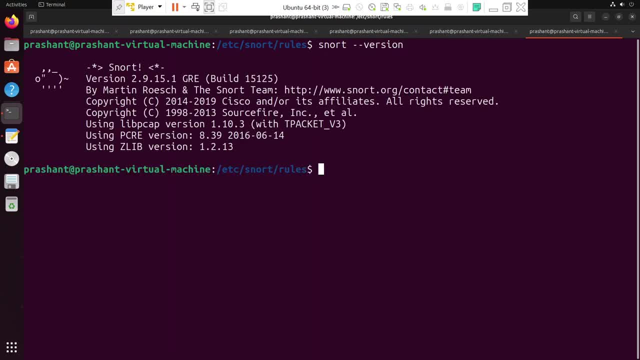 not can be installed. uh, like i have already installed the, already installed the. already installed the. it's not in my system. it's not in my system. it's not in my system, so it's not is installed in my system. so it's not is installed in my system. 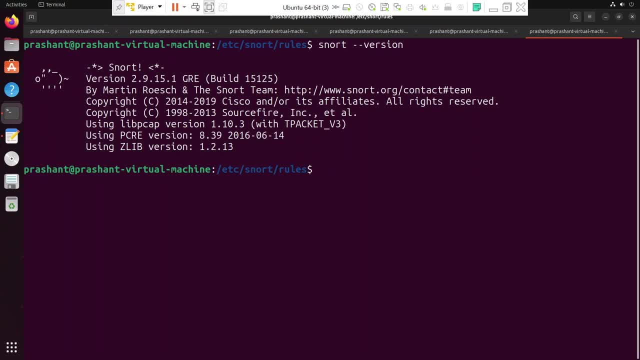 so it's not is installed in my system and what exactly is not is doing just, and what exactly is not is doing just, and what exactly is not is doing just. think of a scenario. think of a scenario. think of a scenario that. think of a scenario that, uh. 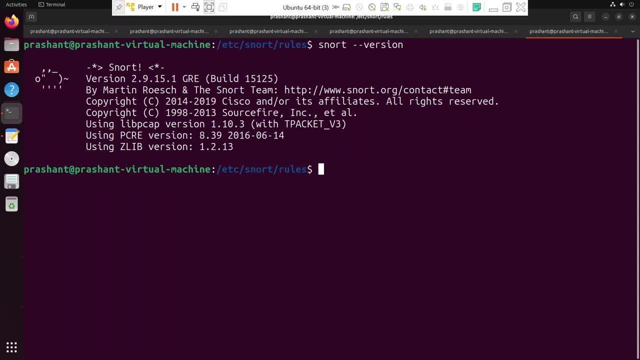 uh, uh, you have, you have. you have uh appliance on which you have installed uh appliance on which you have installed uh appliance on which you have installed this, not this, not this, not now. you want that if somebody ping you now. you want that if somebody ping you. 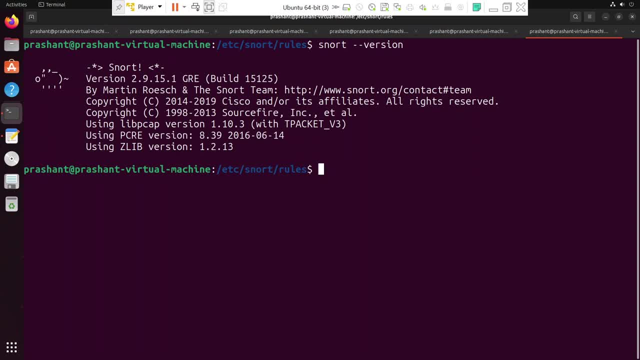 now you want that if somebody ping you, you will get an alert. you will get an alert. you will get an alert. understood what i'm trying to say. you understood what i'm trying to say. you understood what i'm trying to say. you want to want to. 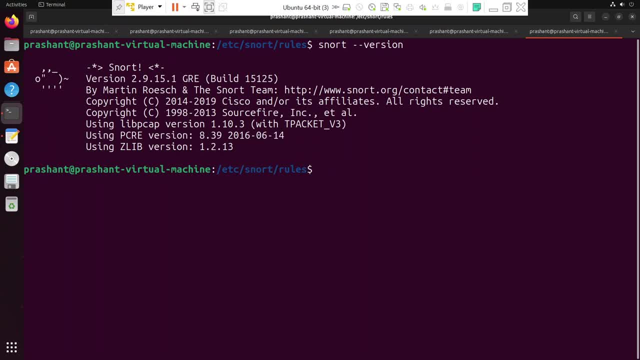 want to set up a scenario where if somebody set up a scenario where if somebody set up a scenario where if somebody ping you, ping you, ping you, you will get an alert. is it right? you will get an alert. is it right? you will get an alert. is it right? is it meaningful or not? 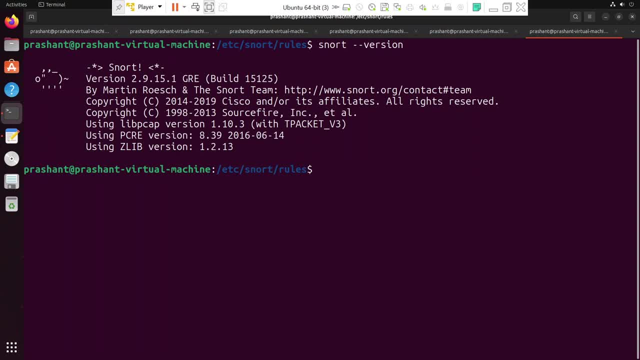 is it meaningful or not? is it meaningful or not if somebody is trying to ping you it? if somebody is trying to ping you it? if somebody is trying to ping you, it will make sense that he is doing the will make sense that he is doing the will make sense that he is doing the reconnaissance on you. 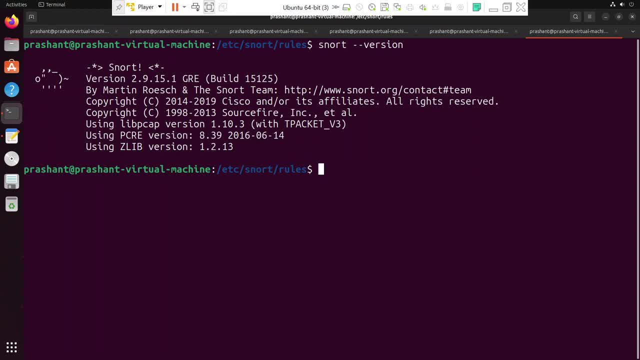 reconnaissance on you. reconnaissance on you, yeah, but sir, where will put this? uh, yeah, but sir, where will put this? uh, yeah, but sir, where will put this? uh system? uh, will it be after the router system? uh, will it be after the router system? uh, will it be after the router? we will put or where, or. 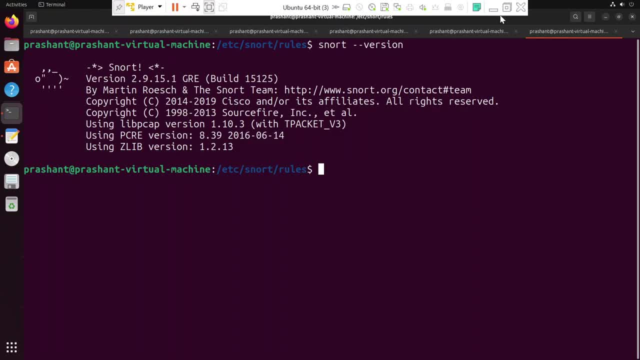 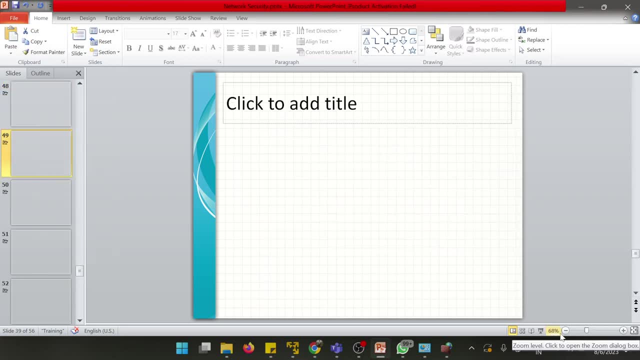 we will put, or where, or we will put, or where, or where, exactly where, exactly where exactly? it's not a something, it's not a something, it's not a something, and you can put, and you can put, and you can put. let me tell you one thing. 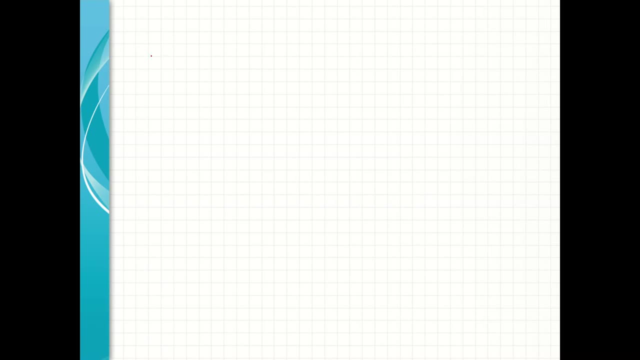 let me tell you one thing. let me tell you one thing: okay, this is a router. okay, this is a router. okay, this is a router. okay, this is your firewall, this is your firewall, this is your firewall, this is your code switch, this is your code switch, this is your code switch and this is your mz dmz. and then okay, 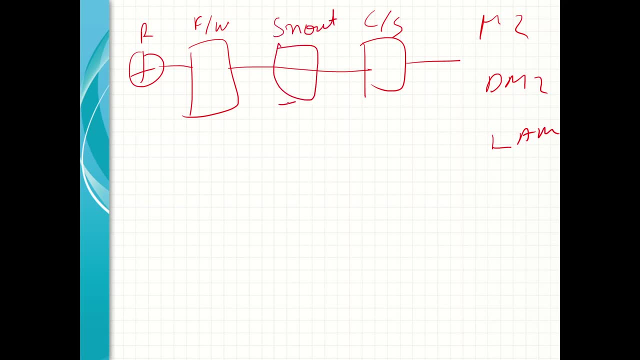 and this is your mz dmz, and then okay, and this is your mz dmz. and then, okay, you can put snot here also. you can put snot here also. you can put snot here also. when you put snot, it will work it as a. 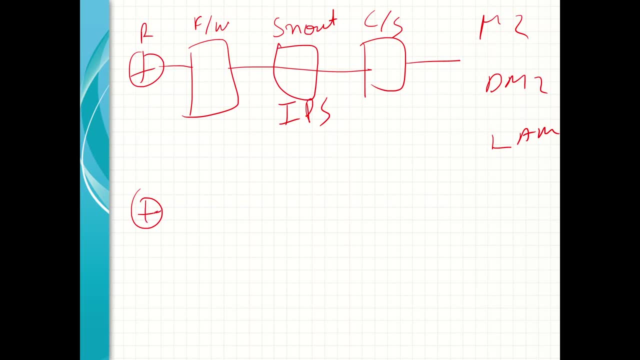 when you put snot, it will work it as a. when you put snot, it will work it as a ips, ips, ips, okay, okay, okay, okay, okay, okay. and when and when and when, when and when, when you put here in parallel to this, it will work as a. 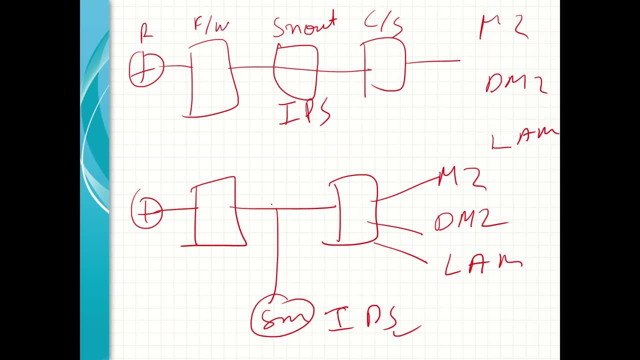 in parallel to this, it will work as a. in parallel to this, it will work as a: ideas, ideas, ideas, okay, okay, okay, mirror the topic and mirror the topic and mirror the topic, and you can wear means. this is a firewall. you can wear means. this is a firewall. 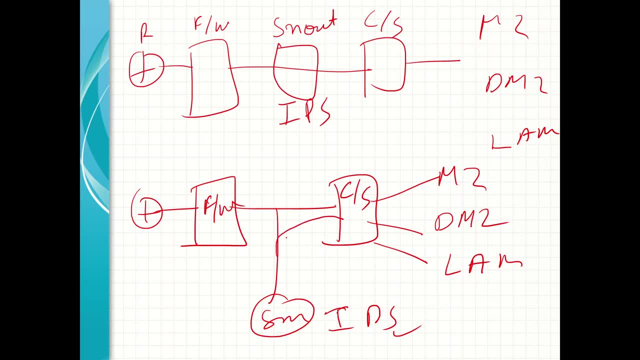 you can wear means. this is a firewall and this is a code switch, so you can and this is a code switch, so you can and this is a code switch, so you can directly connect through this to the, directly connect through this to the, directly connect through this to the code switch, or you can connect it to the. 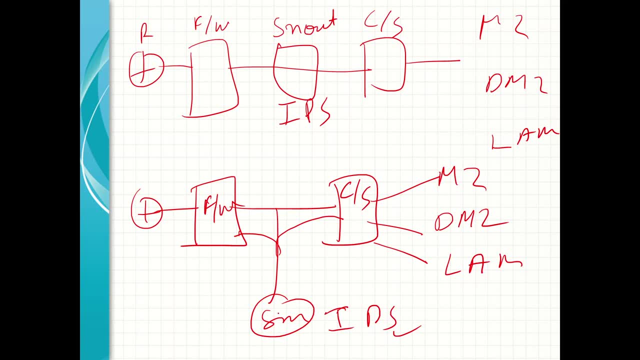 code switch. or you can connect it to the code switch or you can connect it to the firewall. so basically it is between the firewall, so basically it is between the firewall. so basically it is between the firewall and firewall and firewall and code switch, code switch, code switch. so we will be mirroring the traffic that. 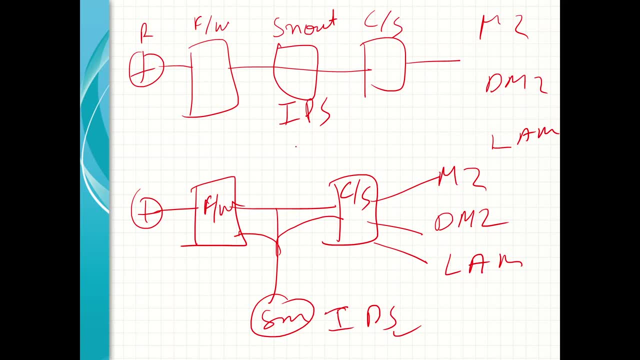 so we will be mirroring the traffic that. so we will be mirroring the traffic that is coming from the firewall to the core, is coming from the firewall to the core, is coming from the firewall to the core switch. yes, what we have to do, we have to. 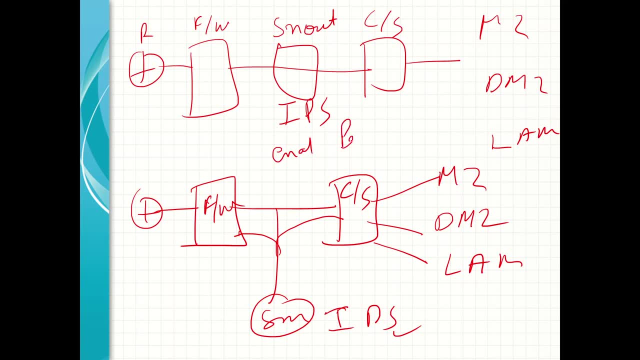 switch. yes, what we have to do. we have to switch. yes, what we have to do. we have to enable the uh, enable the uh, enable the uh port in the promiscuous mode, port in the promiscuous mode, port in the promiscuous mode. okay. 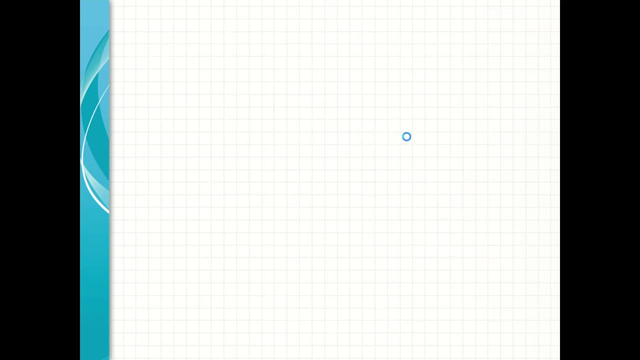 okay, okay, in the promiscuous mode, you need to. in the promiscuous mode, you need to. in the promiscuous mode, you need to. uh uh uh, allow it, allow it, allow it. okay, so we can install stores, not in our pc. so we can install stores, not in our pc. 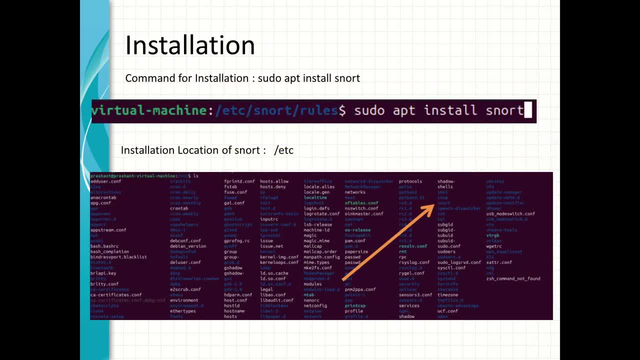 so we can install stores not in our pc as well, as well, as well. yes, this is installed in my pc only, so no, in the previous slide you were so. no in the previous slide, you were so. no, in the previous slide you were telling about the exact position we have. 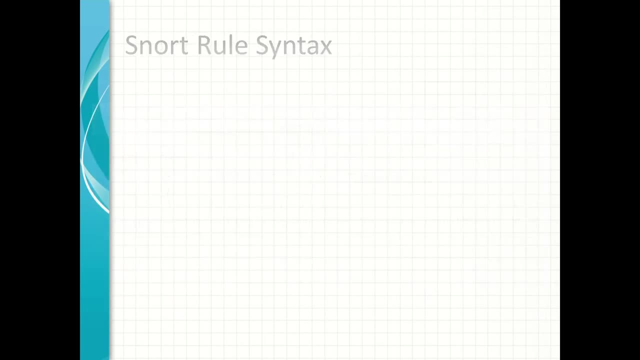 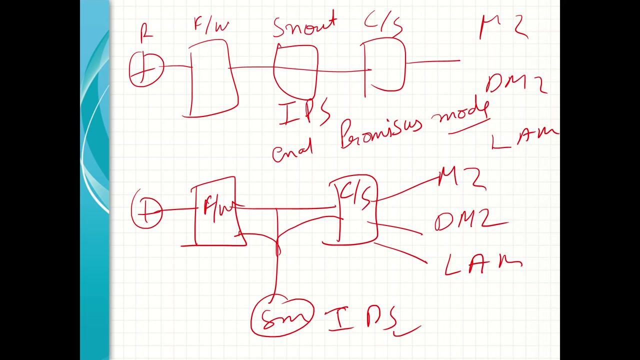 telling about the exact position we have, telling about the exact position we have to put this, note, this one: yeah, yes, yeah, definitely this one. yeah, yes, yeah, definitely this one. yeah, yes, yeah, definitely. end of the day, you have to install it's. end of the day, you have to install it's. 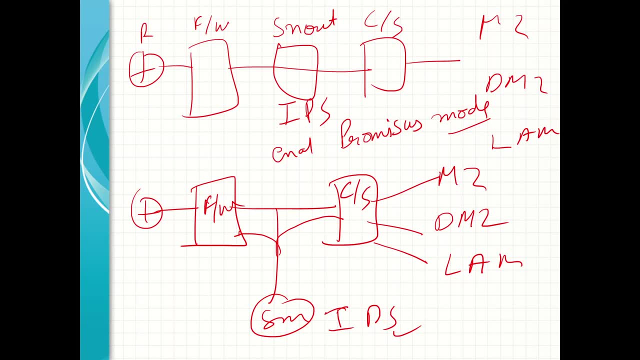 end of the day, you have to install. it's not on to the network on pc. what is the not on to the network on pc? what is the not on to the network on pc? what is the use, use, use, but for the testing and for the but for the testing and for the. 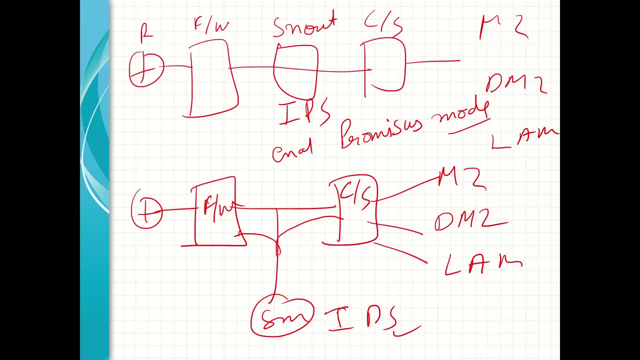 but for the testing and for the development purpose, to creating a rule development purpose, to creating a rule development purpose, to creating a rule testing. the rule you can put also in the testing, the rule you can put also in the testing, the rule you can put also in the in your pc. 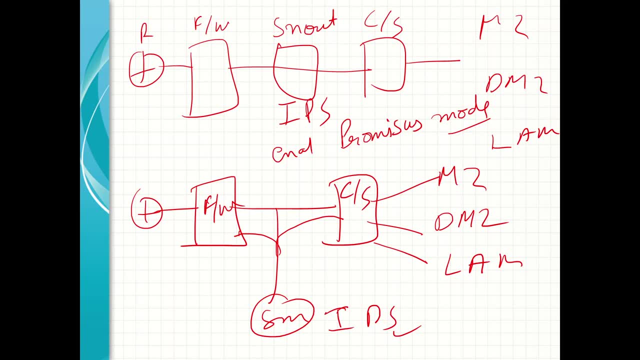 in your pc. in your pc, but like, if i want to teach you, it's not, but like, if i want to teach you, it's not, but like, if i want to teach you, it's not. so i have to install a virtual machine. so i have to install a virtual machine. 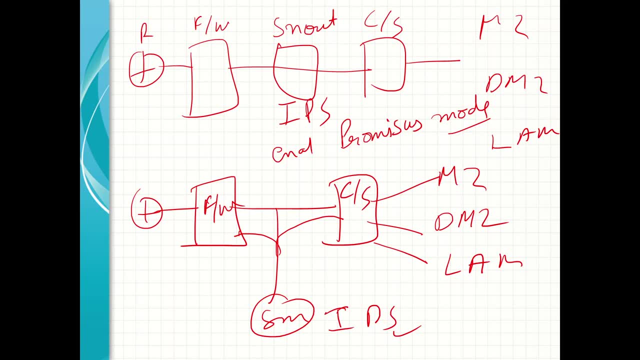 so i have to install a virtual machine, and on that virtual machine i need to, and on that virtual machine i need to, and on that virtual machine i need to install that it's not install, that it's not install, that it's not. but on the real life scenarios, this is: 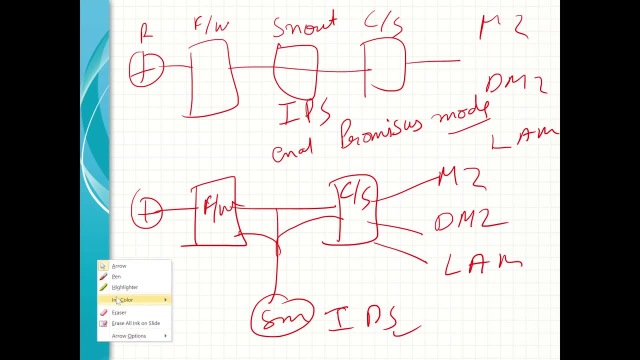 but on the real life scenarios, this is, but on the real life scenarios, this is the, the, the placement of the snort, and the best thing is: this is free, and, and the best thing is: this is free, and, and the best thing is: this is free and it is correct, and it is very much. 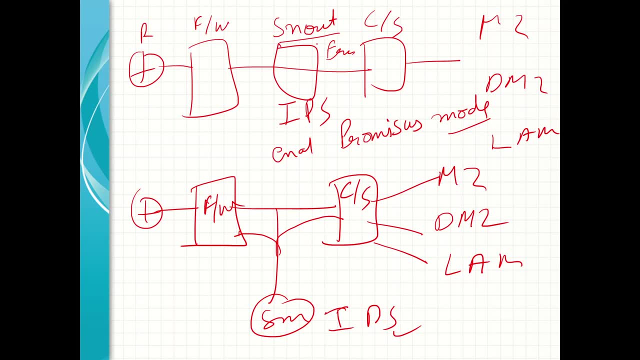 it is correct and it is very much it is correct and it is very much updated, like you can regularly update it, updated, like you can regularly update it, updated, like you can regularly update it, sir. i have a question, sir, when we are, sir, i have a question, sir, when we are. 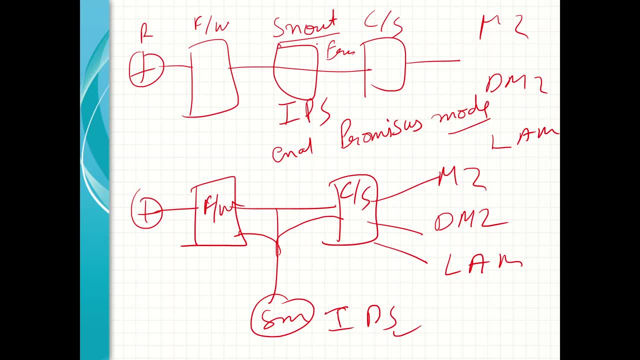 sir, i have a question, sir, when we are talking about this next gen firewall and talking about this next gen firewall and talking about this next gen firewall, and this ips and ids are the part of this, this ips and ids are the part of this. this ips and ids are the part of this feature means next gen viral feature. 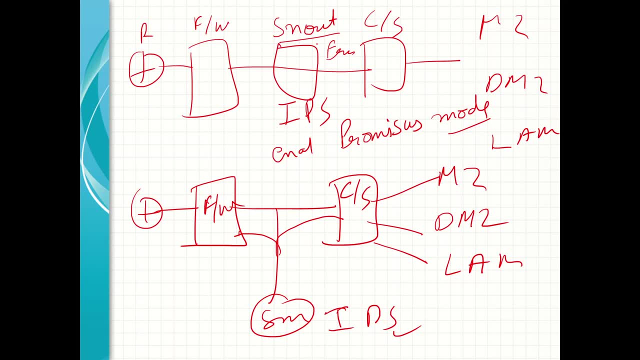 feature means next gen viral feature. feature means next gen viral feature. am i correct so this node will come in? am i correct so this node will come in? am i correct, so this node will come in? that next gen firewall or means how it? that next gen firewall or means how it? 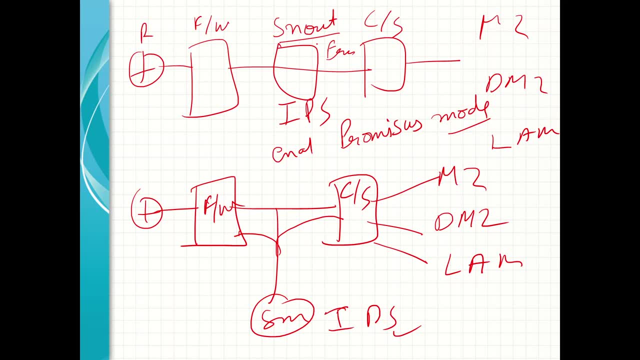 that next gen firewall or means how it will be separate. it will be separate. most will be separate. it will be separate. most will be separate. it will be separate most of the times of the times, of the times when you have a already next-gen firewall, when you have a already next-gen firewall. 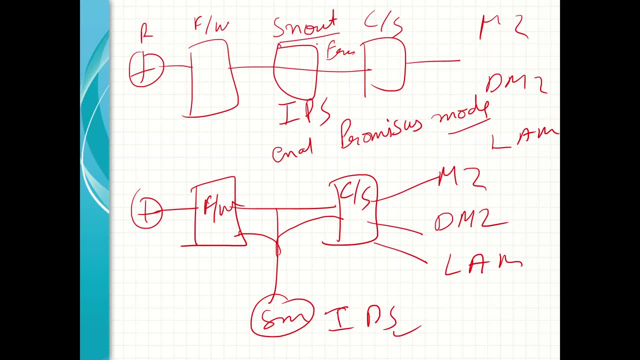 when you have a already next-gen firewall in your, in your, in your organization. you do not need. it's not organization, you do not need, it's not organization, you do not need. it's not okay. but if you want to monitor your ot, okay, but if you want to monitor your ot. 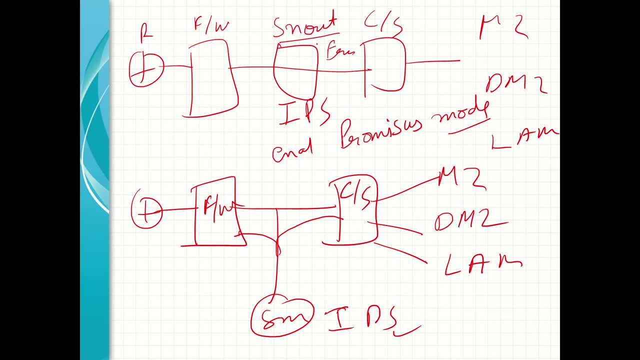 okay, but if you want to monitor your ot- environment, environment, environment- then in that case you can put down this. then in that case you can put down this, then in that case you can put down: this is not on a simple machine in your ot, is not on a simple machine in your ot. 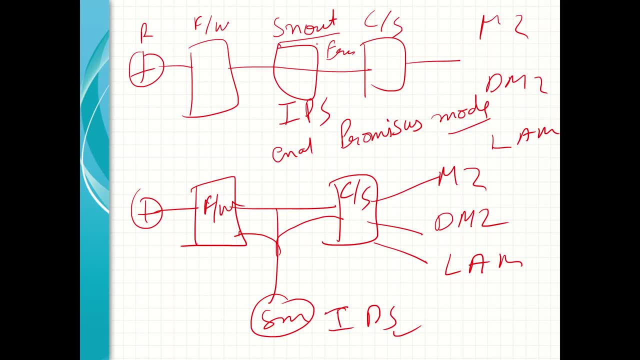 is not on a simple machine, in your ot environment, so that, in case of any environment, so that in case of any environment, so that, in case of any for the like monitoring of the network, for the like monitoring of the network, for the like monitoring of the network, you can use this node. 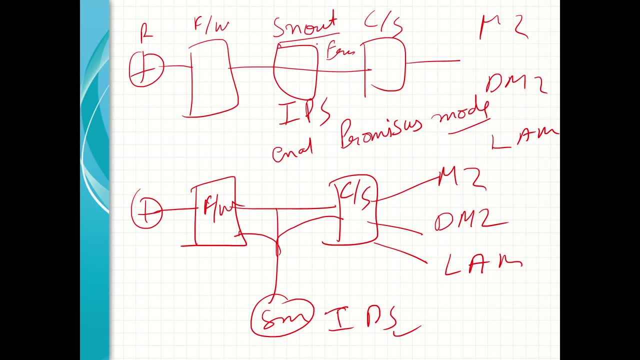 you can use this node. you can use this node. actually, this is a like. it is very actually. this is a like. it is very actually. this is a like. it is very important, to important, to important to talk about ips and ids uh on a separate. talk about ips and ids, uh on a separate. 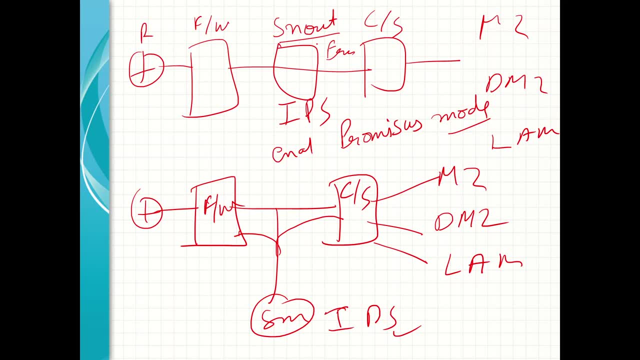 talk about ips and ids. uh, on a separate way. if i talk ips, ideas are the part of way. if i talk ips, ideas are the part of way. if i talk ips, ideas are the part of firewall, then it is of no use because firewall, then it is of no use because 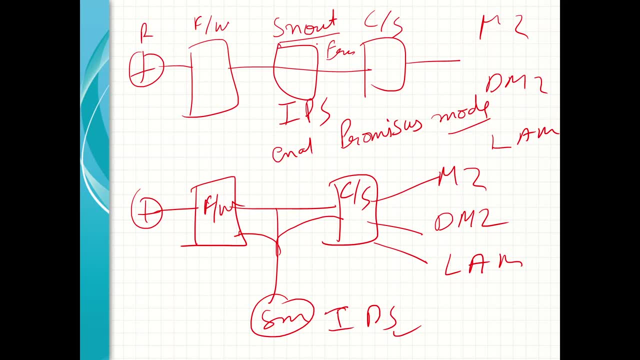 firewall, then it is of no use, because you can understand what is the work of. you can understand what is the work of you can understand what is the work of ips ideas. why i am talking you about ips ideas. why i am talking you about ips ideas. why i am talking you about snort? because snort is a 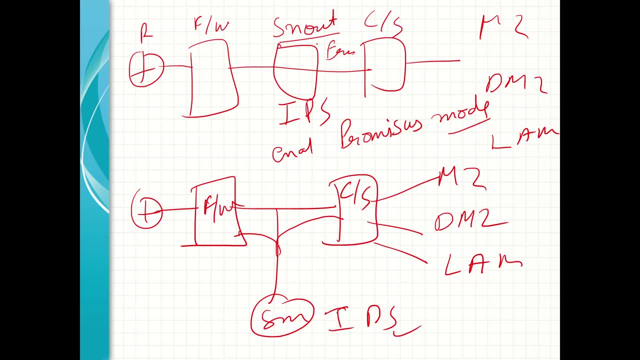 snort because snort is a snort, because snort is a. dedicatedly ips ids. dedicatedly ips ids. dedicatedly ips ids. okay sir, okay sir, okay sir, thank you, thank you, thank you, right, right, right, it's not can be treated as ips. it's not, can be treated as ips. 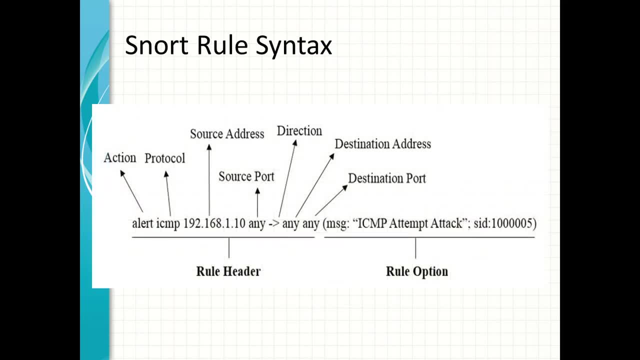 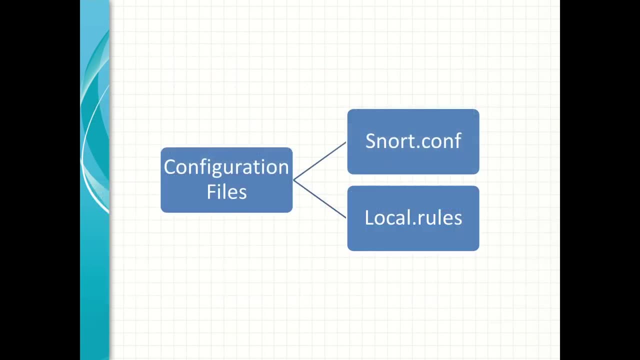 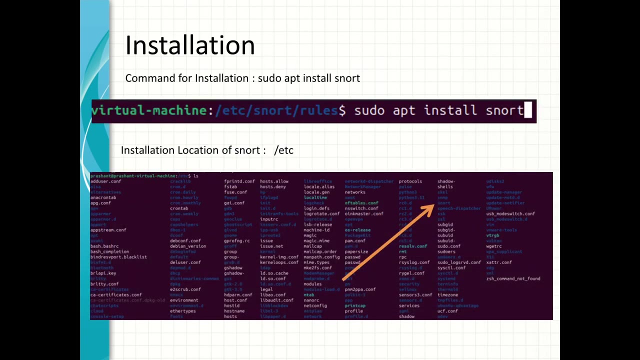 it's not, can be treated as ips because it can also block, because it can also block, because it can also block. you can see here, you can see here, you can see here what is not can do just a moment, just a moment, just a moment, sir, will we have a demonstration? 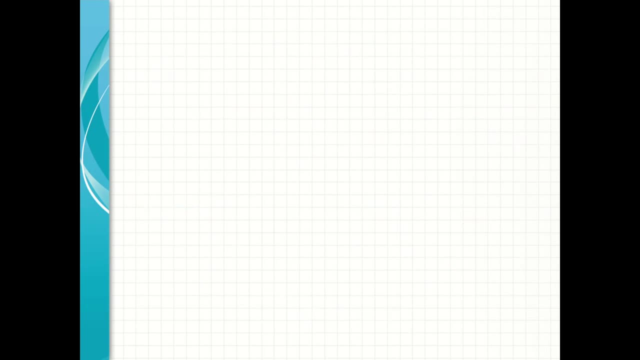 sir? will we have a demonstration, sir? will we have a demonstration? to set up snort on a virtual machine? to set up snort on a virtual machine. to set up snort on a virtual machine. yeah, i will be demonstrating, i'm just. yeah, i will be demonstrating, i'm just. 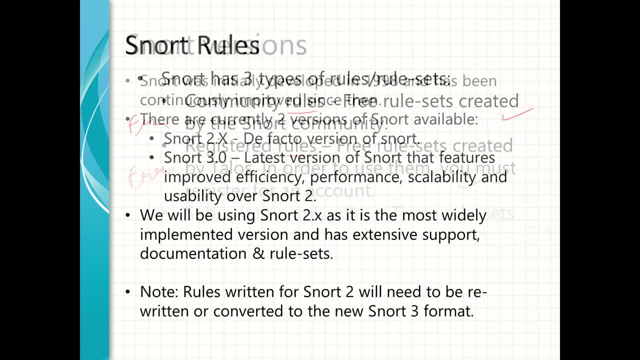 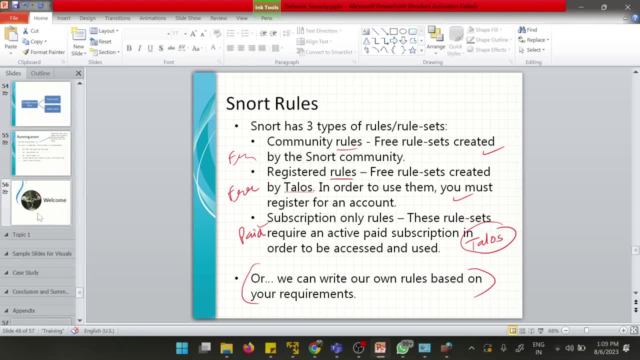 yeah, i will be demonstrating. i'm just telling you some important things. telling you some important things. telling you some important things. okay, let us demonstrate so that you have. okay, let us demonstrate so that you have. okay, let us demonstrate so that you have a better visibility to it. 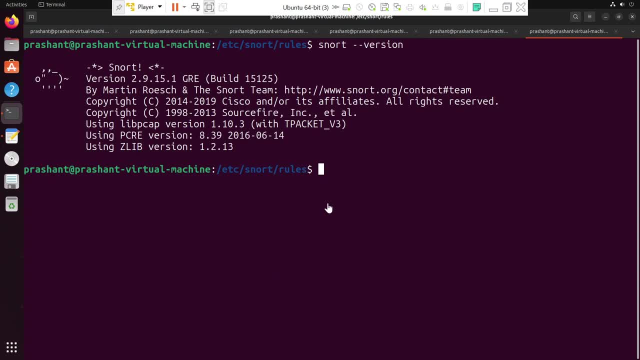 a better visibility to it. a better visibility to it. awesome you were telling about the. what awesome you were telling about the. what awesome you were telling about the. what snot can do. snot can do, snot can do. ah, snot can do. blocking also: snot can do. 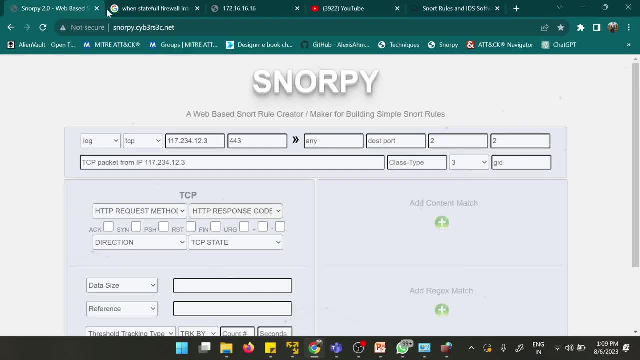 ah, snot can do, blocking also snot can do. ah, snot can do, blocking also snot can do. alert also alert also alert also actually, actually actually. so i have a question if it is so easy. so i have a question if it is so easy. 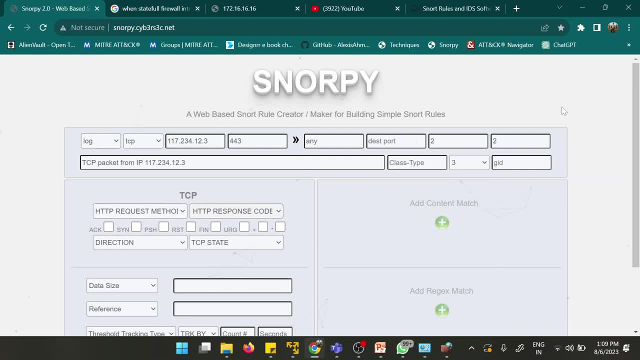 so i have a question: if it is so easy to install the snot it is going to detect, to install the snot it is going to detect, to install the snot it is going to detect and block and block and block the you know the attacks, then why does 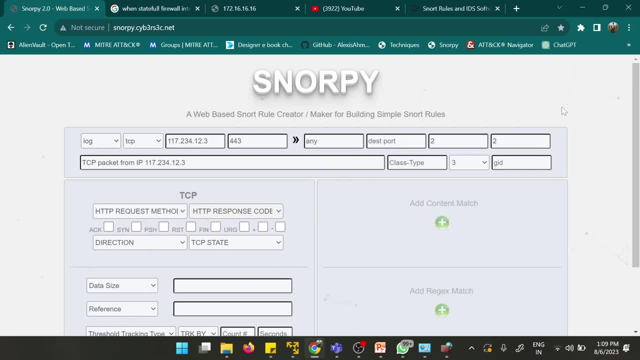 the you know the attacks, then why does the you know the attacks, then why does the attacks happen? suppose i write a, the attacks happen. suppose i write a, the attacks happen. suppose i write a program key: okay, if someone is pinging, program key. okay, if someone is pinging. 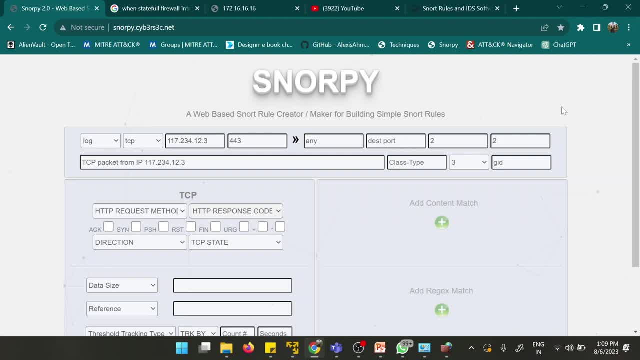 program key. okay, if someone is pinging my pc, my pc, my pc, it is generating an alert and blocking it is generating an alert and blocking. it is generating an alert and blocking that person, then why come there are so that person? then why come there are so? 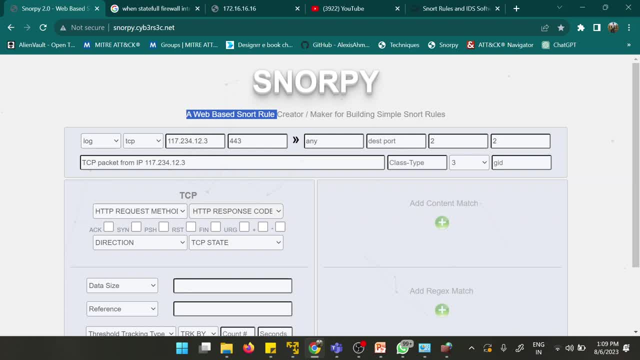 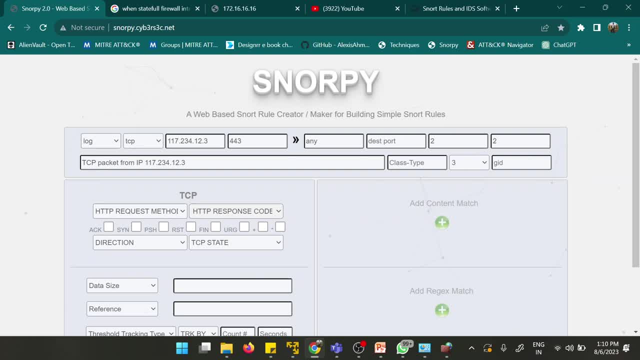 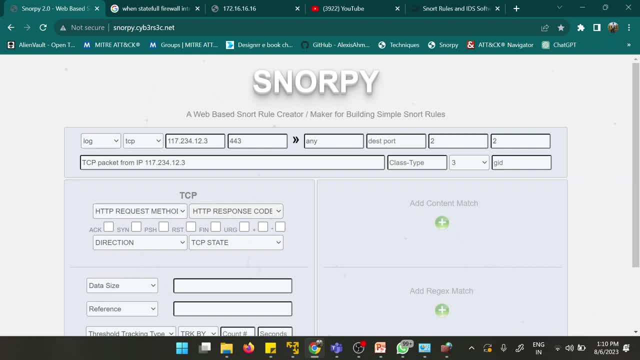 what i have always said in a lot of what i have always said in a lot of platform. i have all always saying platform. i have all always saying platform. i have all always saying: let these firewall vendors and these, let these firewall vendors and these, let these firewall vendors and these companies like cisco and all they are. 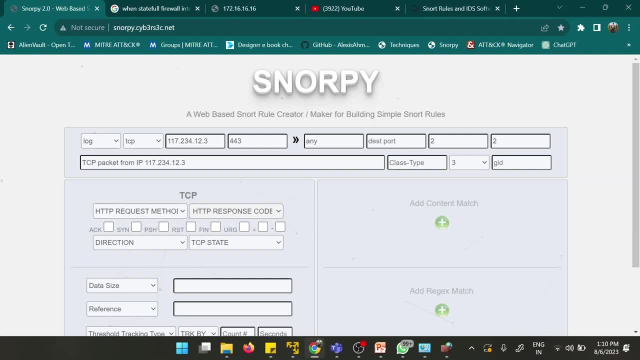 companies like cisco and all. they are companies like cisco and all. they are just selling their products on very high, just selling their products on very high, just selling their products on very high values. and if you are having a good values and if you are having a good 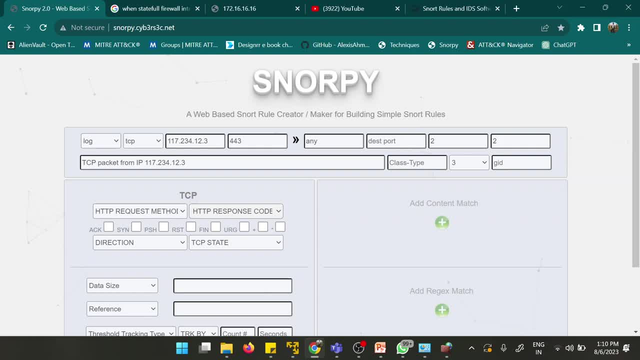 values and if you are having a good cyber security practitioner, you cyber security practitioner, you understand the concept. you can build your devices with these snort type tools which are free of cost. so buying i a firewall of 20 lakh rupees in comparison to this is a risky task, i would say. 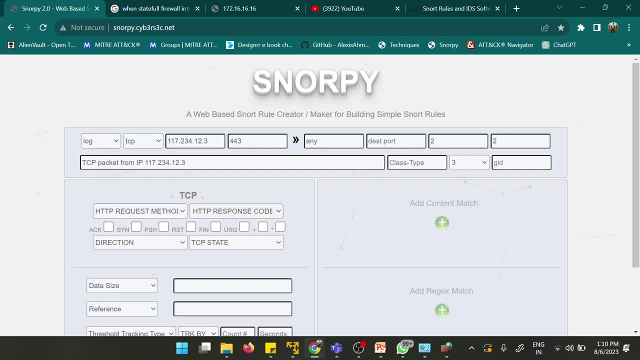 and you and basically the security is all about your efforts. putting a firewall will not help you, so putting a firewall and then configuring well is a good practice. somebody is also all already said that, sir, the configuration of firewall is very important. definitely, firewall configuration is very important. putting a firewall is not in solution provider. okay. 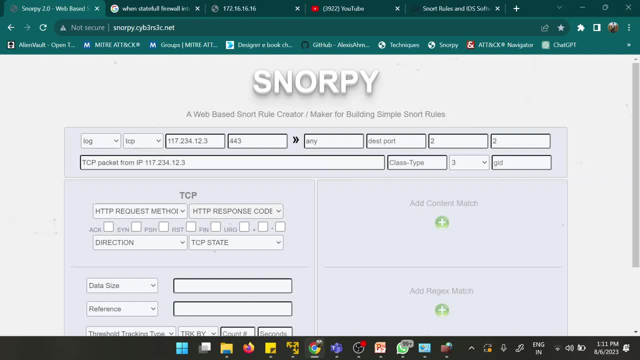 yeah, please, does this not be work on window uh platform or on linux only? no, no, it's not, will not work on window. it is for linux only, because you know the environment in power plant have normally a windows platform. but for network, for network, you can install it on. 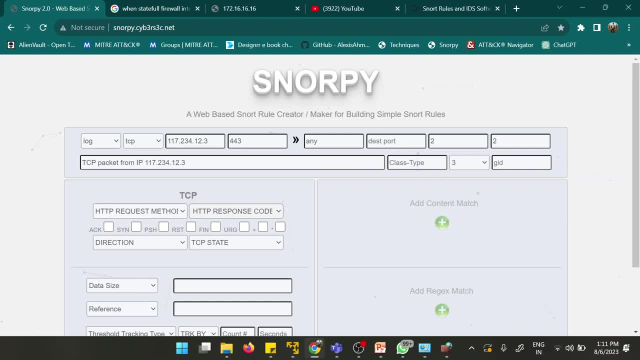 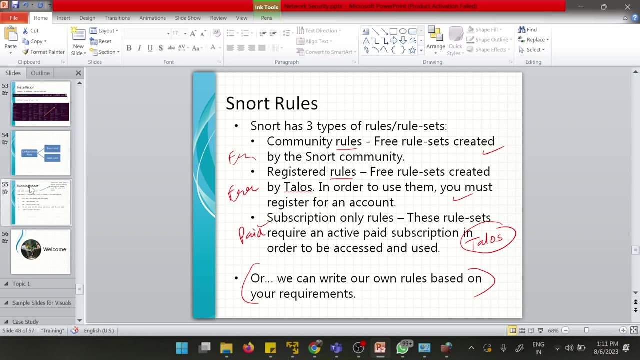 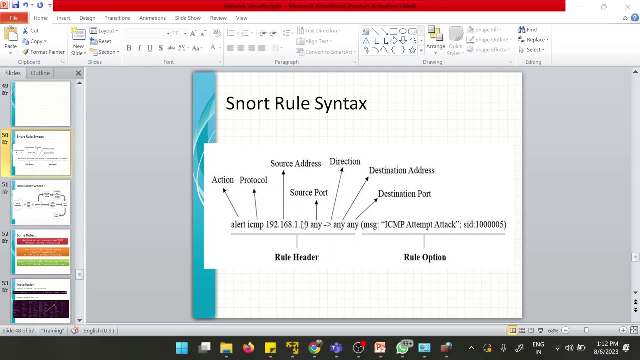 linux and that linux system can be put into your network. understood, yes, okay. so to understand the snort, we need to create some rules, okay, so this is a basic syntax for creating a rule. so what i'm telling you is what type of activities are not going to do? uh, it's not. can alert, it's not. can log. 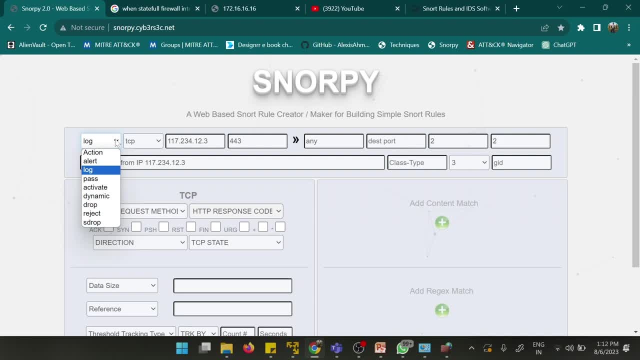 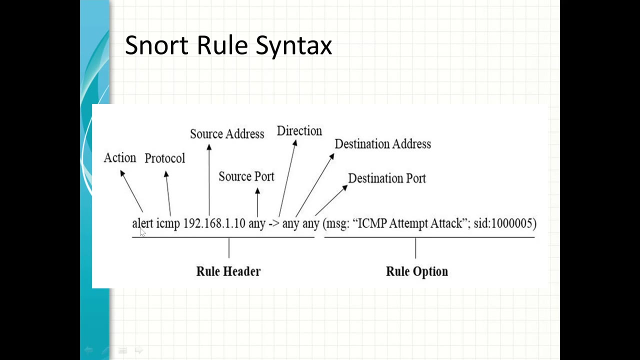 and it's not going to pass an activity. uh, it's not. can drop, reject the packet, okay. so let us see this first. it's not rule syntax, then we will go to snorpy, okay. so in this, this is a syntax where we will going to create a rule, as we have created in firewall. this is alert rule, okay. 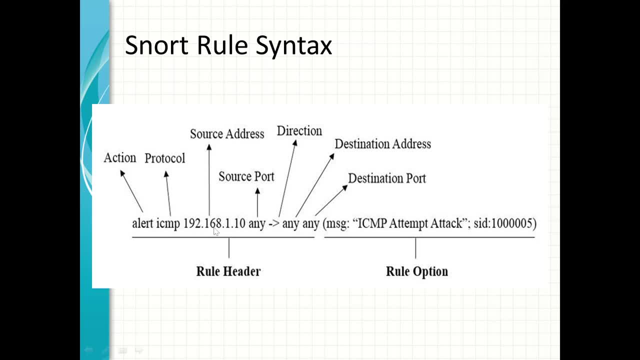 what protocol it will work. it will work for icmp. this is a source port, this is a source address. then this little direction, this the, and it will decide that for which direction this rule will work. for any destination and any destination port it is created, then it will create a message: icmp attack. 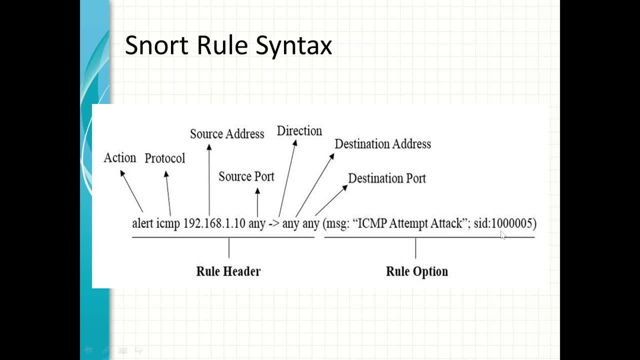 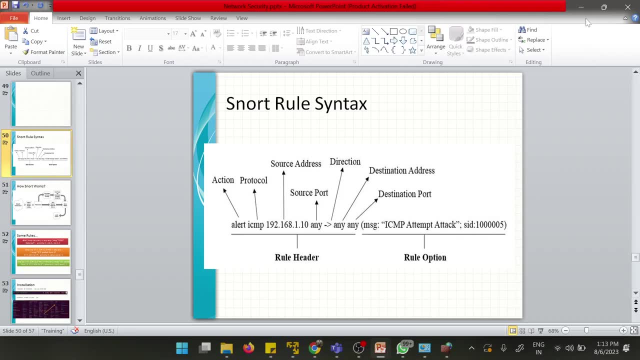 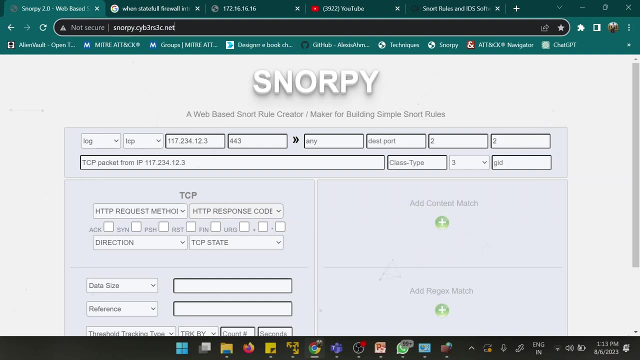 detected, then it will share. you have to write a sid number, serial id, for each and every rule, so now the thing is that creating these type of rules are very hard. so what the some people have done? they have created a website, snorpy it's norpy dot. this i will share. 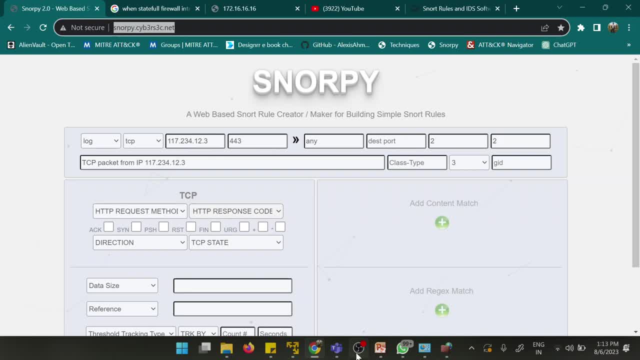 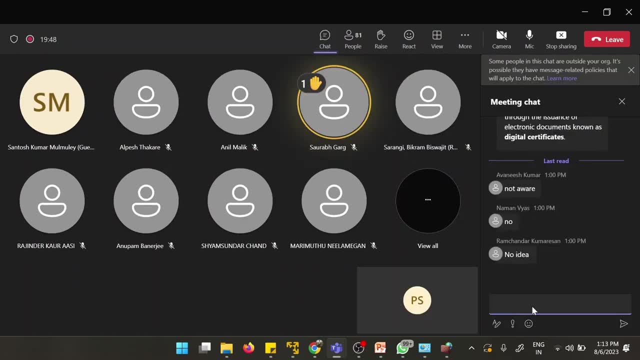 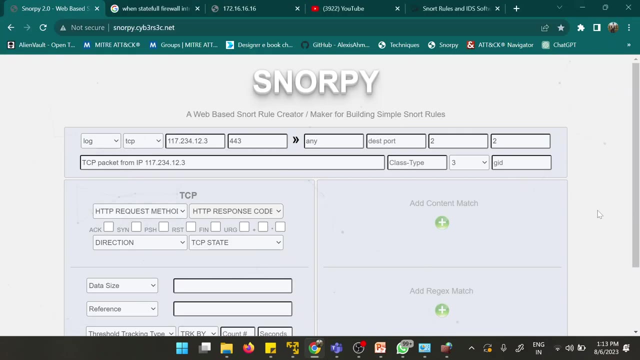 you this in the chat box so that you can: okay, now tell me, now work with me. you want to create a rule to block the icmp? okay, so what will? you will select alert, drop, reject s drop. tell me it's a drop alert. i want to create an alert if somebody ping me, i will. i, i will be getting an alert. 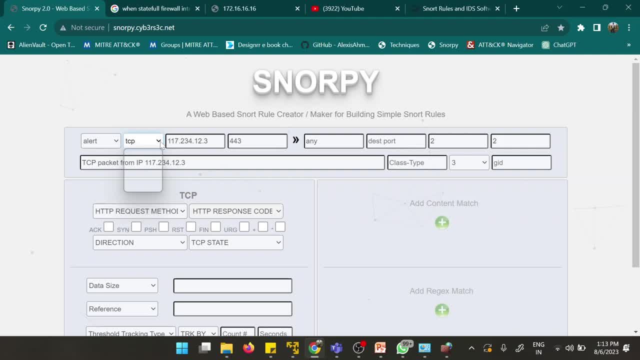 alert, alert. okay, pcp, sorry, icmp, okay, okay. so i am going to say for any source: if from anywhere, uh, icmp is coming, i should be, i should be alerted, okay. and for any ip address: uh, if my traffic is coming, it should be alerted. and then we have a sid number. let us suppose we give sid numbers one, zero one. 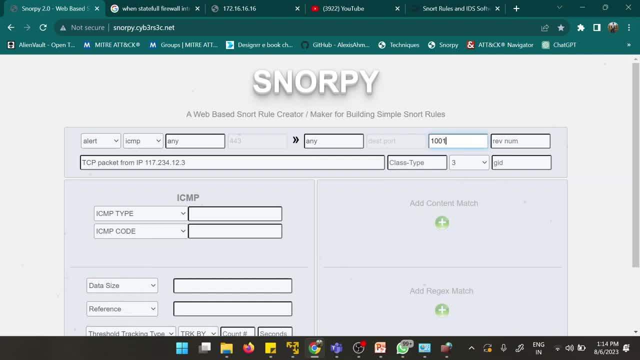 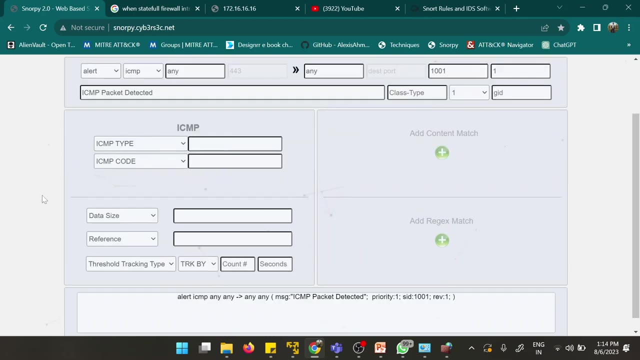 one, zero, zero one. then, where we have a revision number and then we have a priority for this. so the priority: we keep it as one and we create an alert message. icmp packet detected. okay, now it will automatically create a rule for snort. okay, also, if you want to say that, for data size. 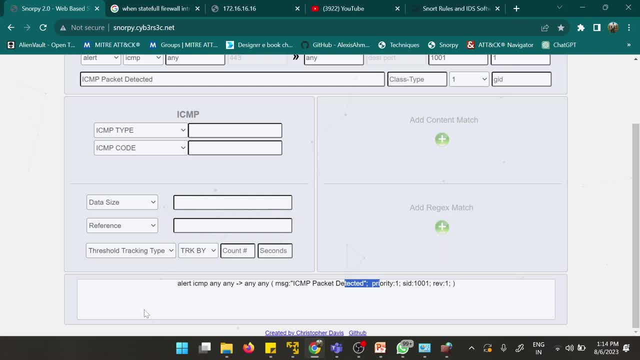 which is bigger than 16 bit. so it will create where d size is greater than 16 bit. okay, so this is the future very much, uh, it's. it's a very good website. you can create such type of rules. so this is a rule i have created that alert icmp from any to any where message is detected. now again, 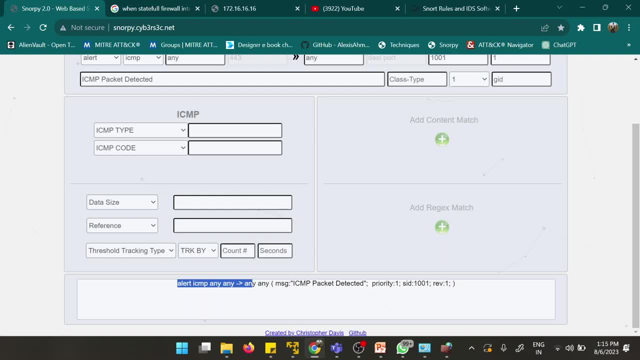 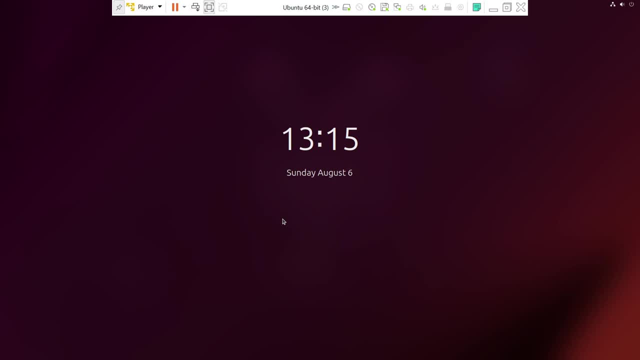 go back to the see, i am telling you on a very fast pace, this is not because it's not itself require at least like two hours for installation and for the deployment. and if you people want, i can take separate class on snort also. okay, sir, then how do we set up this virtual machine? and also 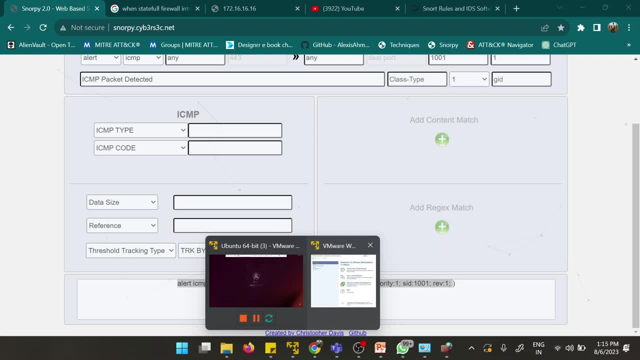 so i can take session on this, because this is now a very, very big topic actually. oh yes, but will it happen in the future classes? thousand one, the destination point, uh, destination port is for what actually you have defined. destination port is where i have defined in that. 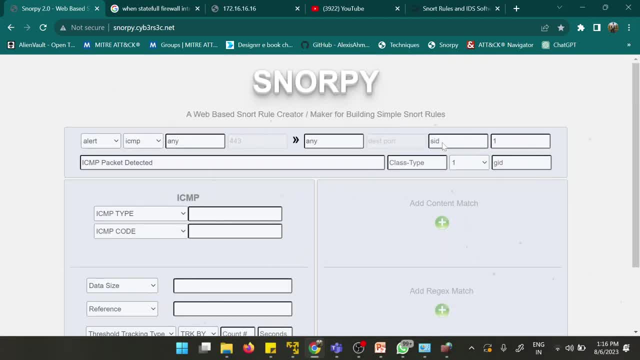 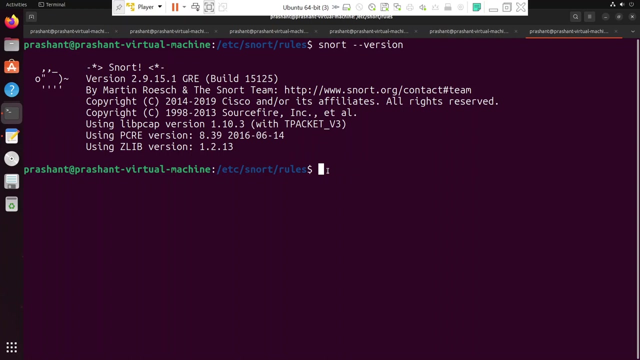 that rule 1001 is: yeah, yeah, this is like any, any number you can put, okay, okay, okay. so can you demonstrate like, yeah, i am demonstrating, i i want to show where the rule is written in the first. okay, so for this you need to find first the ip address of your own system. 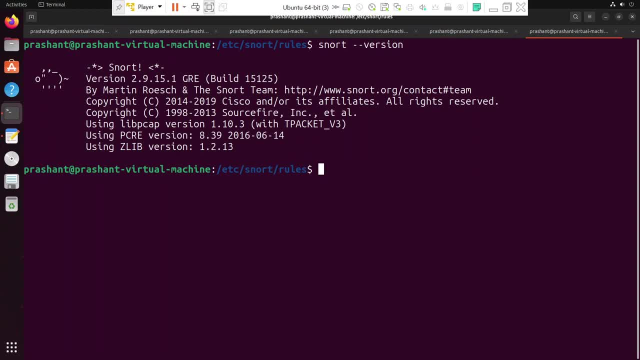 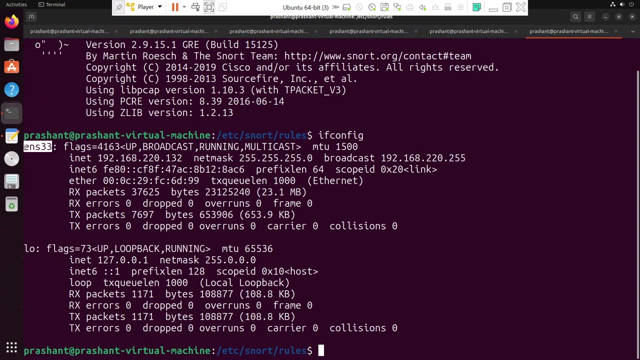 so my ip address is 192.168.222.132 and what is my network id name? ens33. okay, like in windows, you have ethernet 0, ethernet 1 in linux, we have, in ubuntu, ens33. okay, now i am going to see this rule and i am going to show you how to do it. okay, now i am going to see this rule. 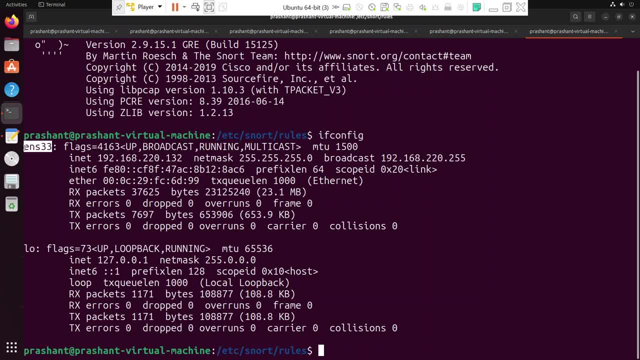 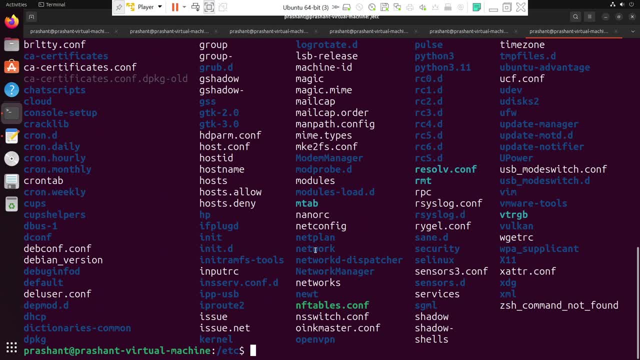 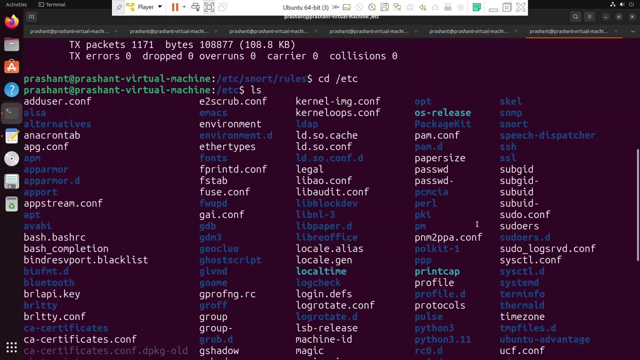 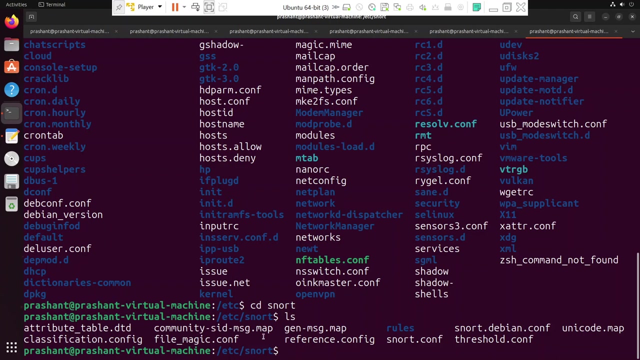 actually the snort is installed in which directory? cd in etc. directory. okay, you can see snort should should be there. you see it's not okay, so it's not. is in this directory after installation. and let me go to the snort directory. now we have two important files. one is a snortconf and other one is the is in the folder rules. 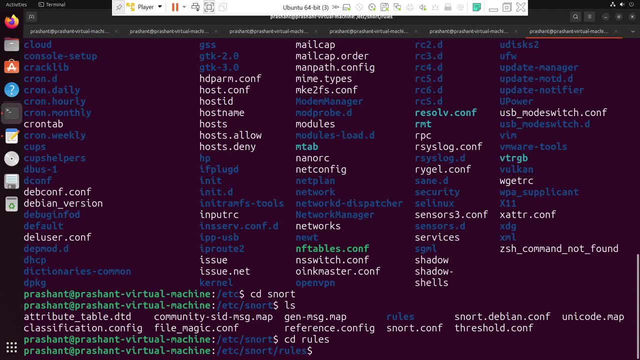 so the local rules is in rules folder, so this local dot rules is a main file, so let me open it. okay, so i have entered this rule that i have created using that. this is the same rule, yes or no? yes, yeah, that's why i've entered this rule. 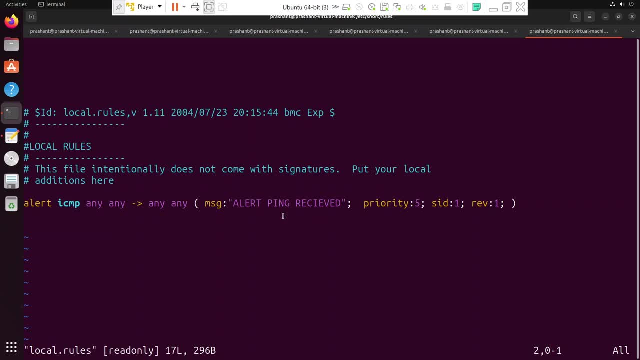 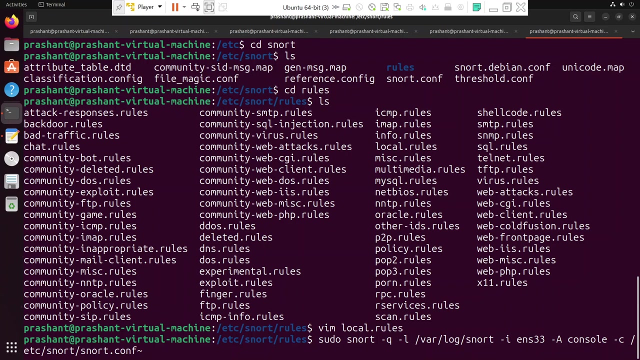 now i will smart start this node, why i put down pseudo. actually, sudo is like when you run a program in windows as an administrator in the same way to running a program in windows as an administrator in the same way to running a program is a beast. the soul boss ten and the living thing is whole done in one step or another. ran house, the best way to run. 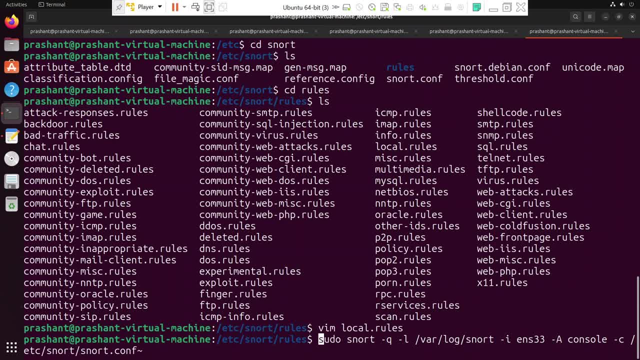 yeah, to run the program as an administrator, you use command sudo in linux. okay, so sudo is not. this will run dash. hyphen q means it will run in a silent mode, okay. hyphen l means the logs will be logged in this folder. hyphen i means the interface for monitoring is ens 33, hyphen a. 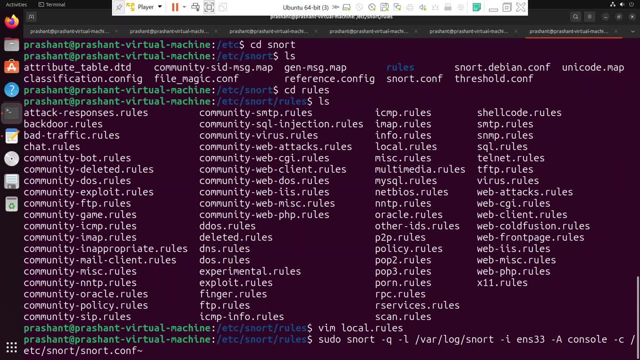 means what type of display is required. so i am using a console display. hyphen c means which configuration file is required. okay, so in this way my snort is running, but before that i need to copy my local ip. can somebody write this local ip in chat box so that i can refer later on? 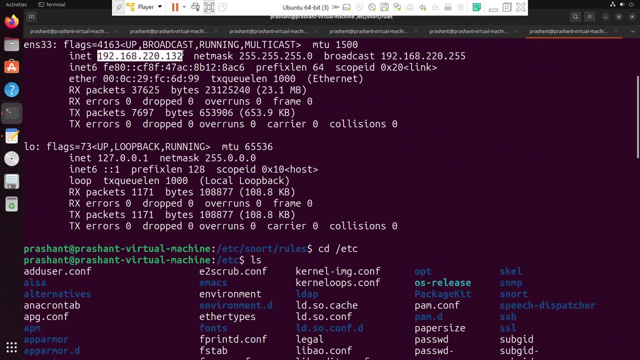 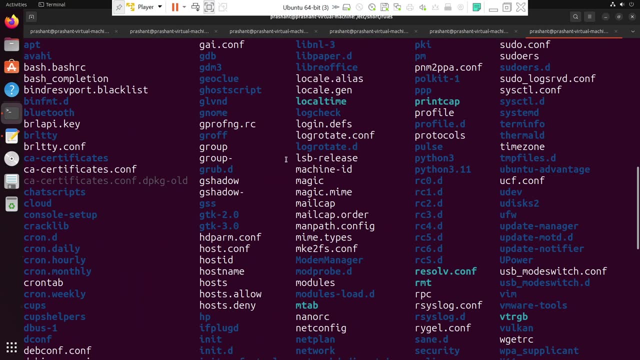 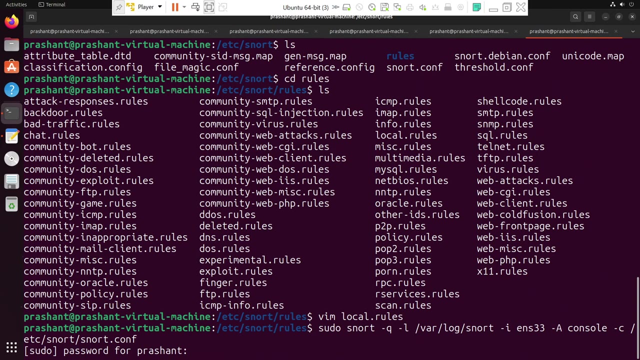 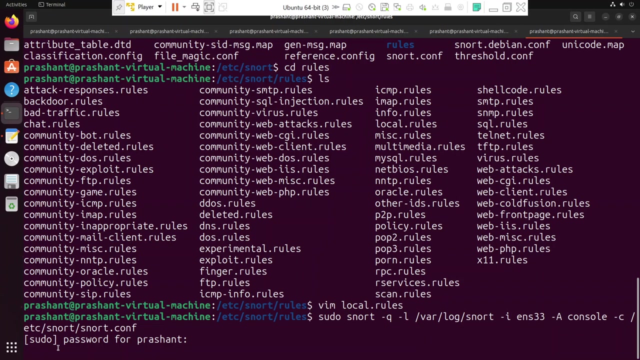 just write this type in chat box, because we required it later on. great, thank you. i will ask for a password. so now my snort is running. if no error is shown, it means snort is running. now let me go to my windows machine and now again ping this. 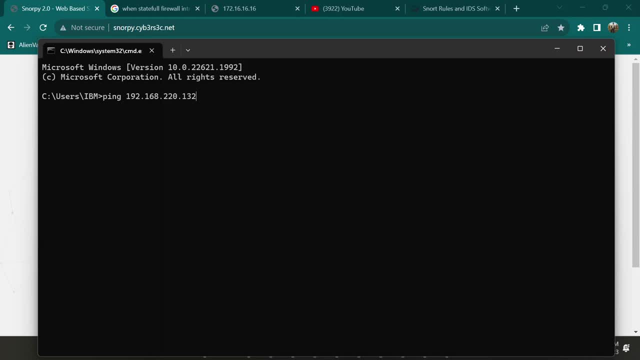 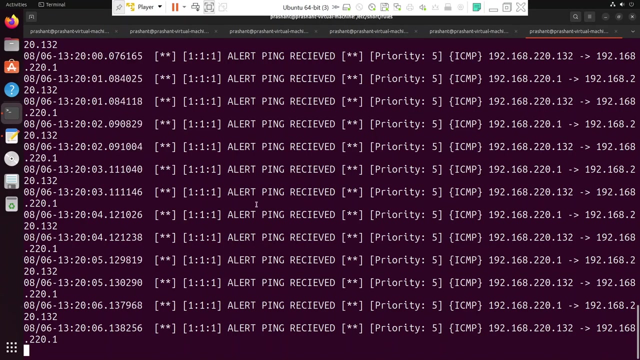 password, you can see alerts are started coming. it is visible and it is showing from which uh IP's alerts are coming. okay, let me stop this not feeding how i found it. you can go to your swarm in the platform and here this is showing name: your account. its name are ppl. 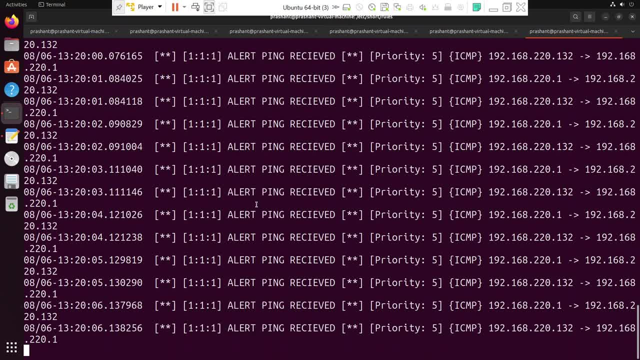 ok, let me paste that by anything that i put next, let me write: Win. Now it is stopped, stopped, yes or no? yes sir, yes sir, let me start again. let me start again. it again started coming. so I have stopped the SNOT. let me stop the pinging. 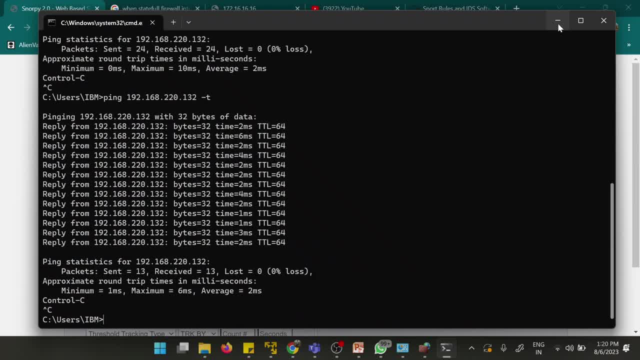 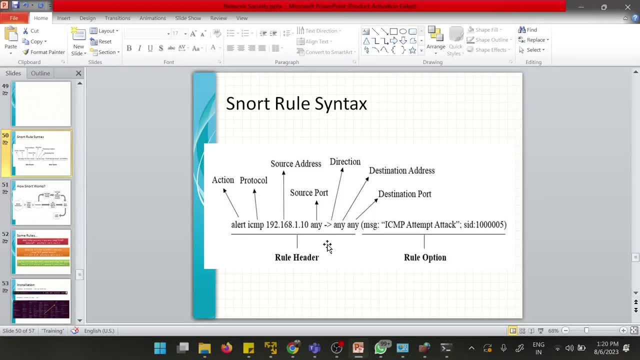 stop the pinging. so this is the way how you can set up a SNOT and these are the rules. you can take use of that Snorpy to create the rules. so this is like a very basic and very wonderful tool you have into an environment to set up such important things. okay. 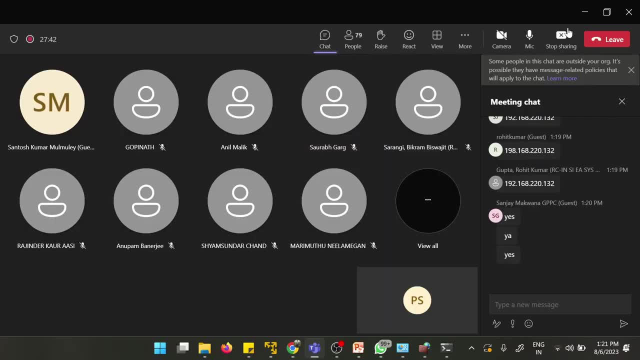 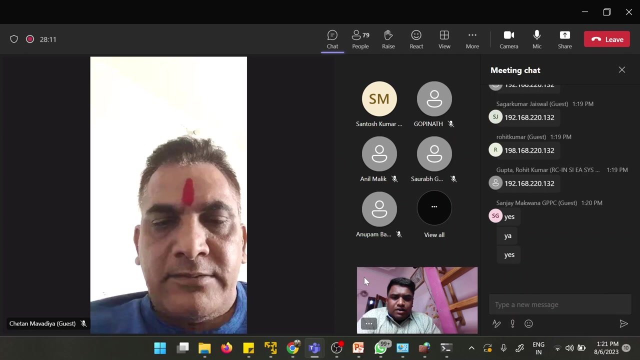 Okay, So am I visible? yes, sir, sir. so this is like today's end of session. so this is today's end of session and we have tried to cover out maximum things that you people required in your routine cyber security. I have tried to cover and make you people explain on a very practical way. I have tried.